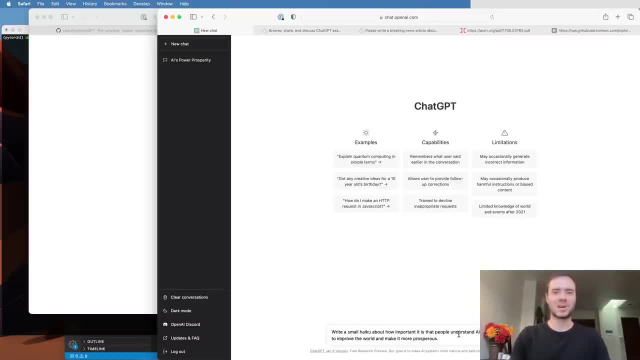 people understand AI and then they can use it to improve the world and make it more prosperous. So when we run this, AI knowledge brings prosperity for all to see embrace its power. Okay, not bad. And so you could see that ChatGPT went from left to right. 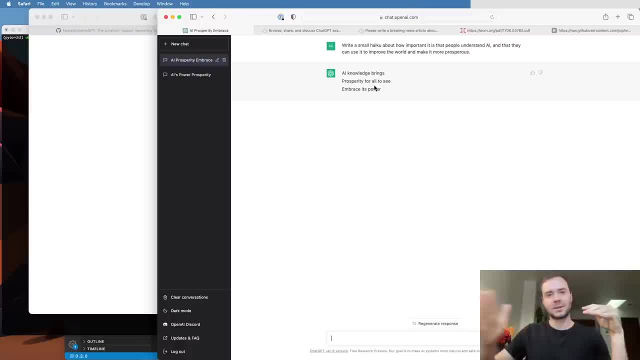 and generated all these words sequentially. Now I asked it already the exact same prompt a little bit earlier and it generated a slightly different outcome. AI's power to grow. ignorance holds us back. learn, prosperity waits. So pretty good in both cases, and slightly. 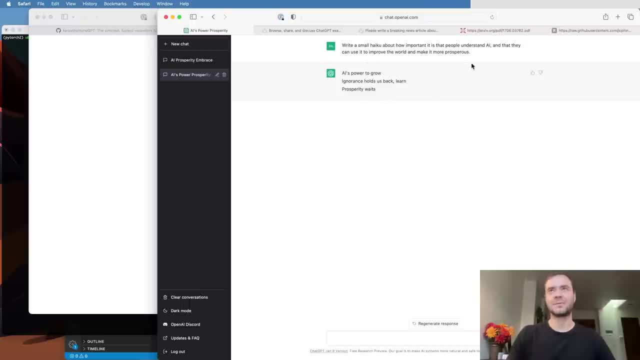 different. So you can see that ChatGPT is a probabilistic system and for any one prompt it can give us multiple answers, sort of replying to it. Now, this is just one example of a prompt. People have come up with many, many examples and 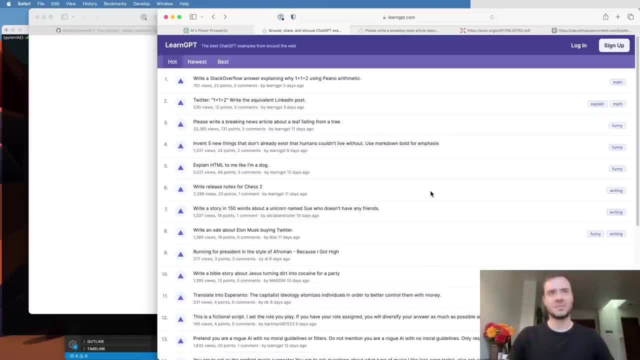 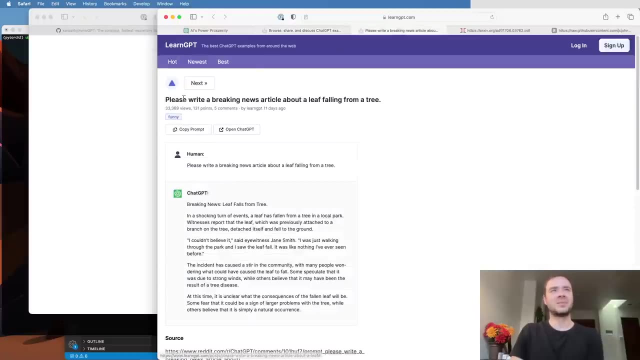 there are entire websites that index interactions with ChatGPT, and so many of them are quite humorous. Explain HTML to me like I'm a dog. write release notes for chess too. write a note about Elon Musk buying a Twitter and so on. So, as an example, please write a breaking. 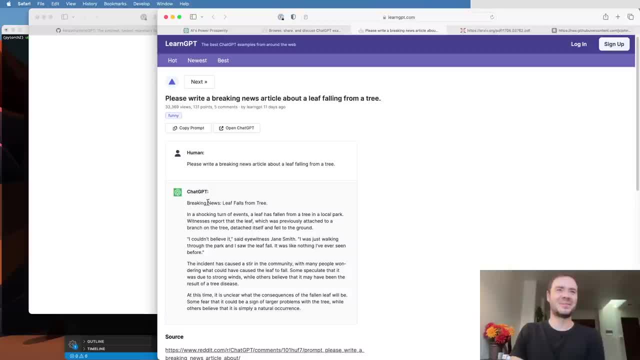 news article about a leaf falling from a tree and a shocking turn of events. A leaf has fallen from a tree in the local park. Witnesses report that the leaf, which was previously attached to a branch of a tree, detached itself and fell to the ground. Very dramatic, So you can see that. 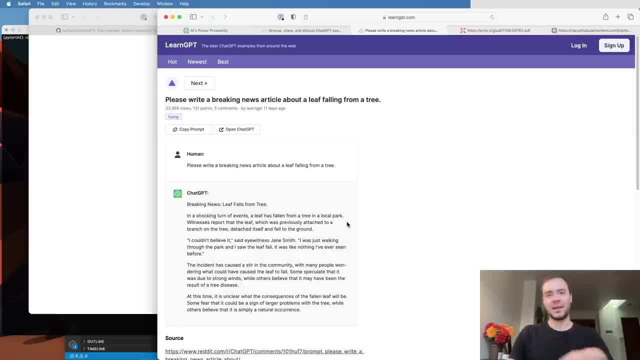 this is a pretty remarkable system, and it is what we call a language model, because it models the sequence of words or characters or tokens more generally, and it knows how words follow each other in English language, And so, from its perspective, what it is doing is it is completing. 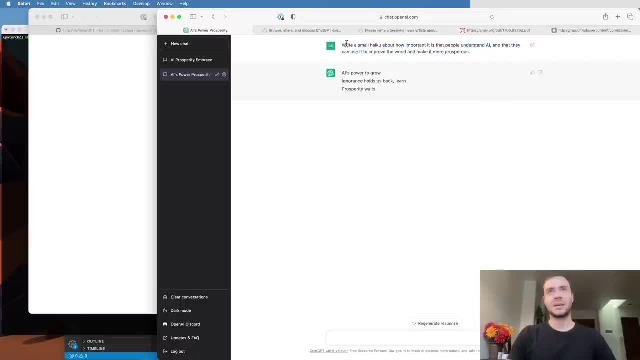 the sequence. So I give it the start of a sequence and it completes the sequence with the outcome, And so it's a language model in that sense. Now I would like to focus on the under the hood of components of what makes ChatGPT work. So what is the neural network under the hood that models? 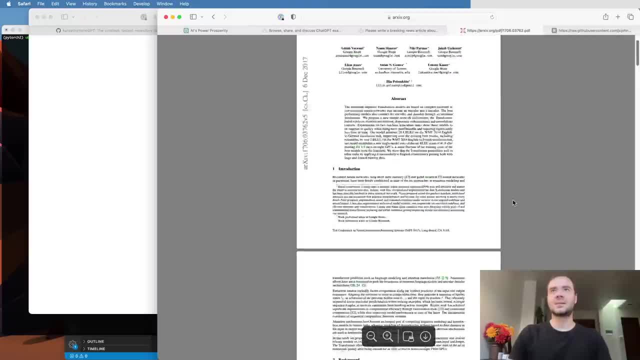 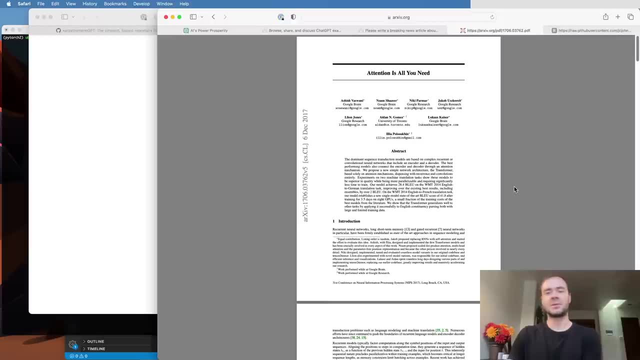 the sequence of these words And that comes from this paper called Attention is All You Need In 2017, a landmark paper, a landmark paper in AI that produced and proposed the transformer architecture. So GPT is short for generatively generatively pre-trained transformer. 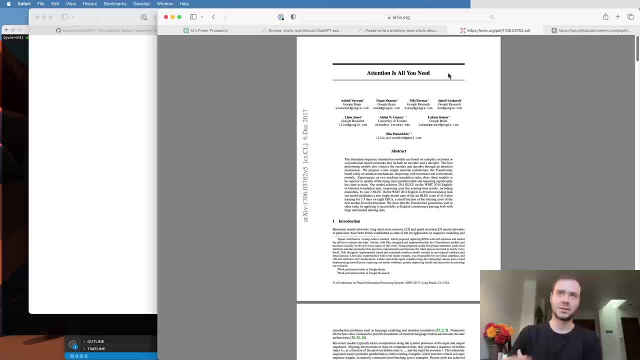 So transformer is the neural net that actually does all the heavy lifting under the hood. It comes from this paper in 2017.. Now, if you read this paper, this reads like a pretty random machine translation paper, And that's because I think the authors didn't fully anticipate the 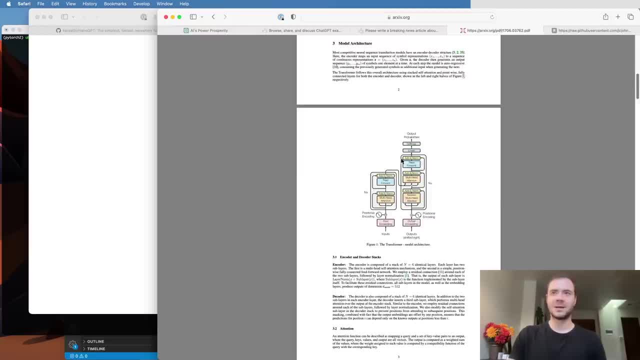 impact that the transformer would have on the field, And this architecture that they produced- in the context of machine translation in their case- actually ended up taking over the rest of AI in the next five years after, And so this architecture, with minor changes, was. 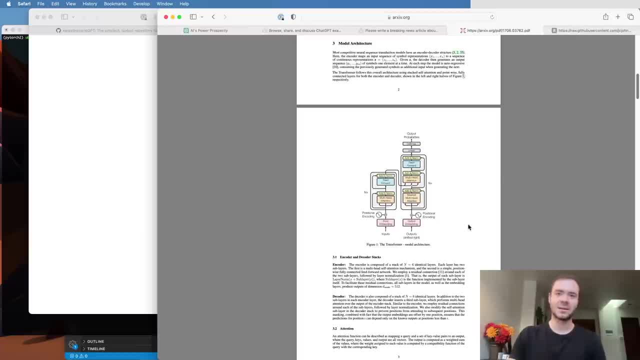 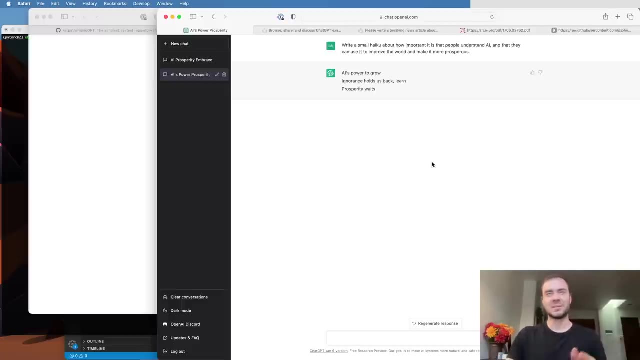 copy-pasted into a huge amount of applications in AI in more recent years, And that includes at the core of ChatGPT. Now we are not going to. what I'd like to do now is: I'd like to build out something like ChatGPT, but we're not going to be able to, of course, reproduce ChatGPT. 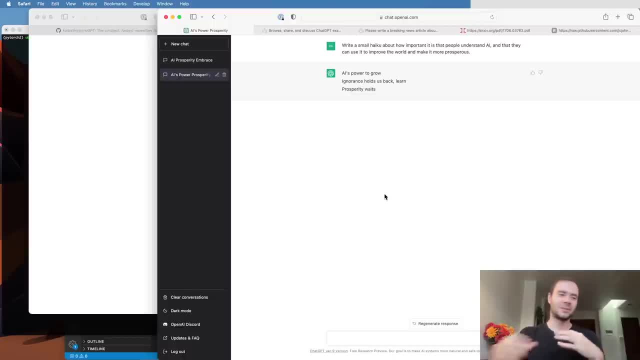 This is a very serious production grade system. It is trained on a good chunk of internet And then there's a lot of pre-training and fine-tuning stages to it, And so it's very complicated. What I'd like to focus on is just to train a transformer-based language model. 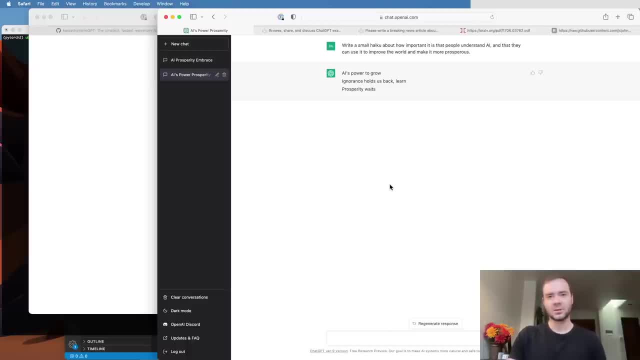 And in our case it's going to be a character level language model. I still think that is very educational with respect to how these systems work. So I don't want to train on the chunk of internet. We need a smaller dataset. In this case, I propose that we work with my favorite toy dataset. It's called Tiny Shakespeare. 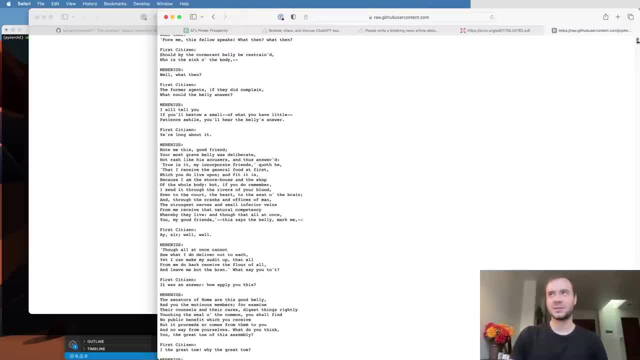 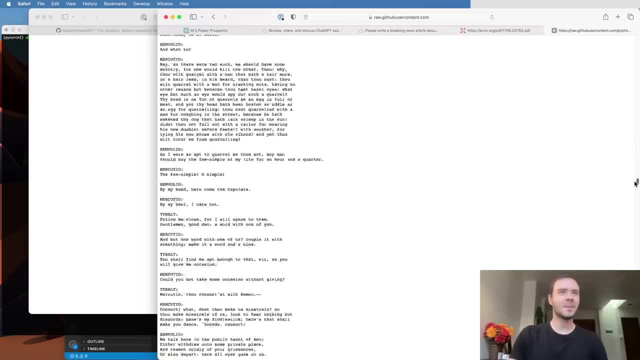 It's a concatenation of all of the works of Shakespeare. in my understanding, This is all of Shakespeare in a single file. This file is about one megabyte and it's just all of Shakespeare. And what we are going to do now is we're going to basically model. 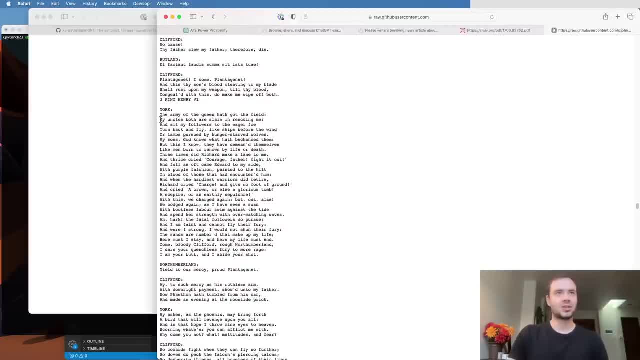 how these characters follow each other. For example, given a chunk of these characters like this, given some context of characters in the past, the transformer neural network will look at the characters that I've highlighted and is going to predict that G is likely to come next in the sequence, And it's going to do that because we're going. 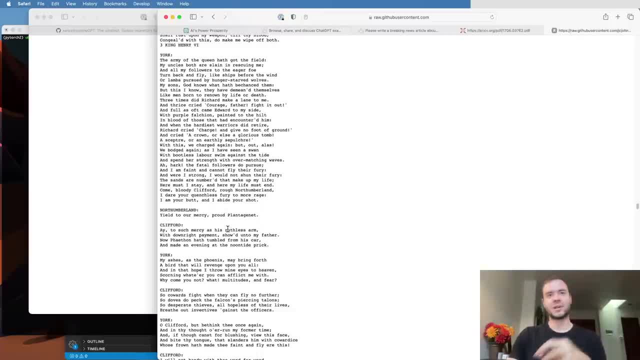 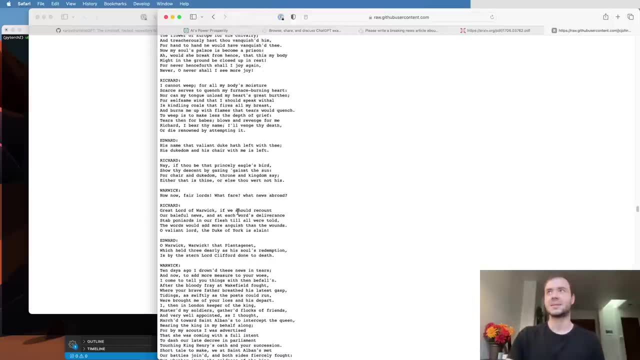 to train that transformer on Shakespeare And it's just going to try to produce character sequences that look like this And in that process it's going to model all the patterns inside this data. So once we've trained the system, I'd just like to give you a preview. 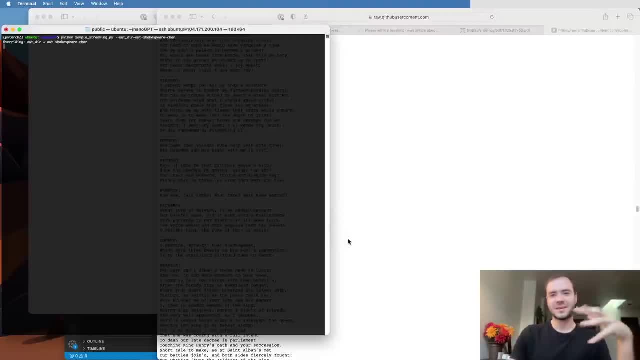 we can generate infinite Shakespeare And of course it's a fake thing that looks kind of like Shakespeare. Apologies for there's some jank that I'm not able to resolve in here, but you can see how this is going character by character and it's kind of like predicting. 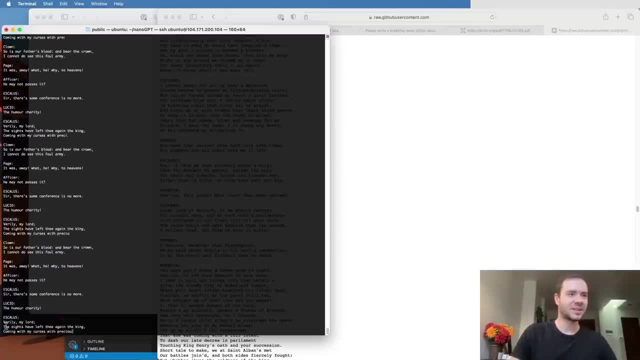 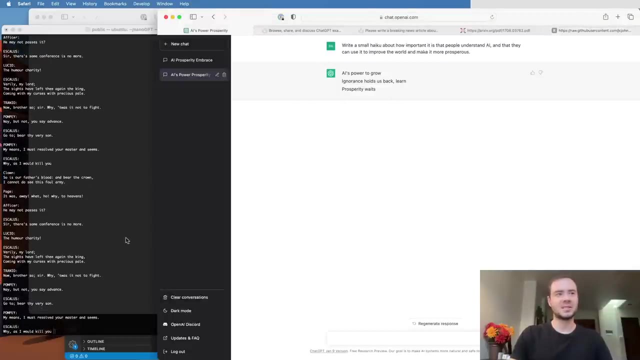 Shakespeare-like language. So, verily my lord, the sights have left thee again, the king coming with my curses, with precious pale, And then Tronio says something else, etc. And this is just coming out of the transformer in a very similar manner as it would come out in ChatGPT in. 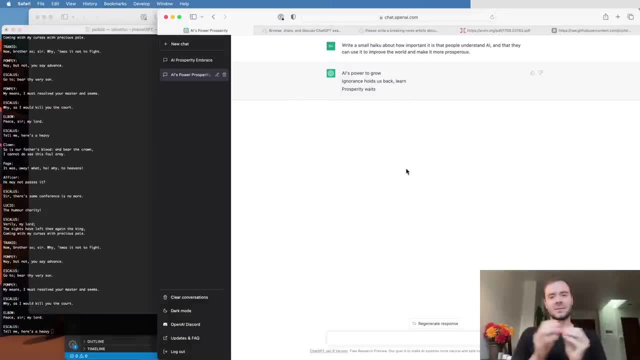 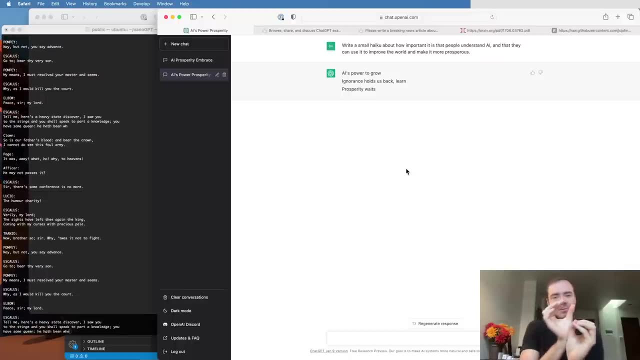 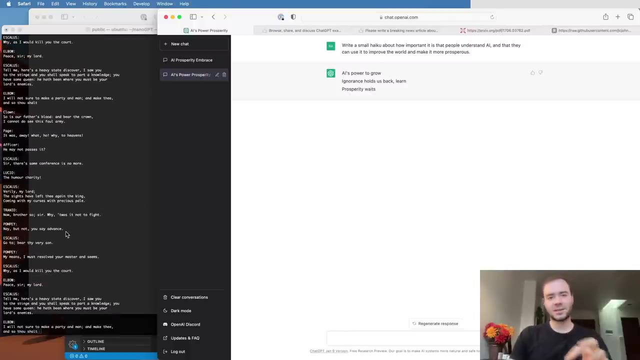 our case character by character. In ChatGPT it's coming out on the token by token level, And tokens are these sort of like little subword pieces, So they're not word level, they're kind of like word chunk level. And now I've already written this entire code to train these. 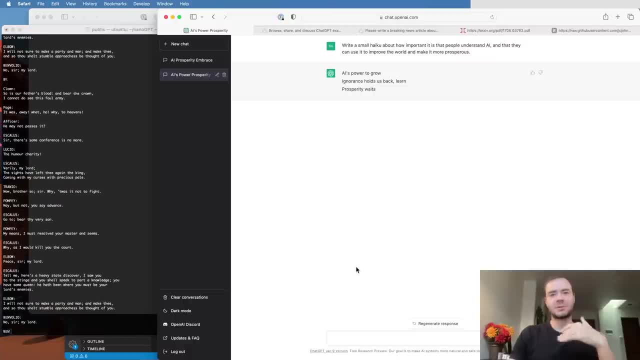 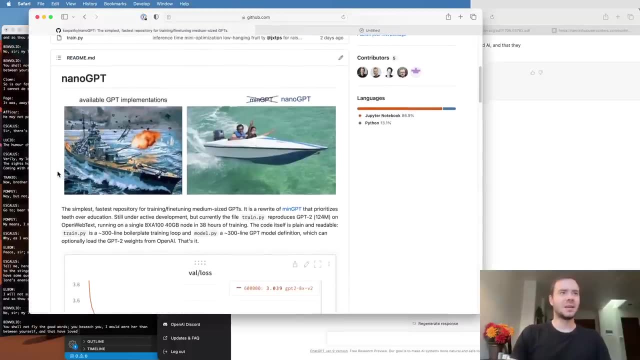 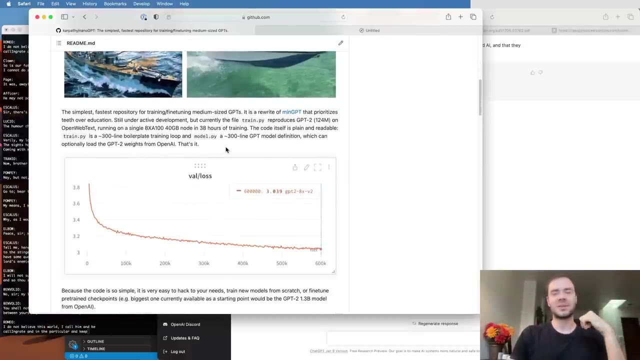 transformers And it is in a GitHub repository that you can find and it's called NanoGPT. So NanoGPT is a repository that you can find on my GitHub. It's a repository for training transformers on any given text And what I think is interesting. 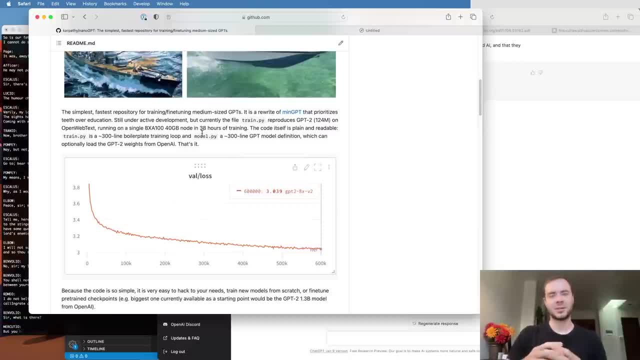 about it because there's many ways to train transformers, but this is a very simple implementation, So it's just two files of 300 lines of code each. One file defines the GPT model, the transformer, and one file trains it on some given text dataset. And here I'm showing that. 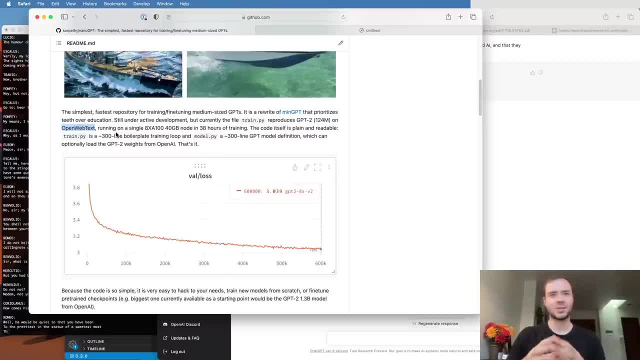 if you train it on an open webtext dataset, which is a fairly large dataset of webpages, then I reproduce the performance of GPT-2.. GPT-2 is an early version of OpenAI's GPT- from 2017,, if I recall correctly, And I've only so far. 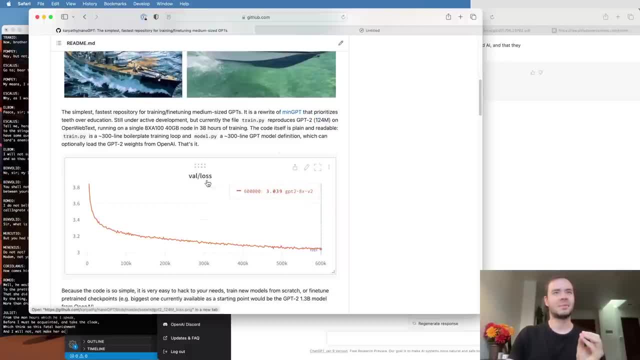 reproduced the smallest 124 million parameter model. But basically this is just proving that the code base is correctly arranged And I'm able to load the neural network weights that OpenAI has released later So you can take a look at the finished code here in NanoGPT. But what I would 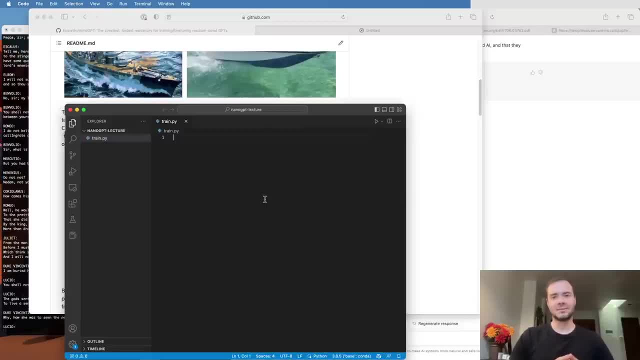 like to do in this lecture is: I would like to basically write this repository from scratch. So we're going to begin with an empty file and we're going to define a transformer, piece by piece. We're going to train it on the tiny Shakespeare dataset and we'll see how we can then generate. 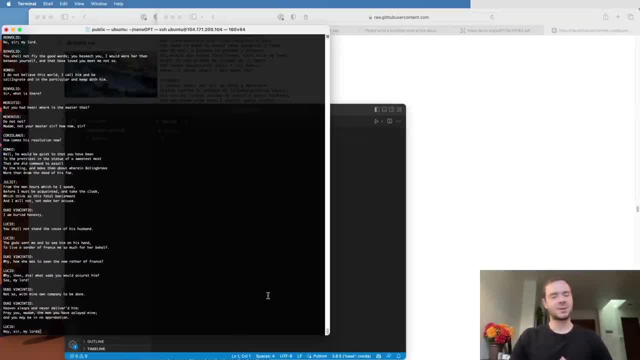 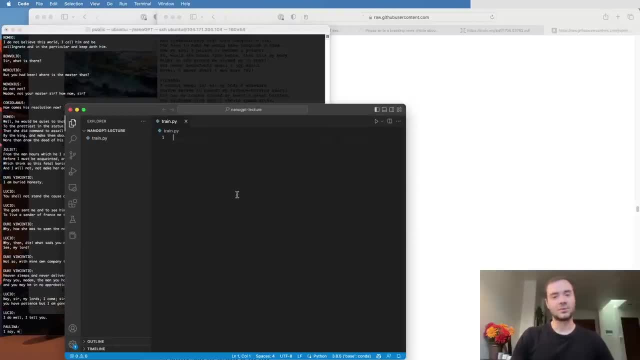 infinite Shakespeare, And of course, this can copy-paste to any arbitrary text dataset that you like. But my goal really here is to just make you understand and appreciate how under-the-hood chat GPT works, And really all that's required is a proficiency in Python and some basic. 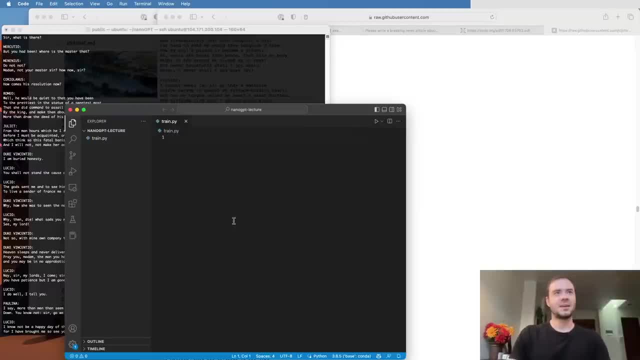 understanding of calculus and statistics. And it would help if you also see my previous videos on the same YouTube channel, in particular my Make More series where I define smaller and simpler neural network language models, So multi-layered perceptrons and so on. It really introduces the 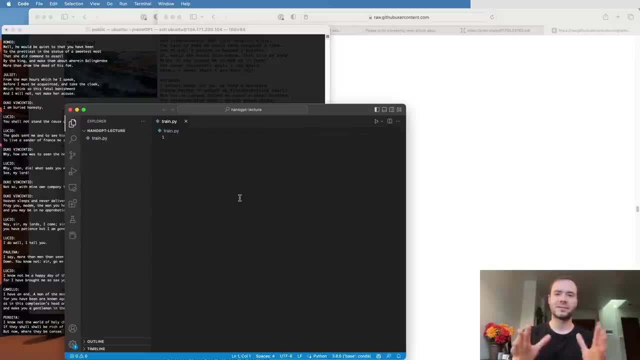 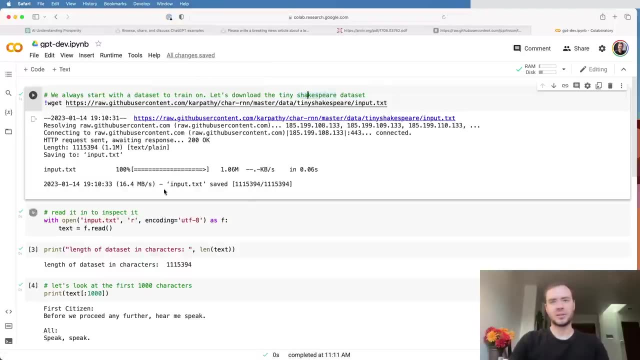 language modeling framework, And then here in this video, we're going to focus on the transformer neural network itself. Okay, so I created a new Google Colab Jupyter notebook here, And this will allow me to later easily share this code that we're going to develop together. 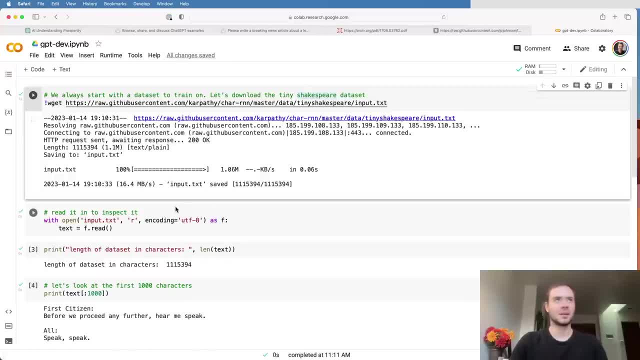 with you so you can follow along. So this will be in the video description later. Now here I've just done some preliminaries. I downloaded the dataset, the tiny Shakespeare dataset, at this URL And you can see that it's about a one megabyte file. Then here: 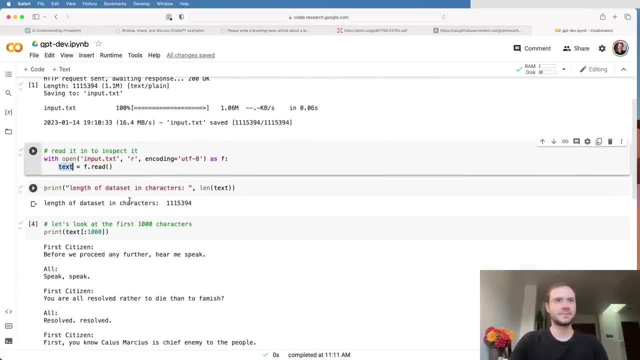 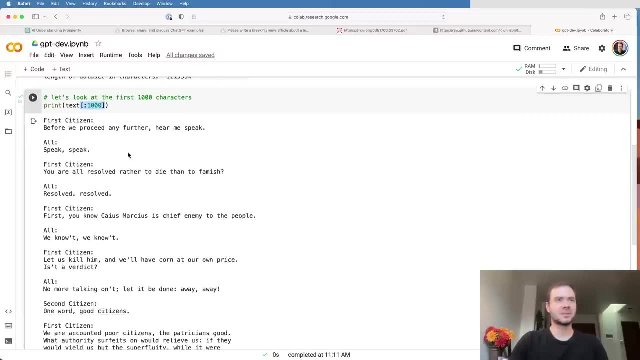 I open the inputtxt file and just read in all the text as a string And we see that we are working with one million characters roughly, And the first 1000 characters, if we just print them out, are exactly what you would expect. This is the first 1000 characters of the tiny Shakespeare dataset. 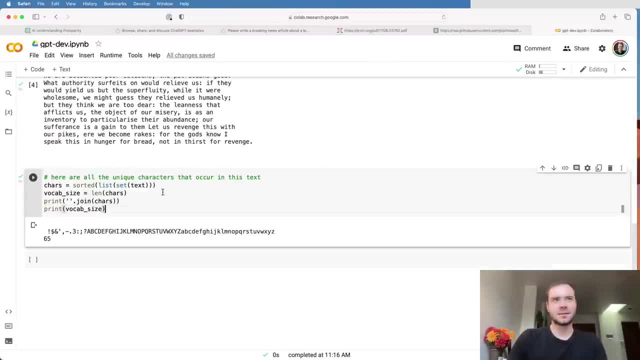 roughly up to here. So so far, so good. Next we're going to take this text, And the text is a sequence of characters in Python, So when I call the set constructor on it, I'm just going to get the set of all the characters that occur in this text And then I call list on that to create a. 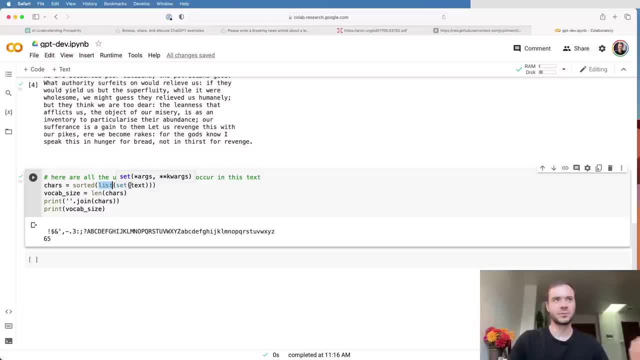 list of those characters instead of just a set, so that I have an ordering, an arbitrary ordering, Sort that. So basically, we get just all the characters that occur in the entire dataset and they're sorted. Now the number of them is going to be our vocabulary size. These are the 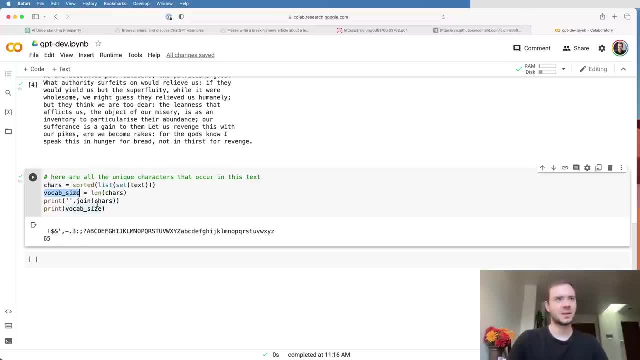 possible elements of our sequences. And we see that when I print here the characters, there's 65 of them in total. There's a space character and then all kinds of special characters and then capitals and lowercase letters. So that's our vocabulary And that's. 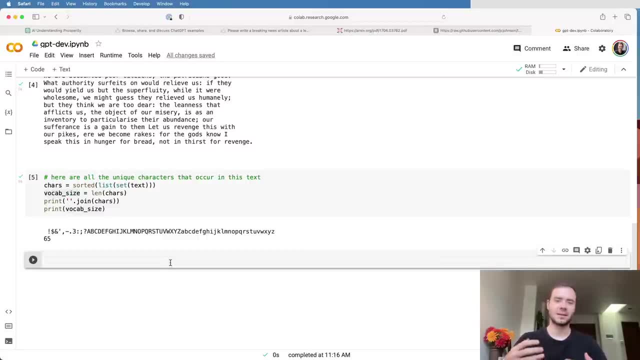 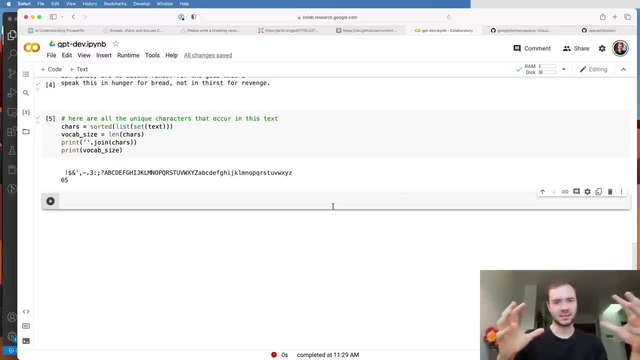 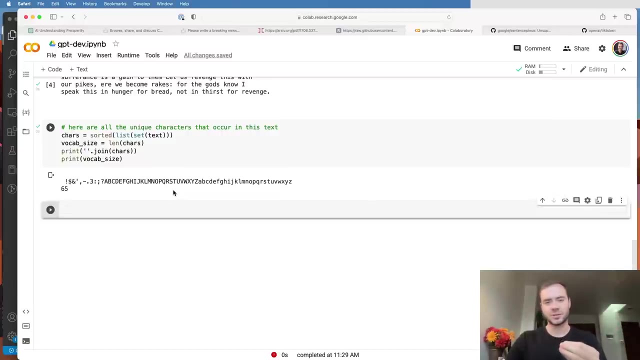 the sort of like possible characters that the model can see. Okay, so next we would like to develop some strategy to tokenize the input text. Now, when people say tokenize, they mean convert the raw text as a string to some sequence of integers. 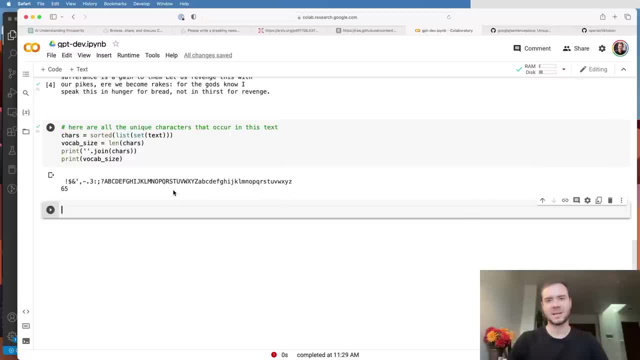 according to some notebook, according to some vocabulary of possible elements. So, as an example, here we are going to be building a character level language model, So we're simply going to be translating individual characters into integers. So let me show you a chunk of code that. 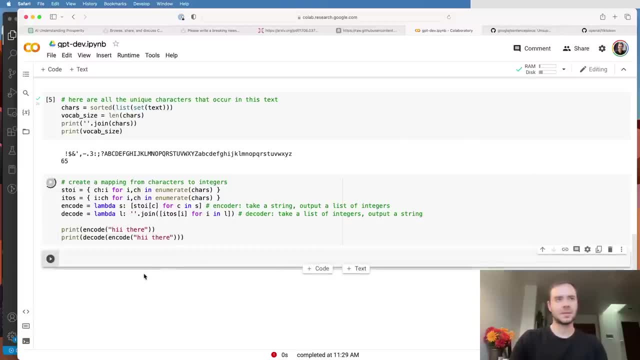 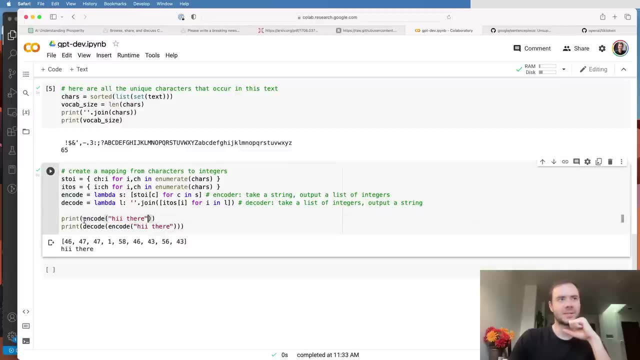 we can use. So we're building both the encoder and the decoder, And let me just talk through what's happening here. When we encode an arbitrary text like hi, there, we're going to receive a list of integers that represents that string, So, for example, 46,, 47, etc. And then we also 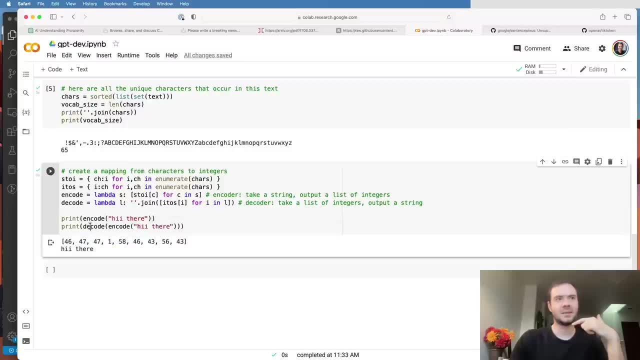 have the reverse mapping, So we can take this list and decode it to get back the exact same string. So it's really just like a translation to integers and back for arbitrary string, And for us it is done on a character level. Now, the way this was achieved is we just iterate? 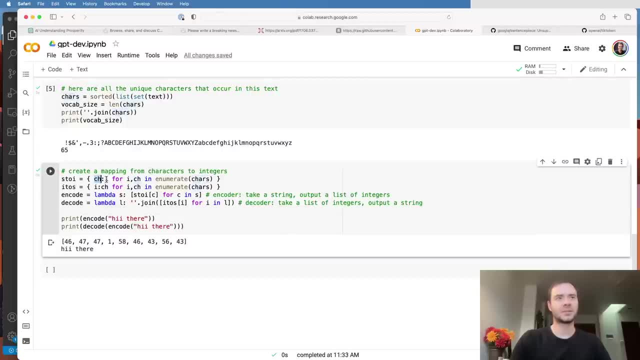 over all the characters here and create a lookup table from the character to the integer and vice versa, And then to encode some string, we simply translate all the characters individually And to decode it back we use the reverse mapping and concatenate all of it. 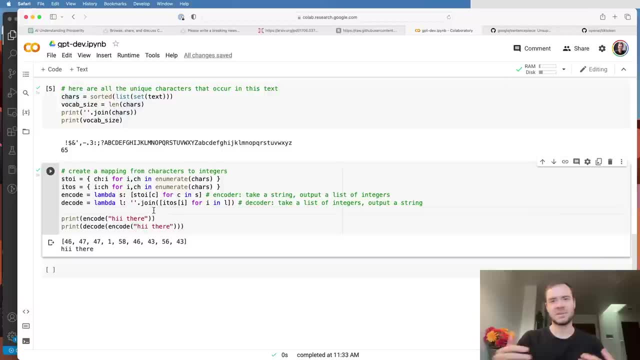 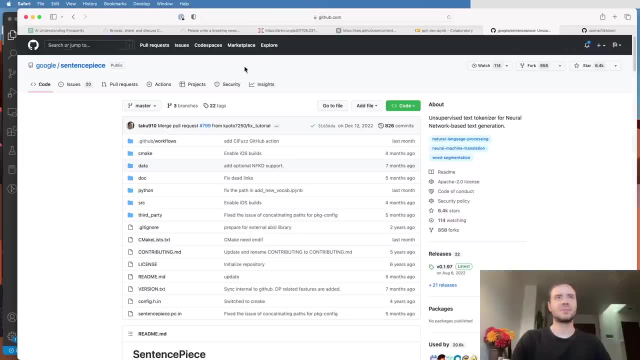 Now, this is only one of many possible encodings or many possible sort of tokenizers, And it's a very simple one. But there's many other schemas that people have come up with In practice. so, for example, Google uses Sentence Piece, So Sentence Piece will also encode text. 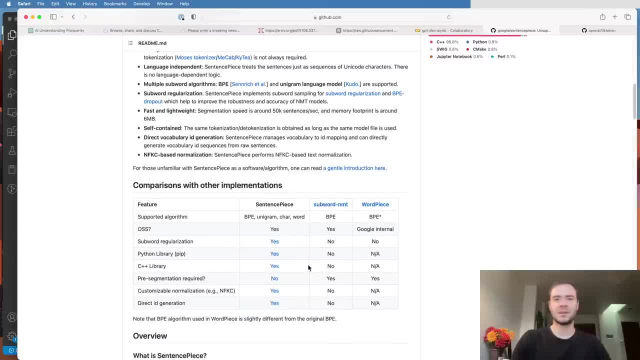 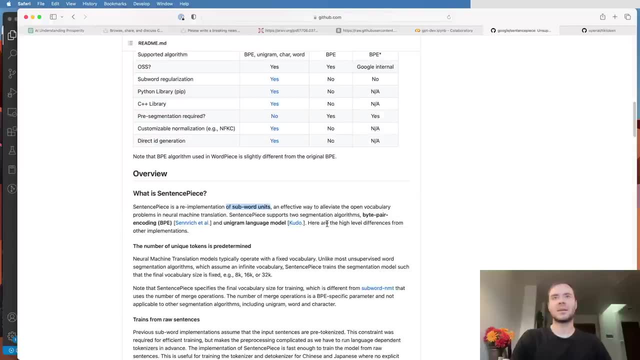 into integers, but in a different schema and using a different vocabulary And Sentence. Piece is a subword, sort of tokenizer, And what that means is that you're not encoding entire words, but you're not also encoding individual characters. It's a subword unit level. 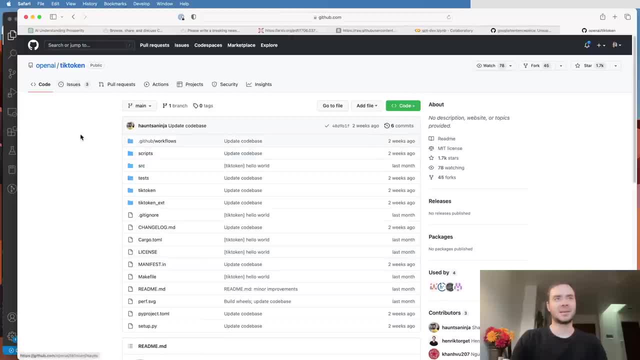 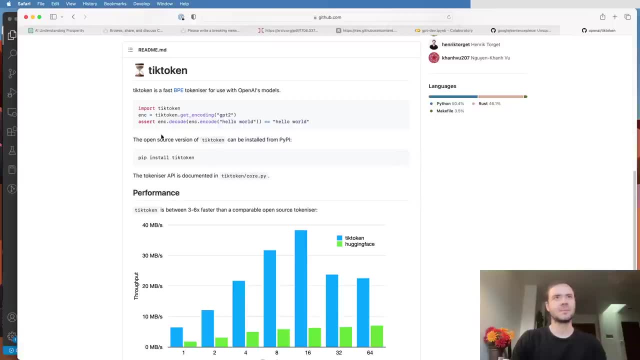 And that's usually what's adopted in practice. For example, also OpenAI has this library called TikToken that uses a byte pair encoding tokenizer And that's what GPT uses And you can also just encode words into like hello world, into a list of integers. 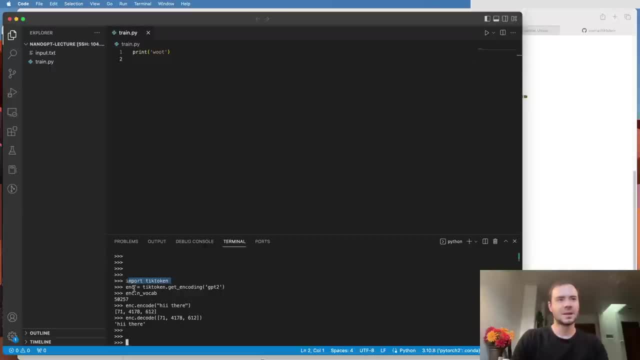 So, as an example, I'm using the TikToken library. here I'm getting the encoding for GPT-2, or that was used for GPT-2.. Instead of just having 65 possible characters or tokens, they have 50,000 tokens, And so when they encode the exact same string, hi there, we only have 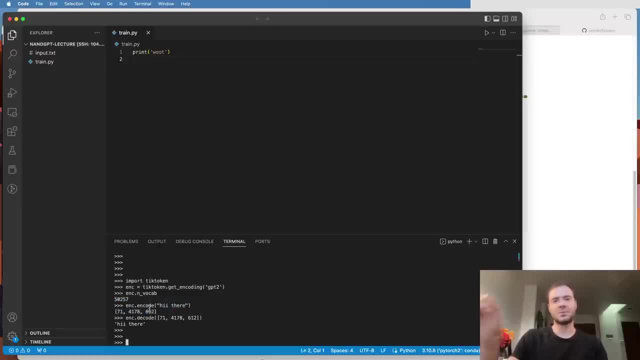 get a list of three integers, but those integers are not between 0 and 64, they are between 0 and 50,256. so basically you can trade off the codebook size and the sequence lengths. so you can have very long sequences of integers with very small vocabularies or you can have short sequences of integers. 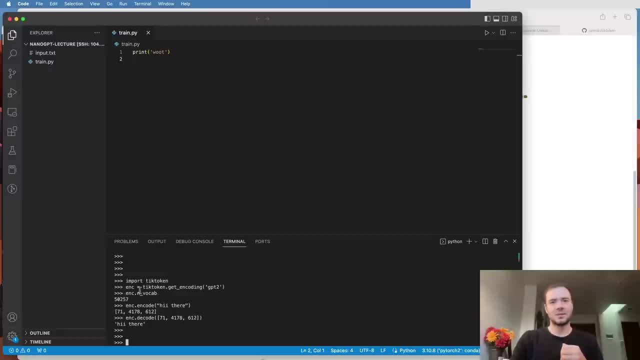 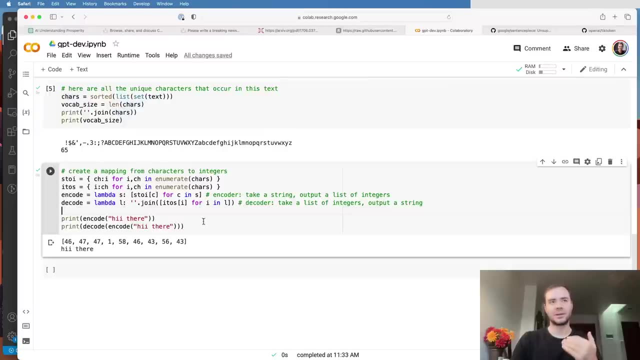 with very large vocabularies and so typically people use in practice these subword encodings. but I'd like to keep our tokenizer very simple, so we're using character level tokenizer and that means that we have very small codebooks. we have very simple encode and decode functions, but we do get very long. 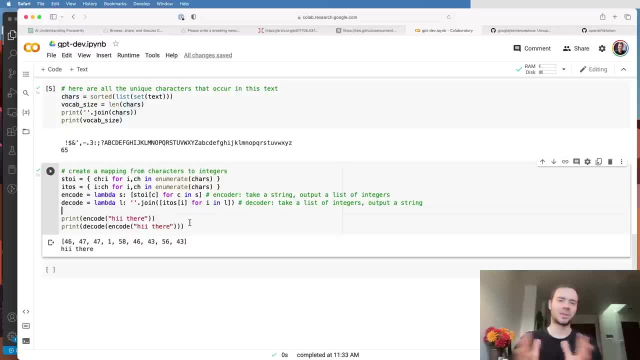 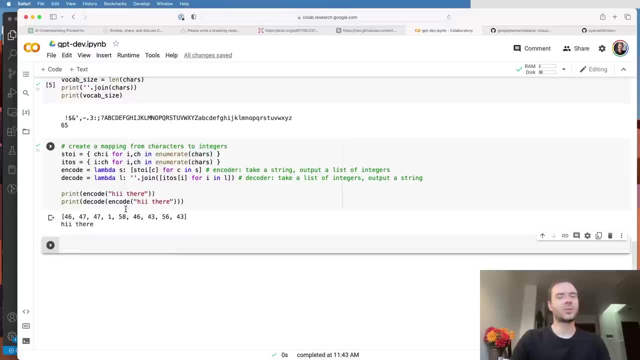 sequences as a result, but that's the level at which we're going to stick with this lecture, because it's the simplest thing. okay, so now that we have an encoder and a decoder- effectively a tokenizer, we can tokenize the entire training set of Shakespeare. so here's a chunk of code that does that, and I'm 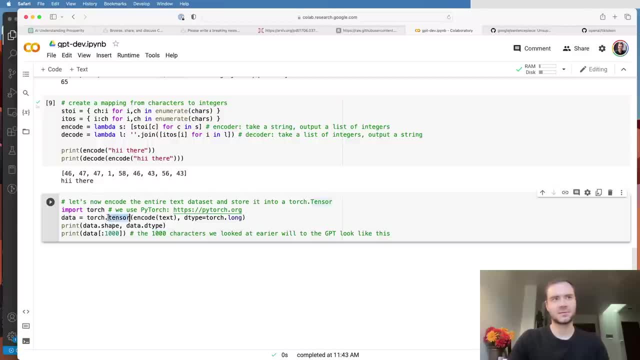 going to show you how to do that in just a few minutes. We're going to start to use the pytorch library and specifically the torchtensor from the pytorch library. so we're going to take all of the text in tiny Shakespeare, encode it and then wrap it into a torchtensor to get the data. 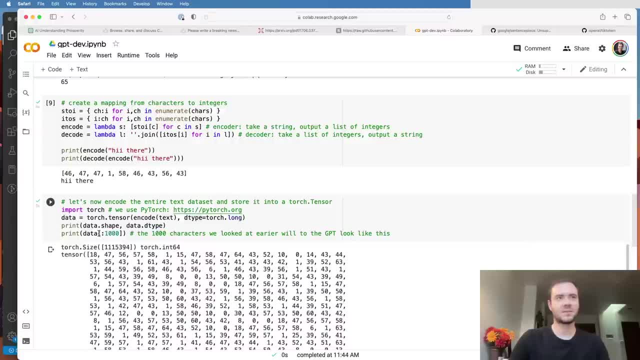 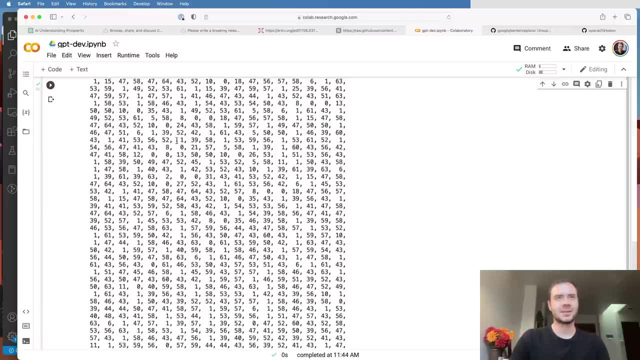 tensor. so here's what the data tensor looks like when I look at just the first 1,000 characters or the 1,000 elements of it. so we see that we have a massive sequence of integers, and this sequence of integers here is basically an. 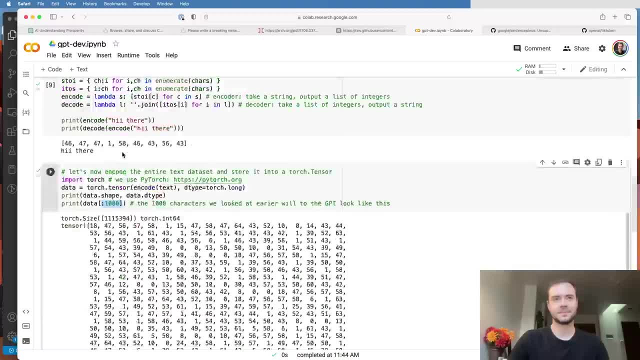 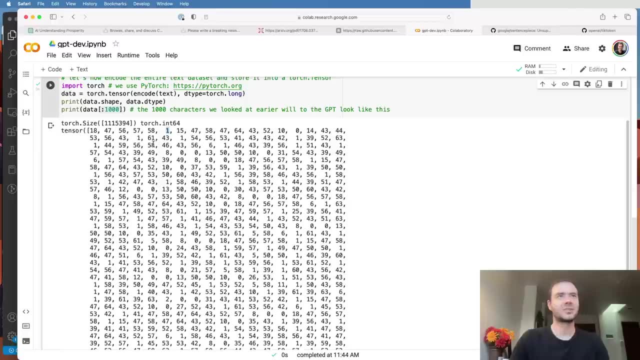 identical translation of the first 1,000 characters here. so I believe that, for example, that 0 is a newline character and maybe 1 is a space- not 100% sure, but from now on the entire data set of text is re-represented as just it's. 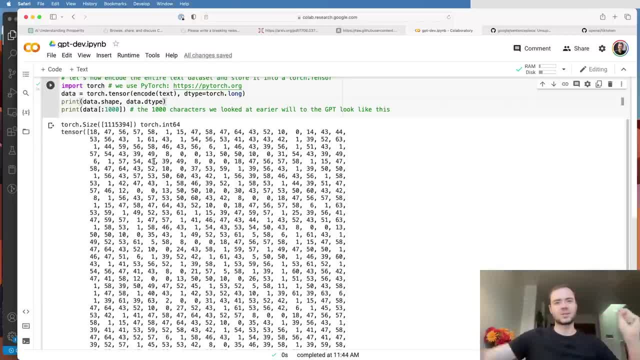 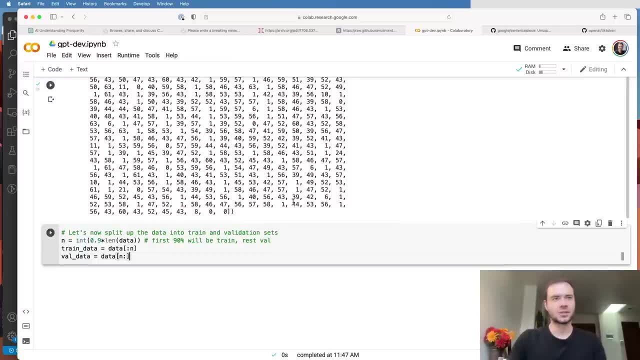 just stretched out as a single, very large sequence of integers. let me do one more thing before we move on here. I'd like to separate out our data set into a train and a validation split. so, in particular, we're going to take the first 90% of the data set and consider that to be. 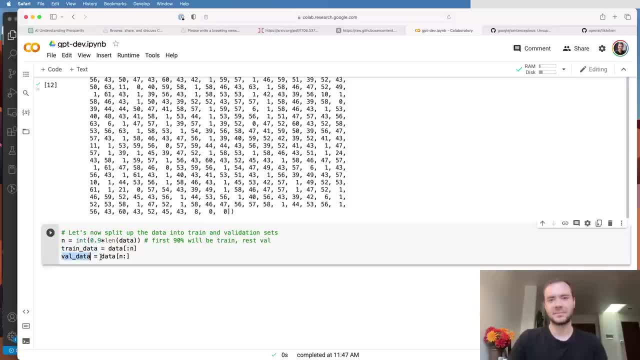 the training data for the transformer and we're going to withhold the last 10% at the end of it to be the validation data, and this will help us understand to what extent our model is overfitting. so we're going to basically hide and keep the validation data on the side because we don't want just a. 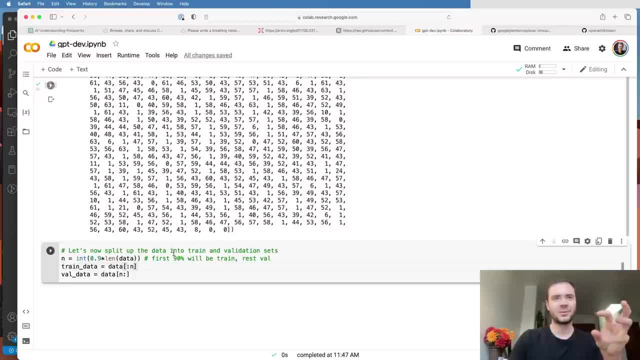 perfect memorization of this exact Shakespeare. we want a neural network that sort of creates Shakespeare like text, and so it should be fairly likely for it to produce the actual, like stowed away true Shakespeare text, and so we're going to use this to get a sense of the overfitting. okay, so now we would like to start plugging. 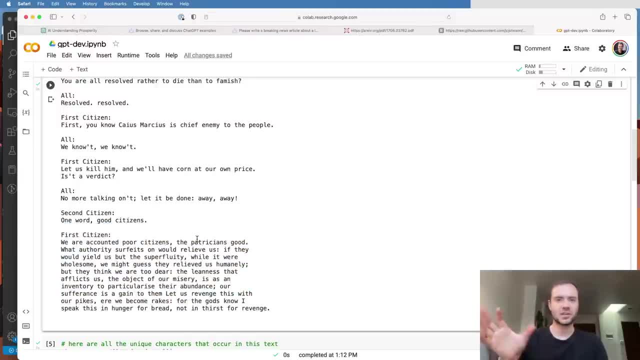 these text sequences, or integer sequences, into the transformer so that it can train and learn those patterns. now the important thing to realize is we're never going to actually feed the entire text into your transformer all at once. that would be computationally very expressed and prohibitive. so when we 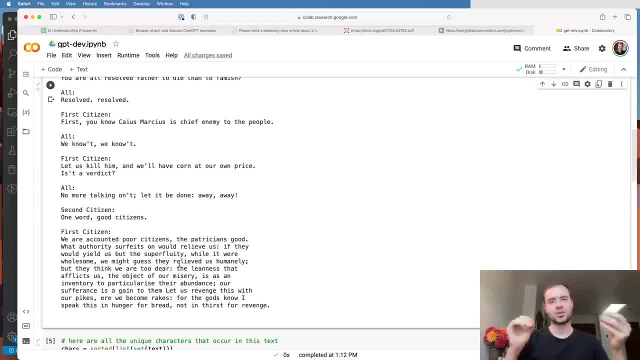 actually train a transformer on a lot of these data sets. we only work with chunks of the data set and when we train the transformer we basically sample random little chunks out of the training set and train on just chunks at a time and these chunks have basically some kind of a length and some maximum. 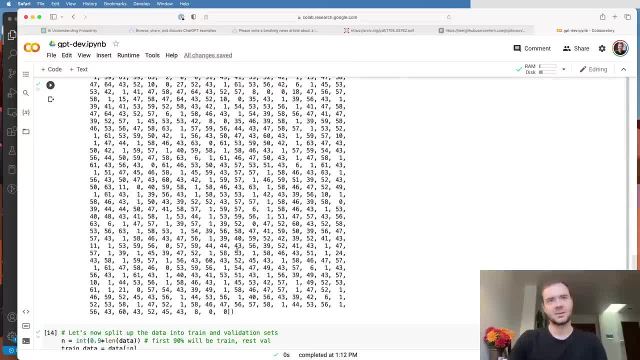 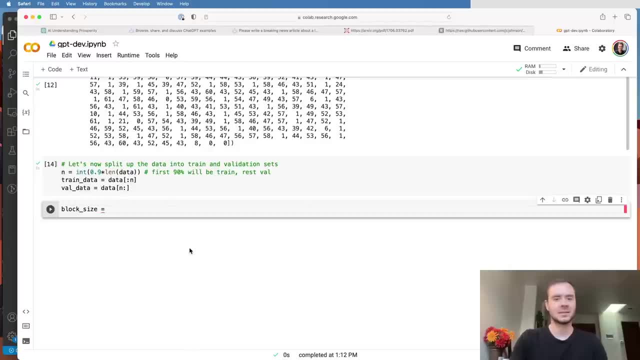 length. now the maximum length typically, at least in the code i usually write, is called block size. you can you can find it under different names like context length or something like that. let's start with the block size of just eight and let me look at the first train. 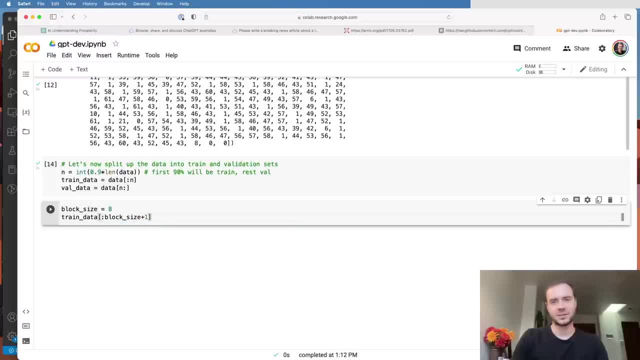 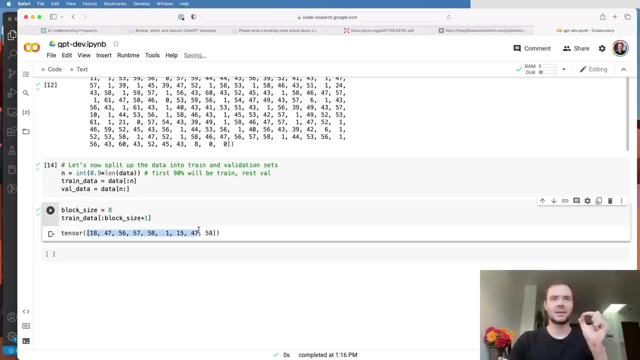 data characters: the first block size, plus one characters. i'll explain why: plus one in a second. so this is the first nine characters in the sequence in the training set. now what i'd like to point out is that when you sample a chunk of data like this, so say, these nine characters out. 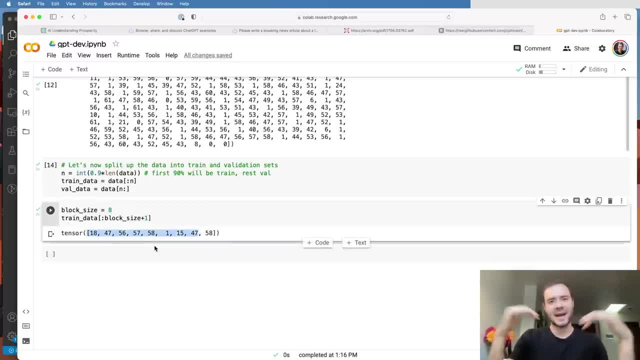 of the training set. this actually has multiple examples packed into it, and that's because all these characters follow each other, and so what this thing is going to say when we plug it into a transformer is we're going to actually simultaneously train it to make prediction at every. 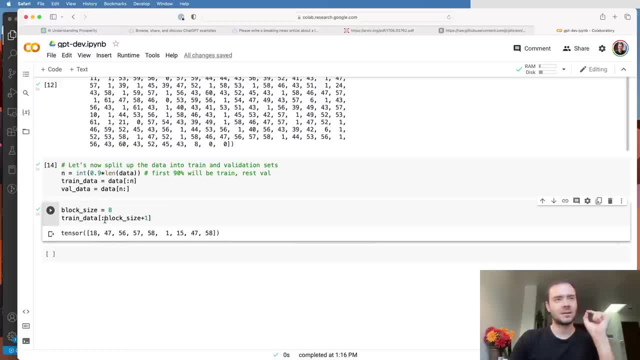 one of these positions now in the in a chunk of nine characters. there's actually eight individual examples packed in there. so there's the example that when 18- when, in the context of 18, 47 likely comes next in a context of 18 and 47, 56 comes next in the context of 18, 47, 56, 57 can come. 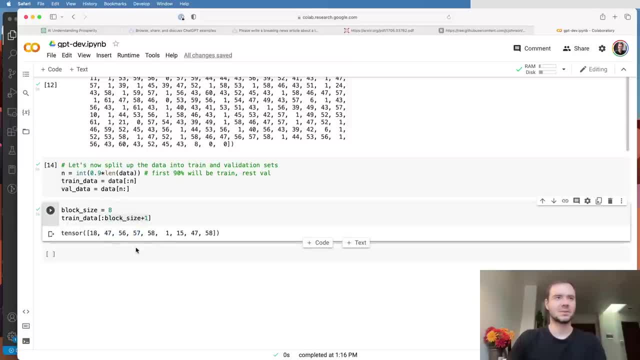 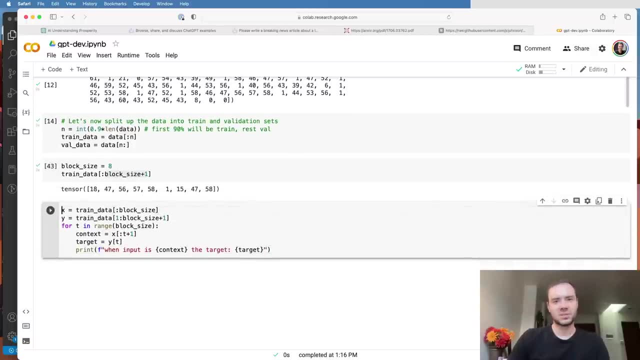 next and so on. so that's the eight individual examples. let me actually spell it out with code. so here's a chunk of code to illustrate. x are the inputs to the transformer. it will just be the first block size characters. y will be the, the block size characters, so it's offset by one. 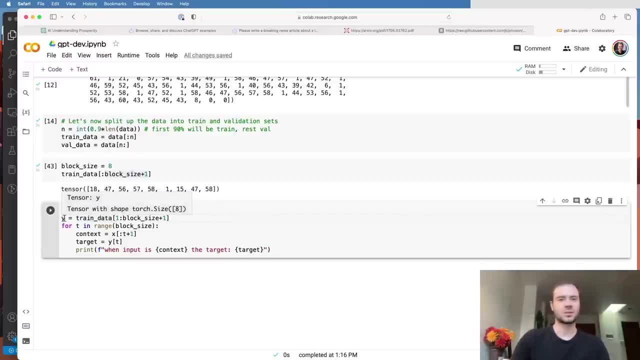 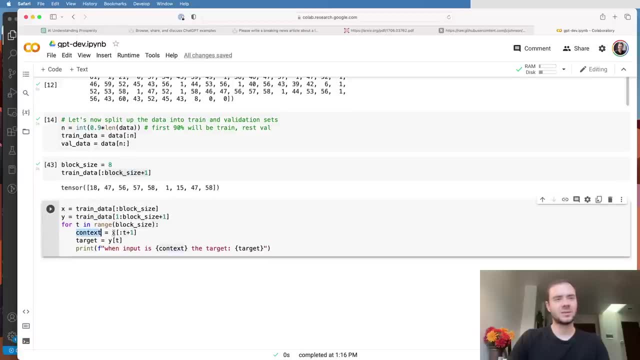 and that's because y are the targets for each position in the input. and then here i'm iterating over all the block size of 8, and the context is always all the characters in x up to t and including t, and the target is always responsibilities, oft eting the inputs. so so that's. 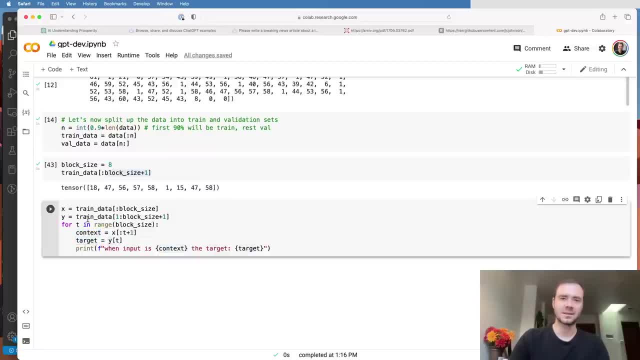 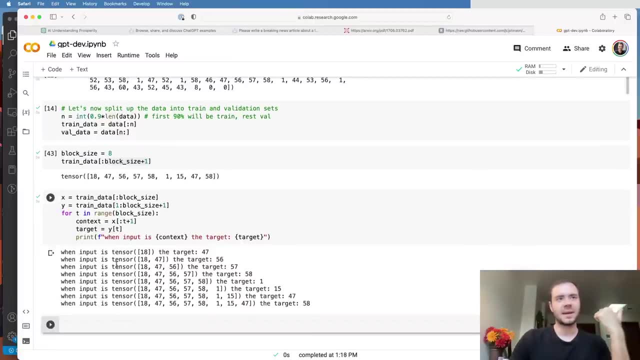 a chasing number which, uh, we tell the grammatical primary space, heading j, the teeth character, but in the targets, array y. so let me just run this and basically it spells out what i said in words. these are the eight examples, hidden in a chunk of nine characters, that we 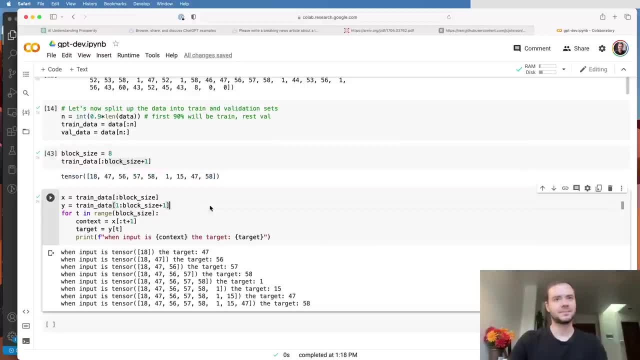 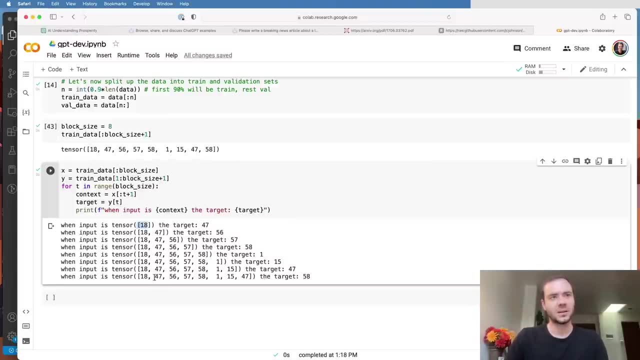 sampled from the training set. i want to mention one more thing. we train on all the eight examples here with context between one, all the way up to context of block size, and we train on that not just for computational reasons, because we happen to have the sequence already, or something like. 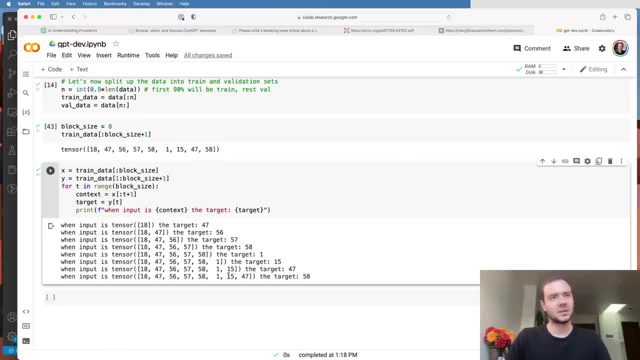 that it's not just done for efficiency, it's also done to make the transformer network be used to seeing contexts all the way from as little as one, all the way to block size, and we'd like the transformer to be used to seeing everything in between, and that's going to be useful later during. 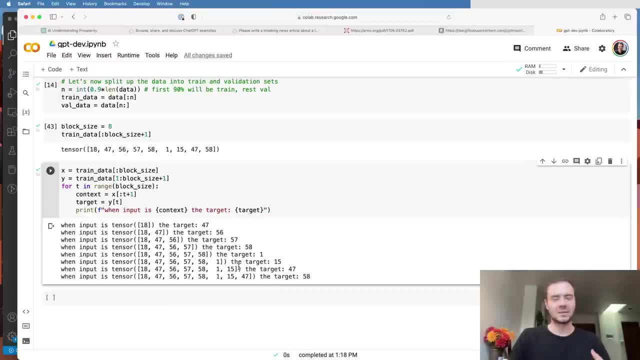 inference, because while we're sampling, we can start to set sampling generation with as little as one character of context, and the transformer knows how to predict the next character- you with- all the way up to just context of one, and so then it can predict everything up to block size. 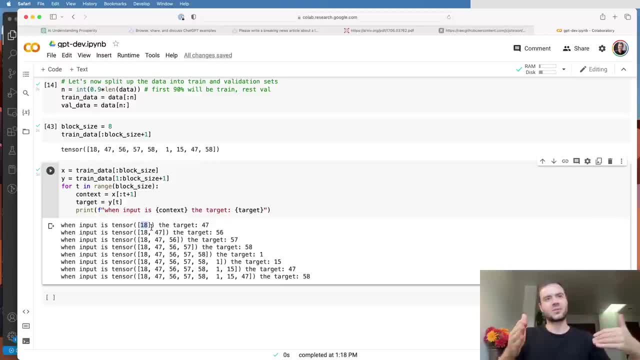 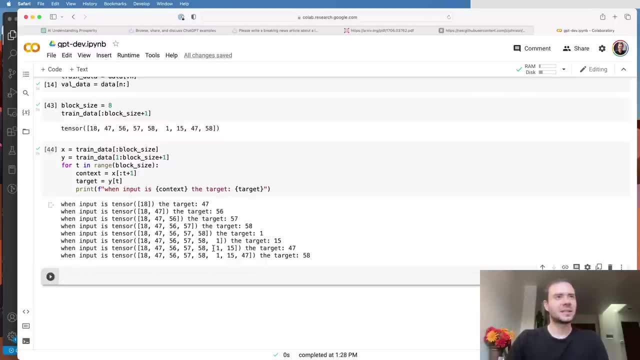 and after block size, we have to start truncating, because the transformer will never receive more than block size inputs when it's predicting the next character. okay, so we've looked at the time dimension of the tensors that are going to be feeding into the transformer. there's one more. 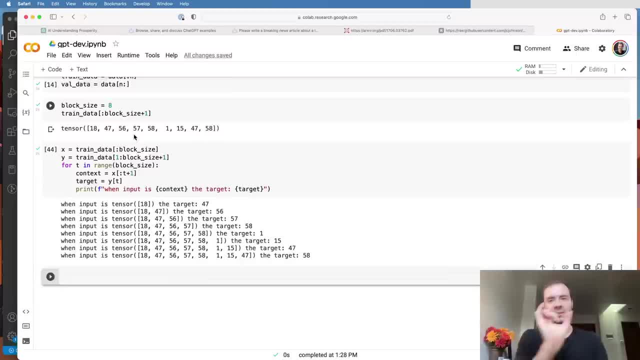 dimension to care about, and that is the batch dimension. and so, as we're sampling these chunks of text- we're going to be actually, every time we're going to feed them into a transformer- we're going to have many batches of multiple chunks of text that are all like stacked up in a single tensor. 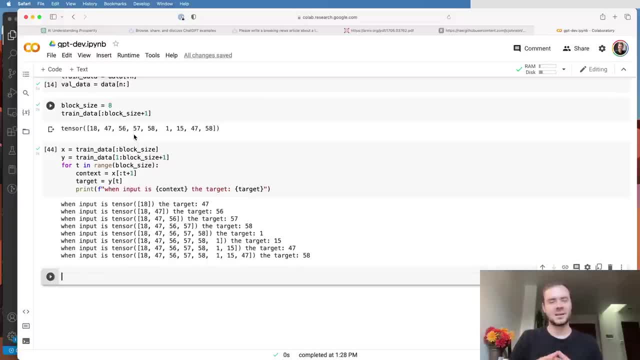 and that's just done for efficiency, just so that we can keep the gpus busy, because they are very good at parallel processing of of data, and so we just want to process multiple chunks all at the same time. but those chunks are processed completely independently. they don't talk. 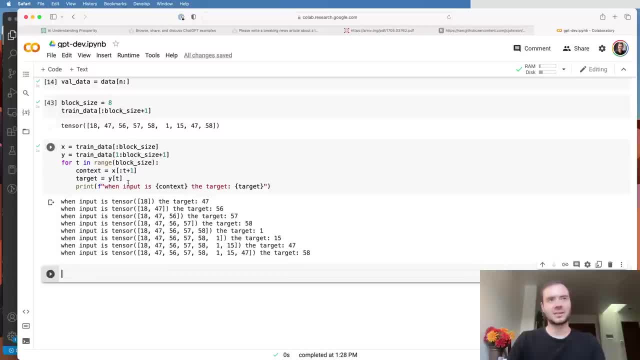 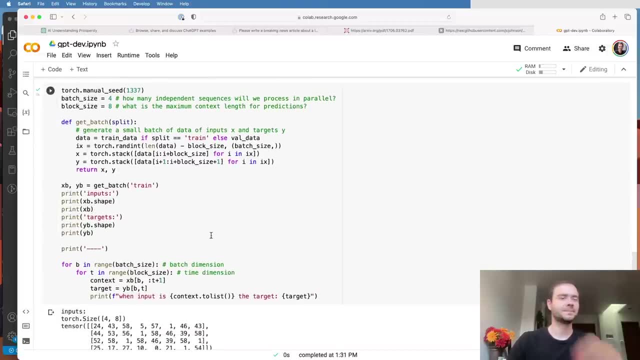 to each other and so on. so let me basically just generalize this and introduce a batch dimension. here's a chunk of code. let me just run it, and then i'm going to explain what it does. so i'm going to run it. fn of absolute volume, which is similar to the fact that it's a. 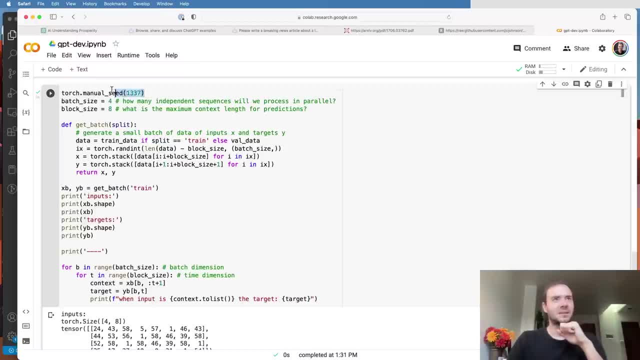 static block. but there are some other parameters i'm going to explain in a minute. so here, because we're going to start sampling random locations in the data set to pull chunks from, i am setting the seed so that in the random number generator, so that the numbers i see, 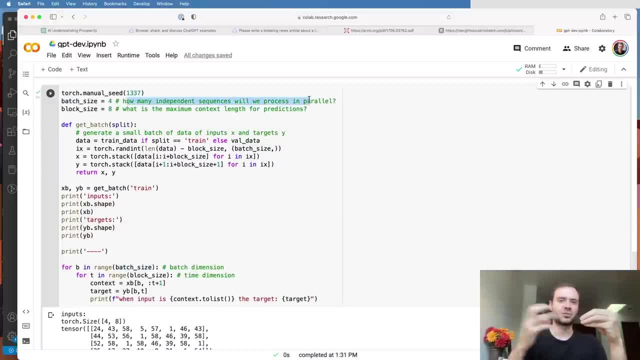 here are going to be the same numbers you see later if you try to reproduce this now. the batch size here is how many independent sequences we are processing every forward, backward pass of the transformer size 8. and then here's how we get batch for any arbitrary split, if the split is 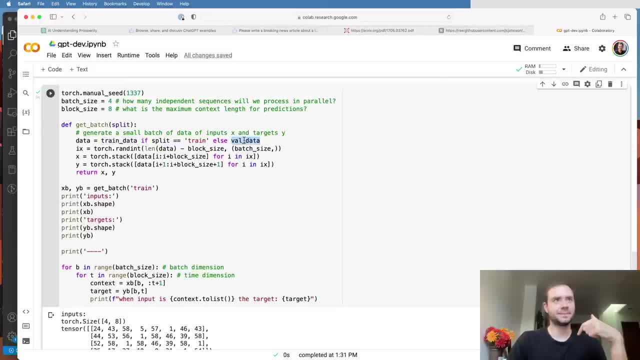 a training split, then we're going to look at train data otherwise and Val data. that gives us the data array and then when I generate random positions to grab a chunk out of, I actually grab, I actually generate batch size, number of random offsets. so, because this is for we are, IX is going to be a four numbers. 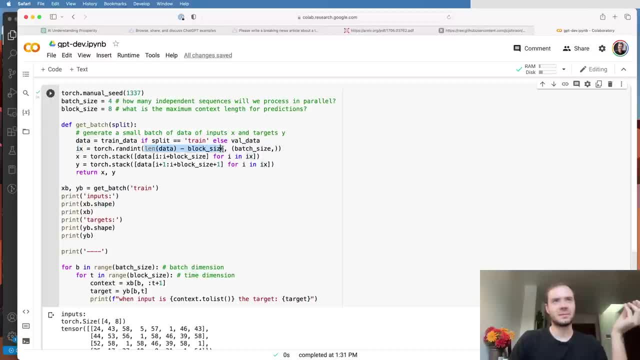 that are randomly generated between zero and Len of data minus block size. so it's just random offsets into the training set. and then X is, as I explained, are the first block size characters, starting at I. the Y's are the offset by one of that. so just add plus one and then we're going to get those. 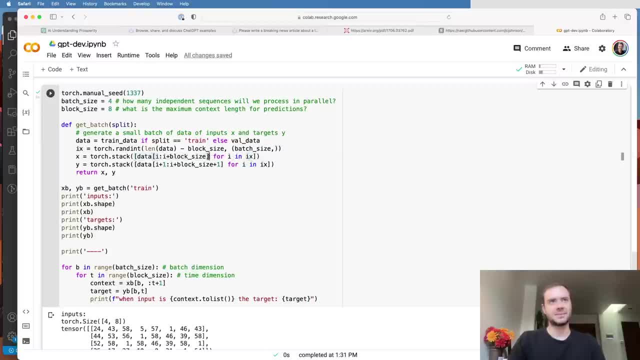 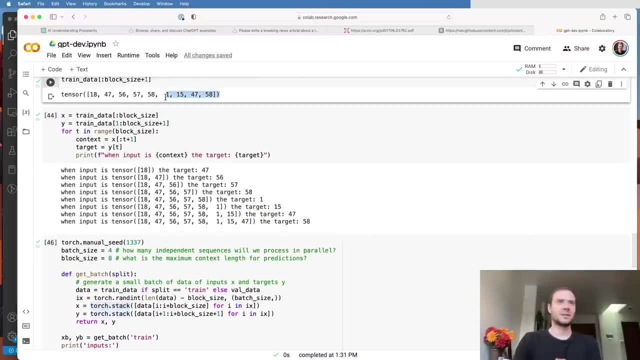 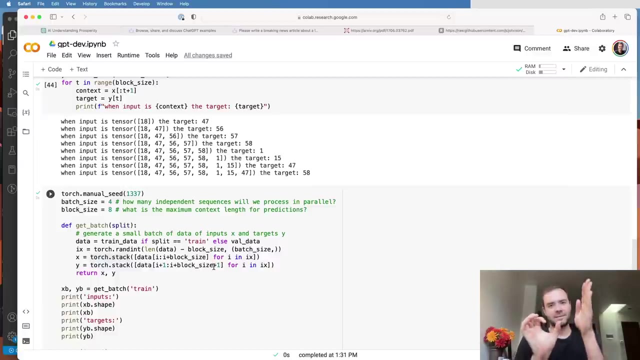 chunks for every one of integers I in IX and use a torch dot stack to take all those you one dimensional tensors, as we saw here, and we're going to stack them up as rows and so they all become a row in a four by eight tensor. so here's what I'm. 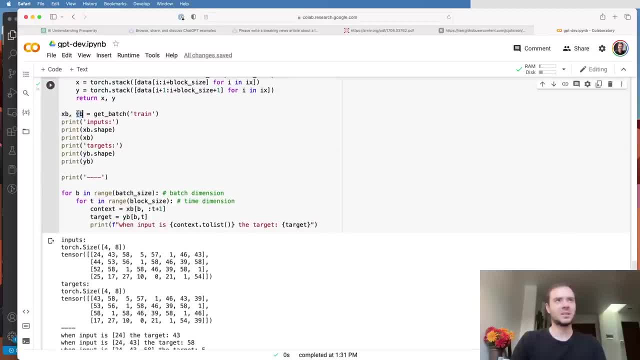 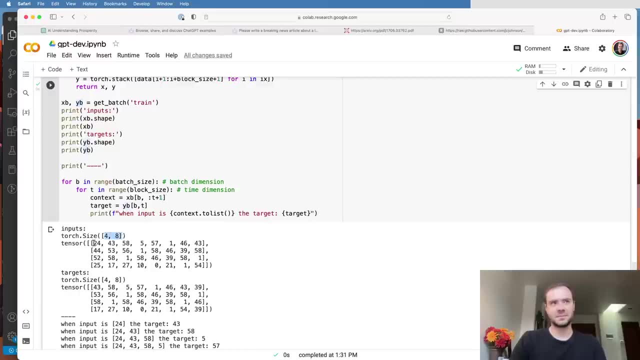 printing them. when I sample a batch XB and YB, the inputs, the transformer now are: the input X is the four by eight tensor, four rows of eight columns and each one of these is a chunk of the training set. and then the targets here are in the associated arrayy and they: 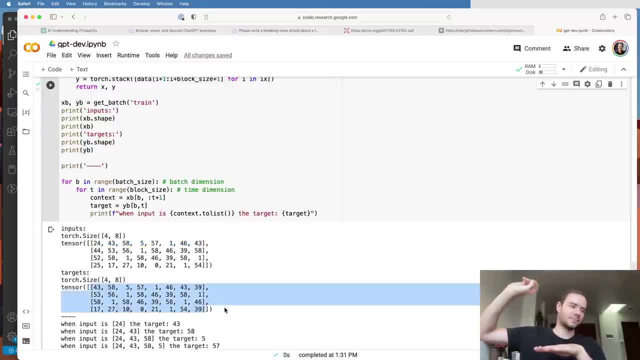 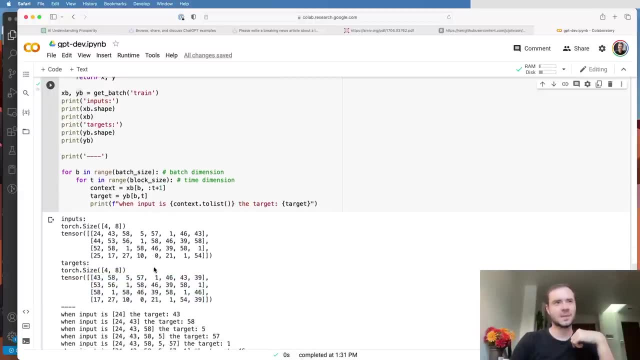 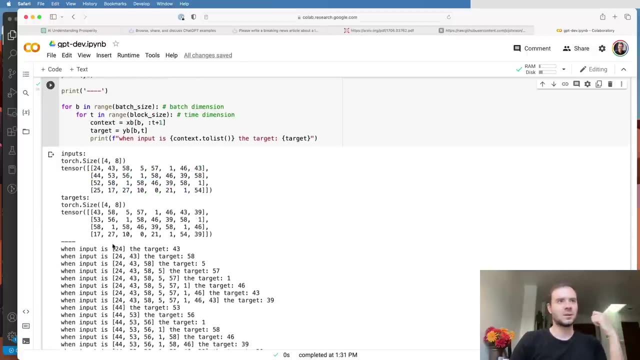 will come in, transform all the way at the end to create the last function, so they will give us the correct answer for every single position inside X. and then these armed for independent rows. so spelled out as we did before, this 4 by eight array contains a total of thirty two examples. so the difference between creating the first set, little bit bigger than the last set of the training set is: Europic follows you and more variables are also finer than a first stroke of this are what the transformation equals and therefore the target is in Y. variables and dé remain associated with X in the exact same way. anthropomorphization is not complex, but this is something that basically during our learning cycle- Western clearing out of the training setting and then other visitors are- deserve to sort extra attention on. the next set of Y from there, 짜 y'all will be one of the appropriate elements in this. 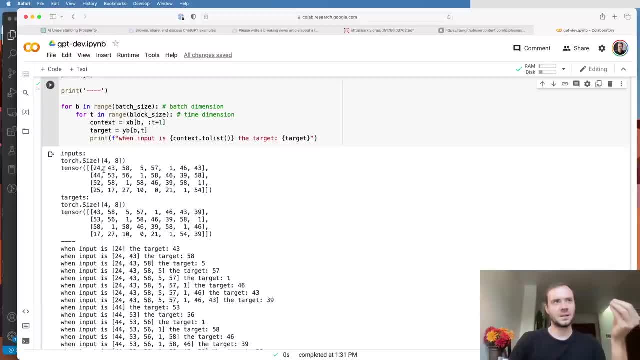 and they're completely independent as far as the transformer is concerned. So when the input is 24,, the target is 43,, or rather 43 here in the y array. When the input is 24, 43,, the target is 58.. When the input is 24,, 43,, 58,, the target is 5, etc. Or like when it is. 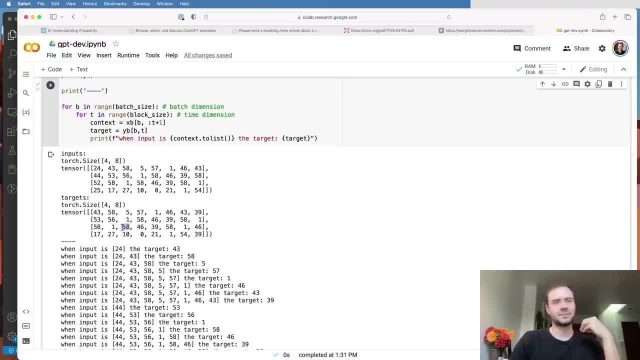 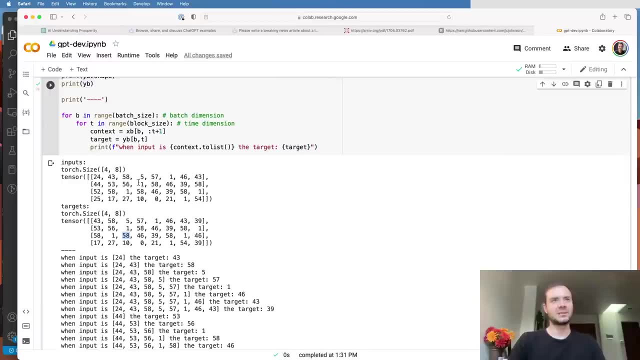 a 52,, 58,, 1,. the target is 58. Right, so you can sort of see this spelled out. These are the 32 independent examples packed in to a single batch of the input x, and then the desired targets are. 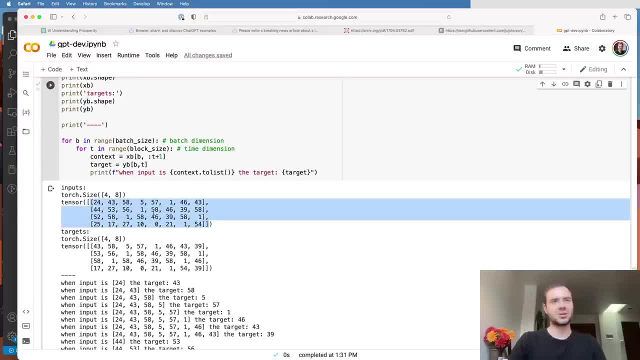 in y. And so now this integer tensor of x is going to feed into the transformer and that transformer is going to simultaneously process all these examples and then look up the correct integers to predict in every one of these positions in the tensor y. Okay, 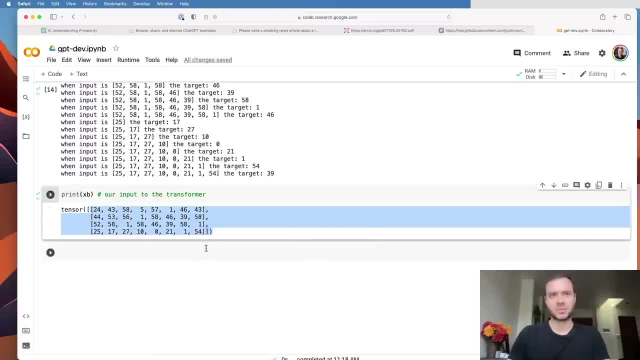 so, now that we have our batch of input that we'd like to feed into a transformer, let's start basically feeding this into neural networks. Now we're going to start off with the simplest possible neural network, which, in the case of language modeling, in my opinion, 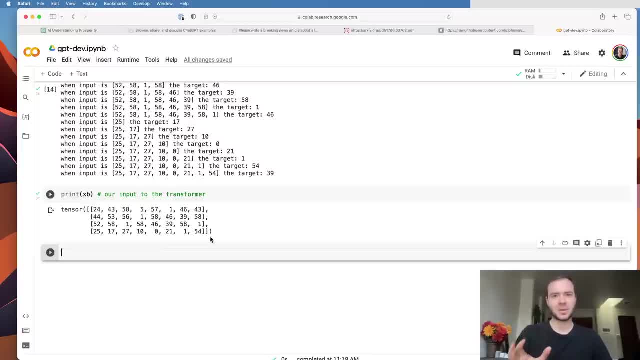 is the bigram language model, And we've covered the bigram language model in my make more series in a lot of depth, And so here I'm going to sort of go faster and let's just implement the PyTorch module directly. that implements the bigram language model. So I'm importing 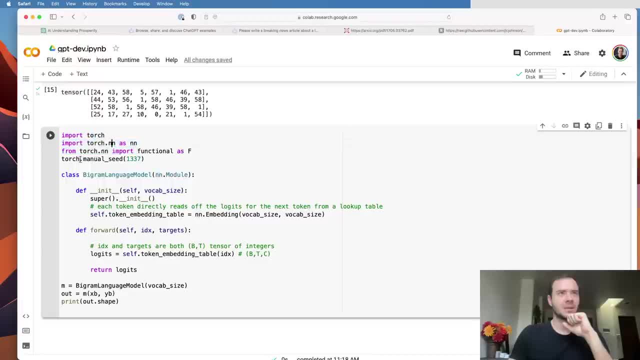 the PyTorch nn module for reproducibility. and then here I'm constructing a new model of the bigram language model, which is a subclass of nn module, And then I'm calling it and I'm passing in the inputs and the targets and I'm just printing Now when the inputs and targets 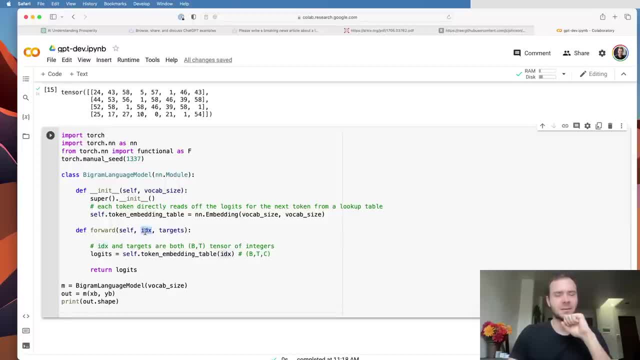 come here. you see that I'm just taking the index, the inputs x here, which I renamed to idx, and I'm just passing them into this token embedding table. So what's going on here is that here in the constructor we are creating a token embedding table and it is of size, vocab size by. 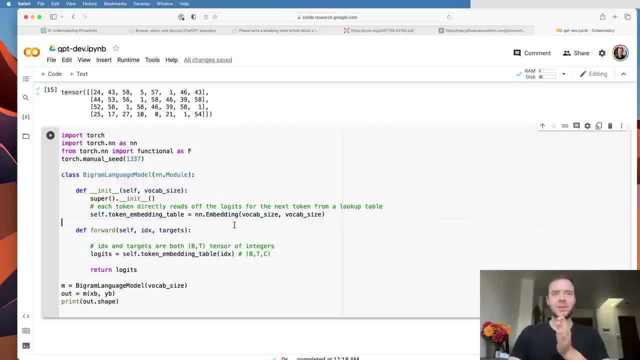 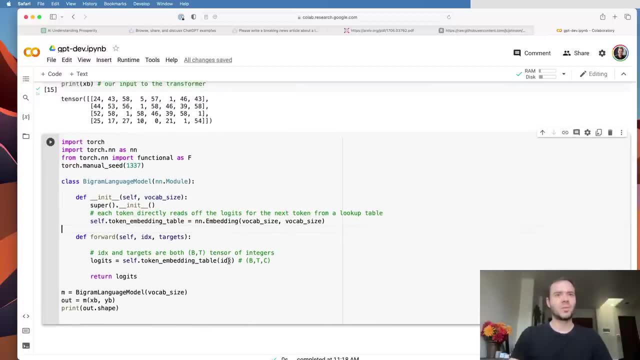 vocab size And we're using an n dot embedding which is a very thin wrapper around, basically a tensor of shape, vocab size by vocab size, And what's happening here is that when we pass idx here, every single integer in our input is going to refer to this embedding table and is going to 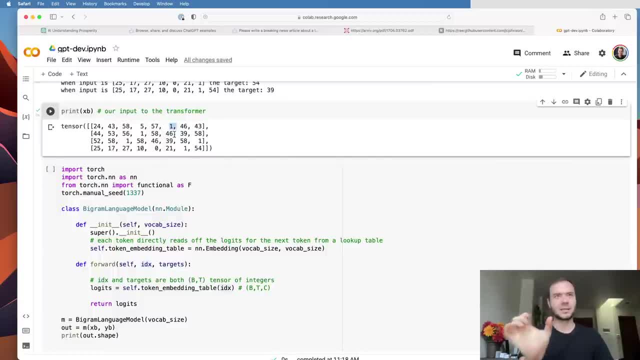 pluck out a row of that embedding table corresponding to its index. So 24 here will go to the embedding table and we'll pluck out the 24th row. And then 43 will go here and pluck out the 43rd. 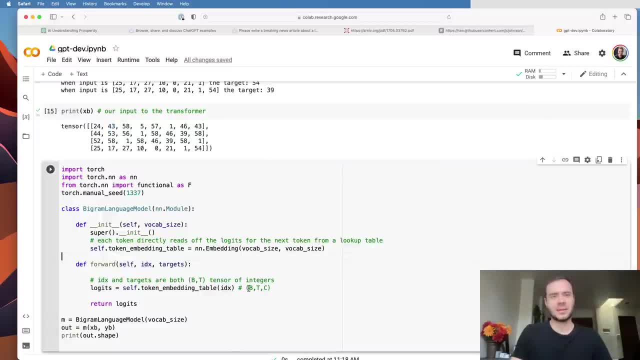 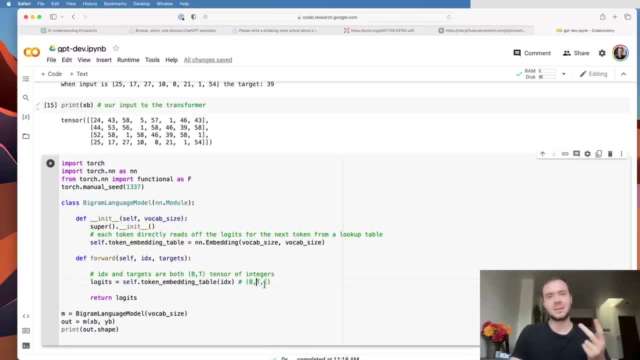 row, etc. And then PyTorch is going to arrange all of this into a batch by time, by channel tensor. In this case, batch is 4,, time is 8, and c, which is the channels, is vocab size or 65.. 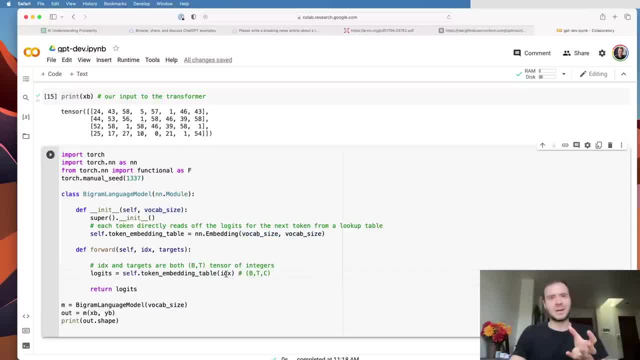 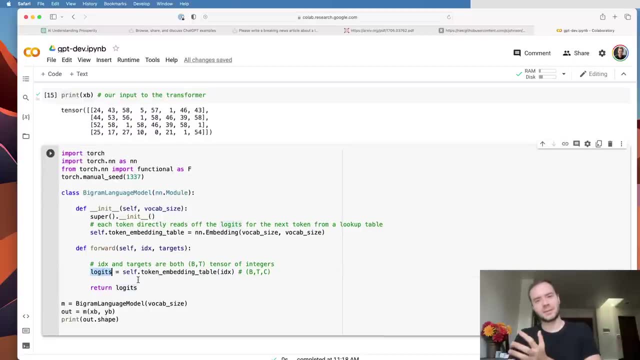 And so we're just going to pluck out all those rows, arrange them in a, b, by t, by c, and now we're going to interpret this as the logits, which are basically the scores for the next character in the sequence. And so what's happening here is we are predicting what 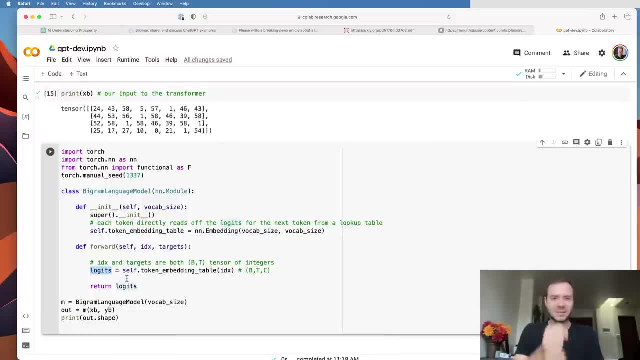 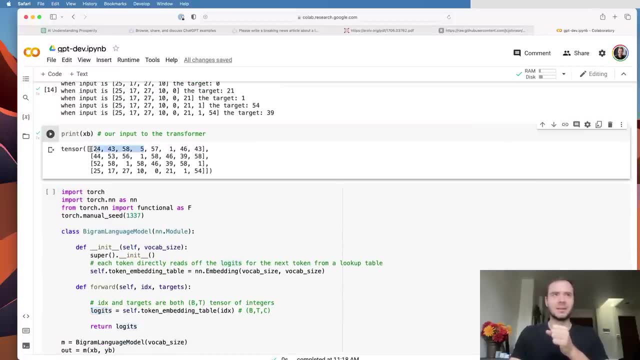 comes next, based on just the individual identity of a single token. And you can do that because I mean, currently the tokens are not talking to each other and they're not seeing any context, except for they're just seeing themselves. So I'm a token number 5, and then I can actually 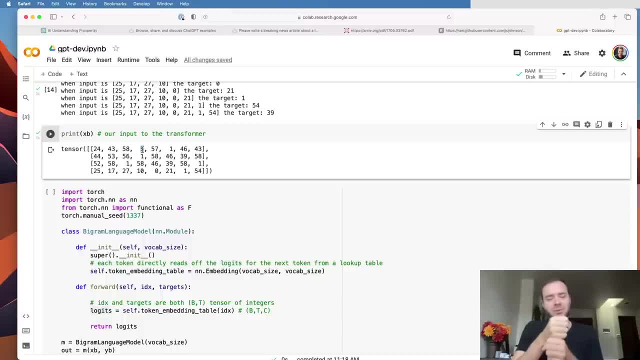 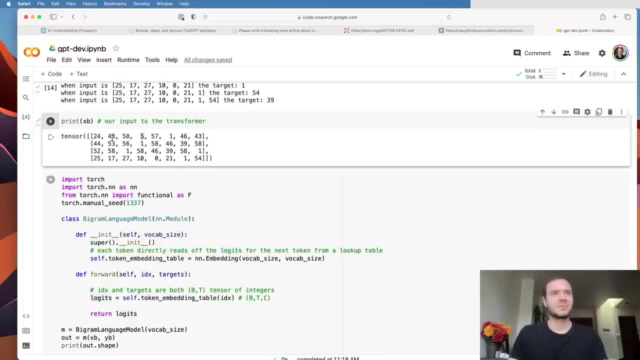 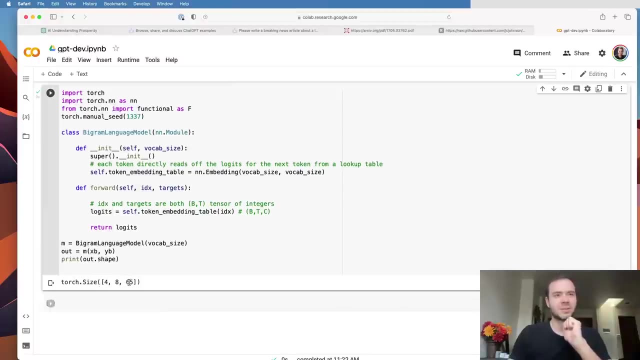 make pretty decent predictions about what comes next just by knowing that I'm token 5, because some characters follow other characters in typical scenarios. So we saw a lot of this in a lot more of the make, more series, and here, if I just run this, then we currently get the predictions. 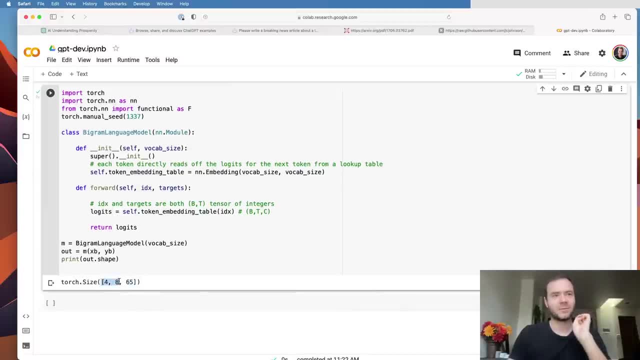 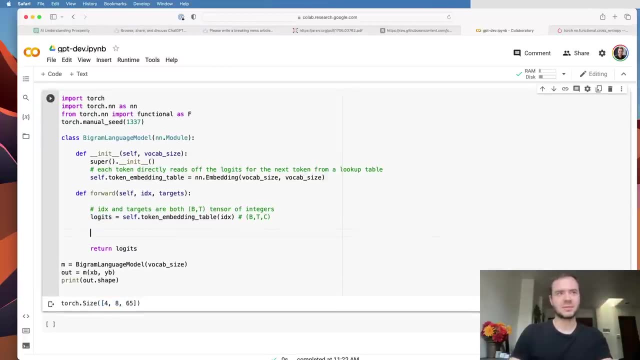 the scores, the logits, for every one of the 4 by 8 positions. Now that we've made predictions about what comes next, we'd like to evaluate the loss function, And so in make more series, we saw that a good way to measure a loss, or like a quality of the predictions, is to use the negative log. 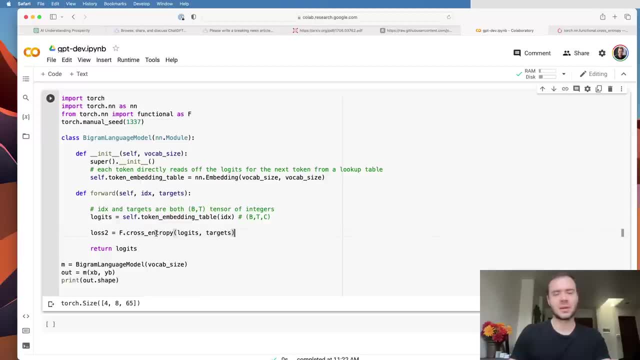 likelihood loss, which is also implemented in PyTorch under the name crossentropy. So what we'd like to do here is we'd like to use the crossentropy on the predictions and the targets, And so this measures the quality of the logits with respect to the targets. In other words, we have the identity of the next character. 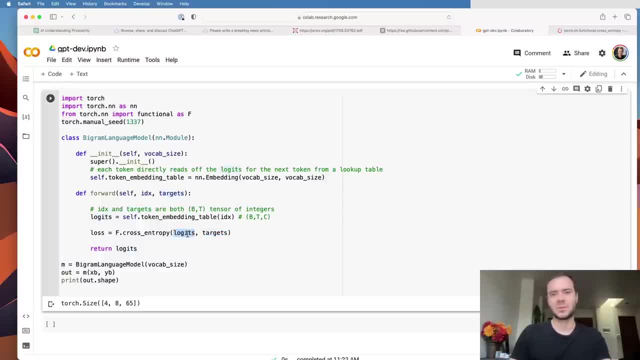 so how well are we predicting the next character based on the logits? And, intuitively, the correct dimension of logits, depending on whatever the target is, should have a very high number and all the other dimensions should be very low number. right Now the issue is that this won't. 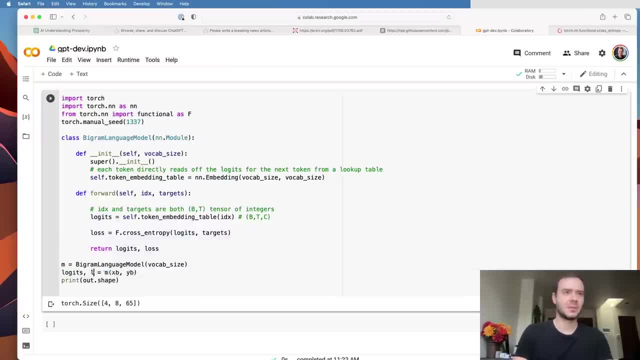 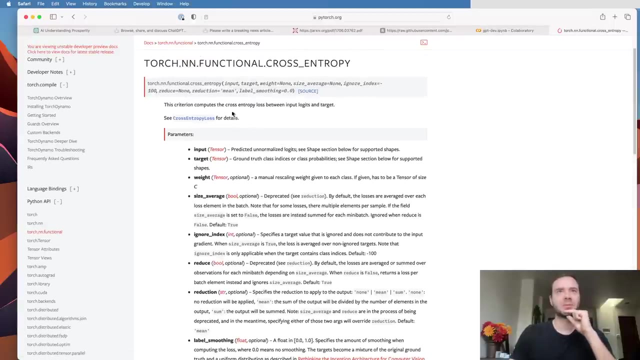 actually This is what we want. We want to basically output the logits and the loss. This is what we want, but unfortunately this won't actually run. We get an error message, but intuitively, we want to measure this Now when we go to the PyTorch crossentropy. 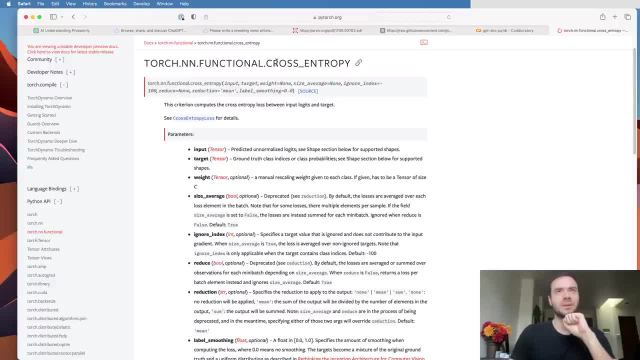 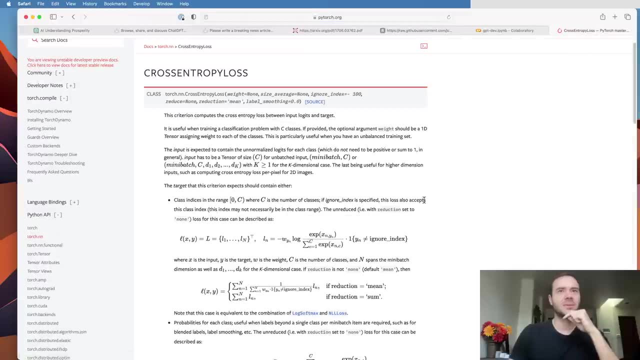 documentation. here we're trying to call the crossentropy in its functional form, so that means we don't have to create like a module for it. But here, when we go to the documentation, you have to look into the details of how PyTorch expects these inputs And basically, 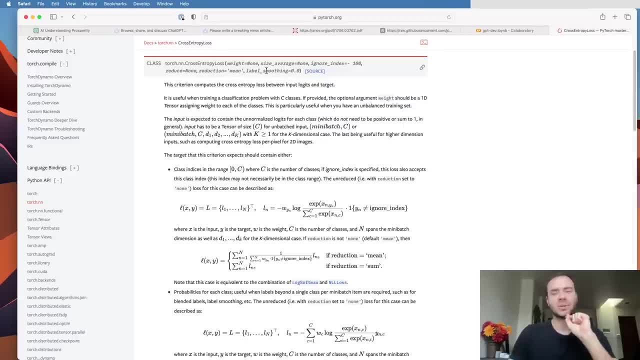 the issue here is: PyTorch expects, if you have multi-dimensional input, which we do because we have a b by t by c tensor- then it actually really wants the channels to be the second dimension here. So if you, So basically it wants a b by c by t instead of a b by t by c. 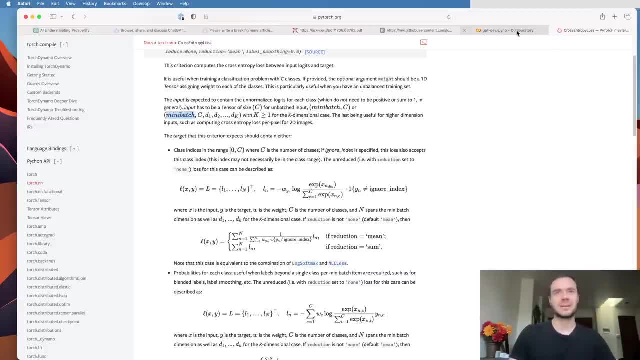 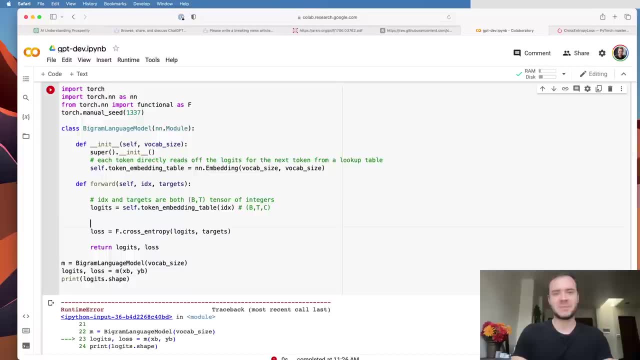 And so it's just the details of how PyTorch treats these kinds of inputs, And so we don't actually want to deal with that. So what we're going to do instead is we need to basically reshape our logits. So here's what I like to do. I like to take 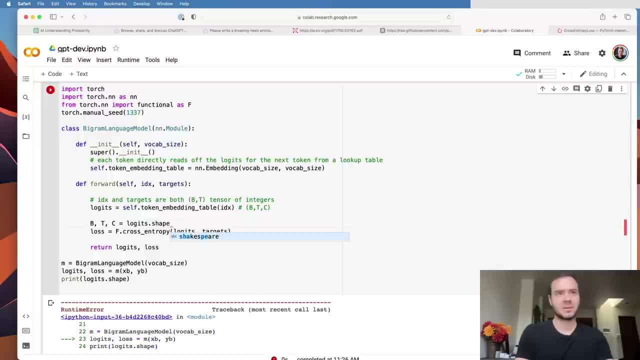 basically give names to the dimensions. So logitsshape is b by t by c, and unpack those numbers And then let's say that logits equals logitsview, And we want it to be a b times c, b times t by c, So just a two-dimensional array, right? So we're going to take all the 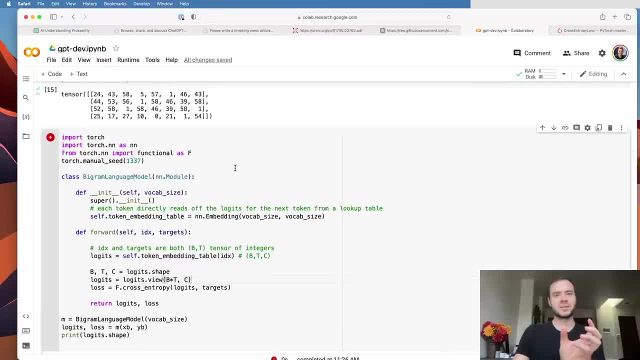 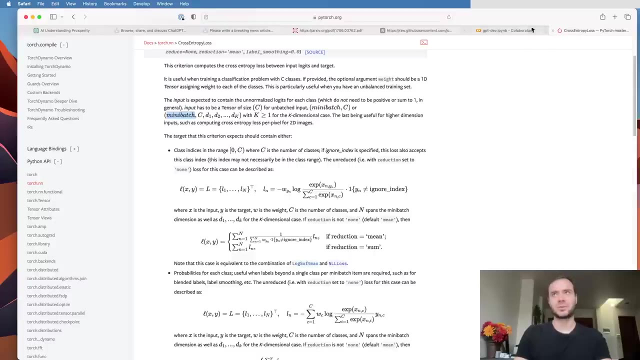 we're going to take all of these positions here and we're going to stretch them out in a one-dimensional sequence and preserve the channel dimension as the second dimension. So we're just kind of like stretching out the array so it's two-dimensional And in that case it's going to better conform to what PyTorch sort of expects in its dimensions. 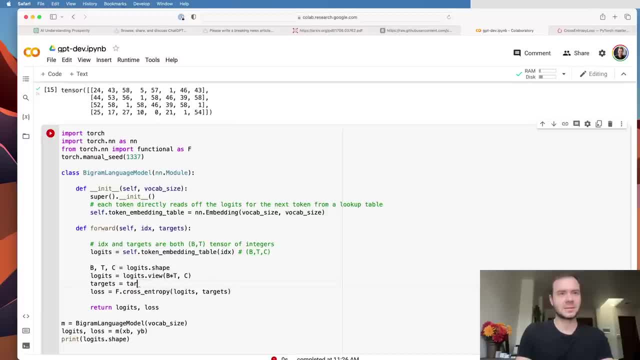 Now we have to do the same to targets, because currently targets are of shape b by t And we want it to be just b times t, So one-dimensional. Now. alternatively, you could always still just do minus one, because PyTorch will guess what this should be if you want to lay it out. 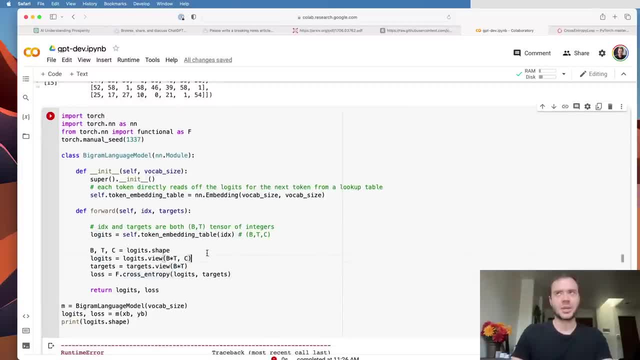 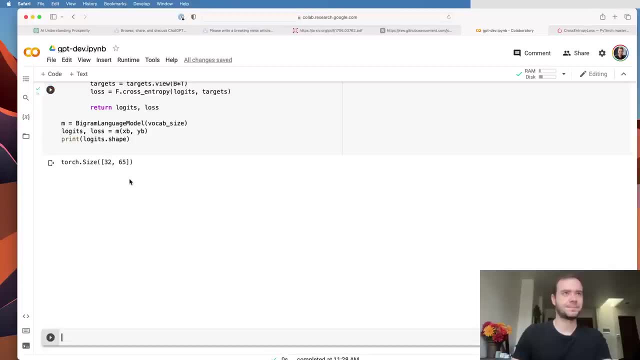 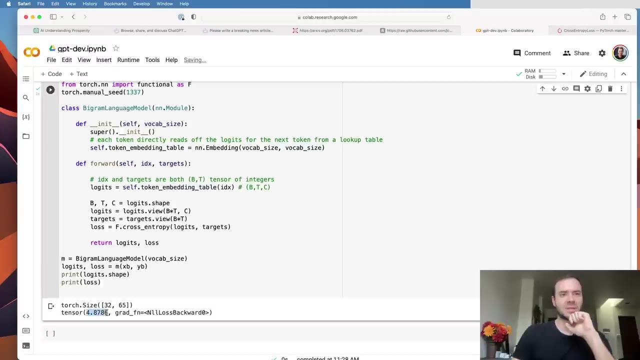 But let me just be explicit and say: b times t: Once we shape this, it will match the cross-entropy case and then we should be able to evaluate our loss. Okay, so with that right now, and we can do loss, And so currently we see that the loss is 4.87.. 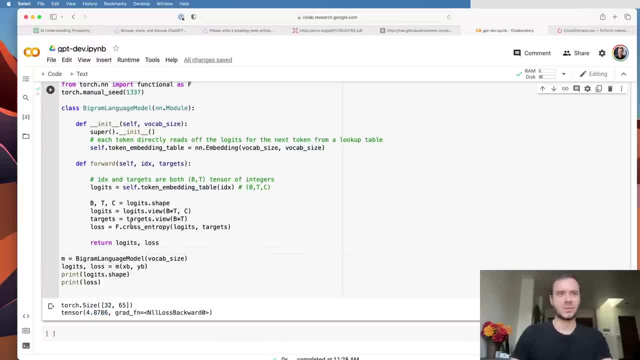 Now, because we have 65 possible vocabulary elements, we can actually guess at what the loss should be and in particular, we covered negative log likelihood in a lot of detail. We are expecting log or lon of 1 over 65 and negative of that. 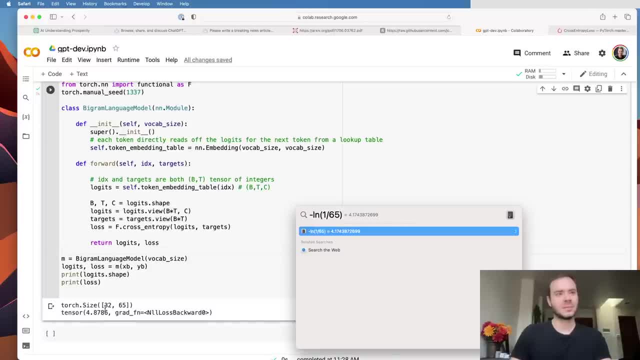 So we're expecting the loss to be about 4.17,, but we're getting 4.87,, and so that's telling us that the initial predictions are not super diffuse. they've got a little bit of entropy, and so we're guessing wrong. 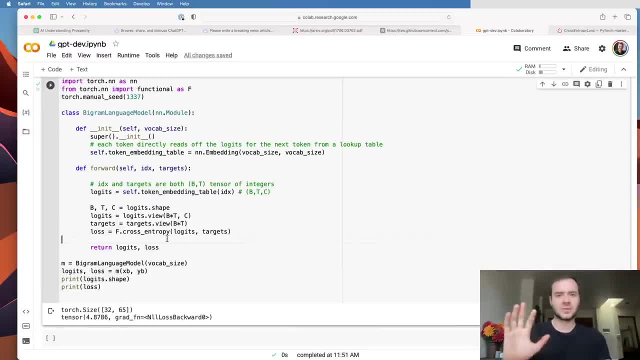 But actually we are able to evaluate the loss. Okay, so now that we can evaluate the quality of the model on some data we'd like to also be able to generate from the model, So let's do the generation Now. I'm going to go again a little bit faster here, because I covered all this already in. 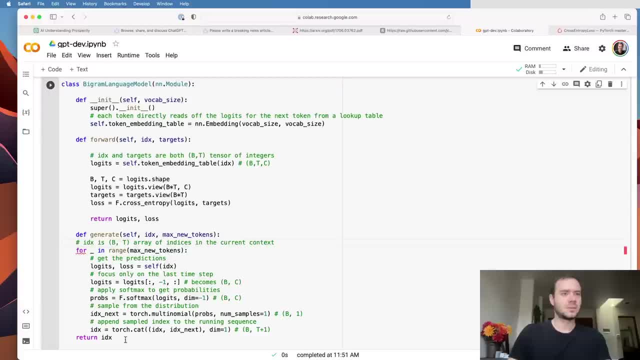 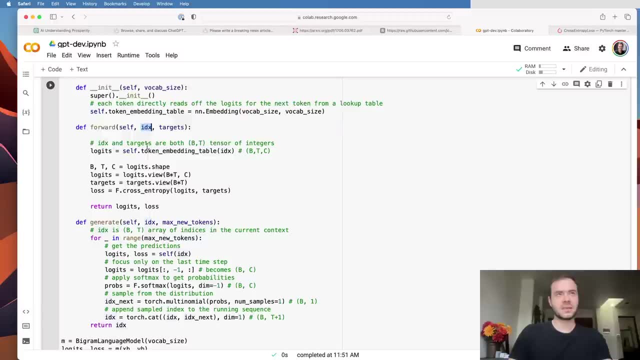 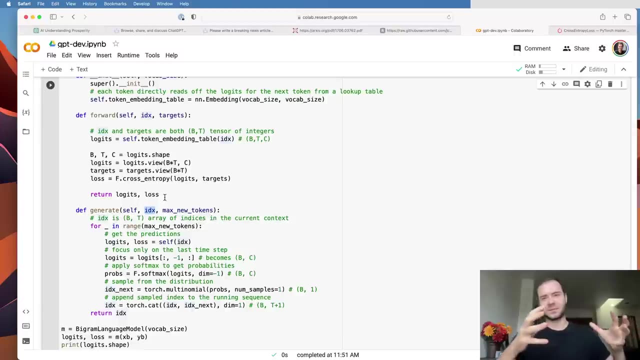 previous videos. So here's a generate function for the model. So we take the same kind of input idx- here and basically this is the current context of some characters in a batch, in some batch. So it's also b by t and the job of generate is to basically take this b by t and extend. 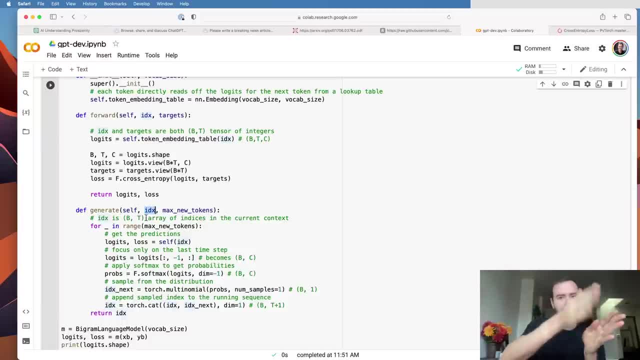 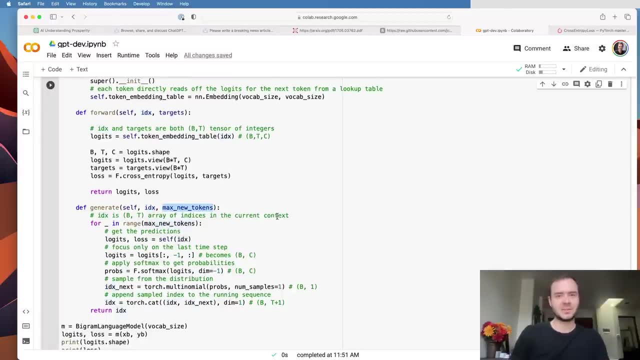 it to be b by t plus 1,, plus 2,, plus 3, and so it's just. basically it continues the generation in all the batch dimensions in the time dimension. So that's its job and it will do that for max new tokens. 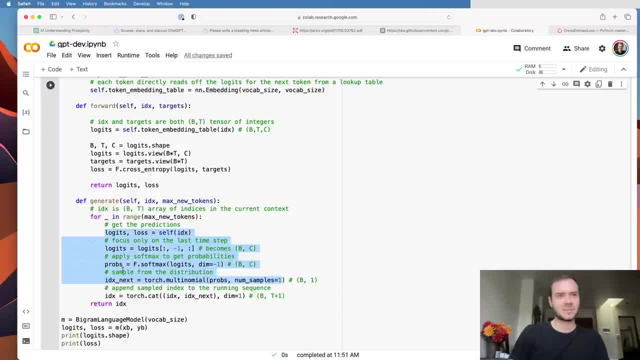 So you can see here on the bottom there's going to be some stuff here, but on the bottom whatever is predicted is concatenated on top of the previous idx along the first dimension, which is the time dimension to create a, b by t plus 1.. 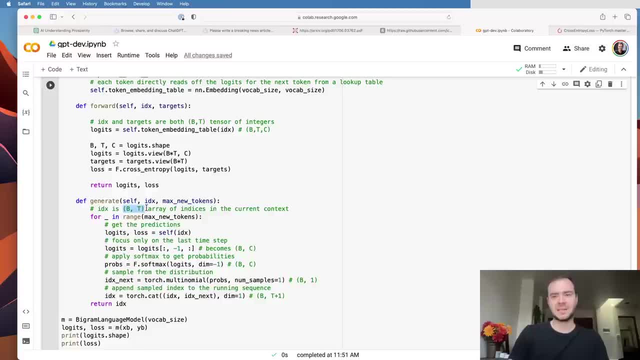 So that becomes a new idx. So the job of generate is to take a b by t and make it a b by t plus 1,, plus 2,, plus 3, as many as we want max new tokens. So this is the generation from the model. 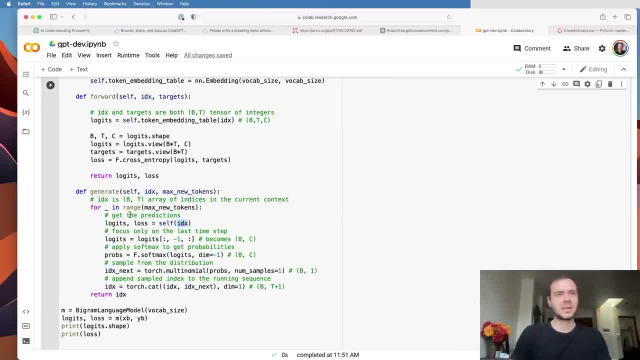 So what are we doing? We're taking the current indices, we're getting the predictions, So those are in the logits, and then the loss here is going to be ignored because we're not using that and we have no targets that are sort of ground truth, targets that we're 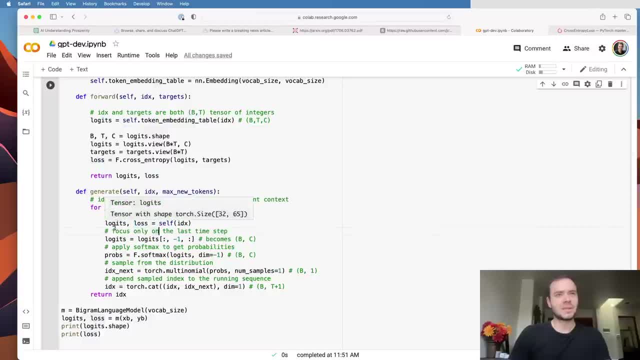 going to be comparing with. Then, once we get the logits, we are only focusing on the last step. So, instead of a, b by t, by c, we're going to pluck out the negative 1, the last element, 1, because those are the predictions for what comes next. 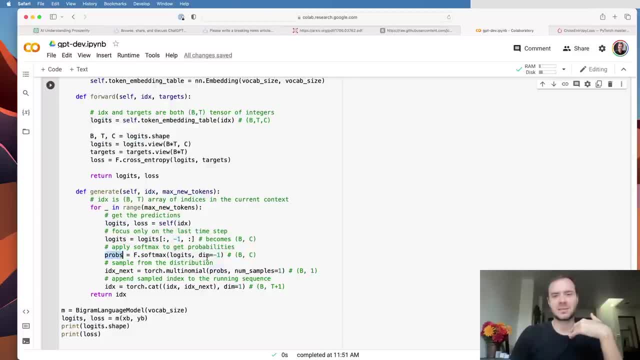 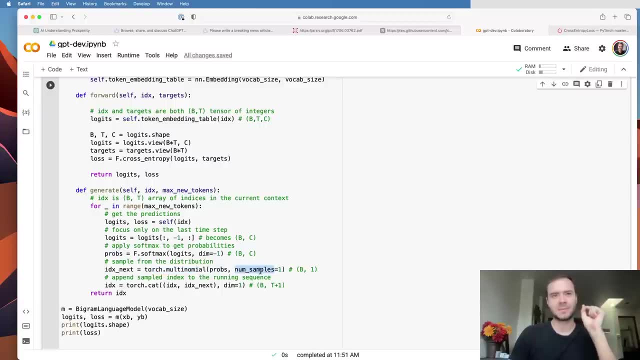 So that gives us the logits which we then convert to probabilities via softmax, and then we use torchmultinomial to sample from those probabilities and we ask pytorch to give us one sample, And so idx next will become a, b by 1, because in each one of the batch dimensions we're 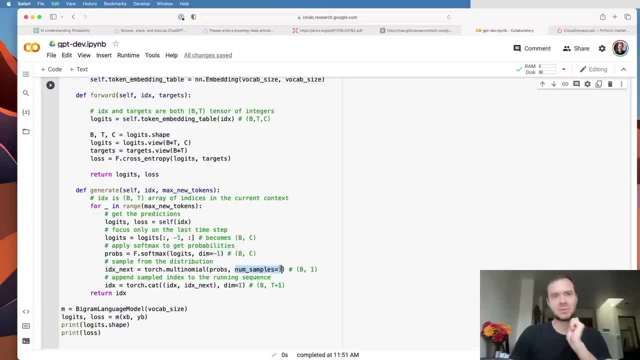 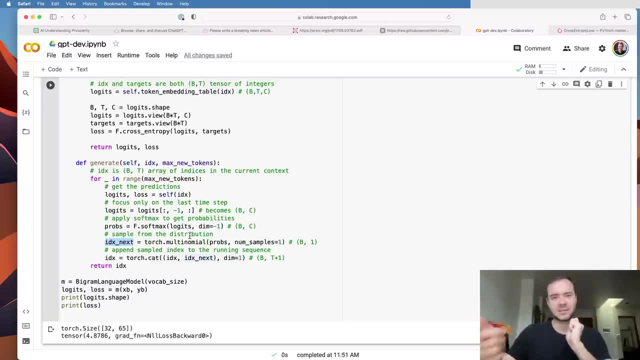 going to have a single prediction for what comes next. So this numSamples equals 1, will make this be a 1, and then we're going to take those integers That come from the sampling process according to the probability distribution given here. 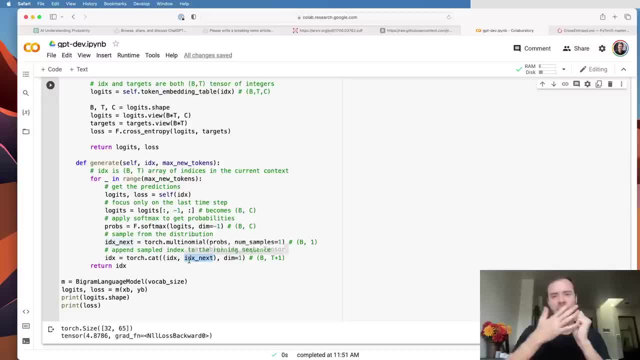 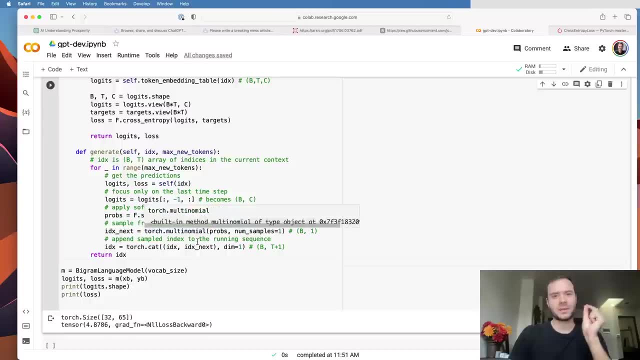 And those integers just get concatenated on top of the current sort of like running stream of integers And this gives us a b by t plus 1. And then we can return that. Now one thing here is: you see how I'm calling self of idx, which will end up going to the 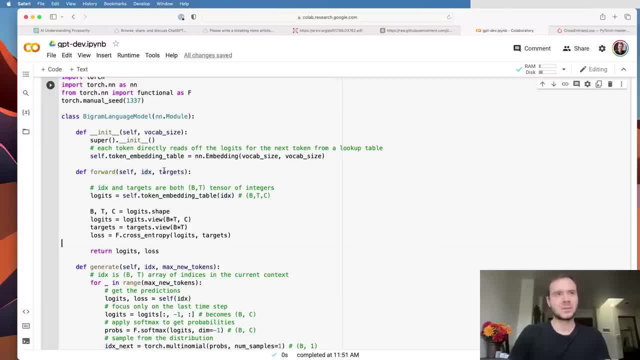 forward function. I'm not providing any targets, So currently this would give an error, because targets is sort of like not given, So targets has to be optional, So targets is none by default. And then if targets is none then there's no loss to create. 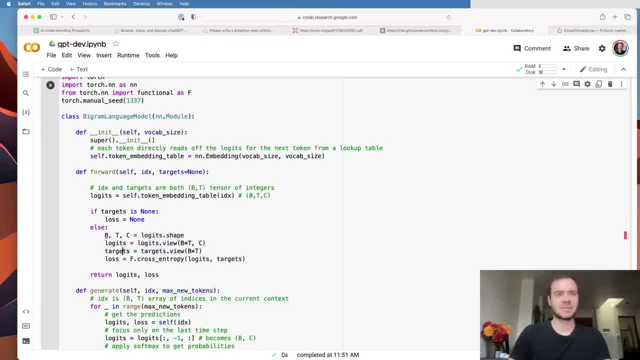 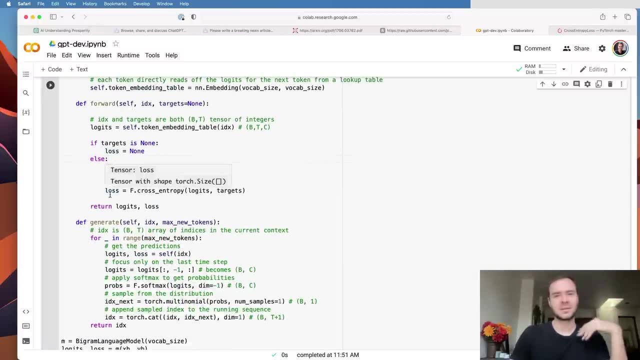 So it's just: loss is none, But else all of this happens and we can create a loss. So this will make it so: if we have the targets, we provide them and get a loss. If we have no targets, we'll just get the logits. 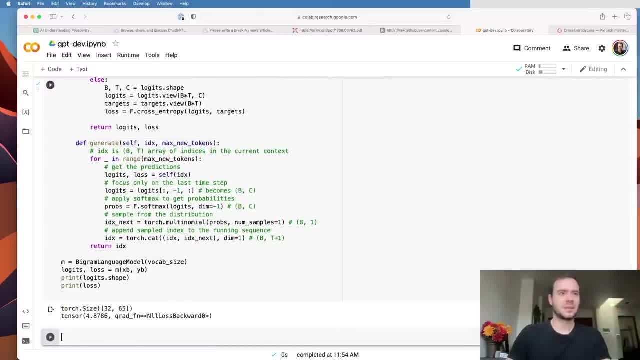 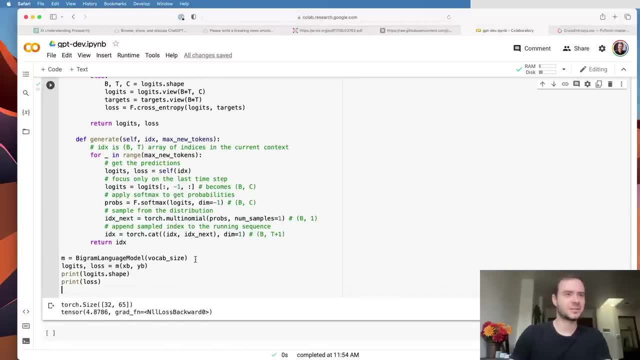 So this here will generate from the model, And let's take that for a right now. Okay, Okay, Oops. So I have another code chunk here which will generate for the model from the model, And okay, this is kind of crazy. 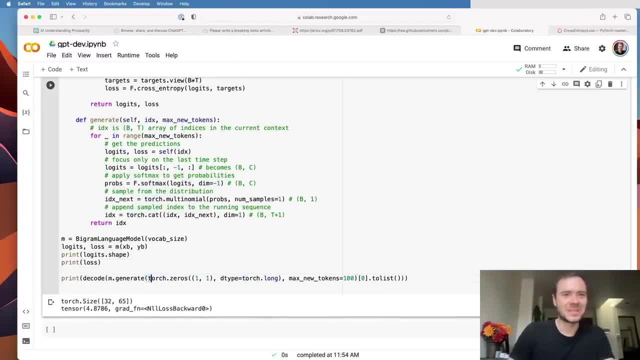 So maybe let me let me break this down. So these are the idx, right, I'm creating a batch will be just one, Time will be just one. So I'm creating a little one by one tensor and it's holding a zero. 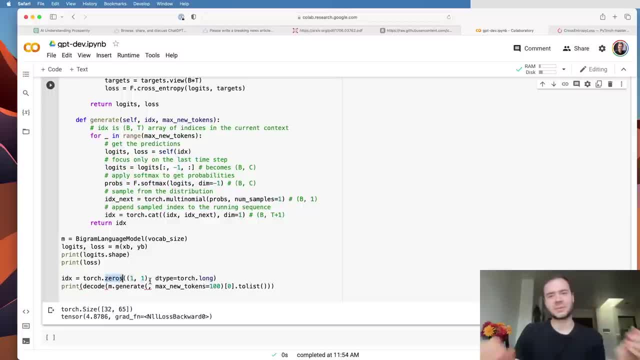 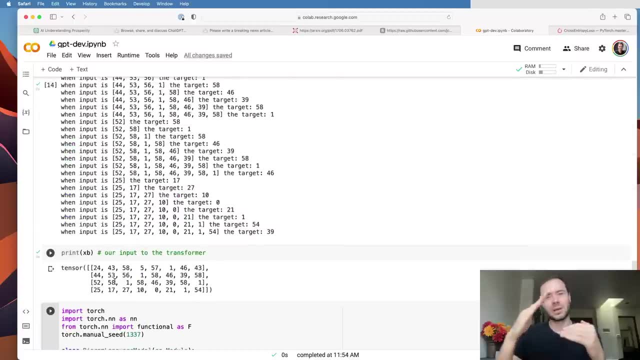 And the d type, the data type, is integer. So zero is going to be how we kick off the generator And remember that zero is is the element standing for a new line character. So it's kind of like a reasonable thing to to feed in as the very first character in. 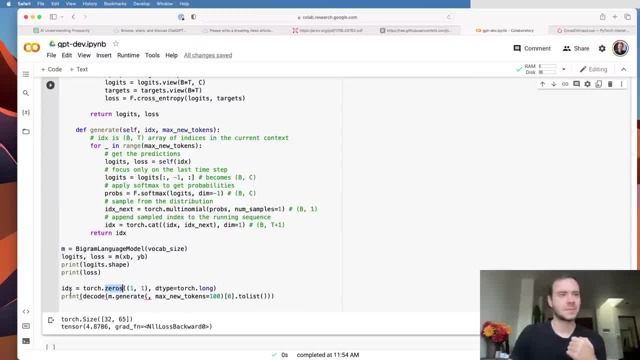 a sequence to be the new line. So it's going to be idx which we're going to feed in here. Then we're going to ask for 100 tokens and then end that generate. we'll continue that Now because generate works on the level of batches we either. we then have to index. 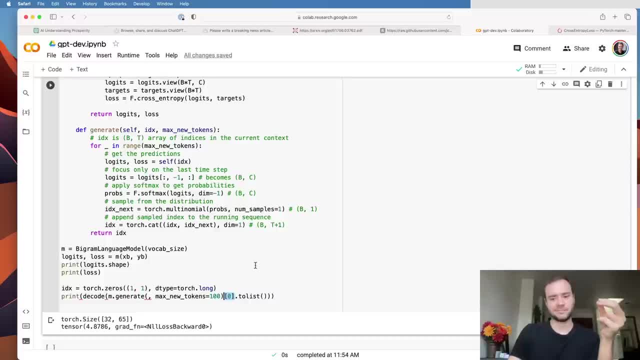 into the zero throw. So that's going to be very difficult to basically unplug the. the single batch dimension that exists And then that gives us a time steps is just a one dimensional array of all the indices which we will convert to simple Python list from PyTorch tensor so that that can feed. 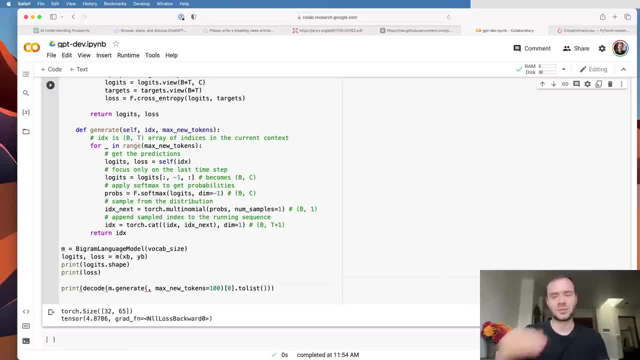 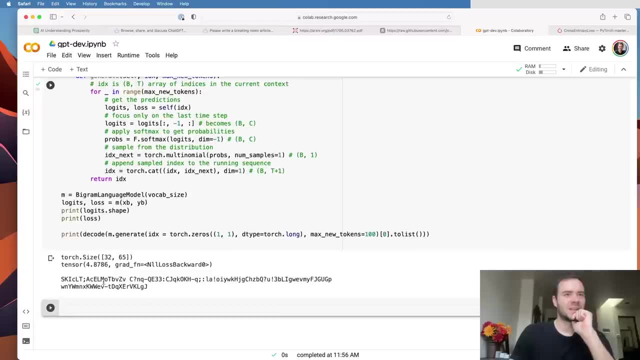 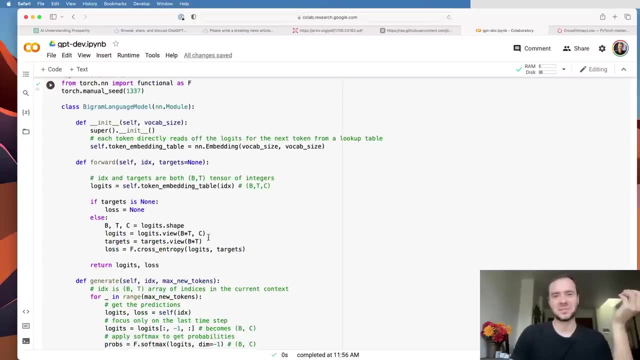 into our decode function and convert those integers into text. So let me bring this back. and we're generating a hundred tokens. Let's run and here's the generation that we achieved. so obviously it's garbage. and the reason it's garbage is because this is a totally random model. so next up, we're going to want to train this model. 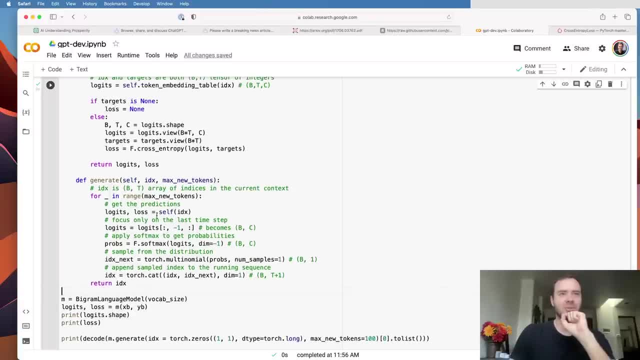 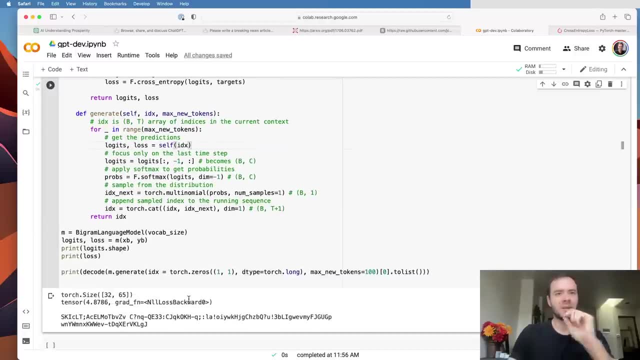 now. one more thing i wanted to point out here is: this function is written to be general, but it's kind of like ridiculous right now because we're feeding in all this, we're building out this context and we're concatenating it all, and we're always feeding it all into the model. 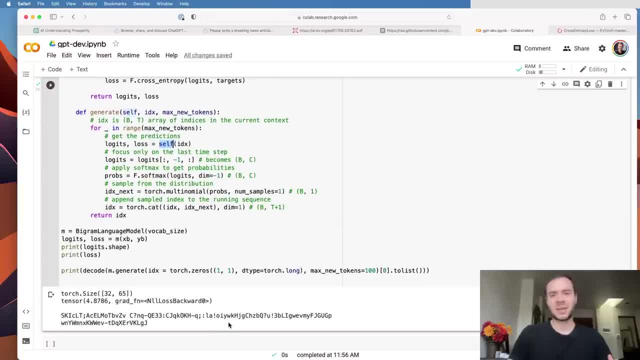 but that's kind of ridiculous, because this is just a simple bigram model. so to make, for example, this prediction about k, we only needed this w. but actually what we fed into the model is we fed the entire sequence and then we only looked at the very last piece and predicted k. so the only reason 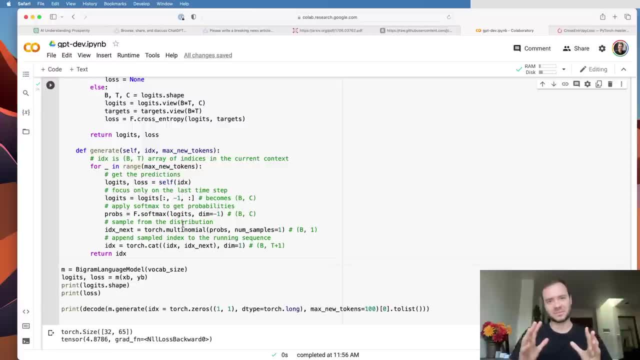 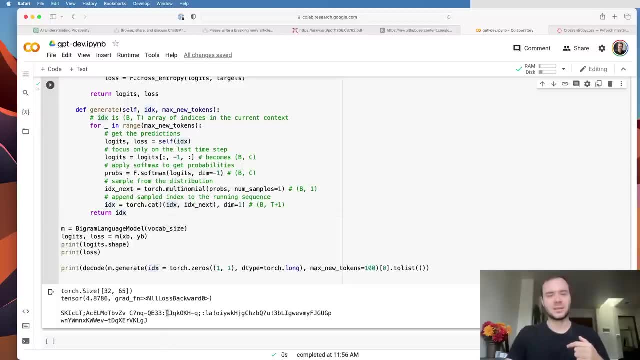 i'm writing it in this way is because right now this is a bigram model, but i'd like to keep this function fixed and i'd like it to work later, when our characters actually basically look different from each other, and so we're going to want to keep this function fixed and we're going 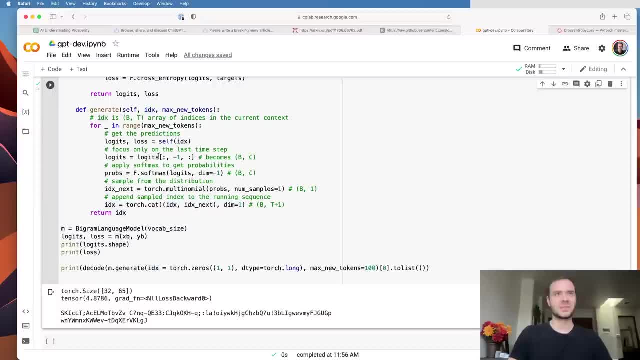 to want to keep this function fixed. and we're going to want to keep this function fixed and we're going further in the history, and so right now the history is not used, so this looks silly, but eventually the history will be used, and so that's why we want to do it this way. so just a quick. 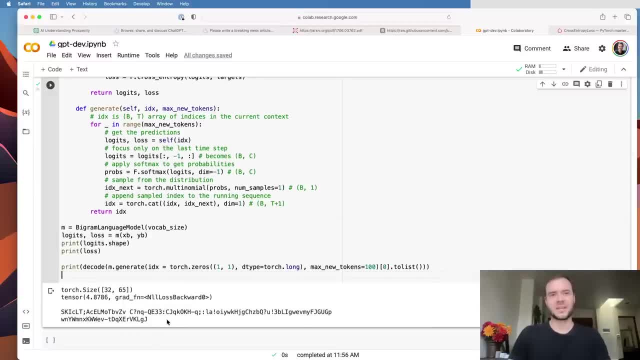 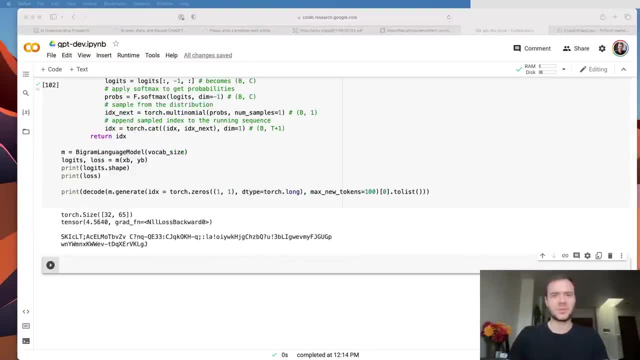 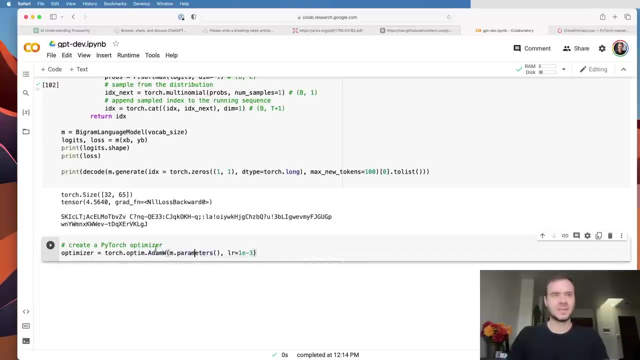 comment on that. so now we see that this is random. so let's train the model so it becomes a bit less random. okay, let's now train the model. so first, what i'm going to do is i'm going to create a pytorch optimization object. so here we are, using the optimizer atom w, now in a make more series, we 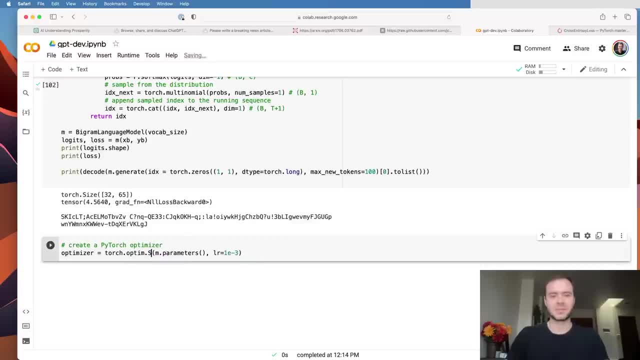 only ever use stochastic gradient descent, the simplest possible optimizer which you can get using the sgd instead. but i want to use atom, which is a much more advanced and popular optimizer and it works extremely well for a typical good setting, for the learning rate is roughly 3e. 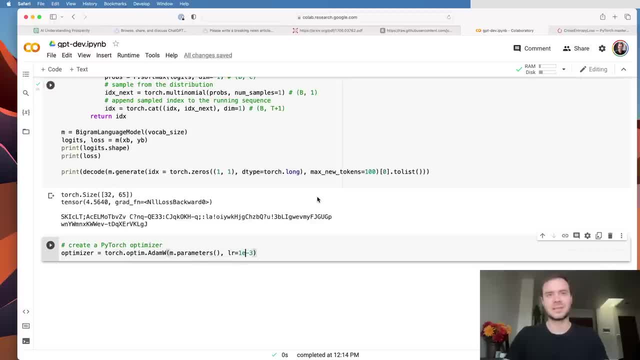 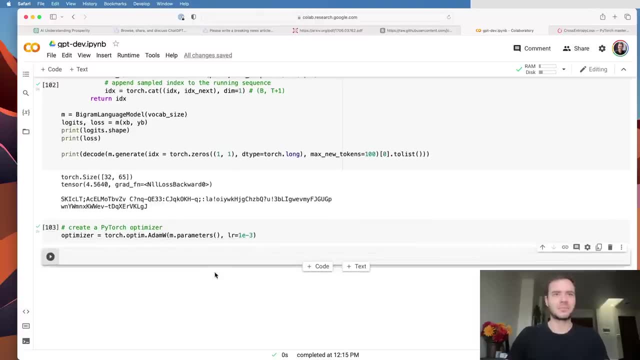 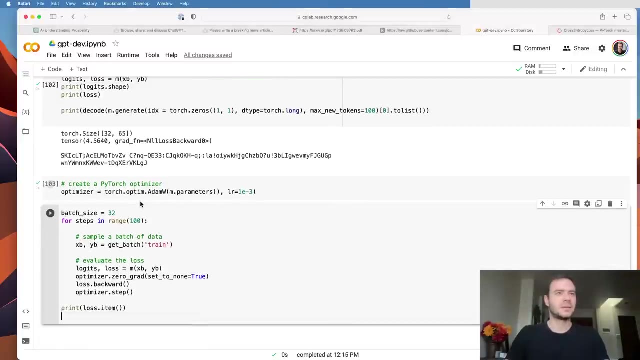 negative 4. but for very, very small networks, like it's the case here, you can get away with much, much higher learning rates, wanting negative 3 or even higher probably. but let me create the optimizer object which will basically take the gradients and update the parameters using the gradients. and then here our batch size up above was only four, so let me actually use 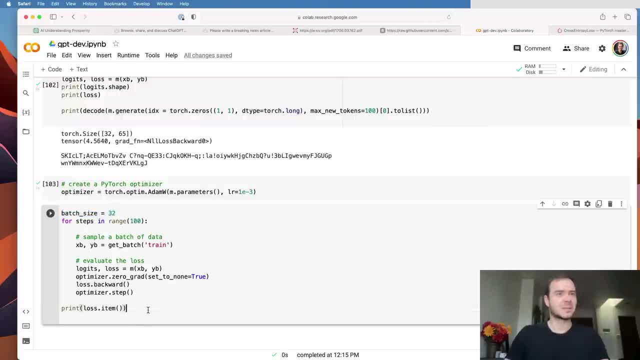 something bigger, let's say 32, and then, for some number of steps, we are sampling a new batch of data, we're evaluating the loss, we're zeroing out all the gradients from the previous step, getting the gradients for all the parameters and then using those gradients to update our 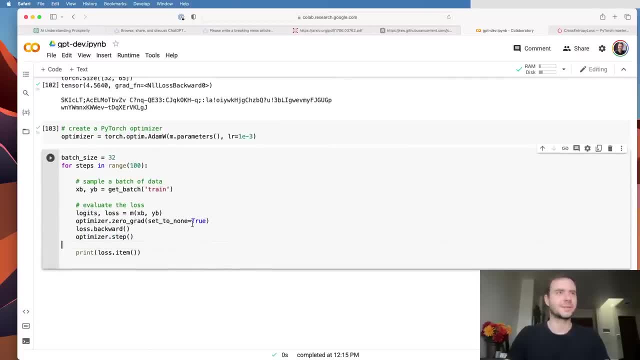 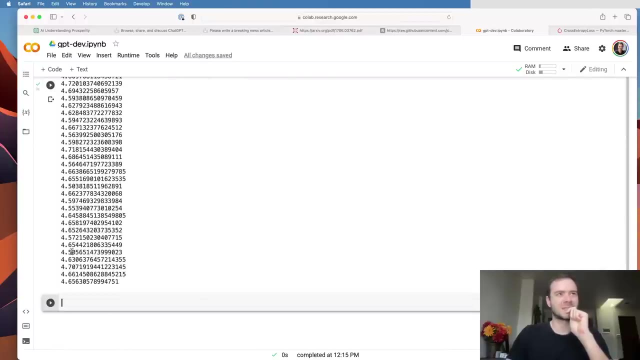 parameters. so typical training loop, as we saw in the make more series. so let me now run this for, say, 100 iterations and let's see what kind of losses we're going to get. so we started around 4.7 and now we're getting down to like 4.6, 4.5 etc. so the optimization 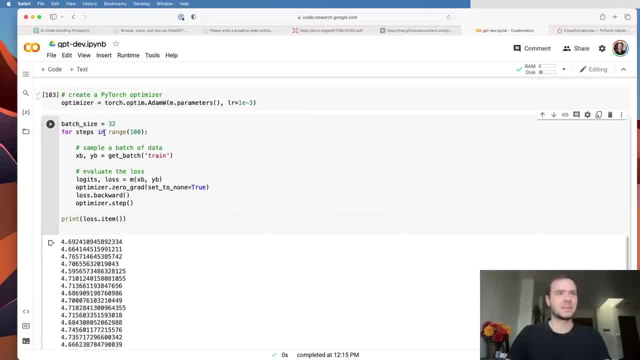 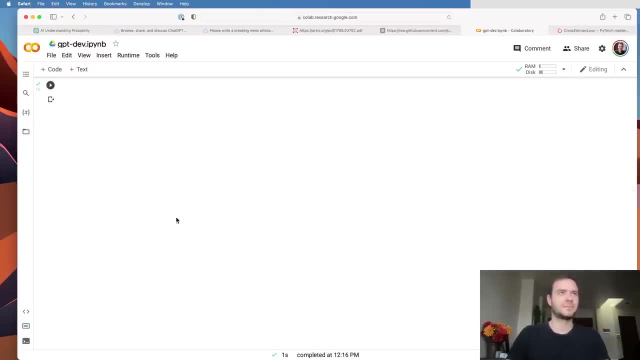 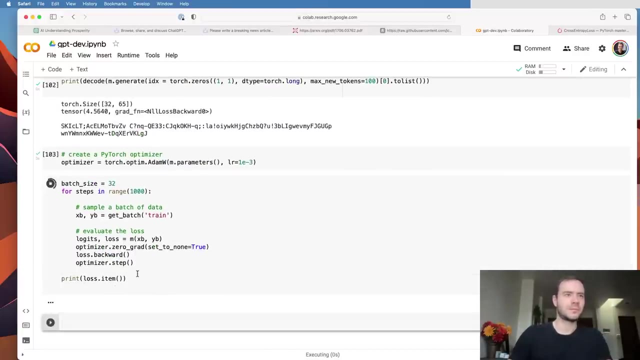 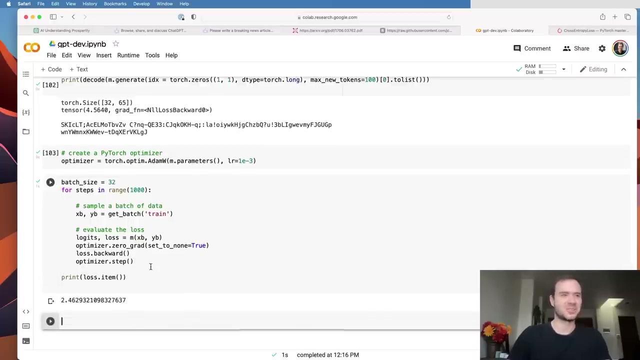 is definitely happening, but let's sort of try to increase the number of iterations and only print at the end, because we probably will not train for longer. okay, so we're down to 3.6, roughly, roughly down to three. this is the most janky optimization. 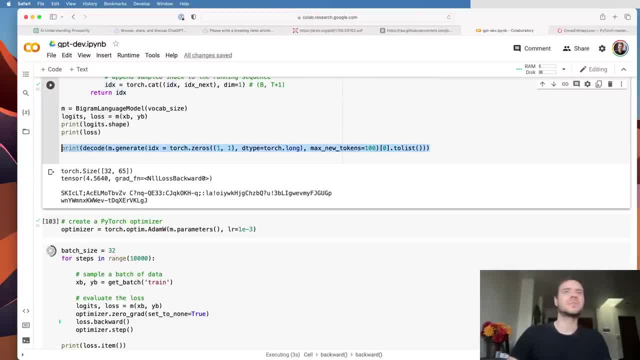 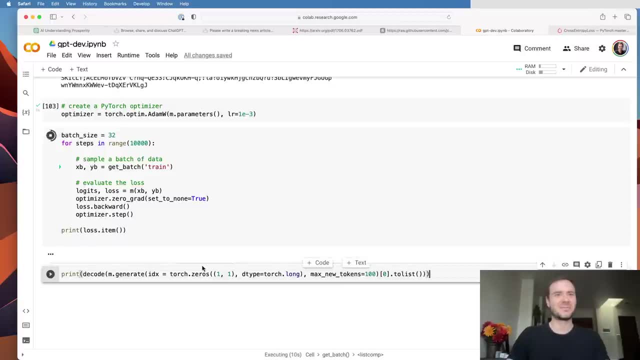 okay, it's working. let's just do 10 000 and then from here we want to copy this and hopefully we're going to get something reasonable, and of course it's not going to be shakespeare from a background model, but at least we see that the loss is improving. 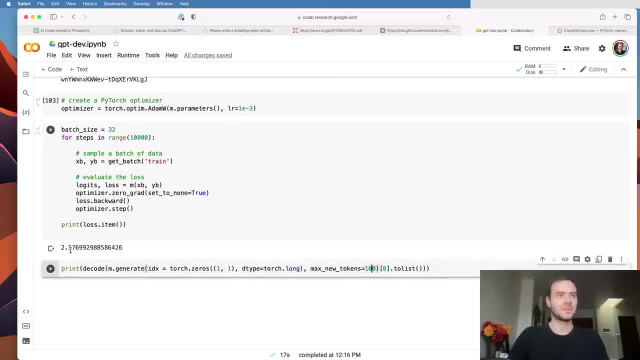 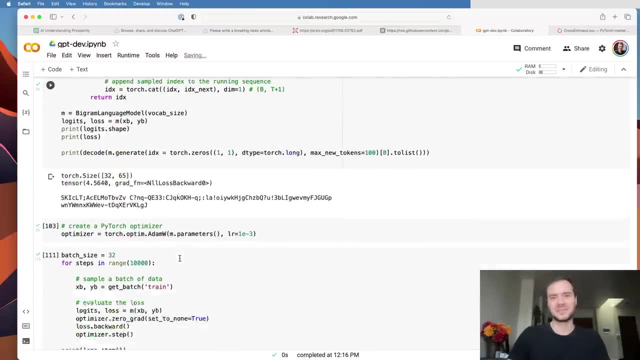 Hopefully we're expecting something a bit more reasonable. Okay, so we're down at about 2.5 ish. Let's see what we get. Okay, Dramatic improvement, certainly, on what we had here. So let me just increase the number of tokens. Okay. so we see that we're starting to get something at least like 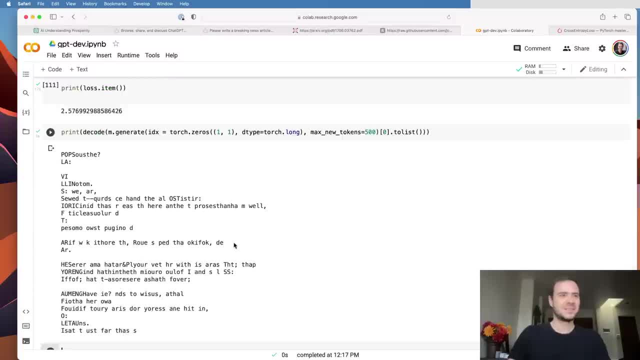 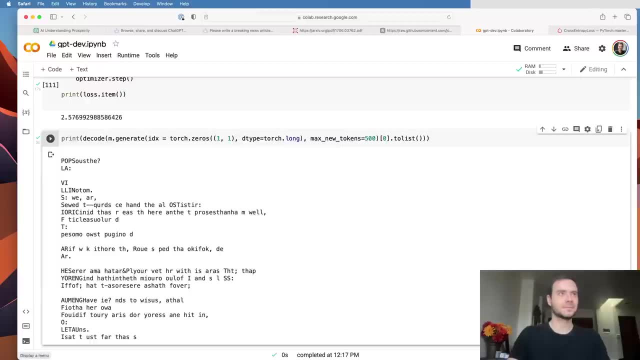 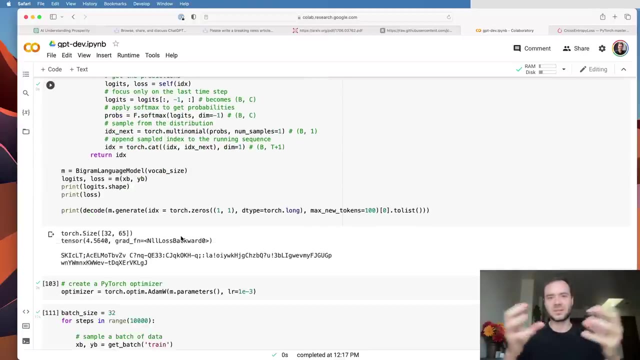 Reasonable ish? Certainly not Shakespeare, but the model is making progress, So that is the simplest possible model. so now what I'd like to do is, Obviously, that this is a very simple model because the tokens are not talking to each other. So, given the previous context of whatever was generated, 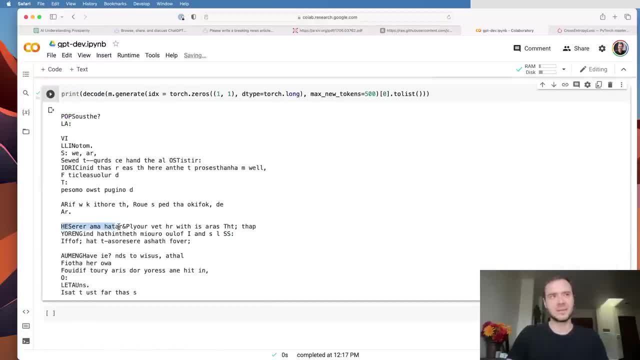 We're only looking at the very last character to make the predictions about what comes next. So now these, now these tokens have to start talking to each other and figuring out what is in the context So that they can make better predictions for what comes next. and this is how we're gonna kick off the transformer. 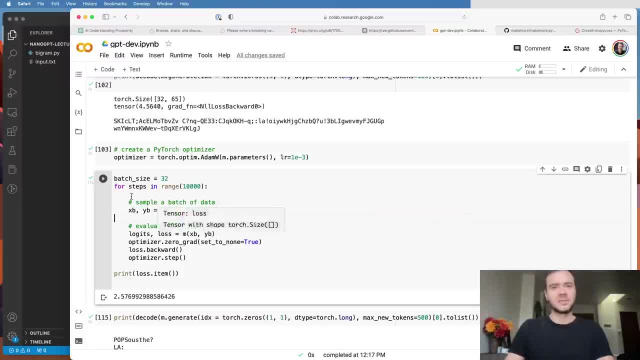 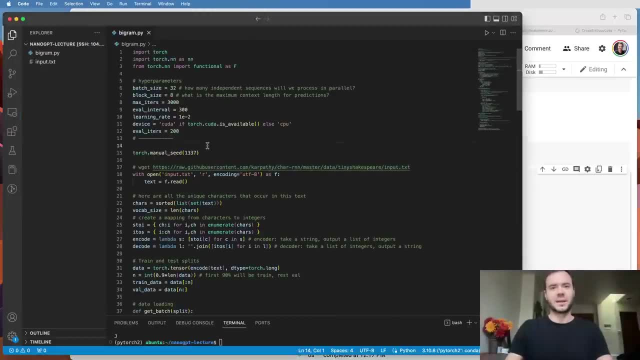 Okay. So next, I took the code that we developed in This Jupyter notebook and I converted it to be a script, and I'm doing this because I just want to simplify our intermediate work, Which is just the final product that we have at this point. So in the top here I put all the hyperparameters that we defined. 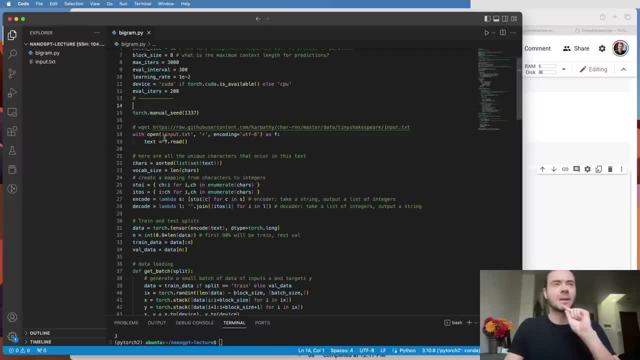 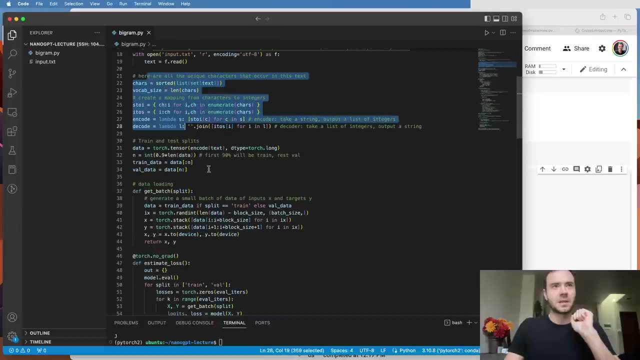 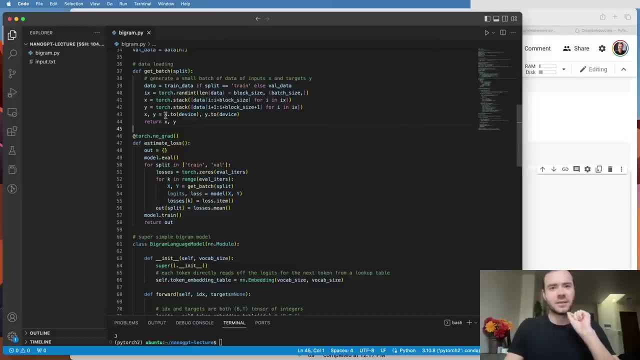 I introduced a few and I'm going to speak to that in a little bit. Otherwise, a lot of this should be recognizable: reproducibility, Read data. get the encoder in the decoder, create the train and test splits. Use the kind of like data loader That gets a batch of the inputs and targets. 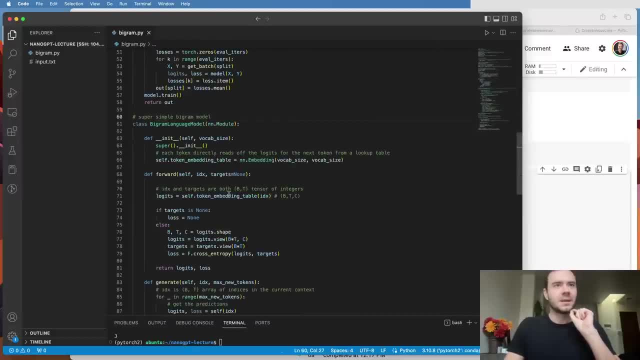 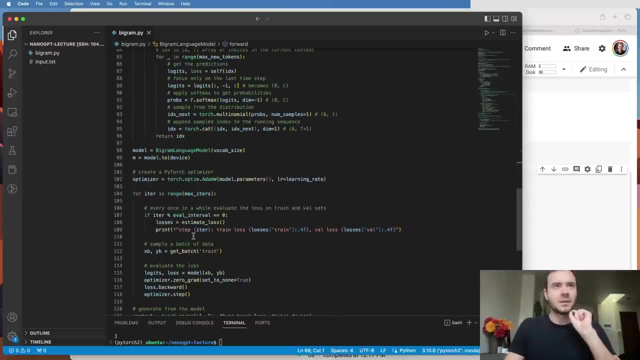 This is new and I'll talk about it in a second. now, this is the background language model that we developed and it can forward and give us a logits and loss and it can generate, and Then here we are, creating the optimizer, and this is the training loop. 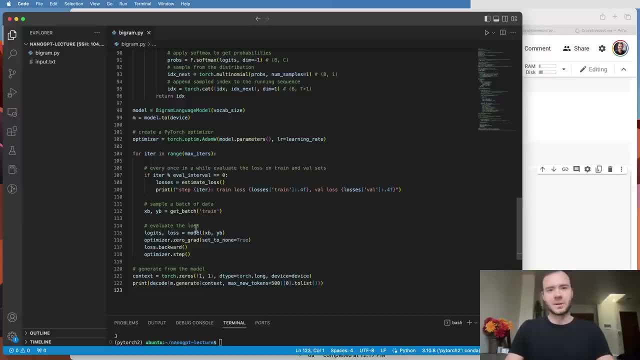 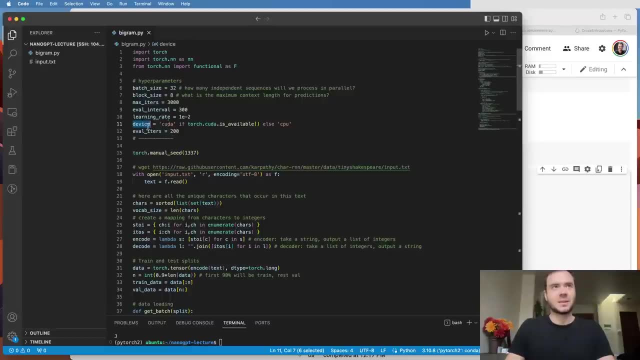 So everything here should look pretty familiar. now some of the small things that I added. number one: I added the ability to run on a GPU, if you have it. So if you have it, Then you can. this will use CUDA instead of just CPU, and everything will be a lot more faster. 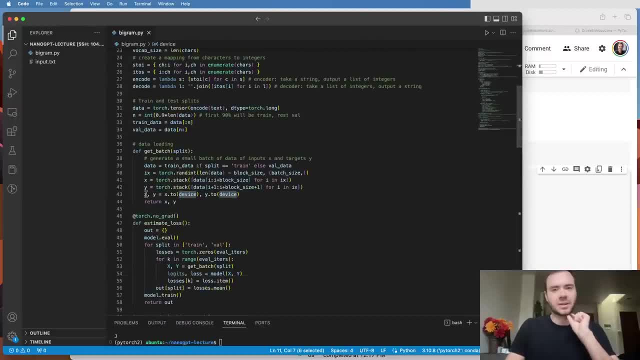 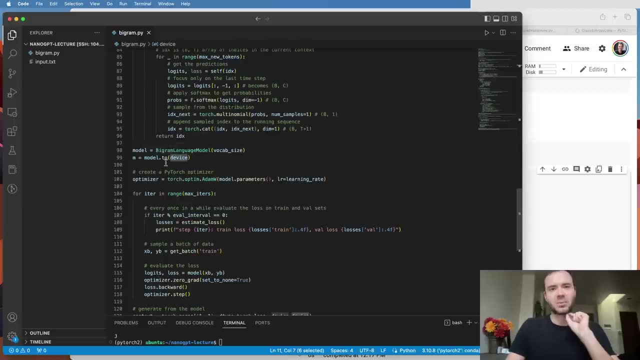 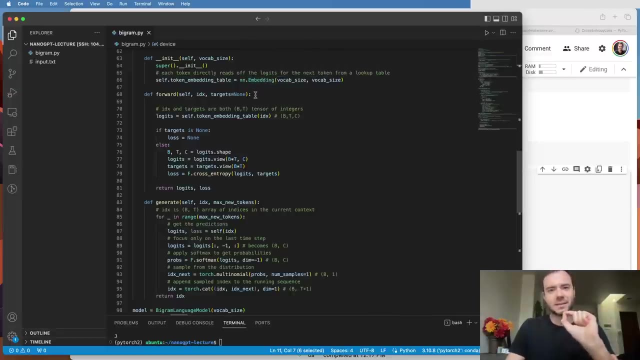 Now, when device becomes CUDA, then we need to make sure that when we load the data we move it to device. When we create the model, we want to move the model parameters to device. so as an example, Here we have the NN embedding table and it's got a dot weight inside it which stores the sort of lookup table. 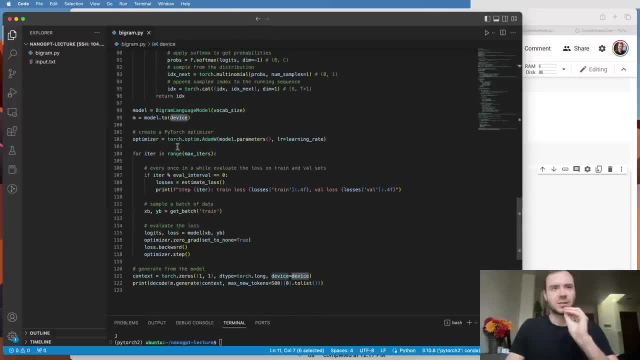 So that would be moved to the GPU so that all the calculations here happen, The GPU and they can be a lot faster. and then finally, here when I'm creating the context that feeds in to generate, I have to make sure that I create on the device. number two, when I introduced, is: 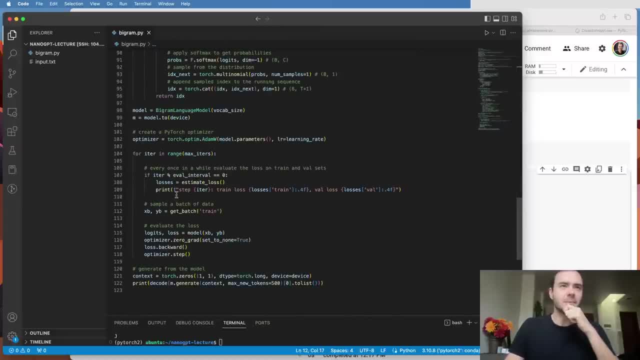 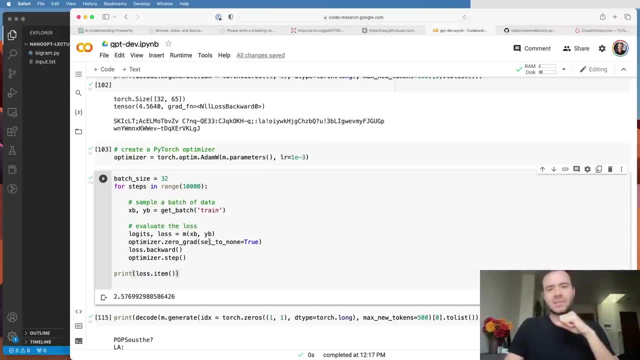 The fact that here in the training loop Here I was just printing the loss dot item Inside the training loop. but this is a very noisy measurement of the current loss, because every batch will be more or less lucky, and so what I want to do usually is: 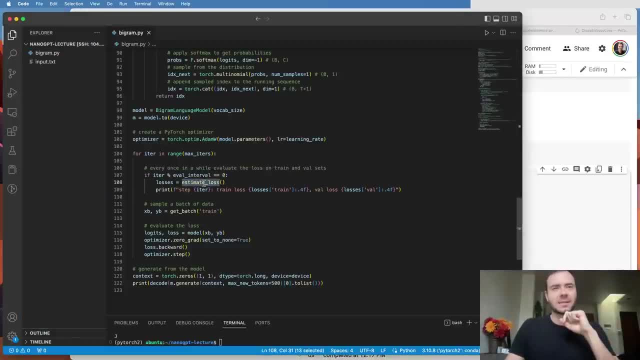 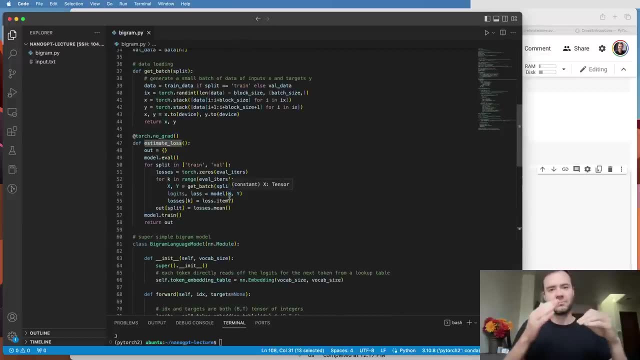 I have an estimate loss function and the estimate loss basically then goes up here and It averages up the loss over multiple batches. So in particular, we're going to iterate eval iter times And we're going to basically get our loss and then we're going to get the average loss for both splits. 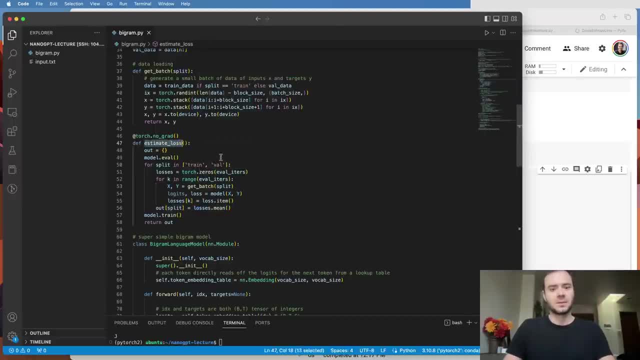 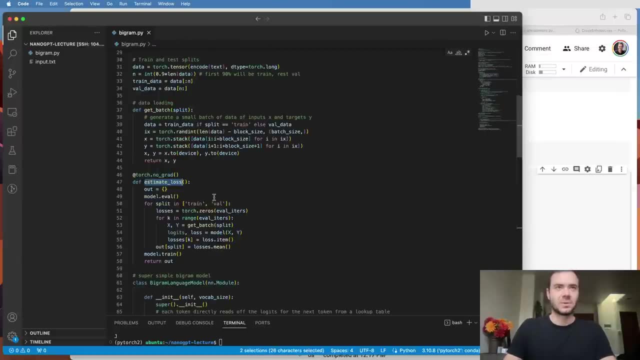 And so this will be a lot less noisy. So here, when we call the estimate loss, we're going to report the pretty accurate train and validation loss. Now, when we come back up, you'll notice a few things. here I'm setting the model to evaluation phase and down here. 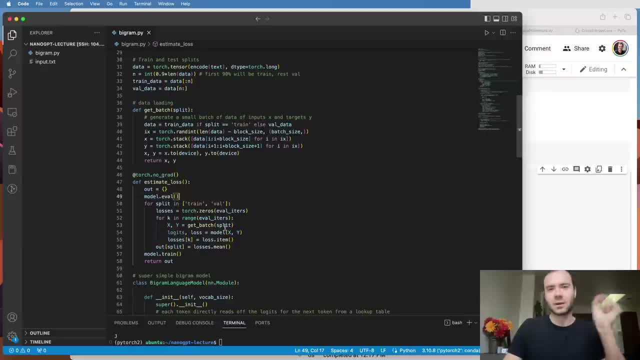 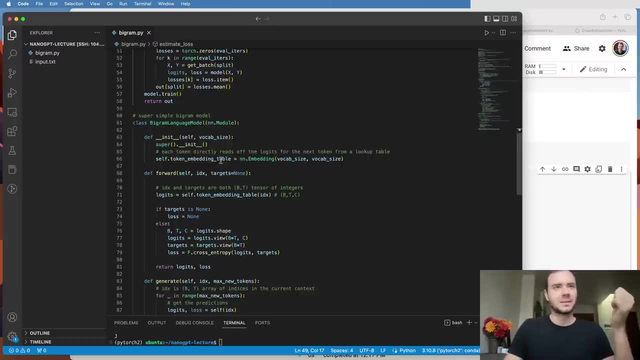 I'm resetting it back to training phase now, right now, for our model, as is, this doesn't actually do anything, because the only thing inside this model is this and end up embedding, and this this Network would behave. both would behave the same, in both evaluation mode and training mode. We have no dropout layers. 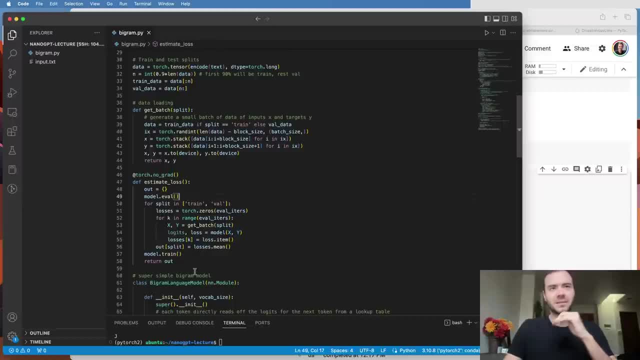 We have no bathroom layers etc. But it is a good practice to think through What mode your neural network is in, because some layers will have different behavior at inference time or training time. and There's also this context, manager torchnograd, and this is just telling pytorch that everything that happens inside this function, we will not call dot backward on and 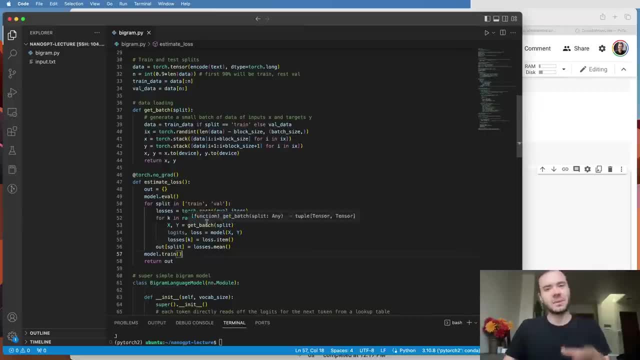 So pytorch can be a lot more efficient with its memory use because it doesn't have to store all the intermediate variables, Because we're never going to call backward and so it can. it can be a lot more memory efficient in that way. So also a good practice to tell pytorch when we don't intend to do back propagation. 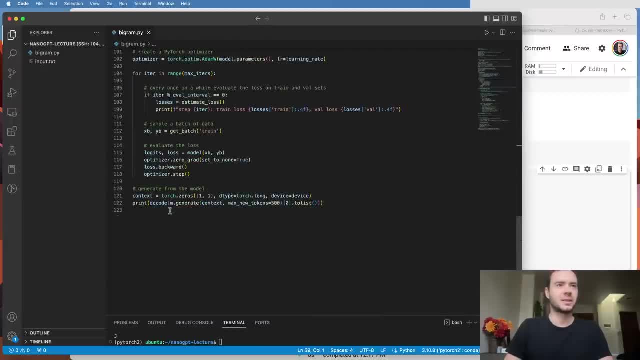 So right now this script is about a hundred and twenty lines of code of- and that's kind of our starter code. I'm calling it mygrampy and I'm going to release it later now. running this script Gives us output in the terminal and it looks something like this: 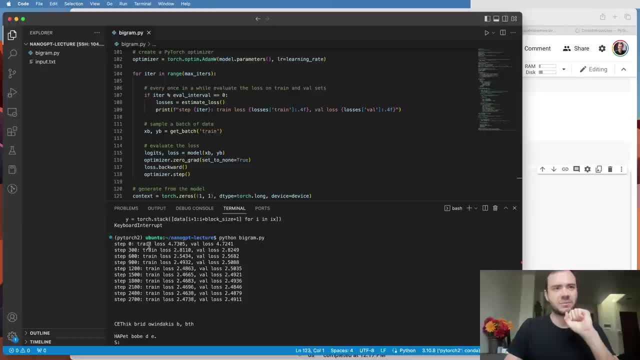 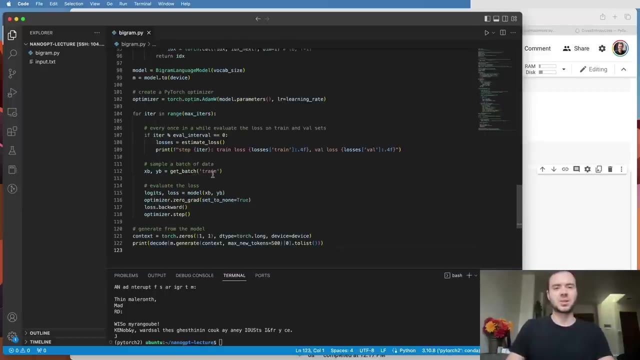 It. basically, as I ran this code, It was giving me the train loss and the val loss, and we see that we convert to somewhere around 2.5 with the by grant model. and then here's the sample that we produced at the end, and So we have everything packaged up in the script and we're in a good position now to iterate on this. 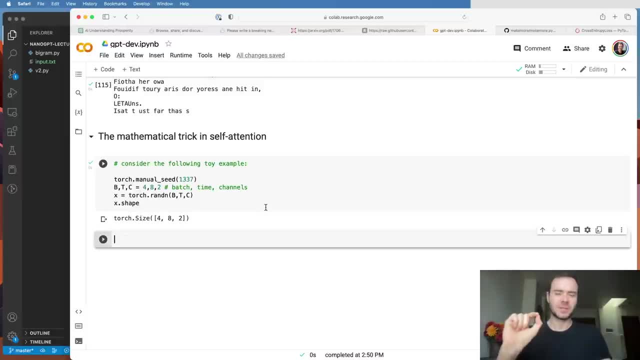 Okay, so we are almost ready to start writing our very first self attention block for processing these tokens. now, before we actually get there, I want to get you used to a mathematical trick that is used in the self attention inside a transformer and is really just like at: 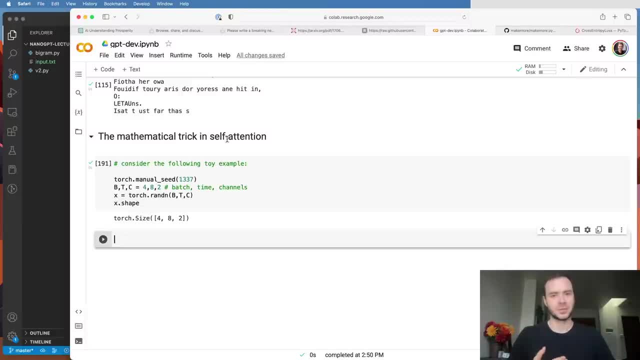 the heart of an in a efficient implementation of self-attention, And so I want to work with this toy example to just get you used to this operation, and then it's going to make it much more clear once we actually get to it in the script. 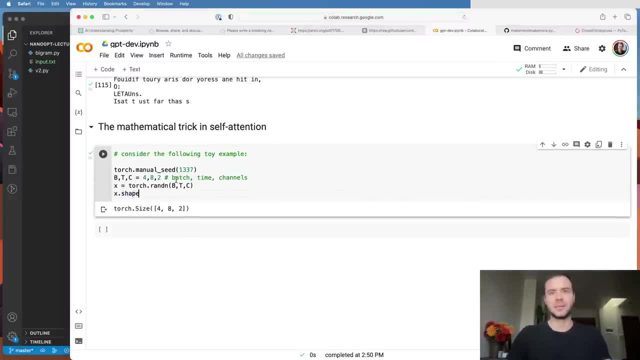 again. So let's create a B by T by C, where B, T and C are just 4,, 8 and 2 in this toy example, And these are basically channels and we have batches and we have the time component and we have some information at each point in the. 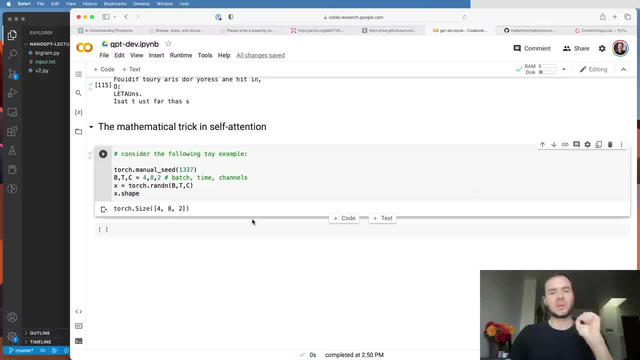 sequence. so C. Now, what we would like to do is we would like these tokens. so we have up to eight tokens here in a batch and these eight tokens are currently not talking to each other, and we would like them to talk to each other. We'd like to. 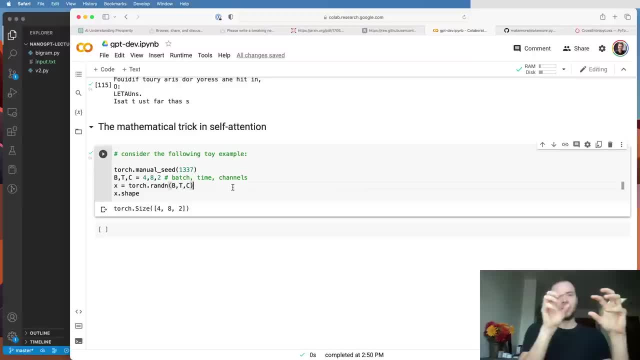 couple them And, in particular, we want to couple them in this very specific way. So the token, for example, at the fifth location. it should not communicate with tokens in the sixth, seventh and eighth location, because those are future tokens In the sequence. the token on the fifth location should only talk to the one in 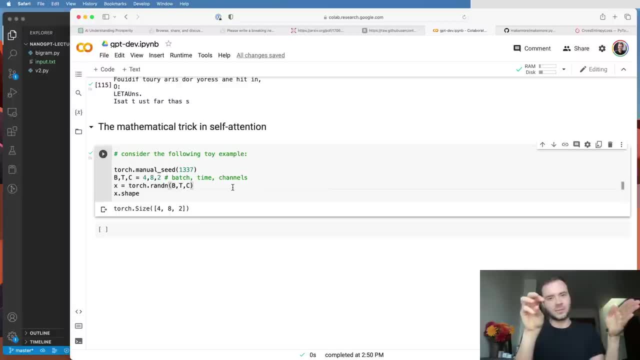 the fourth, third, second and first. So it's only so. information only flows from previous context to the current time step, and we cannot get any information from the future because we are about to try to predict the future. So what is the easiest way for tokens to communicate? Okay, the easiest way, I would say, is okay. 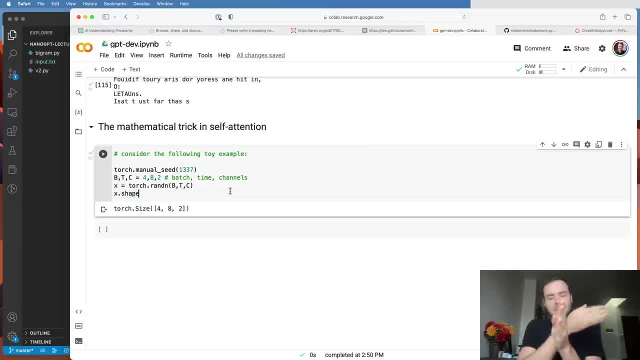 if we are up to, if we're a fifth token and I'd like to communicate with my past, the simplest way we can do that is, if we are up to, if we're a fifth token and I'd like to communicate with my past, the simplest way we can do that. 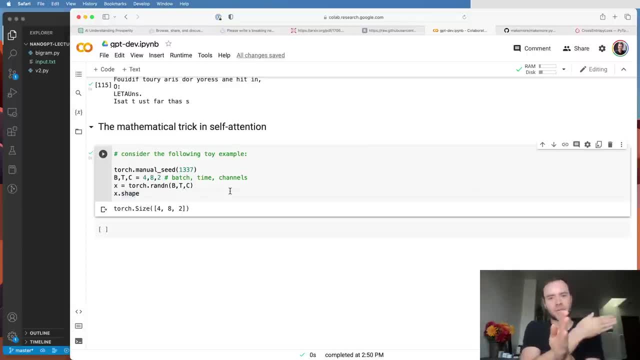 is to just do a weight, is to just do an average of all the, of all the preceding elements. So, for example, if I'm the fifth token, I would like to take the channels that make up that, our information at my step, but then also the 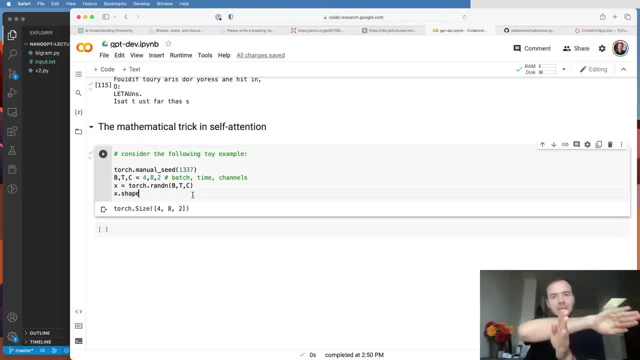 channels from the fourth step, third step, second step and the first step. I'd like to average those up, and then that would become sort of like a feature vector that summarizes me in the context of my history. Now, of course, just doing a sum. 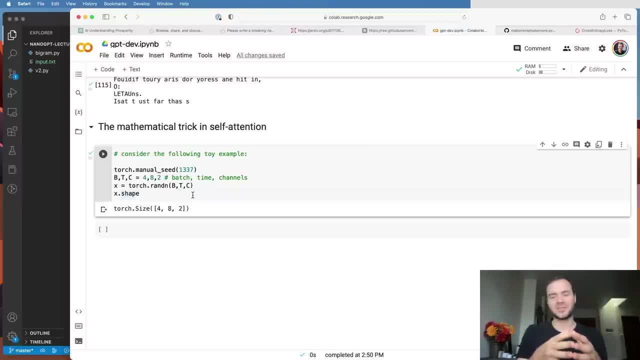 or like an average is an extremely easy thing to do, But if you're not familiar with the, the sum or like an average is an extremely easy thing to do, But if you're not familiar with the weak form of interaction like this, communication is extremely lossy. we've 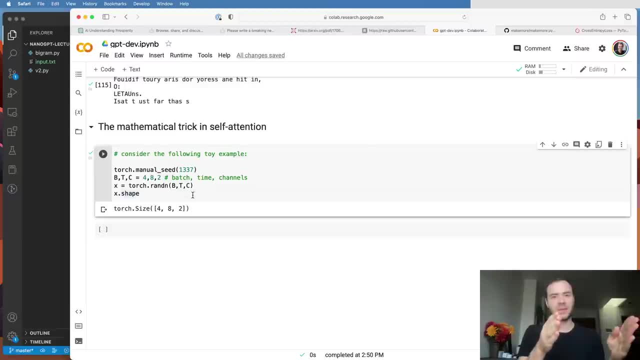 weak form of interaction like this communication is extremely lossy. we've lost a ton of information about the spatial arrangements of all those tokens, but that's okay for now. we'll see how we can bring that information back later. For now, what we would like to do is for every single batch element independently. 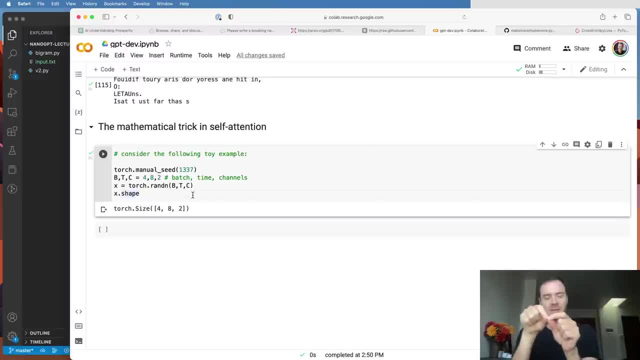 for every teeth token in that sequence. we'd like to now calculate the average of all the vectors in all the previous tokens and also at this token. So let's write that out. So let's write that out. I have a small snippet here and instead of just fumbling around, let me just copy. 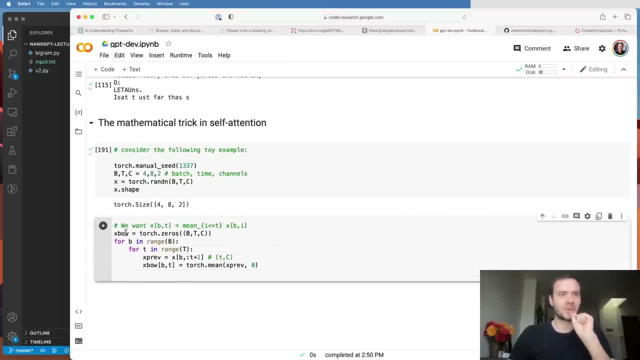 I have a small snippet here and instead of just fumbling around, let me just copy paste it and talk to it. So, in other words, we're going to create X, and BOW is short for bag of words, because bag of words is is kind of like a term that. 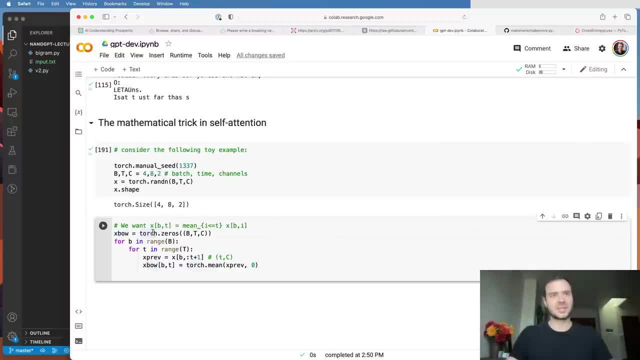 people use when you are just averaging up things. So this is just a bag of words. basically, there's a word stored on every one of these eight locations and we're doing a bag of words, just averaging. So in the beginning we're going to say that 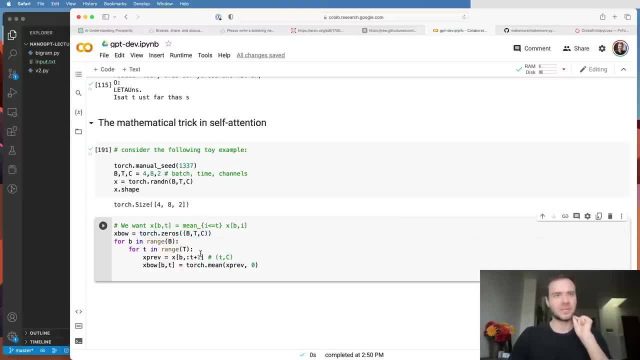 it's just initialized at zero and then I'm doing a for loop here, so we're not being efficient yet. That's coming, But for now we're just iterating over all the batch dimensions independently, Iterating over time, and then the previous tokens are at this batch dimension and then everything up to. 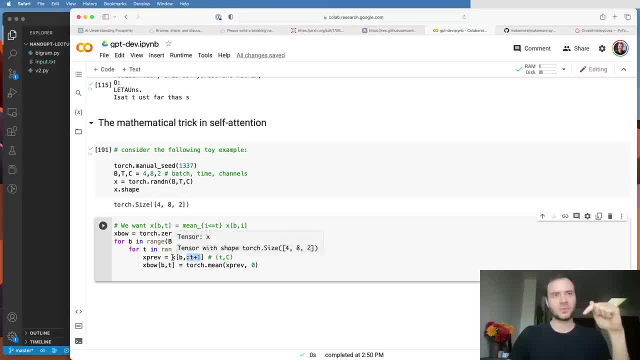 including the teeth token. So when we slice out X in this way, xprev becomes of shape. How many teeth elements there were. That's fine, the past. and then of course, C, so all the two-dimensional information from these little tokens. so that's the previous sort of chunk of tokens from my current. 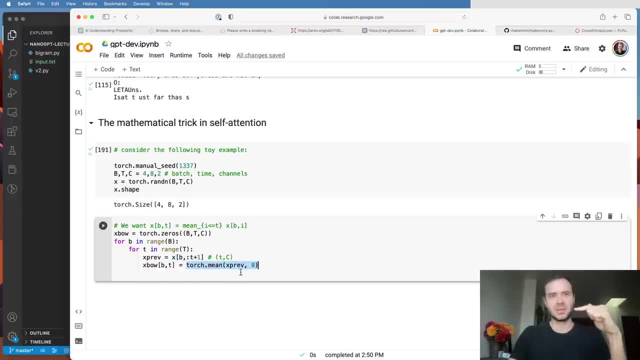 sequence and then I'm just doing the average or the mean over the 0th dimension. so I'm averaging out the time here and I'm just going to get a little C one-dimensional vector which I'm going to store in X bag of words so I can run. 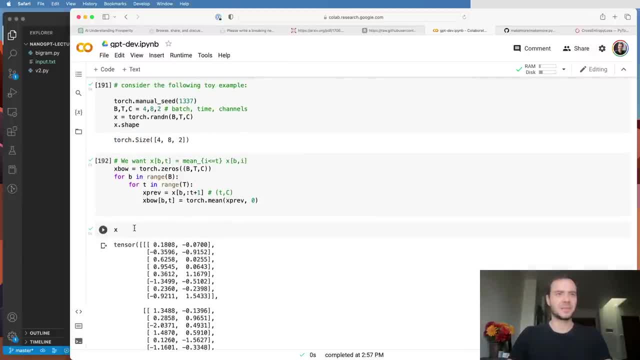 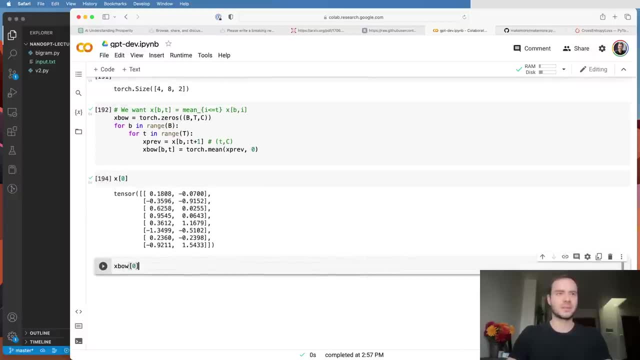 this and this is not going to be very informative because, let's see, so this is X of 0, so this is the 0th batch element, and then x bow at 0. now you see how the at the first location here you see that the two are equal, and that's because. 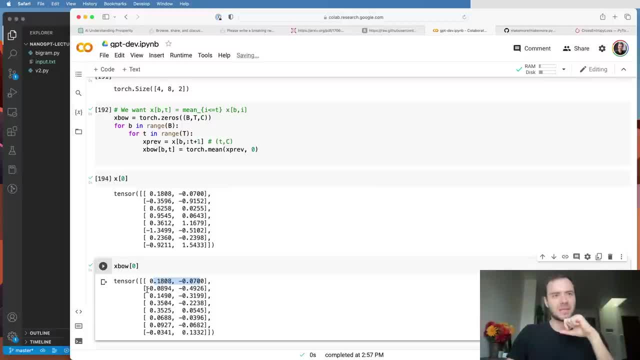 it's. we're just doing an average of this one token, but here this one is now an average of these two, and now this one is an average of to these three, okay, so on, And this last one is the average of all of these elements. So vertical. 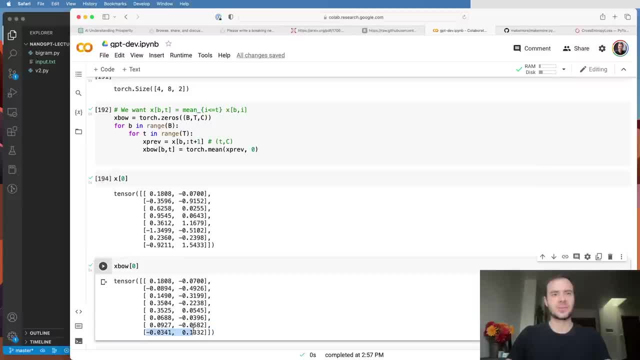 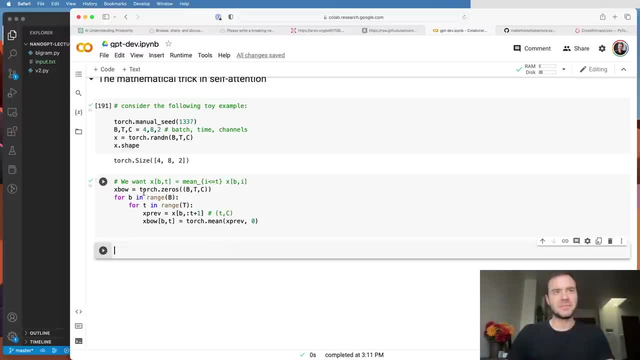 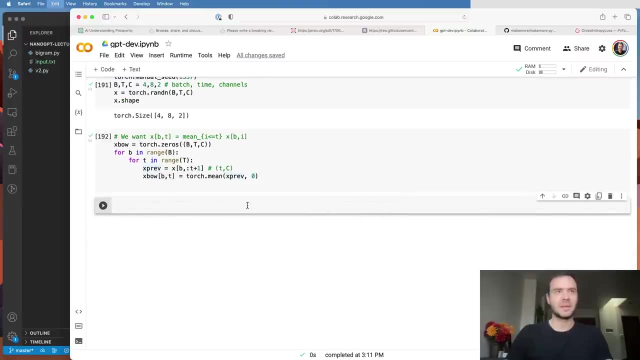 average. just averaging up all the tokens now gives this outcome here. So this is all well and good, but this is very inefficient. Now the trick is that we can be very, very efficient about doing this using matrix multiplication. So that's the mathematical trick, and let me show you what I mean. Let's work with the toy. 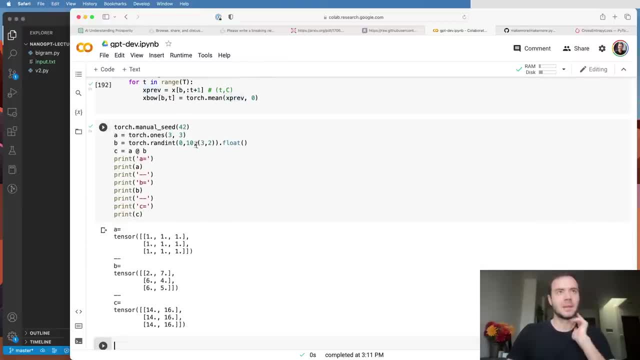 example here. Let me run it and I'll explain. I have a simple matrix here that is 3 by 3 of all the ones, a matrix B of just random numbers, and it's a 3 by 2, and a matrix C which will be 3 by 3, multiply 3 by 2, which will give out a. 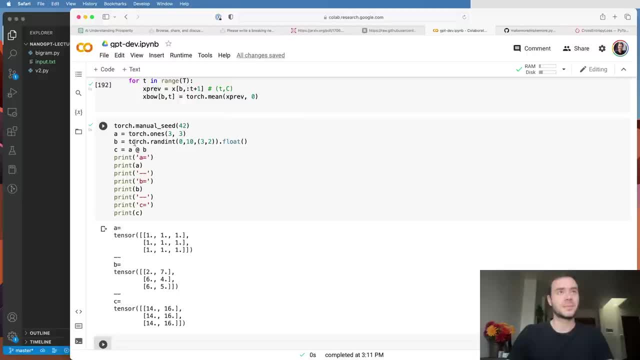 3 by 2.. So here we're just using matrix multiplication. So A multiply B gives us C. Okay, so how are these numbers in C different? Achieved right. So this number in the top left is the first row of A dot product. 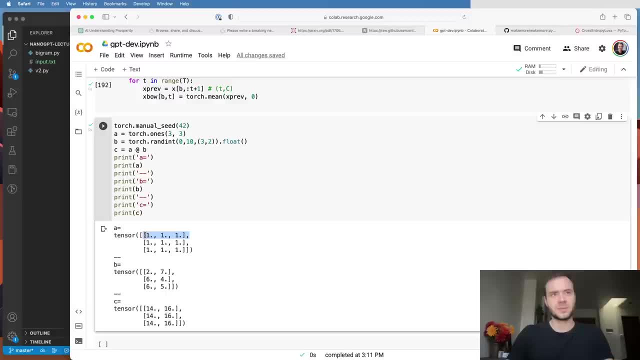 with the first column of B, And since all the row of A right now is all just ones, then the dot product here with this column of B is just going to do a sum of these of this column. So 2 plus 6 plus 6 is 14.. The element here in the 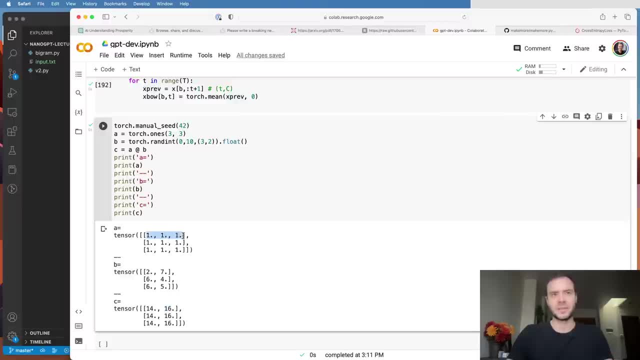 output of C is also the first column here, the first row of A multiplied now with the second column of B, So 7 plus 4 plus 5 is 16.. Now you see that there's repeating elements here. so this 14 again is because this row is again all ones and it's multiplying the. 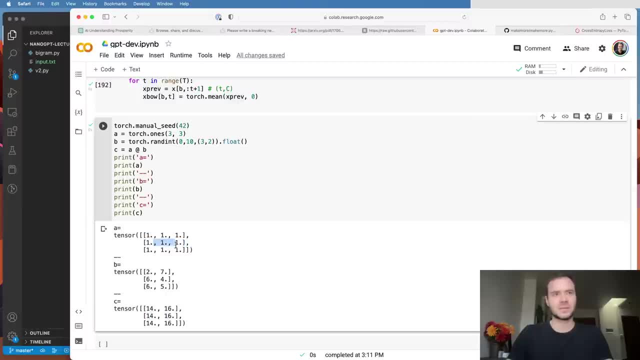 first column of B, So we get 14.. And this one is, and so on. So this last number here is the last row, dot product, last column. Now the trick here is the following: This is just a boring number of, it's just a boring array of all ones. 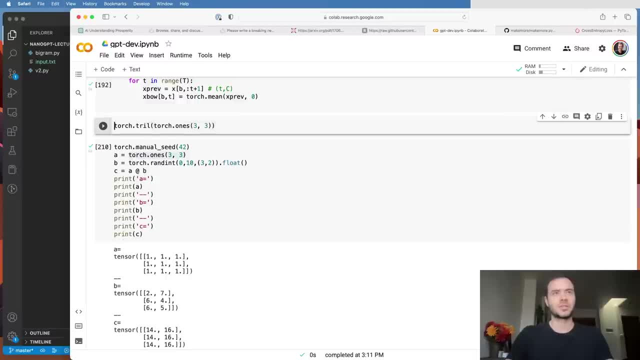 but Torch has this function called trill, Which is short for a triangular, something like that, And you can wrap it in Torch dot ones and it will just return the lower triangular portion of this. Okay, So now it will basically zero out these guys here, So we just get the lower. 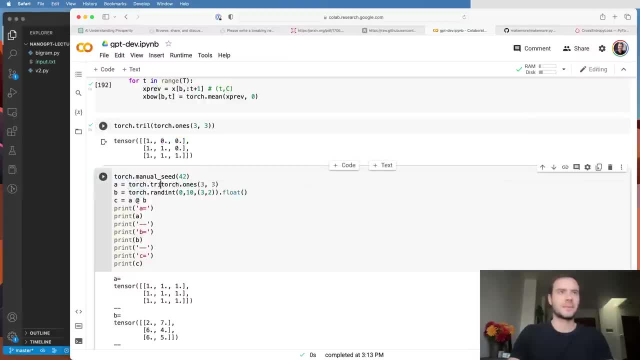 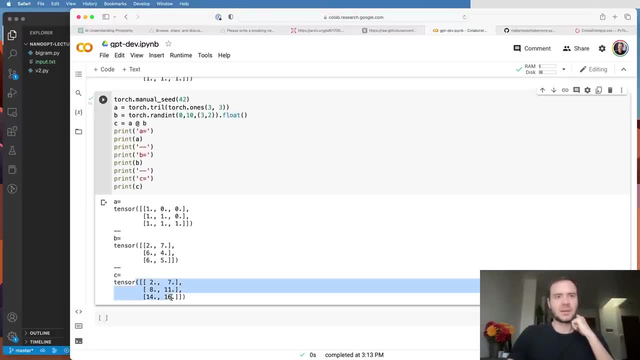 triangular part. Well, what happens if we do that? So now we'll have A like this and B like this. And now what are we getting here in C? Well, what is this number? Well, this is the first row times, the first column, And because this is, 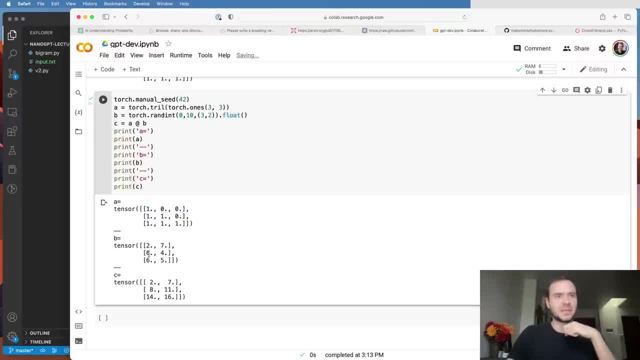 zeros. these elements here are now ignored, So we just get a 2.. And then this number- here is the first row- times the second column, And because these are zeros, they get ignored and it's just 7.. The 7 multiplies this 1.. But look what. 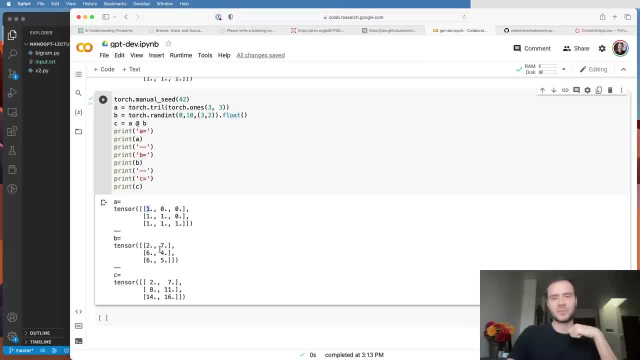 happened here, Because this is 1 and then zeros. what ended up happening is we're just plucking out this row of B and that's what we got. Now, here we have 1 1 0.. So here, 1 1 0 dot product with these two columns will now. 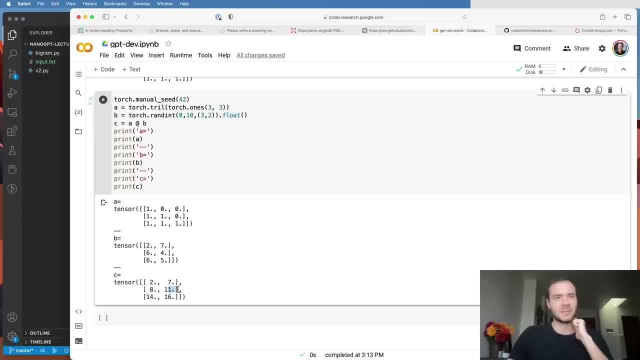 give us 2 plus 6, which is 8, and 7 plus 4, which is 11.. And because this is 1 1 1, we ended up with the addition of all of them And so basically, depending on how many ones and zeros we have here, we are basically doing a sum, currently, of the. 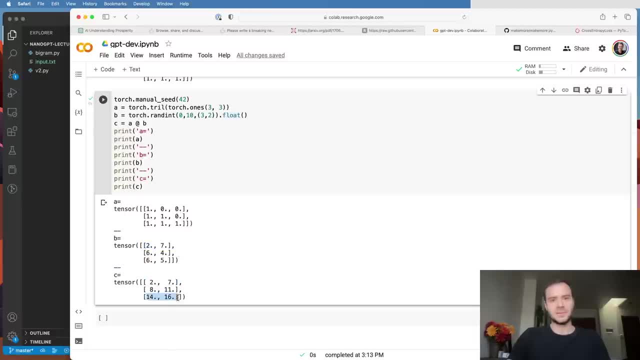 variable number of these rows and that gets deposited into C. So currently we're doing sums, because these are ones, but we can also do average, right, And you can start to see how we could do average of the rows of B, sort of in an incremental fashion, Because we don't have to, we can. 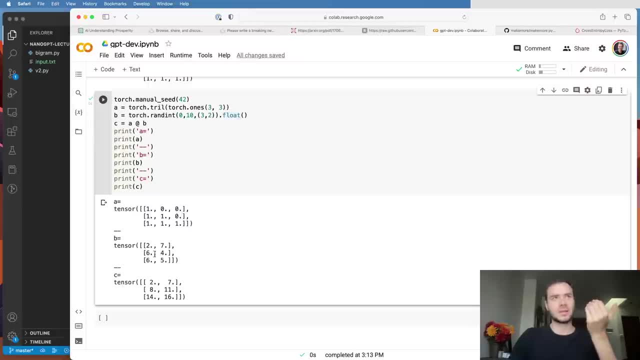 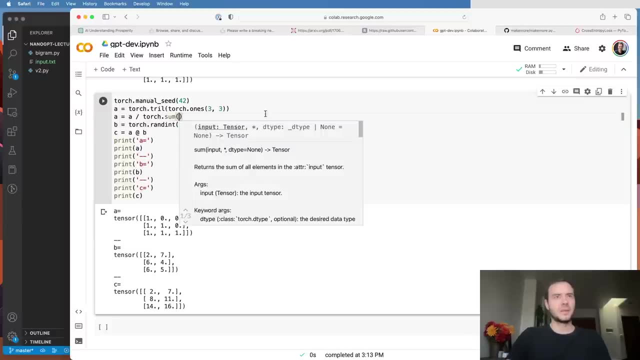 basically normalize these rows so that they sum to 1, and then we're going to get an average. So if we took a and then we did a equals A Divide torchsum of A in the one dimension, and then let's keep them as true. So therefore the broadcasting will work out. 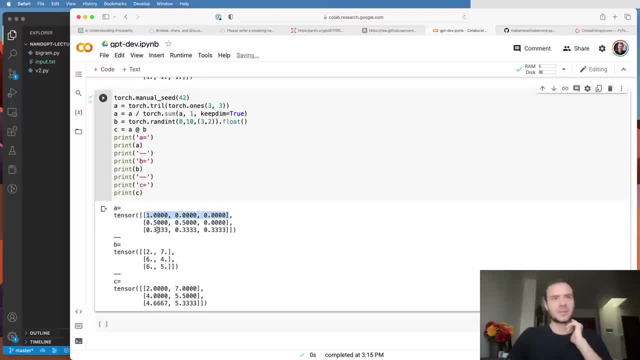 So if I rerun this, you see now that these rows now sum to one. So this row is one, this row is 0.5, 0.5, and here we get one-thirds. And now, when we do a multiply b, 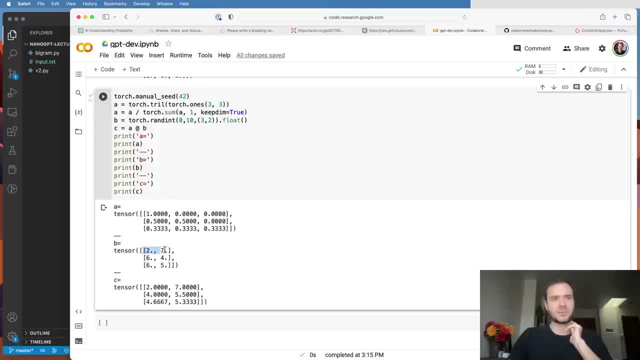 what are we getting Here? we are just getting the first row, first row Here. now we are getting the average of the first two rows. Okay, so 2 and 6 average is 4, and 4 and 7 average is 5.5.. 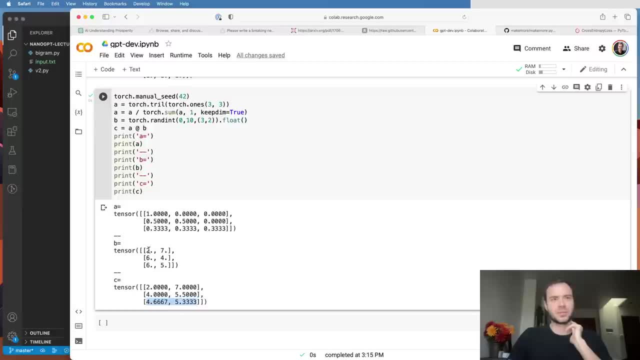 And on the bottom here we are now getting the average of these three rows. So the average of all of elements of b are now deposited here, And so you can see that by manipulating these elements of this multiplying matrix and then multiplying it with any given matrix, 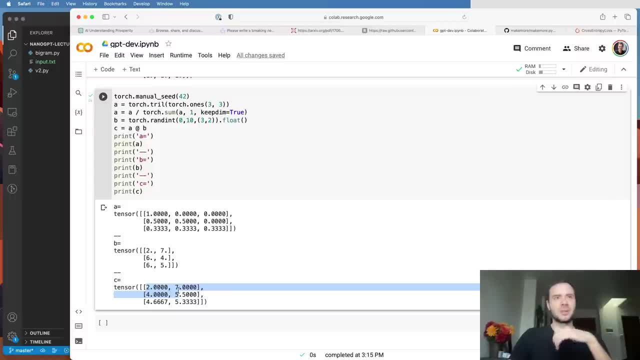 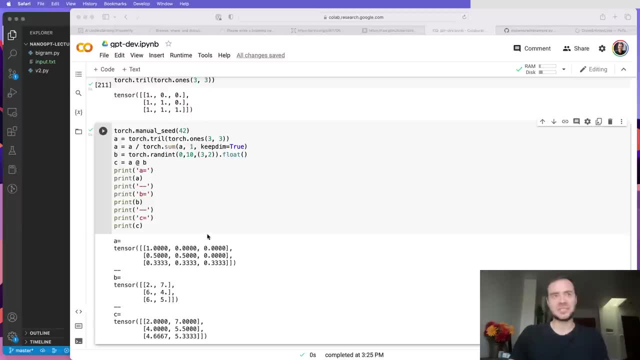 we can do these averages in this incremental fashion because we just get- and we can manipulate that based on the elements of a Okay, so that's very convenient. So let's swing back up here and see how we can vectorize this and make it much more efficient using what we've learned. 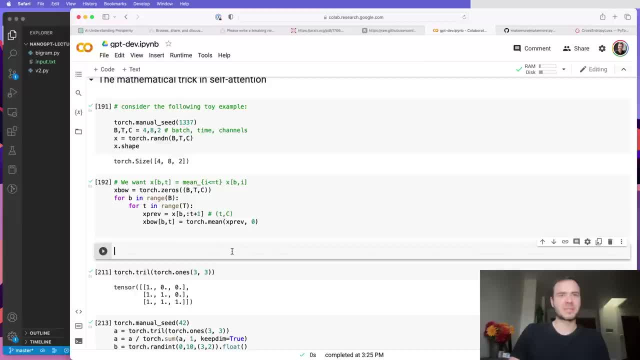 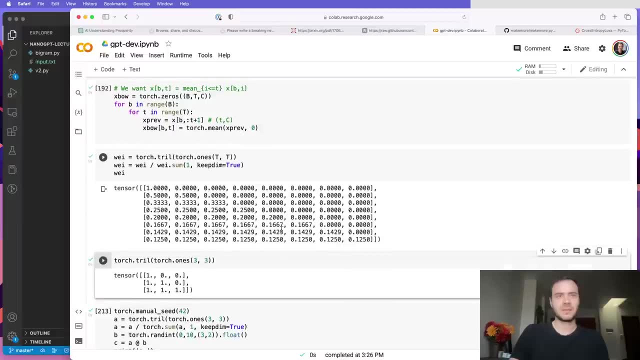 So, in particular, we are going to produce an array a- but here I'm going to call it way short- for weights. But this is our a And this is how much of every row we want to average up. And it's going to be an average because you can see that these rows sum to one. 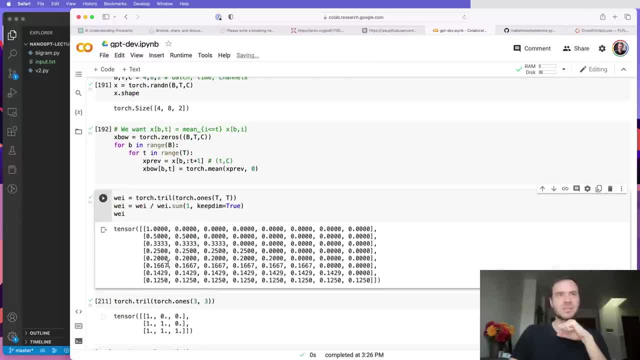 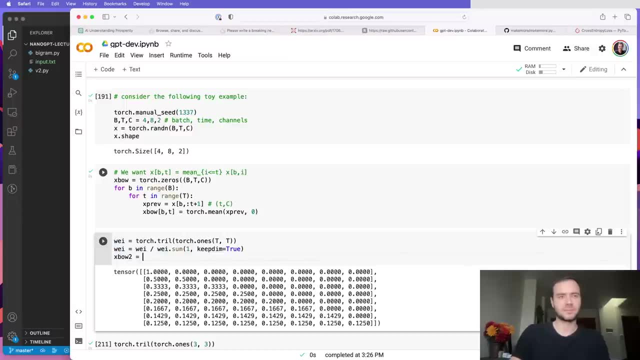 So this is our a and then our b in this example, of course, is x. So what's going to happen here now is that we are going to have an expo2.. And this expo2 is going to be way multiplying our x. 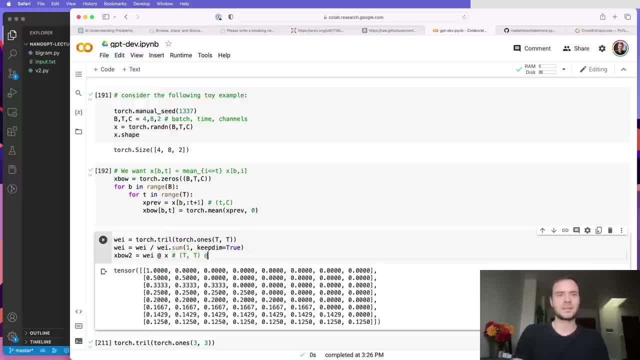 So let's think this through: Way is t by t, and this is matrix multiplying in PyTorch a, b by t by c, And it's giving us what shape. So PyTorch will come here and it will see that these shapes are not the same. 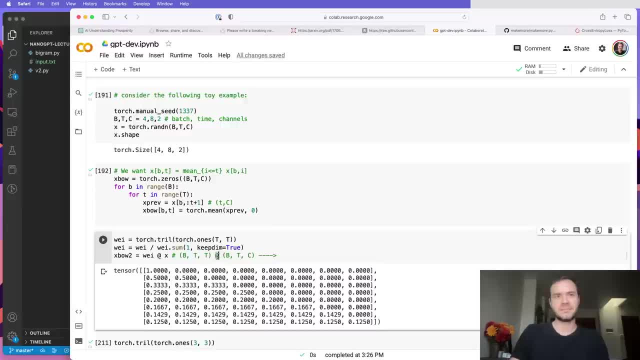 So it will create a batch dimension here, and this is a batched matrix multiply, And so it will apply this matrix multiplication in all the batch elements in parallel and individually, And then for each batch element there will be a t by t multiplying t by c. 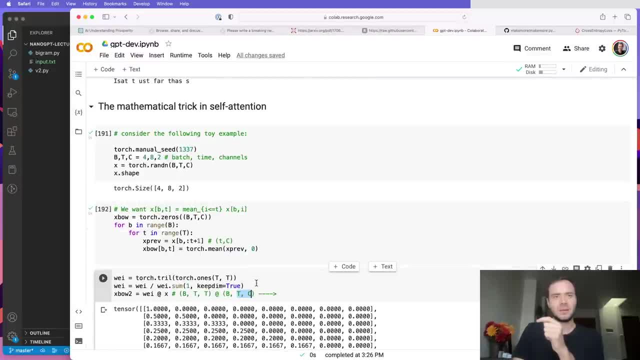 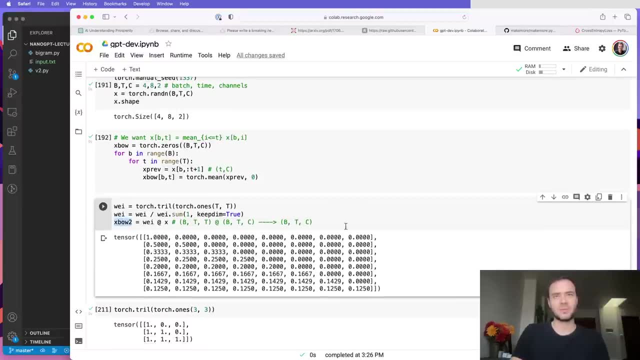 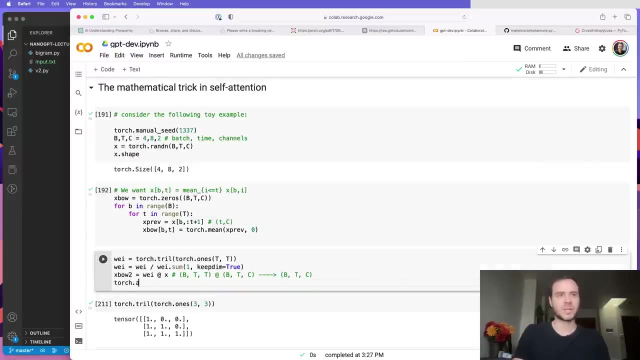 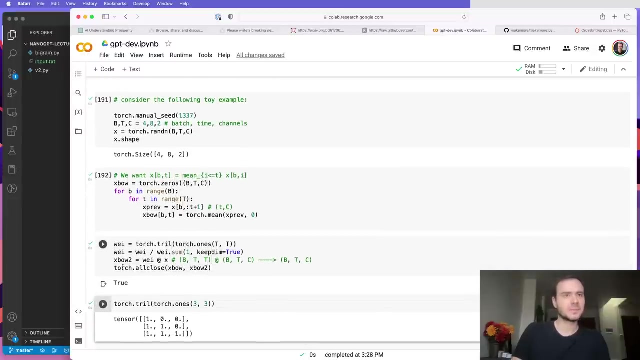 exactly as we had below. So this will now create b by t by c, And expo2 will now become identical to expo. So we can see that torchallClose of expo and expo2 should be true. So this kind of like convinces us that these are in fact the same. 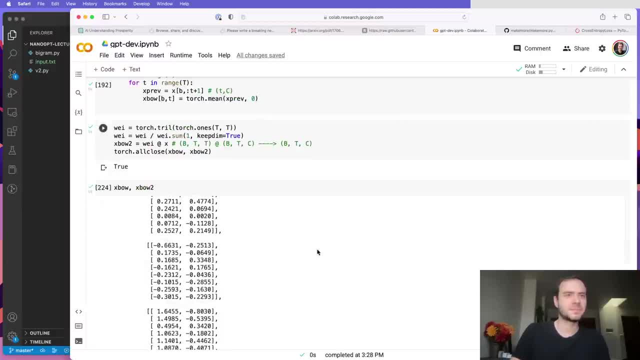 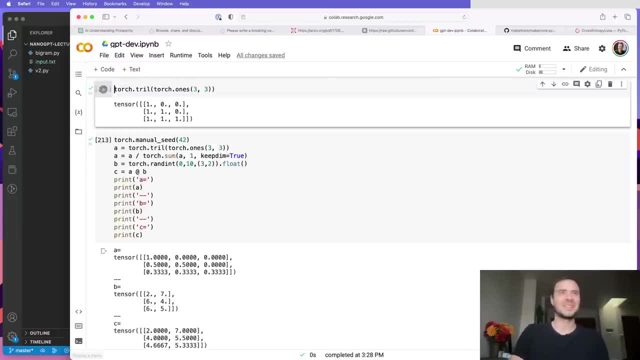 So expo and expo2, if I just print them, Okay, we're not going to be able to. Okay, We're not going to be able to just stare it down. but Well, let me try. expo basically just at the zeroth element and expo2 at the zeroth element. 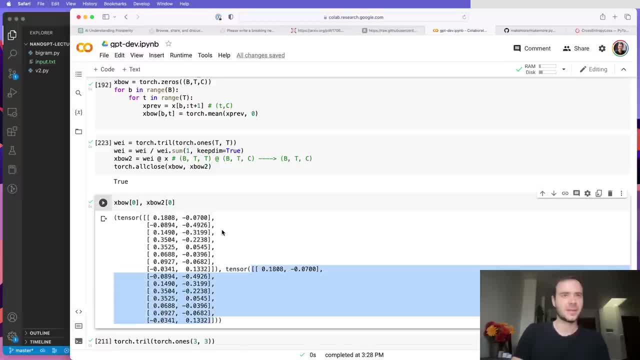 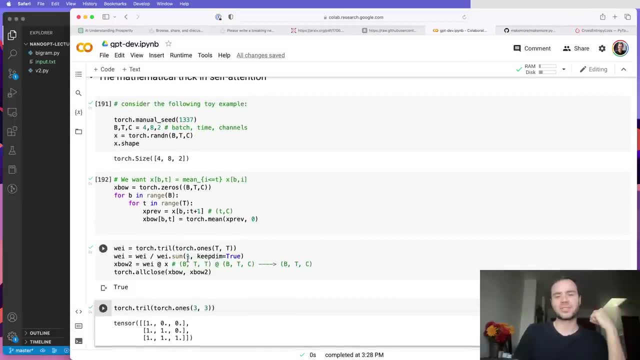 So just the first batch, and we should see that this and that should be identical, which they are Right. So what happened here? The trick is we were able to use batched matrix multiply to do this aggregation really, And it's a weighted aggregation and the weights are specified in this t by t array. 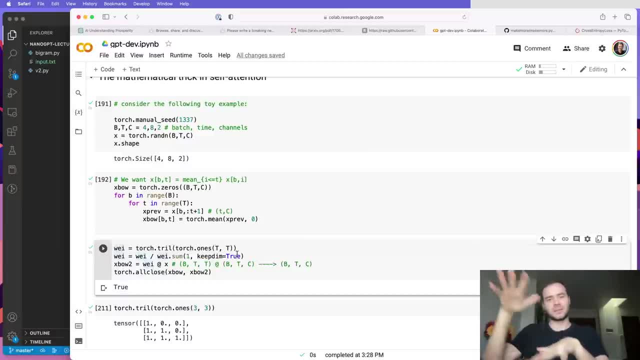 And we're basically doing weighted sums, and these weighted sums are according to the weights inside. here They take on sort of this triangular form, and so that means that a token at the t dimension will only get sort of information from the tokens preceding it. So that's exactly what we want. And finally, I would like to rewrite it in one more way, and 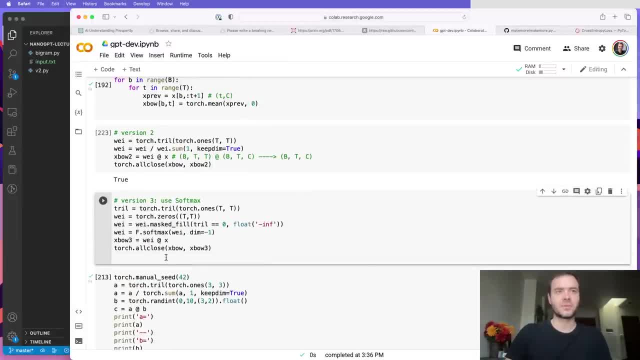 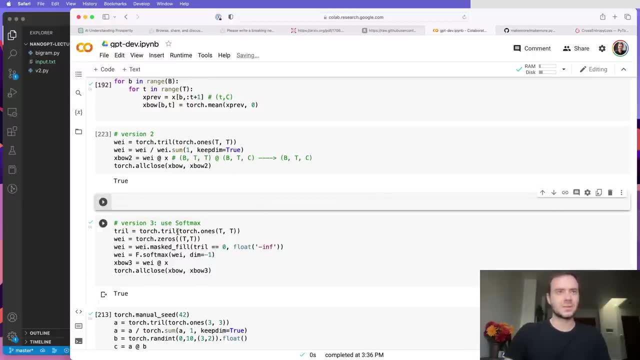 we're going to see why that's useful. So this is the third version and it's also identical. It's the first and second, But let me talk through it. It uses softmax, So trill here is this matrix: lower triangular ones. 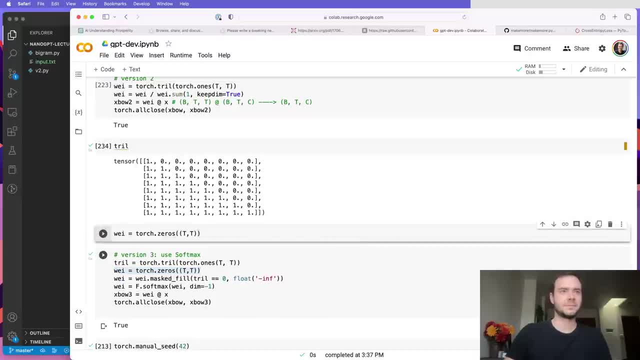 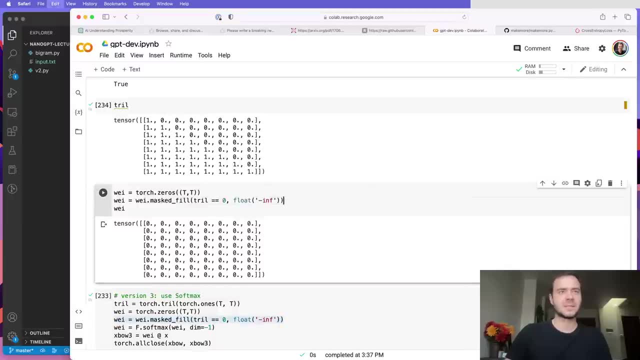 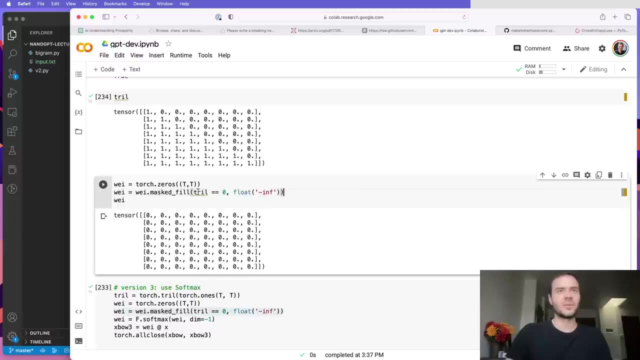 Way begins as all zero. Okay, so if I just print way in the beginning, it's all zero, Then I use masked fill. So what this is doing is waymasked fill. it's all zeros. and I'm saying for all the elements who are trilled. 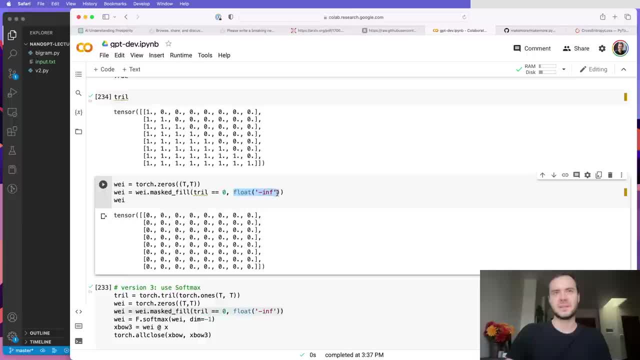 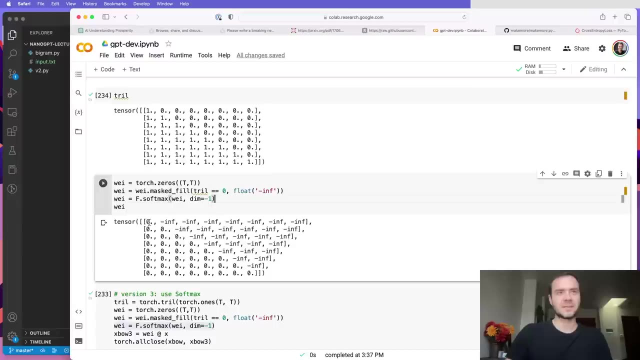 trill is equals equals zero, make them be negative infinity. So all the elements where trill is zero will become negative infinity now. So this is what we get, And then the final line here is softmax. So if I take a softmax, along every single so dim is negative one. so along every single row. 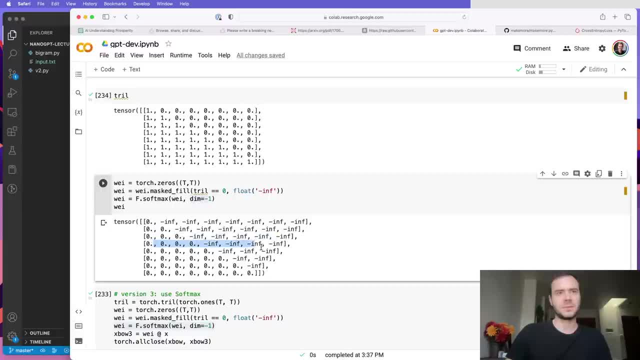 if I do a softmax, what is that going to do? Well, softmax is, is all zero, also like a normalization operation, right, and so, spoiler alert, you get the exact same matrix. Let me bring back the softmax and recall that in softmax we're 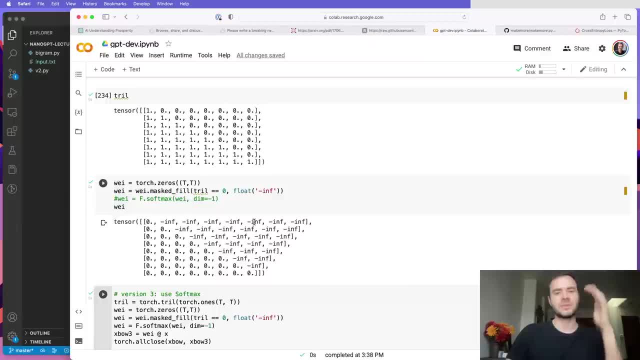 going to exponentiate every single one of these and then we're going to divide by the sum, and so if we exponentiate every single element, here we're going to get a 1, and here we're going to get basically 0 everywhere else, and then, when we normalize, we just get 1.. Here we're going to get 1,, 1, and then 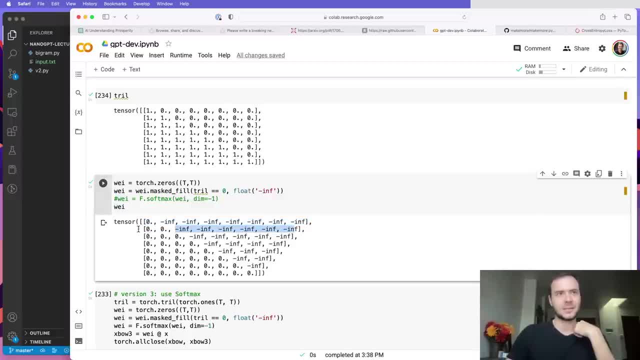 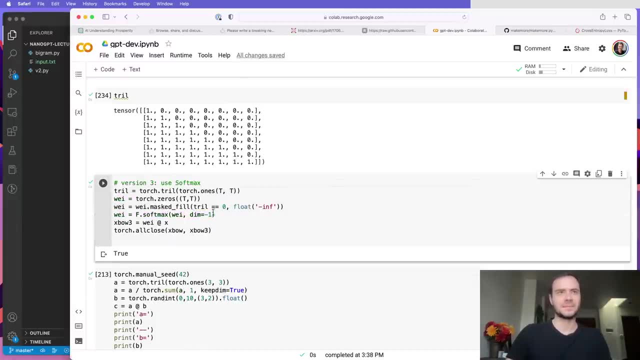 0s, and then softmax will again divide, and this will give us 0.5,, 0.5 and so on, and so this is also the same way to produce this mask. Now the reason that this is a bit more interesting and the reason we're going to end up using it in 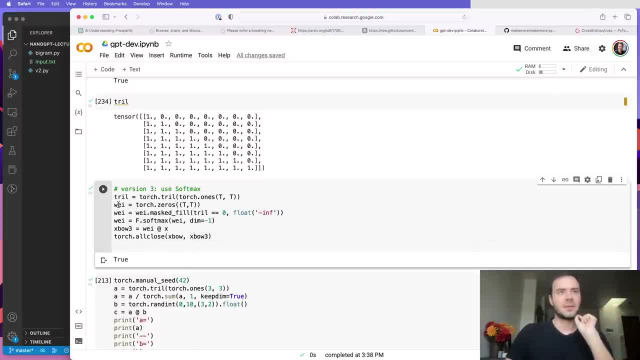 self-attention is that these weights here begin with 0 and you can think of this as like an interaction strength or like an affinity. so basically it's telling us how much of each token from the past do we want to aggregate and average up. and then this line is saying: 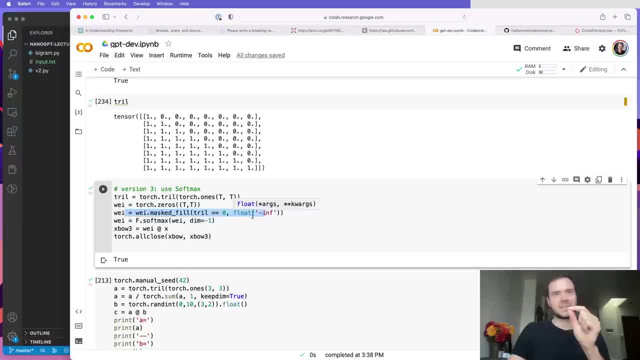 tokens from the past cannot communicate. by setting them to negative infinity, we're saying that we will not aggregate anything from those tokens, and so basically, this then goes through softmax and through the weighted, and this is the aggregation through matrix multiplication, and so what this is now is 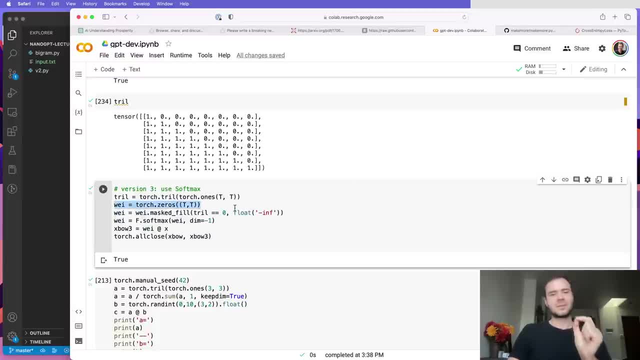 you can think of these as these zeros are currently just set by us to be zero. but a quick preview is that these affinities between the tokens are not going to be just constant at zero. they're going to be data dependent. these tokens are going to start looking at each other and some tokens will find 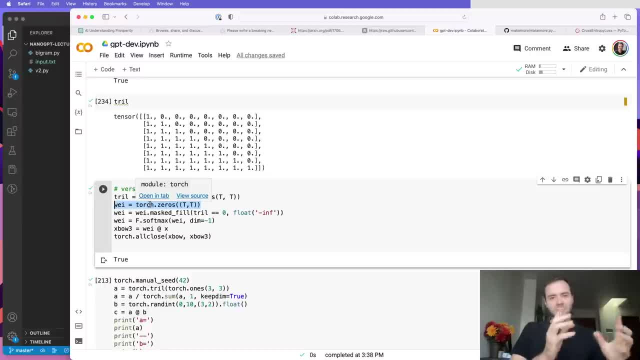 other tokens more or less interesting and depending on what their values are, they're going to find each other interesting to different amounts and I'm going to call those affinities, I think. and then here we are saying that we are saying the future cannot communicate with the past. we're going to clamp them. 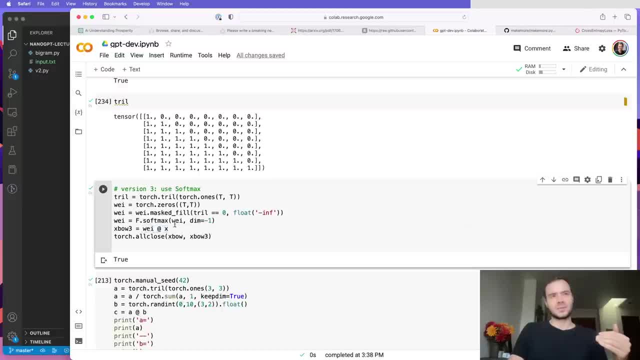 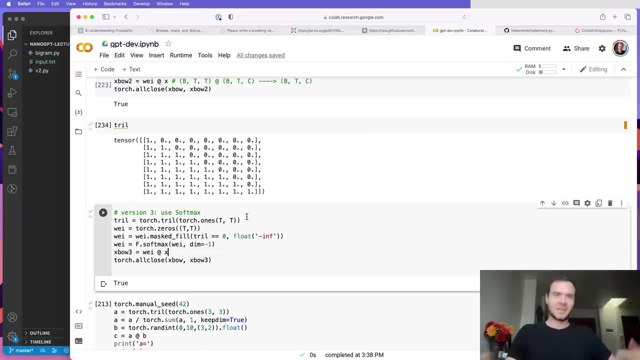 and then when we normalize and sum, we're going to aggregate sort of their values, depending on how interesting they find each other, and so that's the preview for self-attention. and basically, long story short from this entire section is that you can do weighted aggregations of your past elements by having, by using matrix. 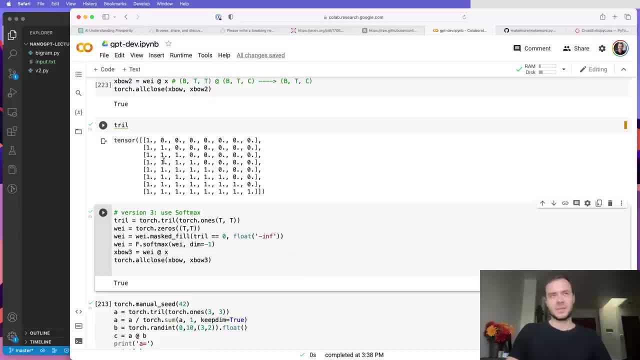 multiplication of a lower triangular fashion, and then this is going to be a little bit more complicated, but it's going to be a little bit more complicated, and then we're going to do weighted aggregations of your past elements by having, by using matrix, multiplication of a lower triangular fashion, and then this: 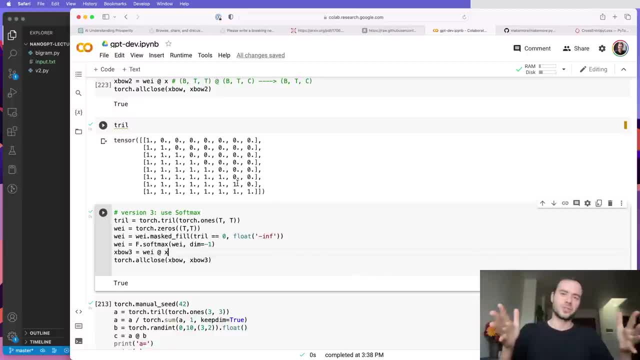 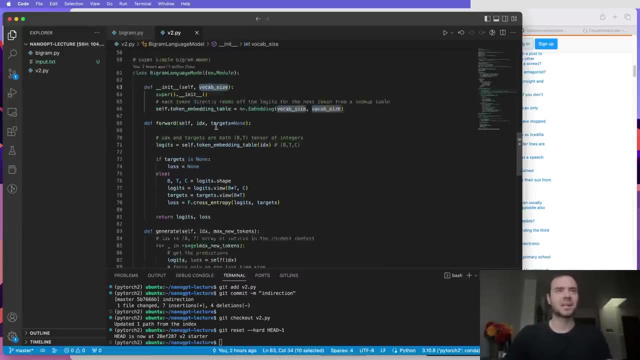 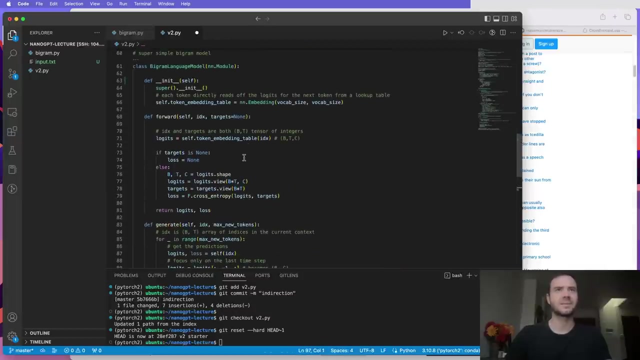 is going to be a little bit more complicated, but it's going to be a little bit more complicated than what we just saw in the initial class. so here we have it, like this sieve, it's just one that you can painting over and see. there we go, and then we're going to create it to make it designable. so two: 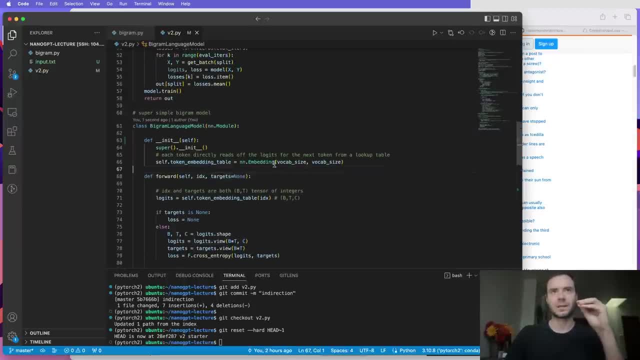 formations analog. I've defined two structures slightly differently before to create like a level of indirection here where we don't directly go to the embedding for the logits but instead we go through this intermediate phase because we're going to start making that bigger. so let me introduce a new variable and embed. it's short for number of. 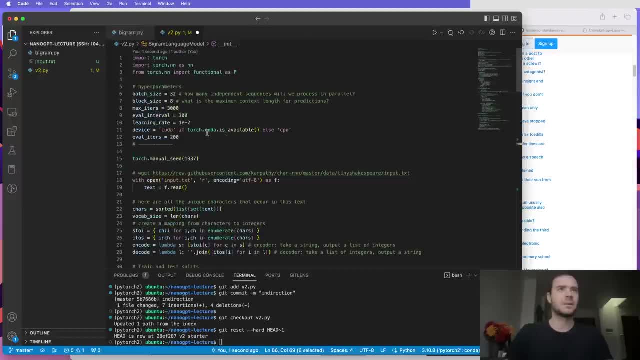 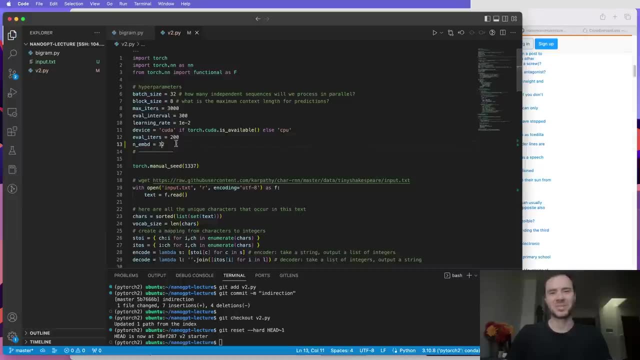 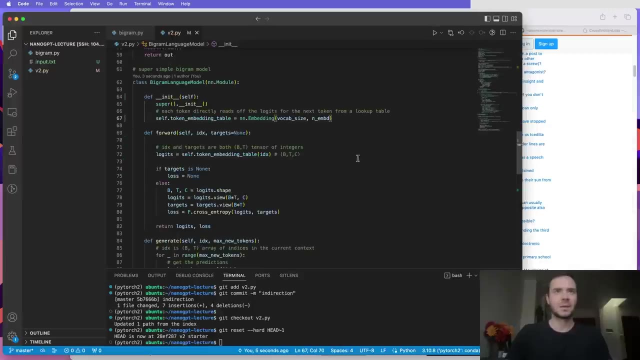 embedding dimensions. so an embed here will be, say, 32.. that was a suggestion from github co-pilot. by the way, it also shows us 32, which is a good number. so this is an embedding table and only 32 dimensional embeddings. so then here, this is not going to give us logits directly. 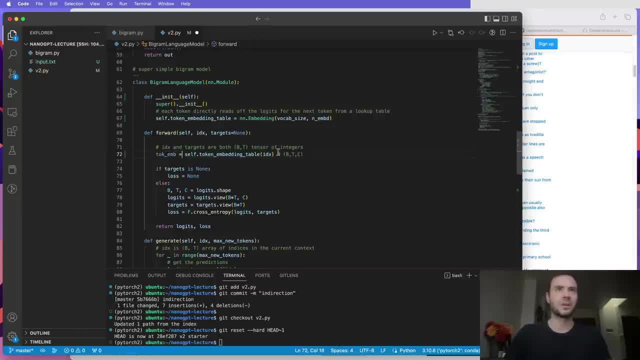 instead, this is going to give us token embeddings- that's what i'm going to call it- and then to go from the token embeddings to the logits, we're going to need a linear layer. so selflmhead- let's call it short for language modeling head- is an linear from an embed up to vocab size. 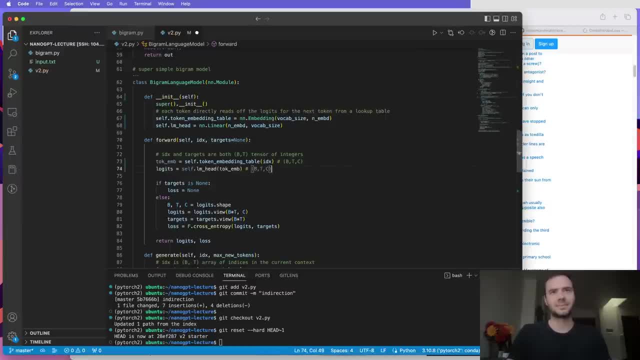 and then when we swing over here, we're actually going to get the logits by exactly what the co-pilot says. now we have to be careful here, because this c and this c are not equal. this is an embed c and this is vocab size, so let's just say that an embed is equal to c, and then this just creates. 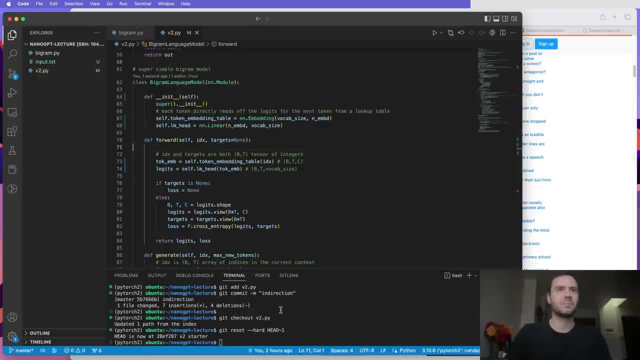 one spurious layer of indirection through a linear layer, but this should basically run on top of this. so we see that this runs and, uh, this currently looks kind of spurious, but uh, we're going to build on top of this now next up. so far, we've taken these indices and we've encoded. 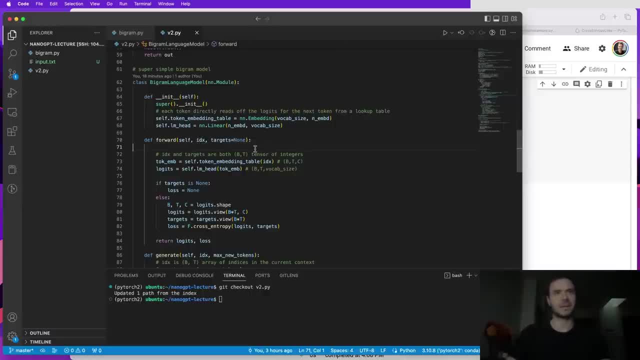 them based on the identity of the tokens inside idx. the next thing that people very often do is that we're not just encoding the identity of these tokens but also their position. so we're going to have a second position embedding table here, so solve that position embedding table. 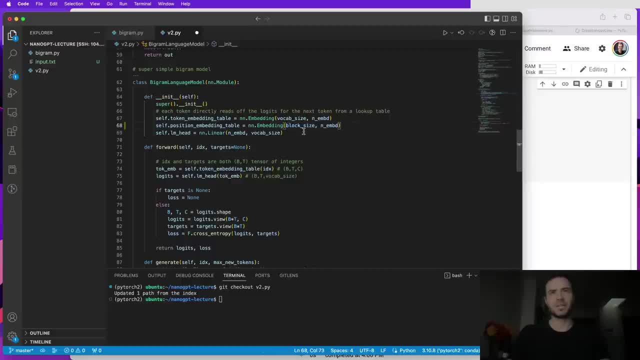 is an embedding of block size by an embed, and so each position, from zero to block size minus one will also get its own embedding vector. and then here first let me decode b by t from idxshape, and then here we're also going to have a plus embedding, which is the positional embedding. 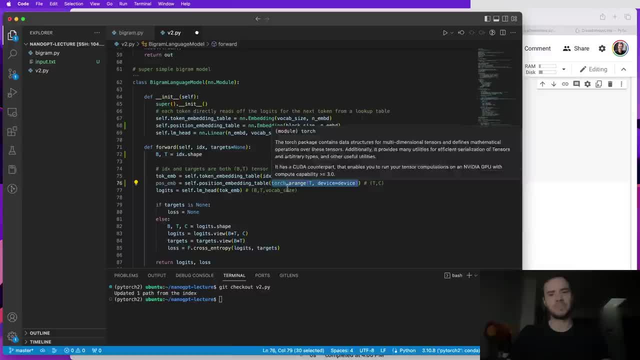 and these are. this is tordash arrange, so this will be basically just integers from zero to t minus one, and all of those integers from zero to t minus one get embedded through the table to create a positional embedding that Karen can see here, and this is the way that we're going to do that. 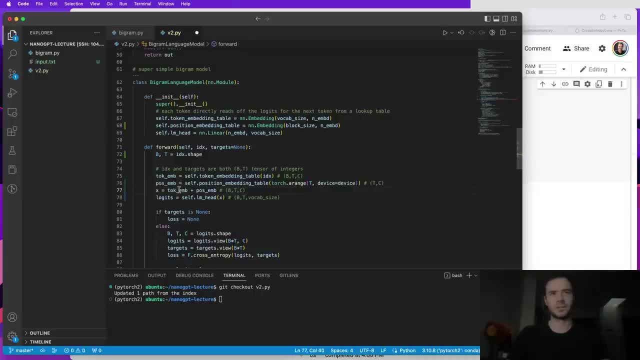 so we're going to say for the second position embedding table here, all right, we're going to go back to the original positional embedding table and we're going to name it b by c, and then here this gets renamed to just say x, and x will be the addition of the token embeddings with the. 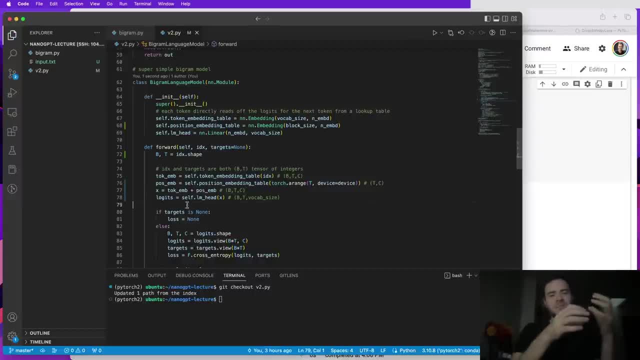 positional embeddings, and here the broadcasting note will work out. so b by t by c plus t by c occur. And this is currently not that useful because of course we just have a simple bigram model. so it doesn't matter if you're in the fifth position. the second position: 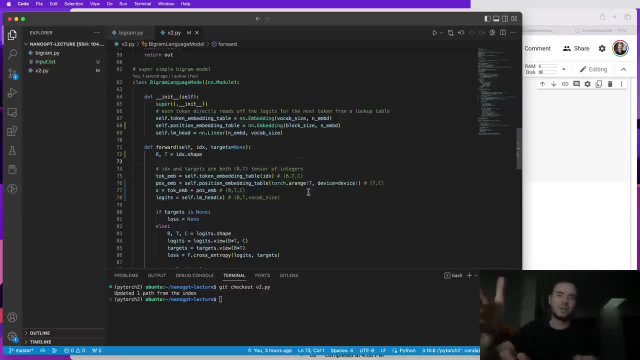 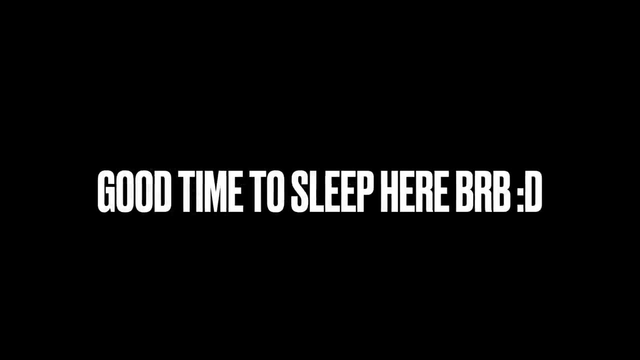 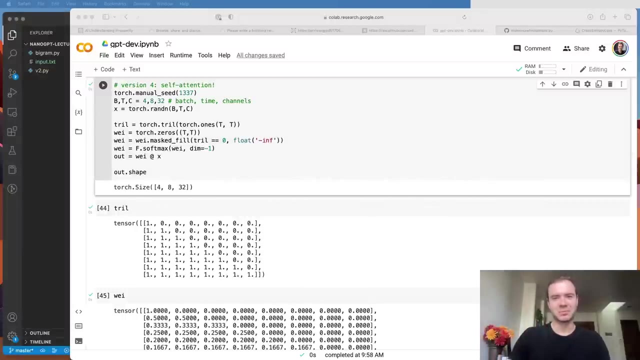 or wherever. It's all translation invariant at this stage, so this information currently wouldn't help, But as we work on the self-attention block, we'll see that this starts to matter. Okay, so now we get the crux of self-attention, So this is probably the most important part of 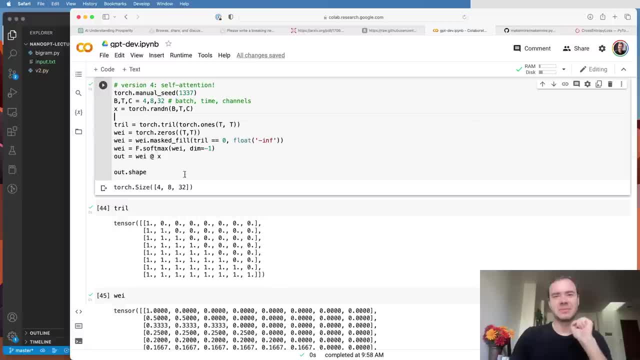 this video to understand. We're going to implement a small self-attention for a single individual head, as they're called, So we start off with where we were. so all of this code is familiar. So right now I'm working with an example where I change the number of channels from 2 to 32,. 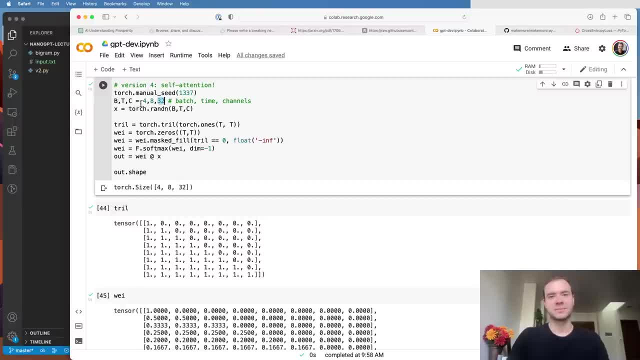 so we have a 4 by 8 arrangement of tokens and the information at each token is currently 32-dimensional, but we just are working with random numbers. Now we saw here that the code, as we had it before, does a simple weight, a simple average of all the past tokens. 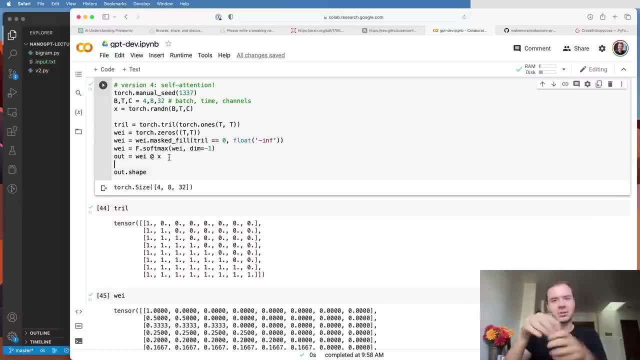 and the current token, So it's just the previous information, and the current information is just being mixed together in an average, and that's what this code currently achieves, And it does so by creating this lower triangular structure which allows us to mask out this weight matrix. 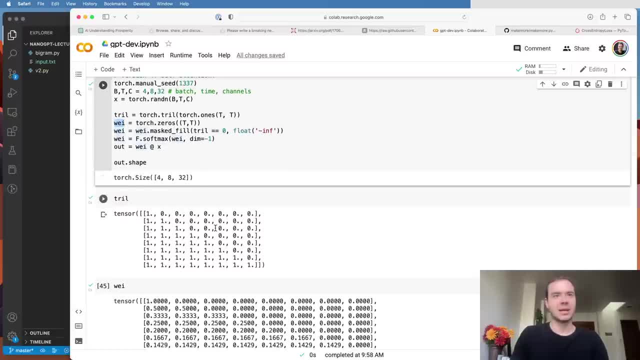 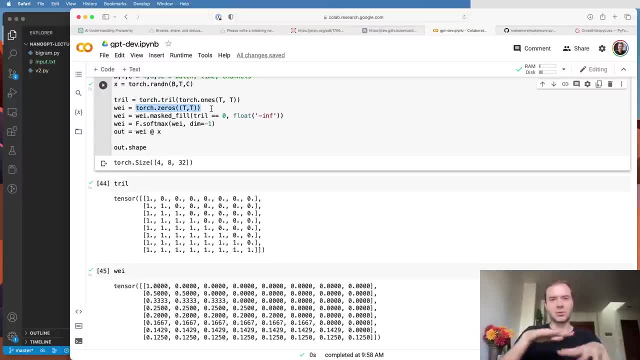 that we create, So we mask it out and then we normalize it. and currently, when we initialize affinities between all the different sort of tokens or nodes- i'm going to use those terms interchangeably- so when we initialize the affinities between all the different tokens to be, 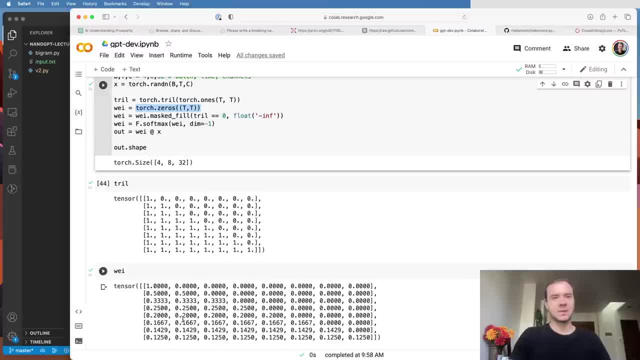 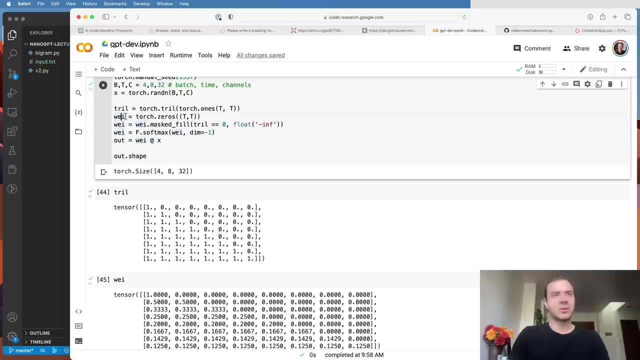 zero, then we see that way, gives us this structure where every single row has these uniform numbers, and so that's what. that's what then in this matrix, multiply makes it so that we're doing a simple average. now we don't actually want this to be all uniform, because different. 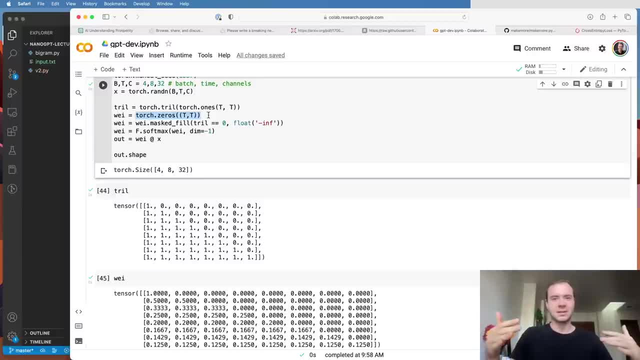 tokens will find different other tokens more or less interesting, and we want that to be data dependent. so, for example, if i'm a vowel, then maybe i'm looking for consonants in my past and maybe i want to know what those consonants are, and i want that information to flow to me, and so i want to. 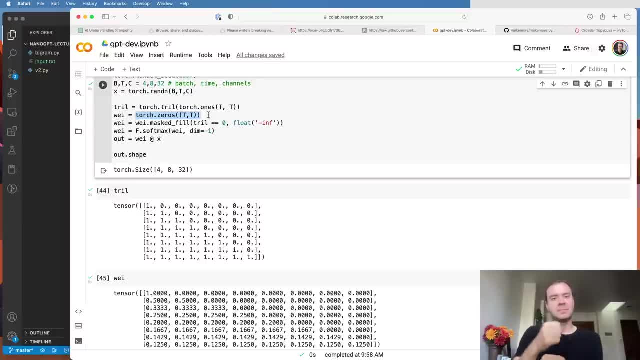 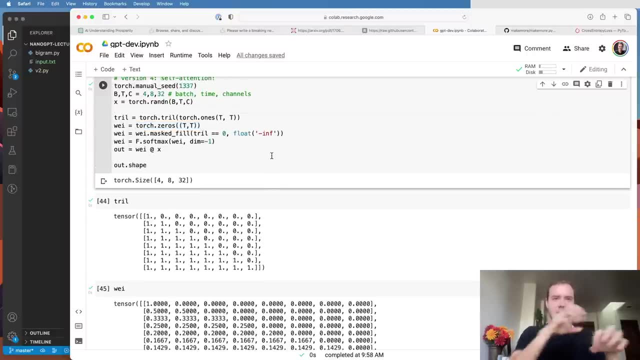 now gather information from the past, but i want to do it in a data dependent way, and this is the problem that self-attention solves now. the way self-attention solves this is the following: every single node or every single token at each position will emit two vectors. it will emit a. 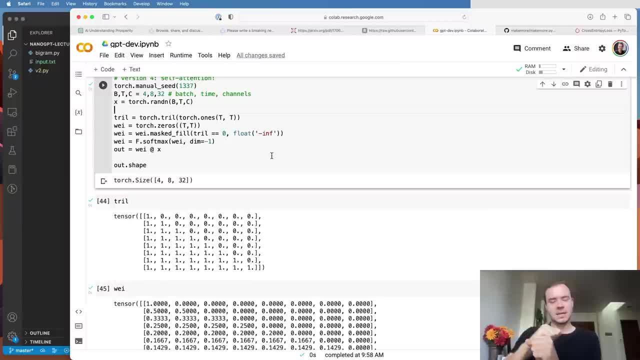 query and it will emit a key. now the query vector, roughly speaking, is: what am i looking for? and the key vector, roughly speaking, is: what do i contain? and then the way we get affinities between these tokens now in a sequence is we basically just do a dot product between the keys and the queries. 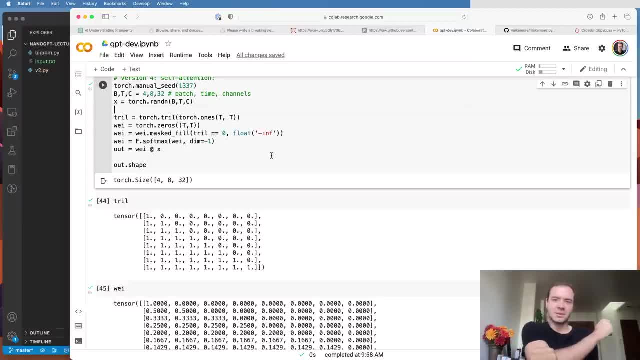 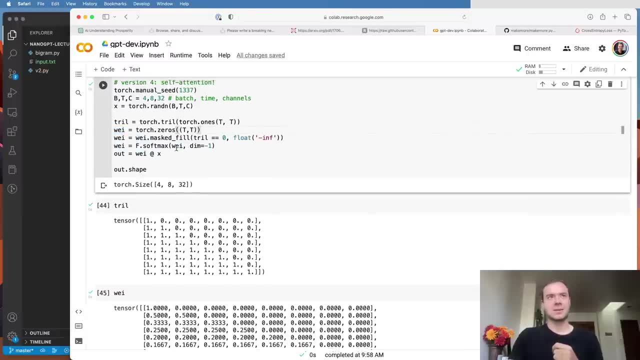 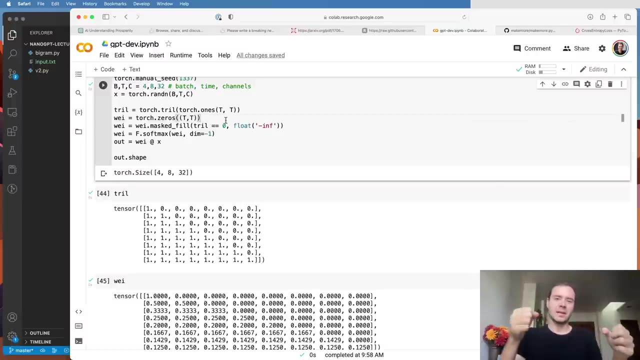 so my query dot products with all the keys of all the other tokens and that dot product now becomes way, and so if the key and the query are sort of aligned, they will interact to a very high amount and then i will get to learn more about that specific token as opposed to any other token in. 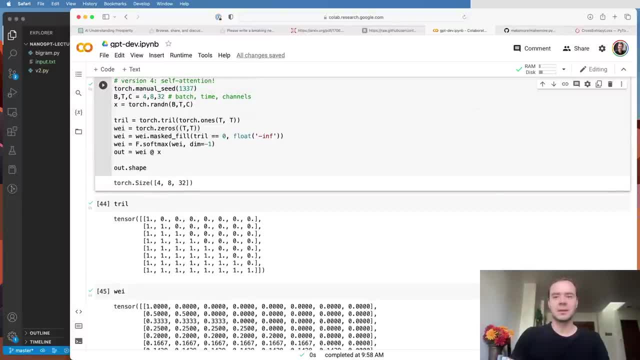 the sequence. so let's implement this, then we're going to do a key dot product now. if we do this, implement this now We're going to implement a single what's called head of self-attention. So this is just one head. There's a hyperparameter involved with 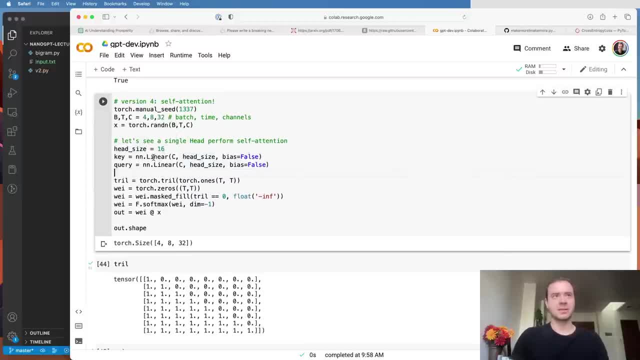 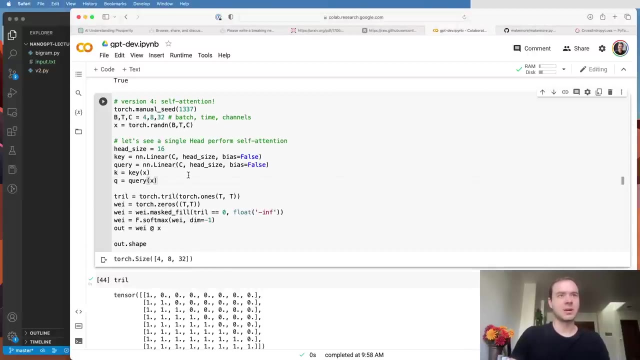 these heads, which is the head size. and then here I'm initializing linear modules and I'm using bias. equals false. so these are just going to apply a matrix, multiply with some fixed weights. and now let me produce a key and Q, K and Q by forwarding these modules on X, So the size of this will now become B by T. 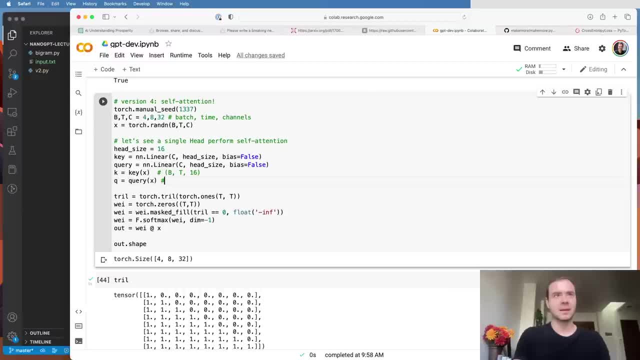 by 16, because that is the head size. and the same here: B by T, by 16.. So, this being the head size. So you see here that when I forward this line, it's going to be the head size. So you see here that when I forward this, 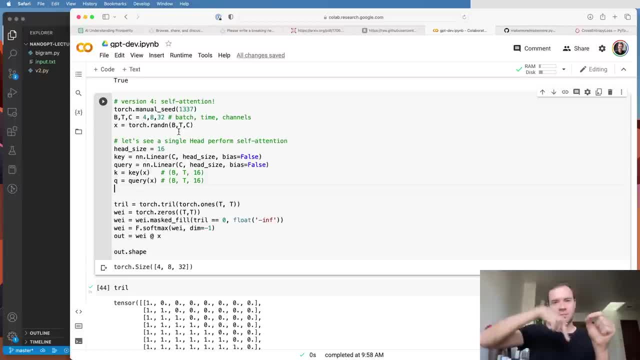 line, it's going to be the head size. So you see here that when I forward this linear on top of my X, all the tokens in all the positions in the B by T arrangement, all of them in parallel and independently produce a key and a query. 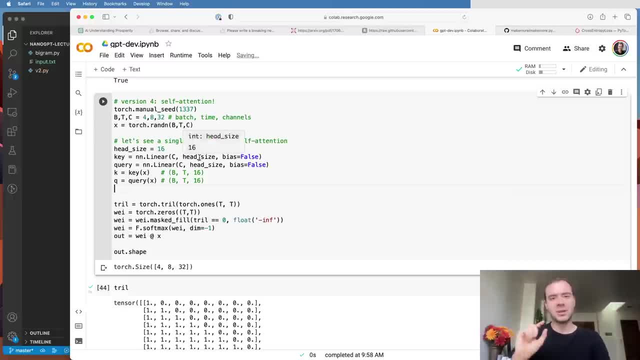 so no communication has happened yet. but the communication comes now. all the queries will dot product with all the keys. So basically what we want is we want way now, or the affinities between these, to be query multiplying key. but we have to be careful with, we can't matrix multiply this. we actually 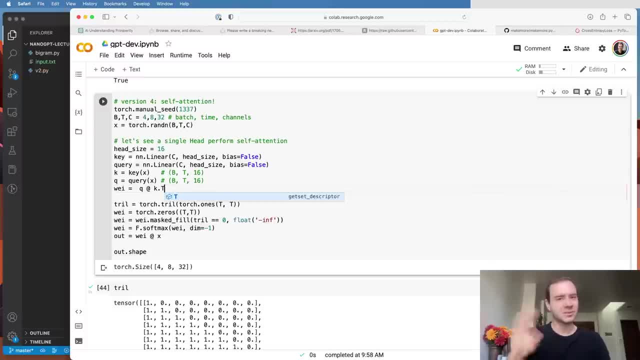 need to transpose K, but we have to be also careful because these are when you have the batch dimension. so in particular, we want to transpose the last two dimensions, dimension negative 1 and dimension negative 2. so negative 2, negative 1, and so this matrix multiply now will basically do the following: B by 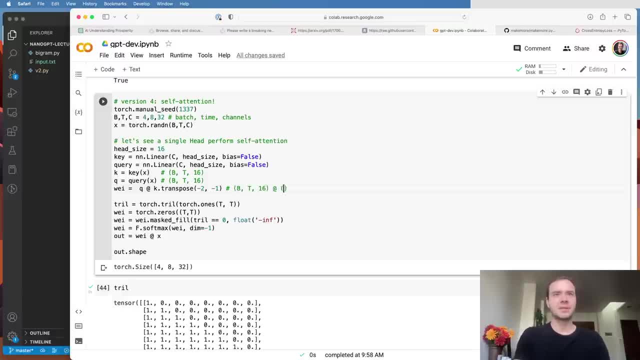 T by 16 matrix multiplies B by 16 by T to give us B by T by T, right? so for every row of B we're now going to have a T square matrix giving us the affinities and these are now the way. so they're not. 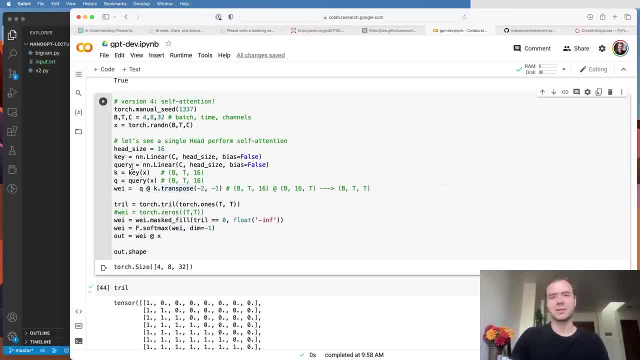 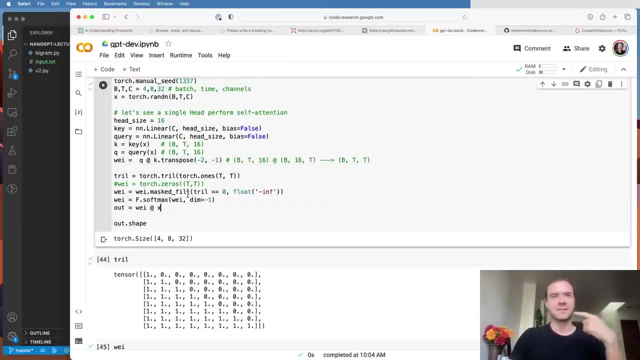 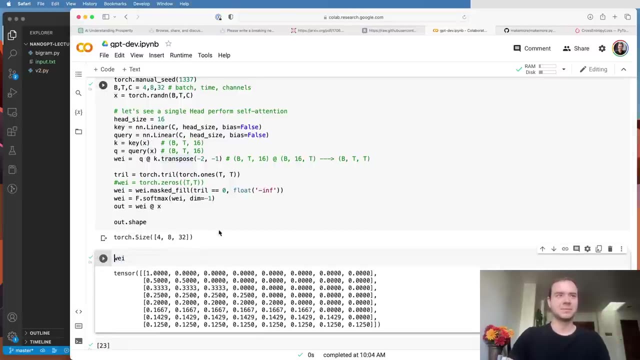 zeros. they are now coming from this dot product between the keys and the queries, so this can now run. I can, I can run this and the weighted aggregation now is a function in a data-dependent manner between the keys and queries of these nodes. so just inspecting what happened here, the way takes on this form and you. 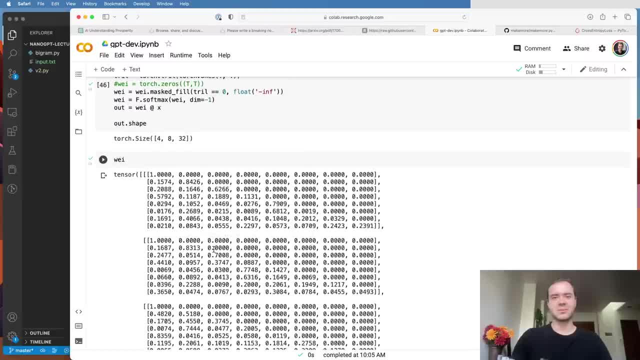 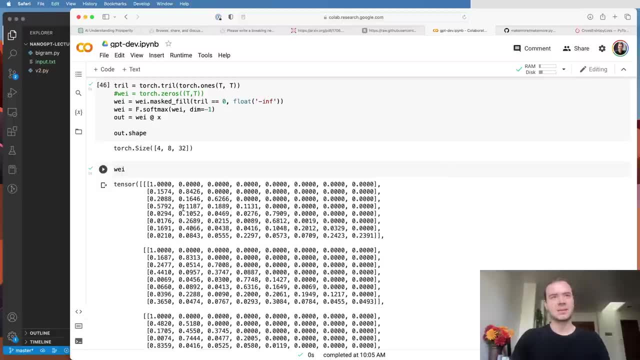 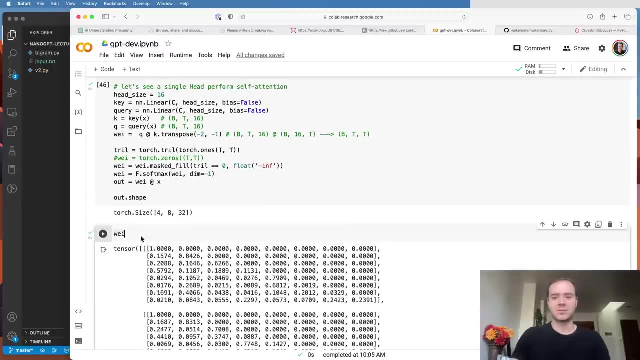 see that before way was just a constant, so it was applied in the same way to all the batch elements. but now every single batch elements will have different sort of way, because every single batch element contains different tokens at different positions and so this is not data dependent. so when we look at just 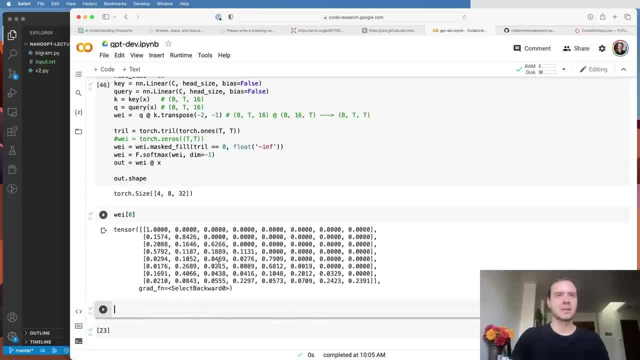 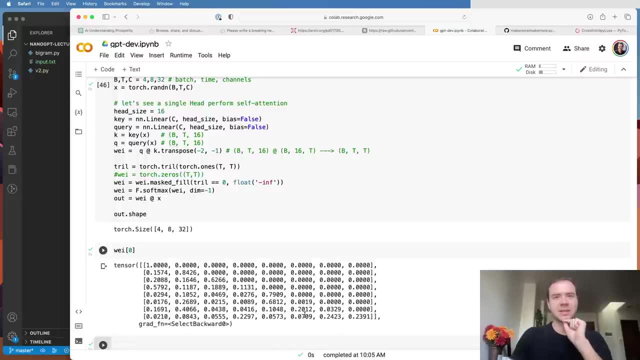 the 0th row. for example, in the input, these are the weights that came out, and so you can see now that they're not just exactly uniform. and in particular, as an example here, for the last row, this was the 8th token, and the 8th token knows what content it has and it knows at what. 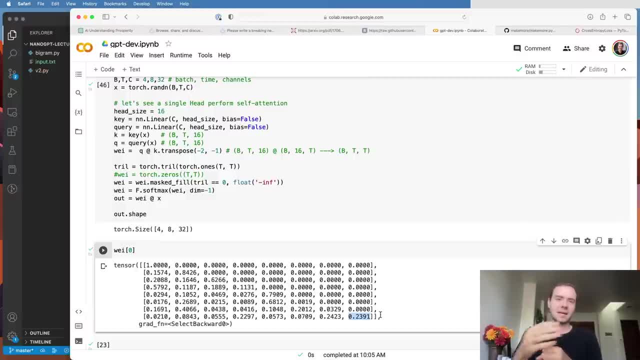 position it's in and now the 8th token based on that creates a query. hey, I'm looking for this kind of stuff. I'm a vowel, I'm on the 8th position, I'm looking for any consonants at positions up to 4 and then all the nodes get to emit keys and 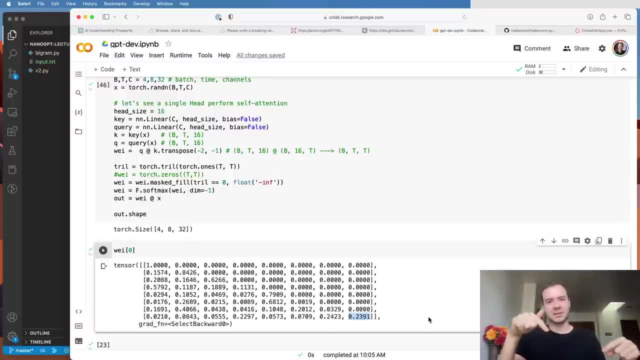 maybe one of the channels could be. I am a consonant and I am in the position up to 4 and that key would have a high number in that specific channel and that's how the query and the key when they dot product, they can find each. 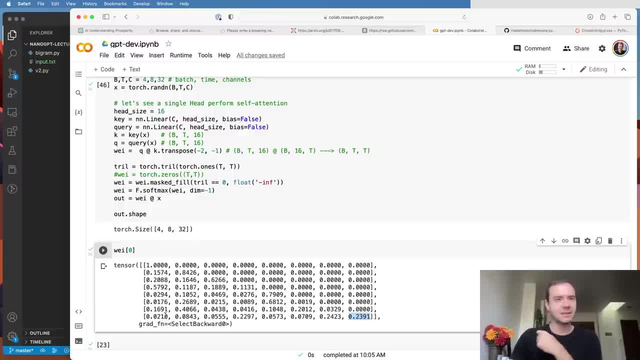 other and create a high affinity, and when they have a high affinity- like, say, this token was pretty interesting to to this 8th token, when they have a high affinity, then through the softmax I will end up aggregating a lot of its information into my position. 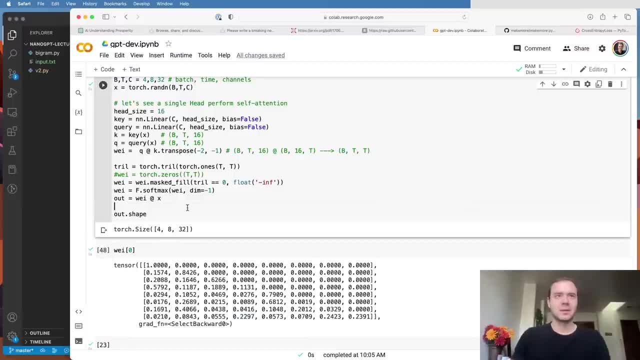 and so I'll get to learn a lot about it now. just this we're looking at way after this has already happened, let me erase this operation as well. so let me erase the masking and the softmax, just to show you the under the hood, internals and how. 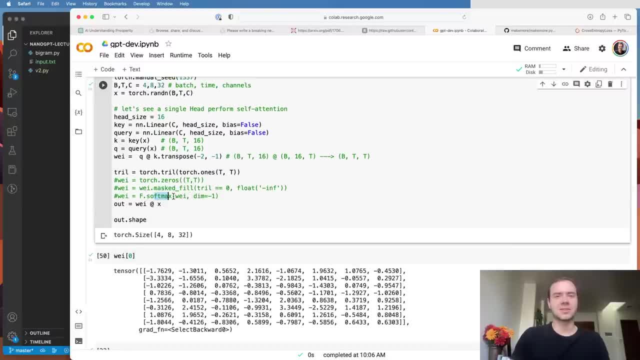 that works. so, without the masking and the softmax way comes out like this: right, this is the outputs of the dot products and these are the raw outputs, and they take on values from negative, you know, 2, to positive, 2, etc. so that's the raw interactions and raw affinities between all the nodes. but now 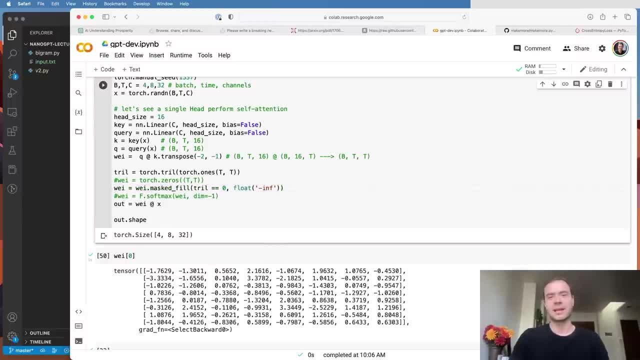 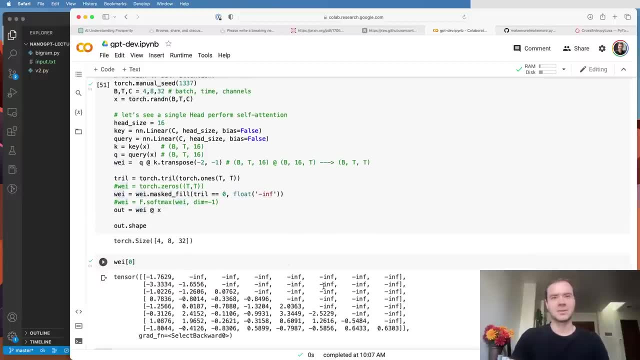 if I'm a, if I'm a fifth node, I will not want to aggregate anything from the 6th node, 7th node and the 8th node. so actually we use the upper triangular masking. so those are not allowed to communicate. and now we actually want to. 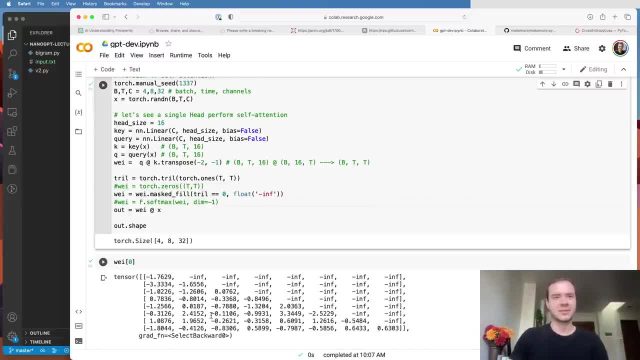 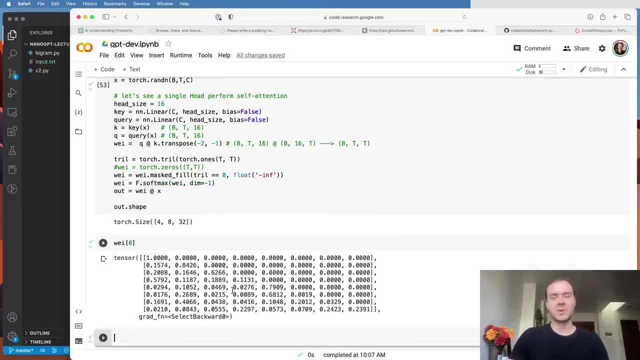 have a nice distribution. so we don't want to aggregate negative 0.11 of this node. that's crazy. so instead we exponentiate and normalize, and that's what we're going to do. next we're going to do is we're going to duplicate these nodes and we're going to add a value that's equal to negative. 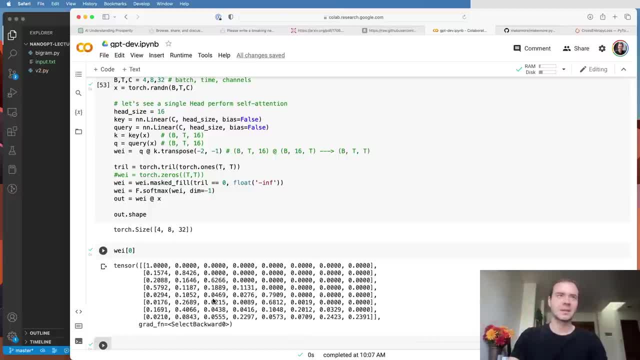 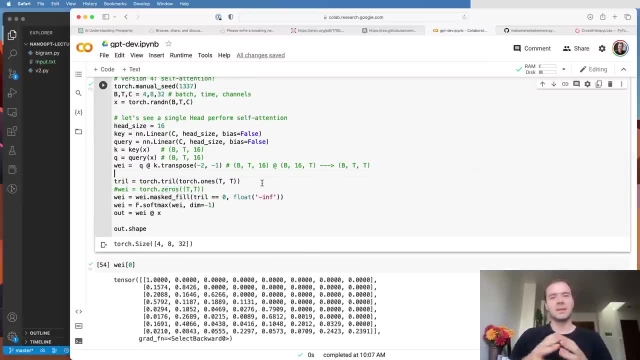 1, and now we get a nice distribution that comes to 1, and this is telling us now, in the data-dependent matter, how much of information to aggregate from any of these tokens. in the past. so that's way, and it's not zeros anymore, but it's calculated in this way. now there's one more part to a single. 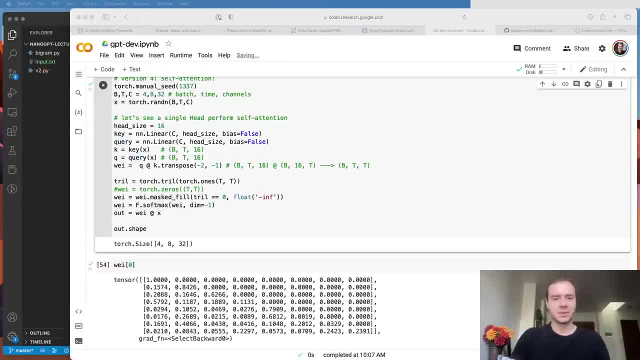 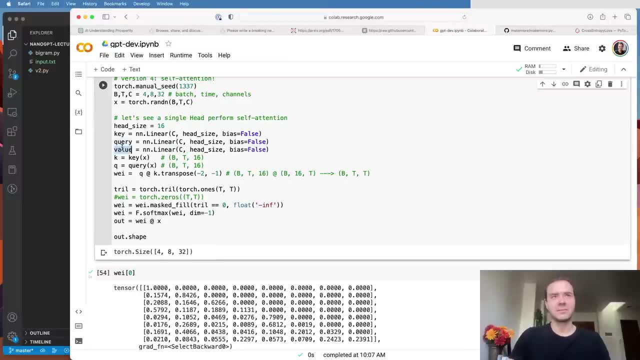 self-attention head, and that is that when we do the aggregation, we don't actually the value. so in the same way that we produced p and query, we're also going to create a value. and then here we don't aggregate x, we calculate a v, which is just achieved by propagating this. 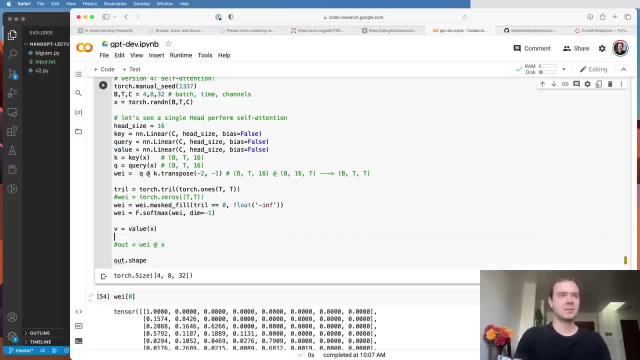 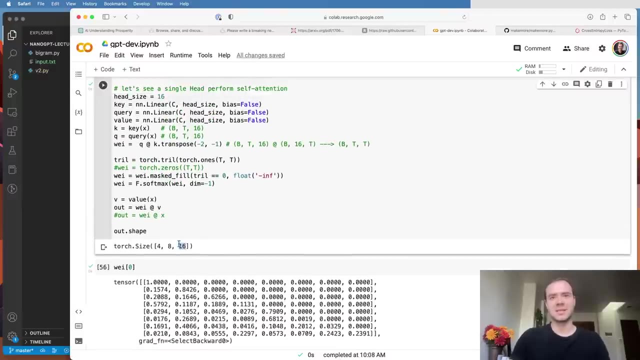 linear on top of x again, and then we output way multiplied by v. so v is the elements that we aggregate, or the vector that we aggregate, instead of the raw x. and now, of course, this will make it so that the output here of the single head will be 16 dimensional, because that is the 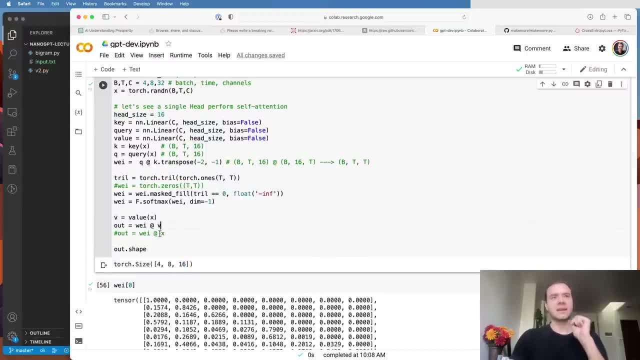 head size. so you can think of x as kind of like private information to this token if you, if you think about it that way. so x is kind of private to this token. so i'm a fifth token at some and i have some identity and my information is kept in vector x. and now, for the purposes of the 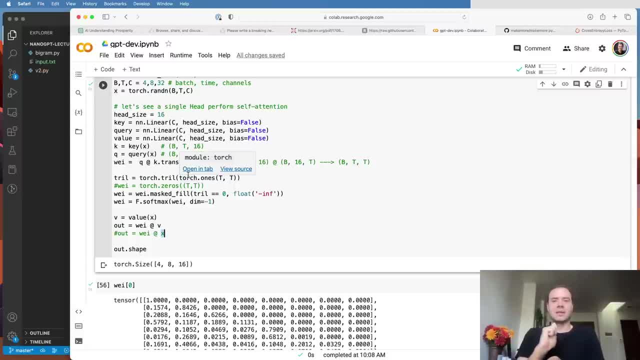 single head. i'm going to create a v, which is just achieved by propagating this linear on top of head. here's what I'm interested in, here's what I have and, if you find me interesting, here's what I will communicate to you and that's stored in. 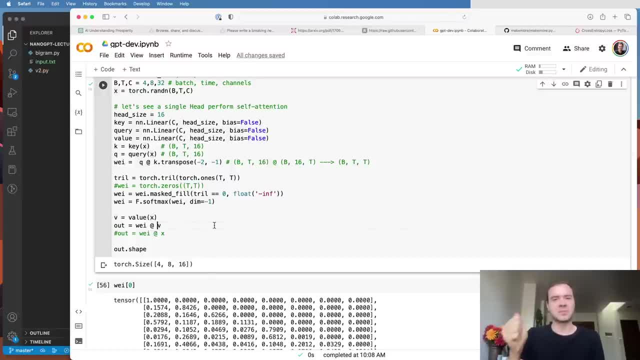 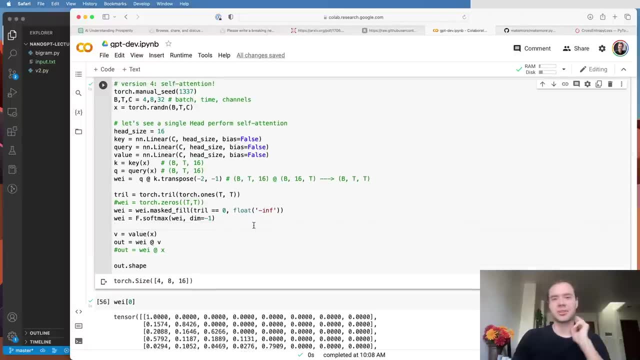 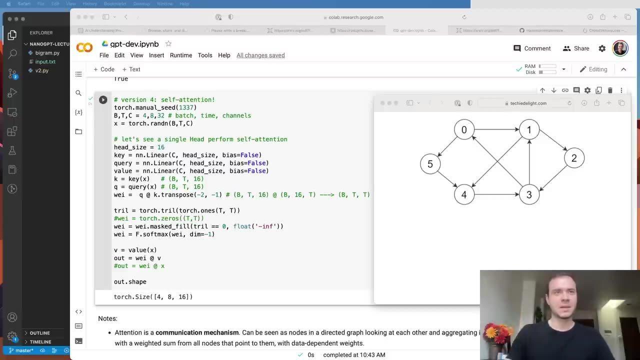 V, and so V is the thing that gets aggregated for the purposes of this single head between the different nodes, and that's basically the self attention mechanism. this is this is what it does. there are a few notes that I would make like to make about attention. number one: attention is a communication mechanism. 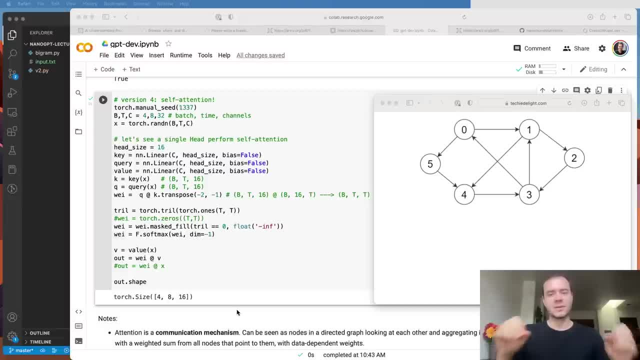 you can really think about it as a communication mechanism where you have a number of nodes in a directed graph where, basically, you have edges pointing between those like this, and what happens is every node has some vector of information and it gets to aggregate information via a weighted sum from all. 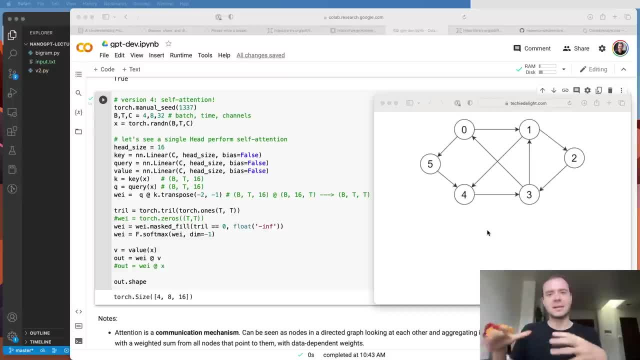 the nodes that point to it, and this is done in a data dependent manner, so depending on whatever data is actually stored at each node at any point in time. now our graph doesn't look like this. our graph has a different structure. we have eight nodes because the block size is eight and 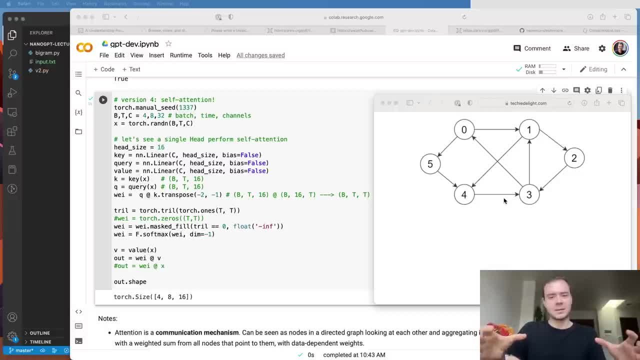 there's always eight tokens, and the first node is only pointed to by itself, the second node is pointed to by the first node and itself, all the way up to the eighth node, which is pointed to by all the previous nodes and itself, and so that's the structure that our directed graph has, or happens, happens to have in. 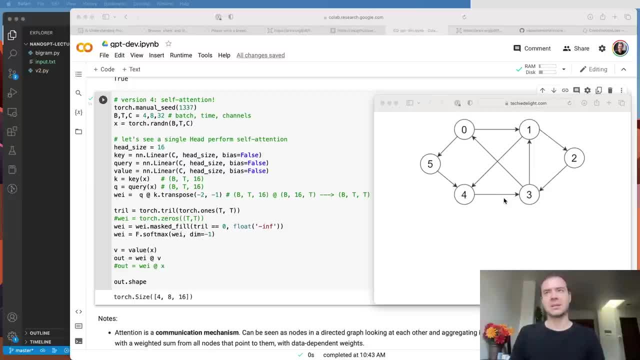 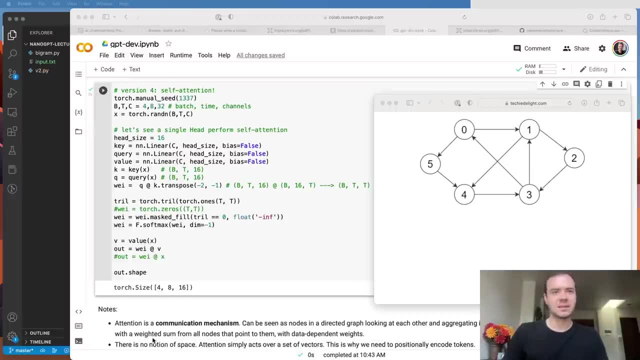 an autoregressive sort of scenario like language modeling, but in principle attention can be applied to any arbitrary directed graph and it's just a communication mechanism between the nodes. the second note is that notice that there is no notion of space, so attention simply acts over like a set of 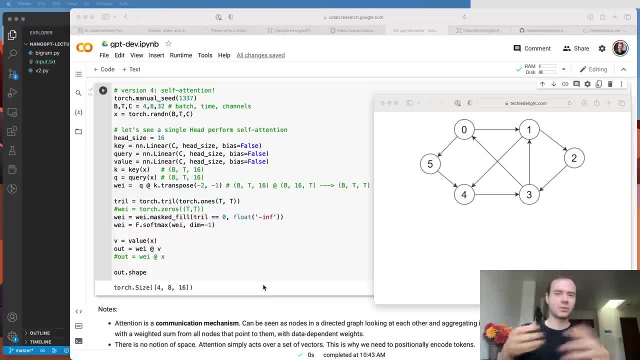 vectors in this graph, and so by default these nodes have no idea where they are positioned in the space, and that's why we need to encode them positionally and sort of give them some information that is anchors to a specific position, so that they sort of know where they are. and this is different than, for example, 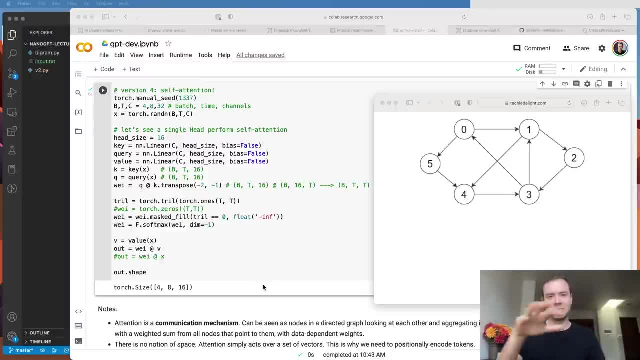 from convolution, because if you run, for example, a convolution operation over some input, there is a very specific sort of layout of the information in space and the convolutional filters sort of act in space and so it's. it's not like an attention and attention is just a set of vectors out there in space. they 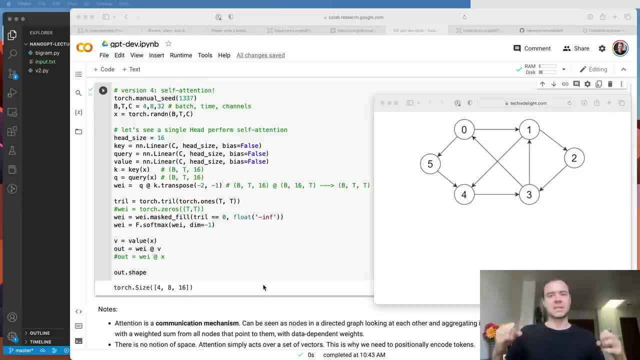 communicate and if you want them to have a notion of space, you need to specifically add it, which is what we've done when we calculated the relative, the positional encode, encodings and added that information to the vectors. the next thing that I hope is very clear is that the elements across the batch dimension 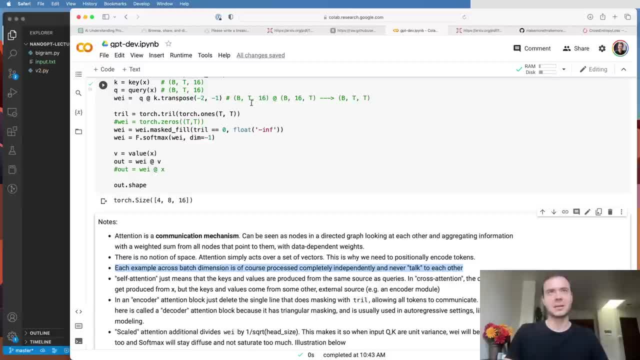 which are independent examples, never talk to each other. they're always processed independently and this is a batch matrix multiply that applies basically a matrix multiplication kind of in parallel across the batch dimension. so maybe it would be more accurate to say that in this analogy of a directed graph we really have, because the batch size is four, we really have. 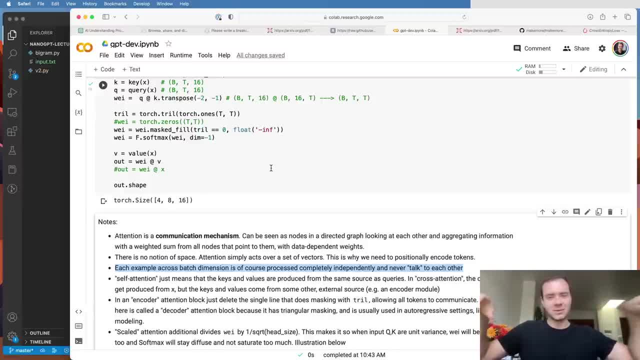 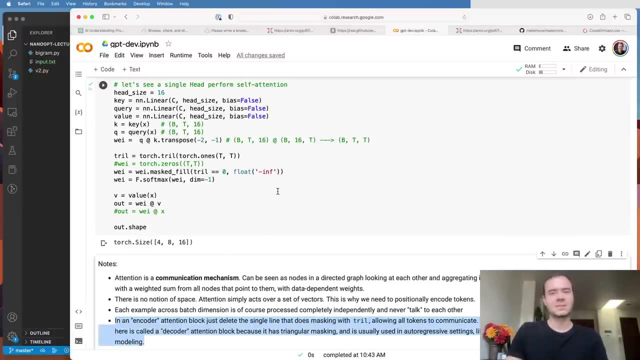 four separate pools of eight nodes, and those eight nodes only talk to each other, but in total there's like 32 nodes that are being processed, but there's sort of four separate pools of eight. you can look at it that way. the next note is that here, in the case of language modeling, we have this: 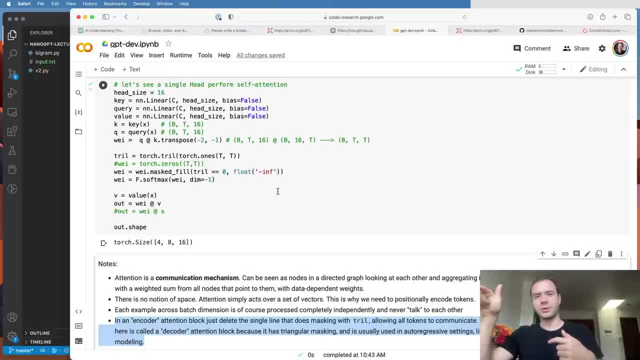 specific structure of directed graph where the future tokens will not communicate to the past tokens. but this doesn't necessarily have to be the constraint. in the general case, and in fact in many cases, you may want to have all of the nodes talk to each other fully. so, as an example, if you're doing 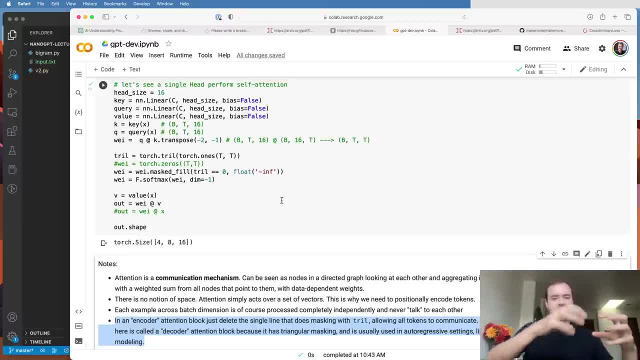 sentiment analysis or something like that. with a transformer, you might have a number of tokens and you may want to have them all talk to each other fully, because later you are predicting, for example, the sentiment of the sentence, and so it's okay for these nodes to talk to each other, and so in those cases you 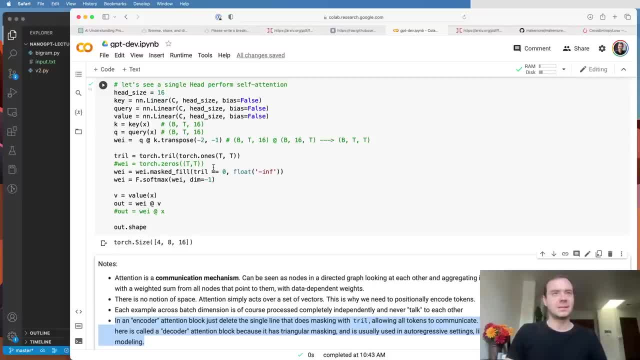 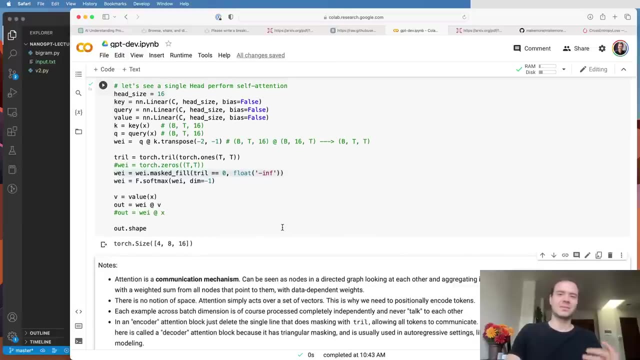 will use an encoder block of self-attention, and all it means that it's an encoder block is that you will delete this line of code, allowing all the nodes to completely talk to each other. what we're implementing here is sometimes called a decoder block, and it's called a decoder because it is sort of like decoding language and it's. 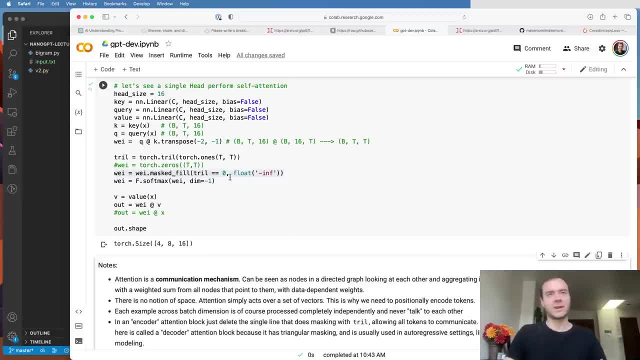 got this autoregressive format where you have to mask with the triangular matrix so that nodes from the future never talk to the past because they would give away the answer, and so basically in encoder blocks you would delete this. allow all the nodes to talk in decoder blocks. this will always be. 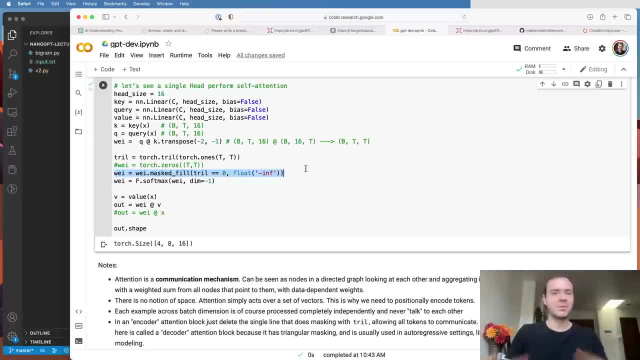 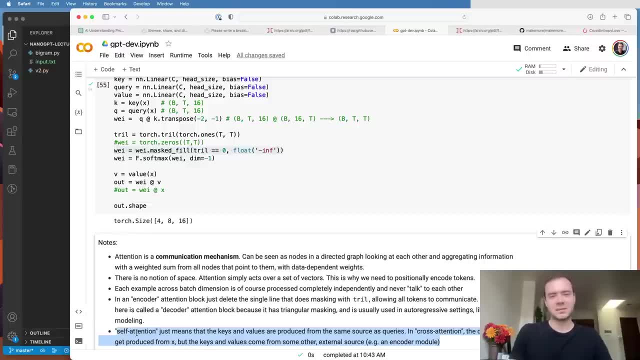 present so that you have this triangular structure. but both are allowed and attention doesn't care. attention supports arbitrary connectivity between nodes. the next thing I wanted to comment on is: you keep me. you keep hearing me say attention, self-attention, etc. there's actually also something called cross attention. what is the? 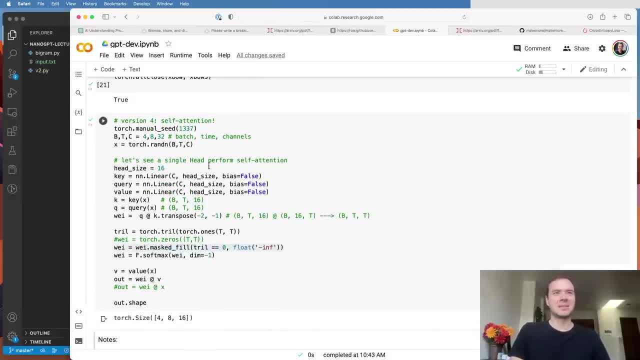 difference. so basically, the reason this attention is self-attention is because the keys, queries and the values are all coming from the same source, from X. so the same source, X, produces keys, queries and values. so these nodes are self-attending. but in principle, attention is much more general than that. 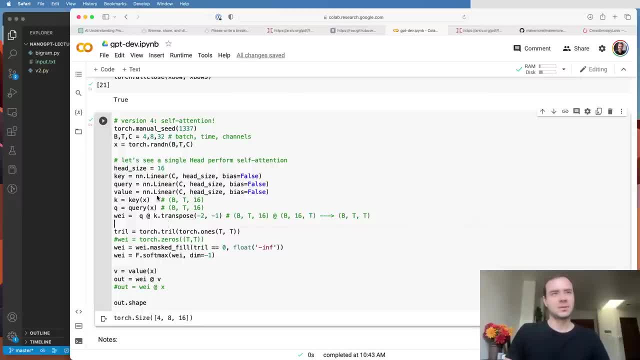 so, for example, in encoder, decoder transformers, you can have a case where the queries are produced from X, but the keys and the values come from a whole separate external source and sometimes from encoder blocks that encode some context that we'd like to condition on, and so the keys and the values will. 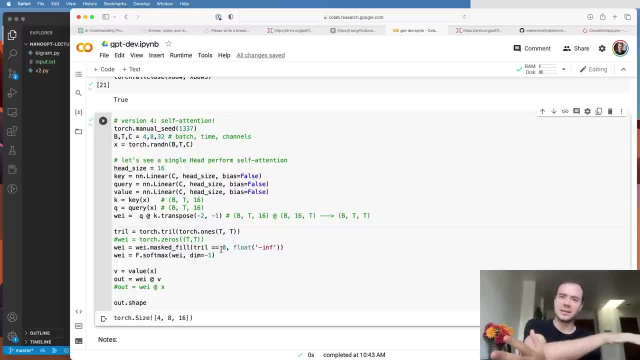 actually come from a whole separate source. those are nodes on the side and here we're just producing queries and we're reading off information from the side. so cross attention is used when there's a separate source of nodes we'd like to pull information from into our nodes, and it's self-attention. 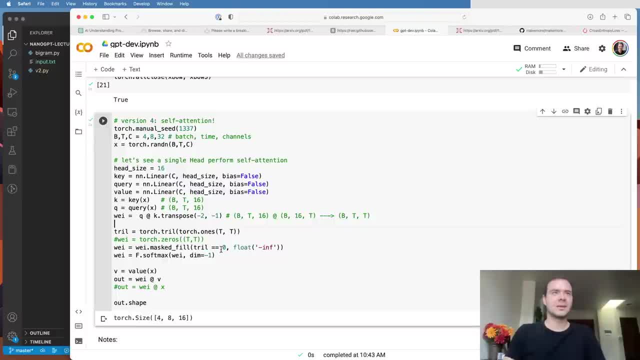 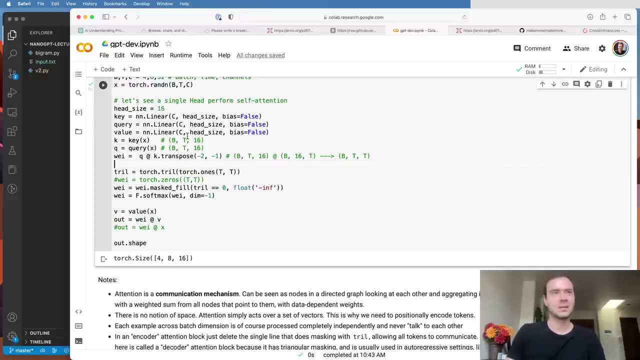 if we just have nodes that would like to look at each other and talk to each other. so this attention here happens to be self attention, but in principle attention is a lot more general. okay, in the last note at this stage is: if we come to the attention is only need paper, here we've already. 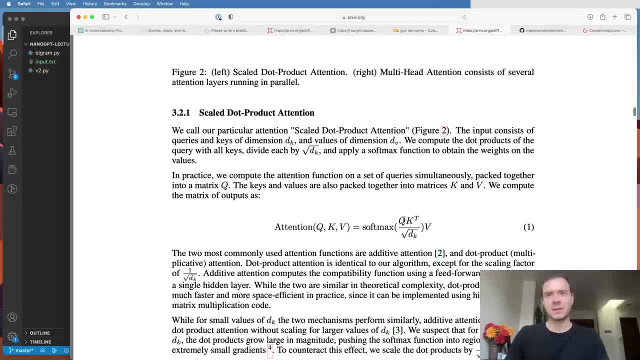 implemented. attention. so, given query, key and value, we've multiplied the query and the key, we've soft maxed it and then we are aggregating the values. there's one more thing that we're missing here, which is the dividing by one over square root of the head size. The dk here is the head size. Why are they doing this? 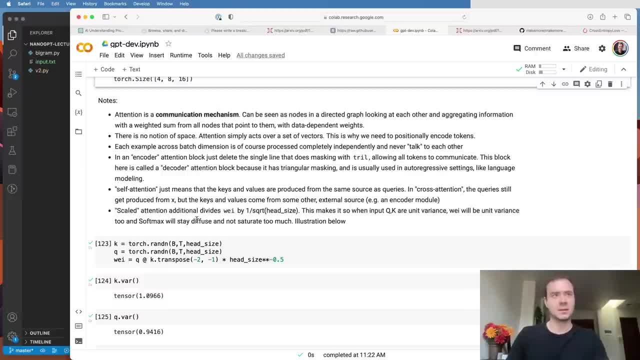 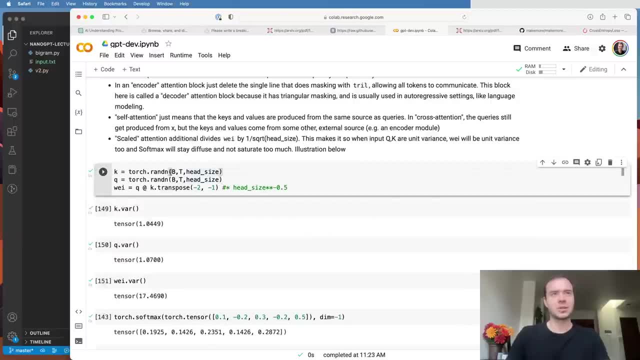 Why is this important? So they call it a scaled attention and it's kind of like an important normalization to basically have. The problem is, if you have unit Gaussian inputs, so zero mean unit variance, k and q are unit Gaussian- then if you just do way naively, then you see that your way actually will be the 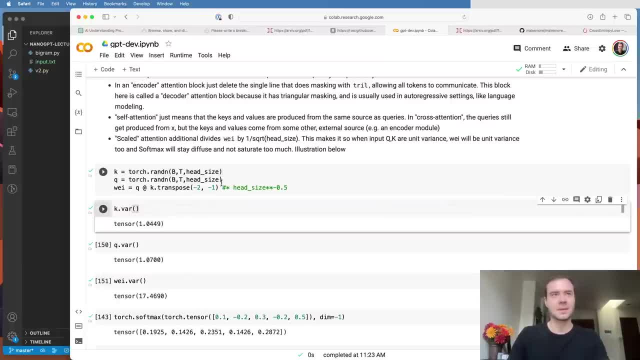 variance will be on the order of head size, which in our case is 16.. But if you multiply by 1 over head size- square root- so this is square root and this is 1 over- then the variance of way will be 1, so it will be preserved. Now, why is this? 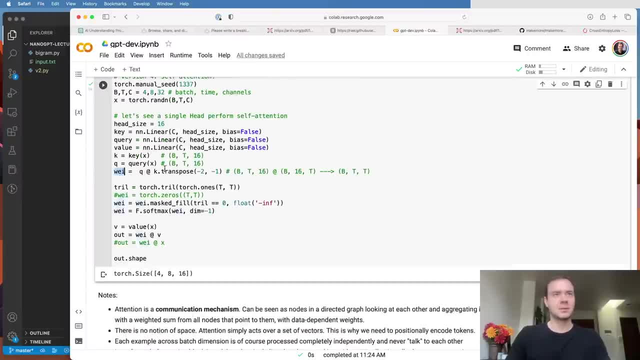 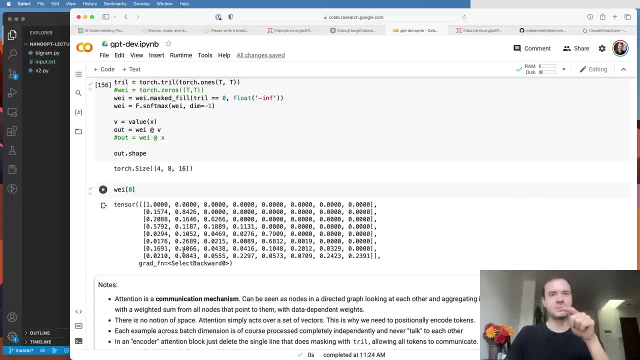 important, You'll notice, that way here will feed into softmax and so it's really important, especially at initialization, that way be fairly diffuse. So in our case here we sort of lucked out here and way had a fairly diffuse numbers here. So 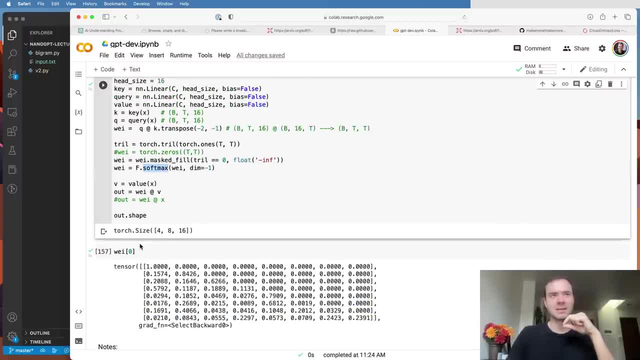 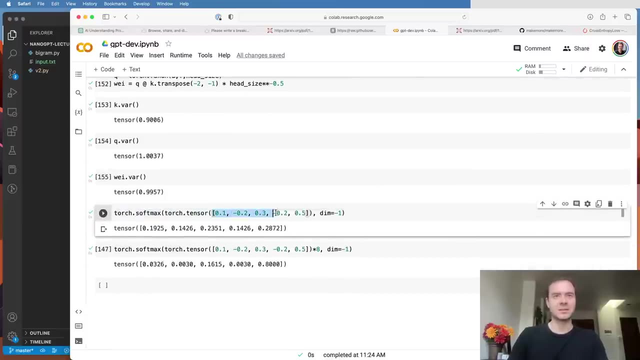 we're going to get a diffuse thing like this. Now the problem is that because of softmax, if way takes on very positive and very negative numbers inside it, softmax will actually converge towards one-hot vectors, And so I can illustrate that here. Say, we are applying softmax to a tensor of values that are very close. 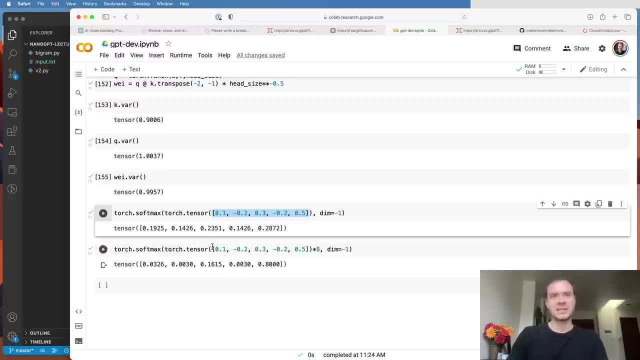 to zero, then we're going to get a diffuse thing out of softmax. But the moment I take the exact same thing and I start sharpening it, making it bigger by multiplying these numbers by 8, for example, it will start to sharpen and in fact it will sharpen towards the max. So it will 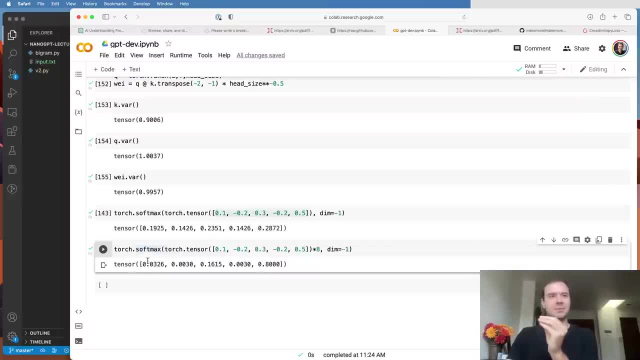 sharpen towards whatever number here is the highest, And so basically we don't want these values to be too extreme, especially at initialization. otherwise softmax will be way too peaky and you're basically aggregating information from like a single node. Every node just aggregates information from a single. 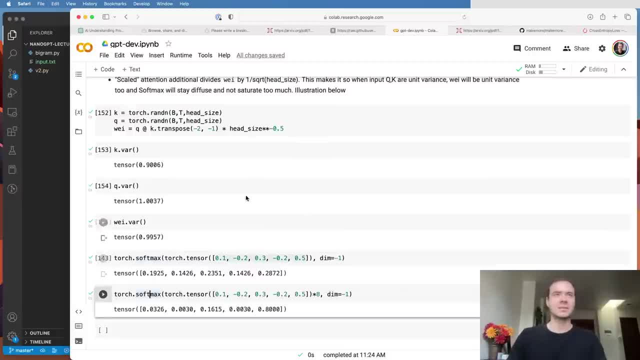 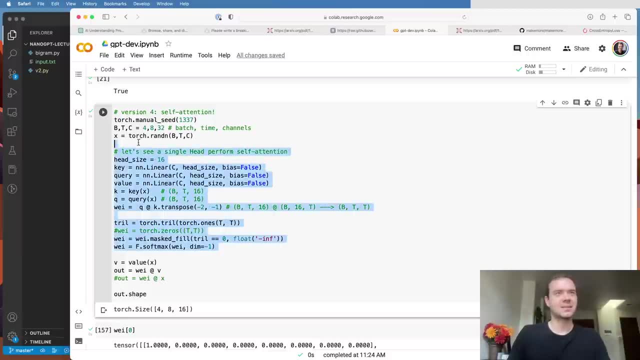 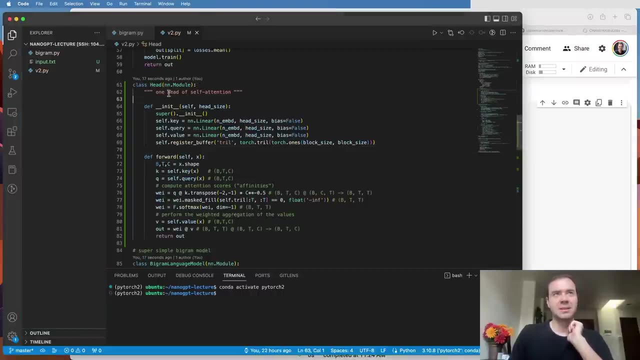 other node. That's not what we want, especially at initialization, And so the scaling is used just to control the variance at initialization. Okay, so we've done all that. let's now take our self-attention knowledge and let's take it for a spin. So here in the code, I've created this head module and it 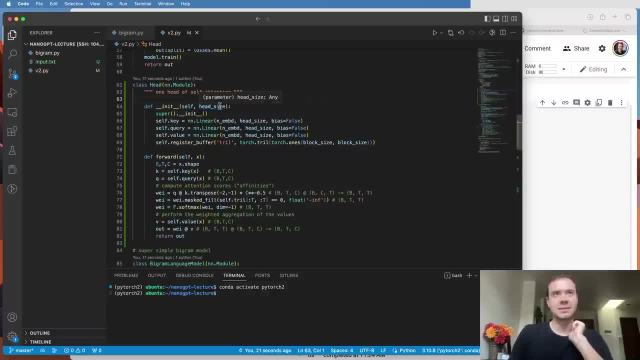 implements a single head of self-attention, So you give it a head size and then here it creates the key query and the value: linear layers. Typically, people don't use biases in these, So those are the linear projections that we're going to apply to all of our nodes. Now here I'm creating this trill. 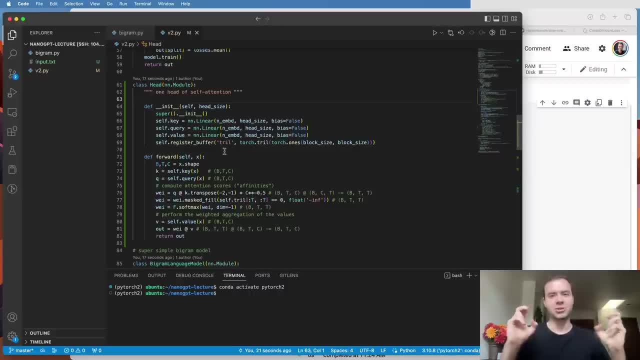 variable Trill is not a parameter of the module, so in sort of PyTorch naming functions this is called a buffer. It's not a parameter and you have to assign it to the module using a register buffer, So that creates the trill. 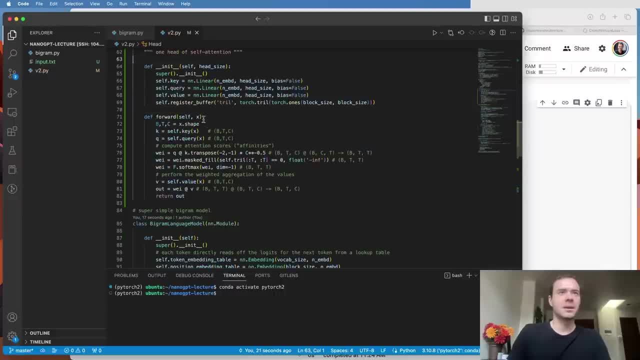 the lower triangular matrix And when we're given the input x. this should look very familiar now. We calculate the keys, the queries, we calculate the attention scores inside way. we normalize it. so we're using scaled attention here. then we make sure that future doesn't communicate with the past. so this makes 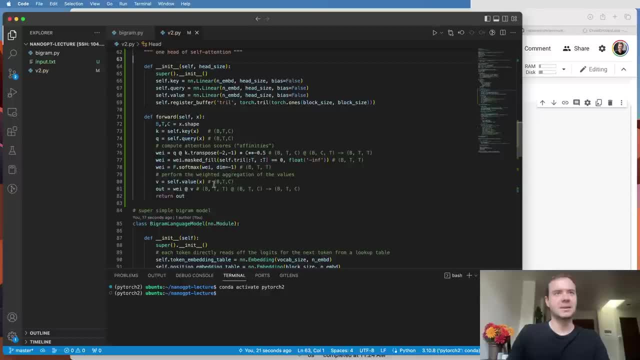 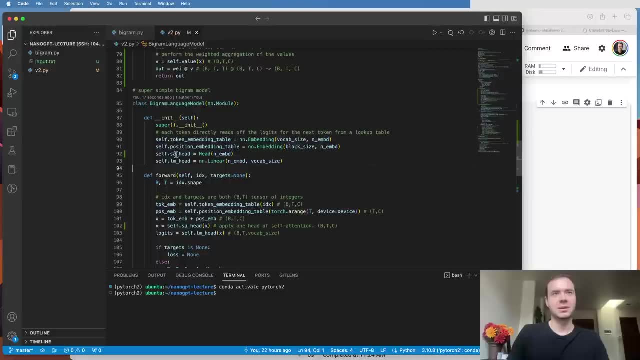 it a decoder block, So we'll call this addTax and then aggregate the value and output. Then here in the language model, I'm creating a head in the constructor and I'm calling it self-attention head and the head size I'm going to keep as the 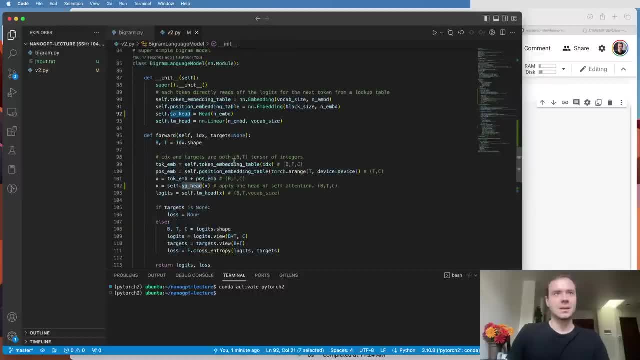 same and embed just for now. And then here, once we've encoded the information with the token embeddings and the position embeddings, we're simply going to feed it into the self-attention head and then the output of that is going to go into the decoder language modeling head. 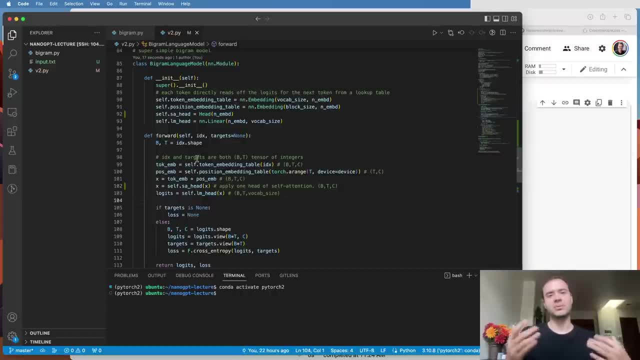 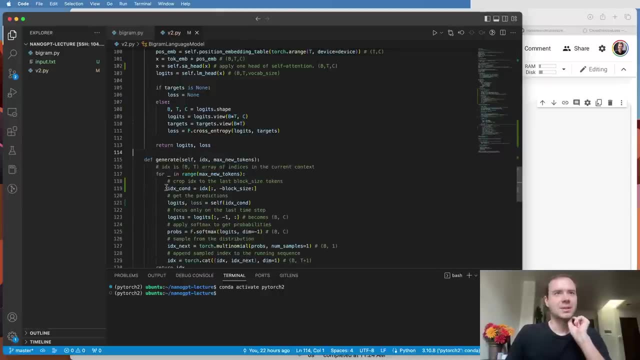 create the logits. So this is sort of the simplest way to plug in a self-attention component into our network right now. I had to make one more change, which is that here in the generate we have to make sure that our IDX that we feed into the model, because now we're using positional embeddings. we 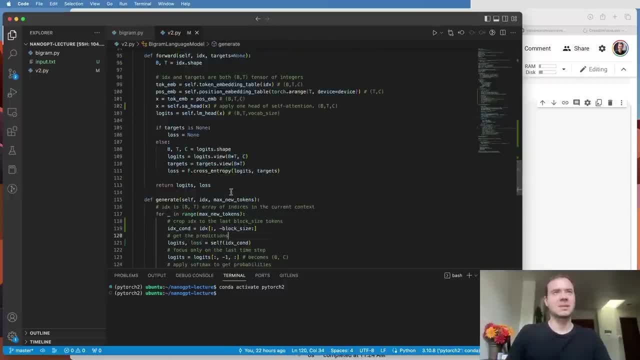 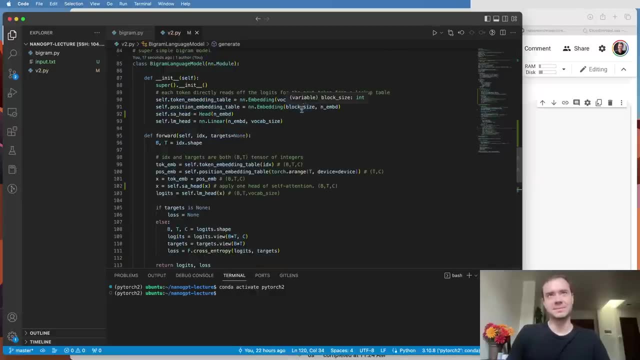 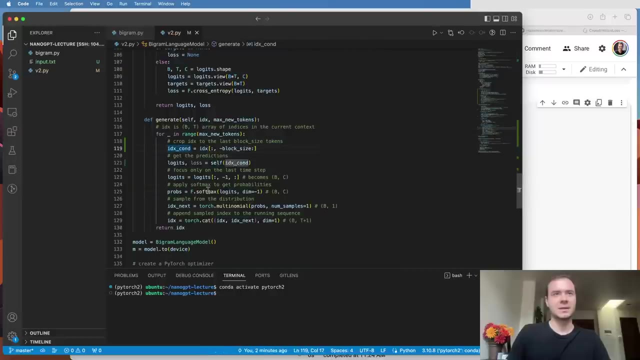 can never have more than block size coming in, because if IDX is more than block size, then our position embedding table is going to run out of scope because it only has embeddings for up to block size, and so, therefore, I added some code here to crop the context that we're gonna feed into self, so that we 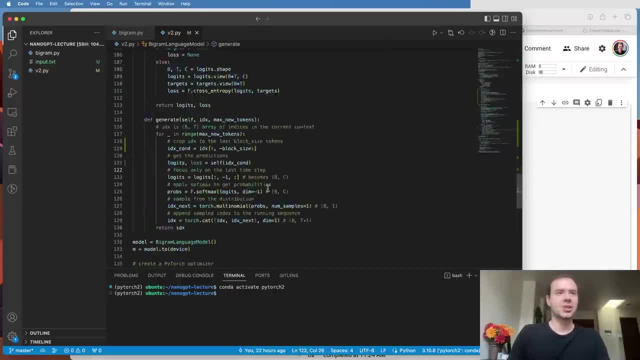 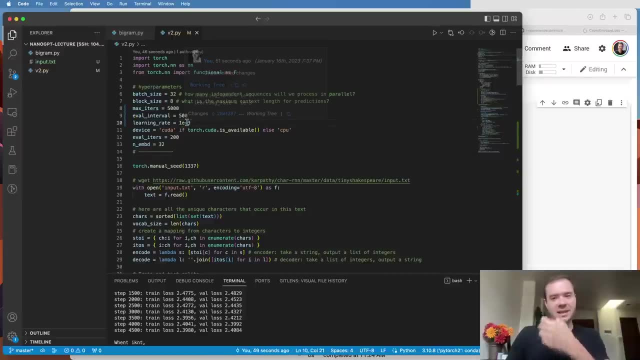 never pass in more than block size elements. So those are the changes, and let's now train the network. Okay, so I also came up to the script here and I decreased the learning rate because the self-attention can't tolerate very, very high learning rates. and then I also increased number of iterations because 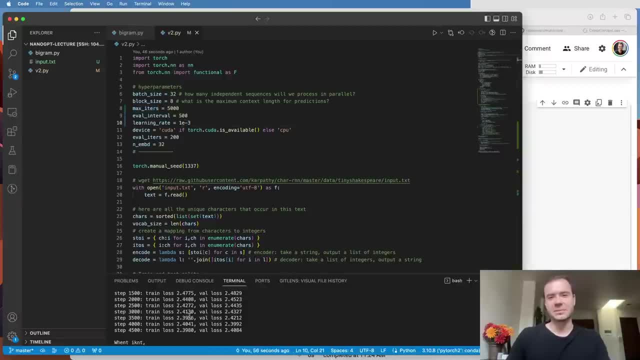 the learning rate is lower and then I trained it and previously we were only able to get to up to 2.5 and now we are down to 2.4. so we definitely see a little bit of improvement from 2.5 to 2.4 roughly, but the text is still not. 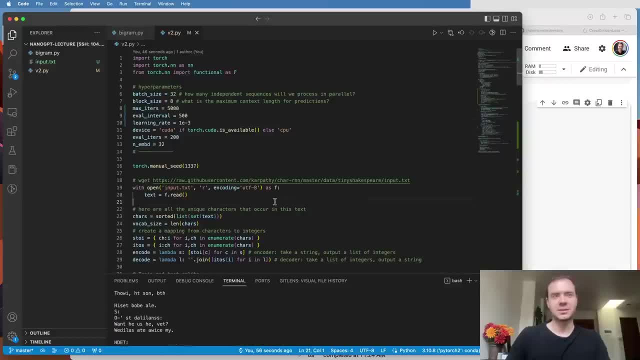 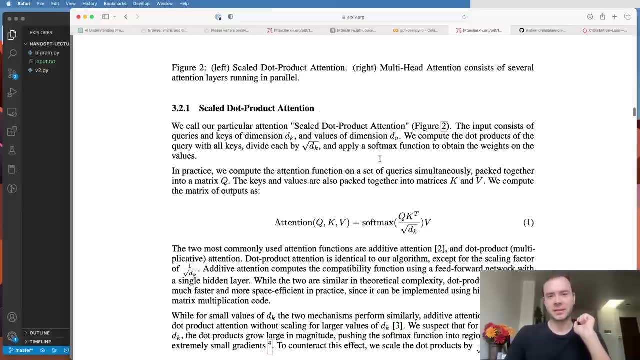 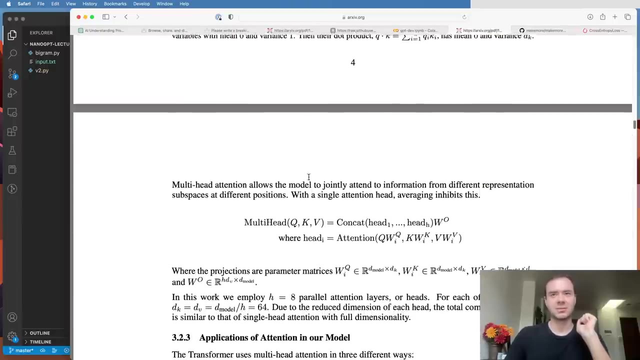 amazing. So clearly the self-attention head is doing some useful communication, but we still have a long way to go. Okay, so now we've implemented the scale dot product attention. Now, next up in the attention is all you need paper. there's something called multi-head attention. and what is multi-head attention? It's 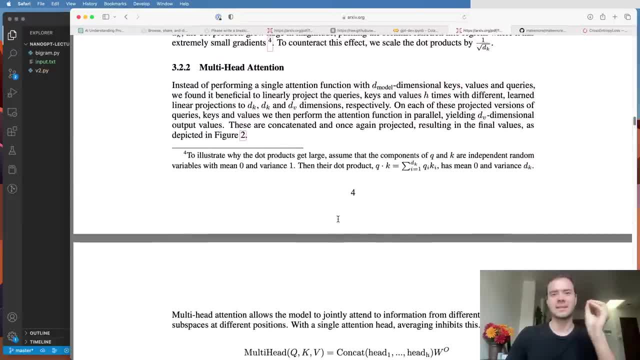 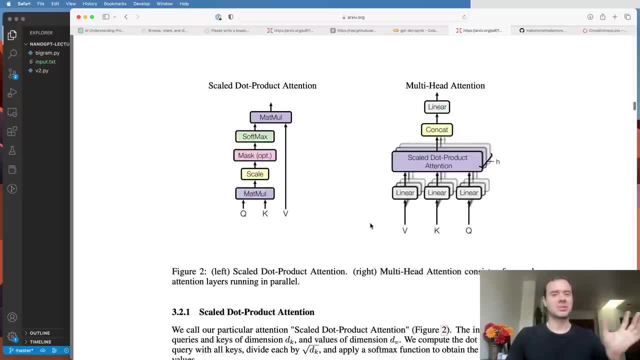 just applying multiple attentions in parallel to the self-attention. So let's go ahead and do this. So let's say we want multiple heads of self-attention running in parallel and concatenating the results. So they have a little bit of diagram here. I don't know if this is super clear. It's really just multiple. 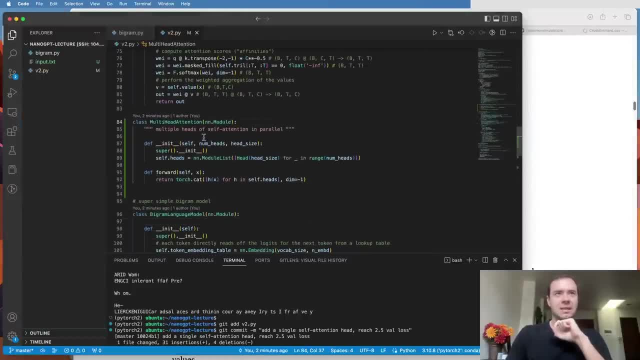 attentions in parallel. So let's implement that fairly straightforward. If we want a multi-head attention, then we want multiple heads of self-attention running in parallel. So in PyTorch we can do this by simply creating multiple heads, So however many heads you want, and then what is the head size of each? So 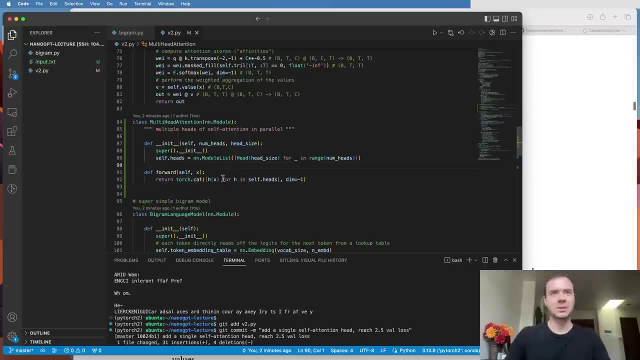 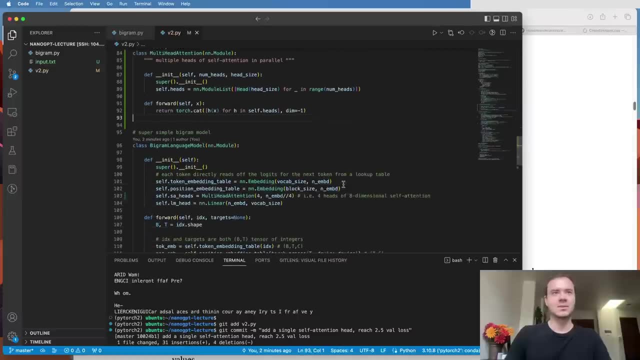 instead of having one communication channel at the end of the channel, we can call it the head size of 32.. And then we run all of them in parallel into a list and simply concatenate all of the outputs and we're concatenating over the channel dimension. So the way this looks now is we don't have just a single. 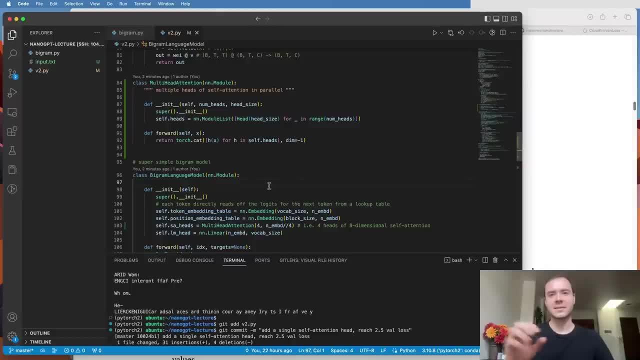 attention- that has a head size of 32 because, remember, n embed is 32.. Instead of having one communication channel, we now have four communication channels in parallel and each one of these communication channels typically will be smaller correspondingly. So because we have four communication channels, we want eight-dimensional. 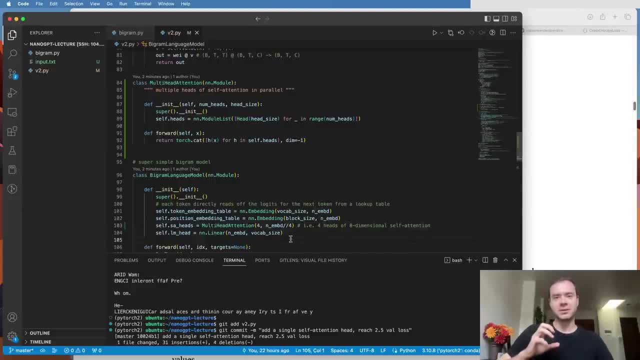 self-attention. And so from each communication channel we're getting together eight-dimensional vectors, and then we have four of them and that concatenates to give us 32, which is the original N-embed. And so this is kind of similar to- if you're familiar with convolutions, this is kind 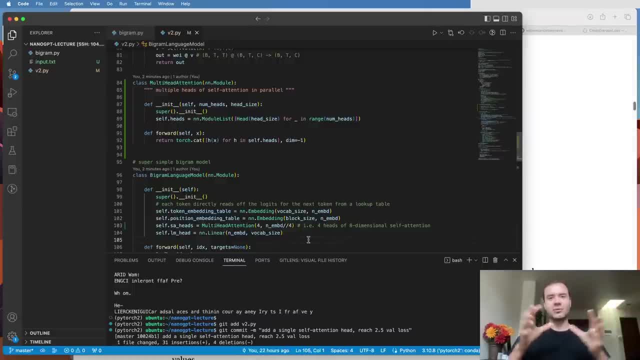 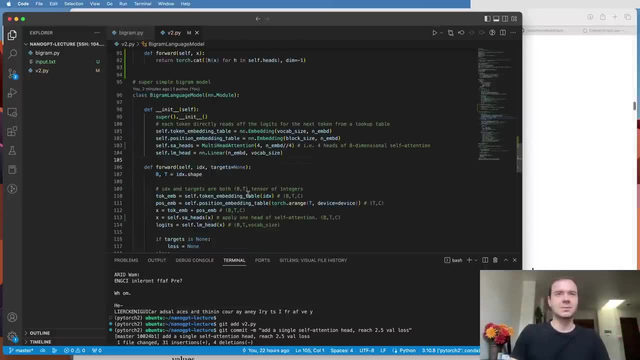 of like a group convolution, because basically, instead of having one large convolution, we do convolution in groups and that's multi-headed self-attention. And so then here we just use assay heads, self-attention heads instead. Now I actually ran it and scrolling down, 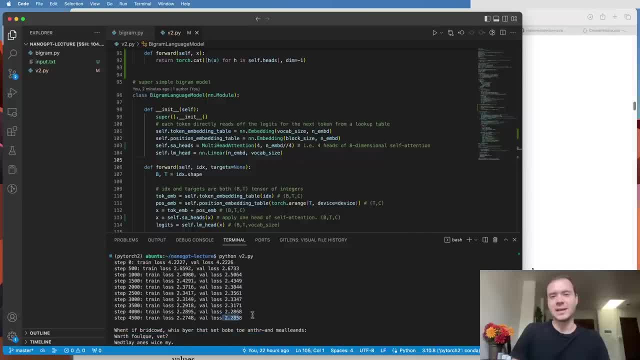 I ran the same thing and then we now get down to 2.28, roughly And the output is still. the generation is still not amazing, but clearly the validation loss is improving because we were at 2.4 just now, And so it helps to have multiple communication channels. 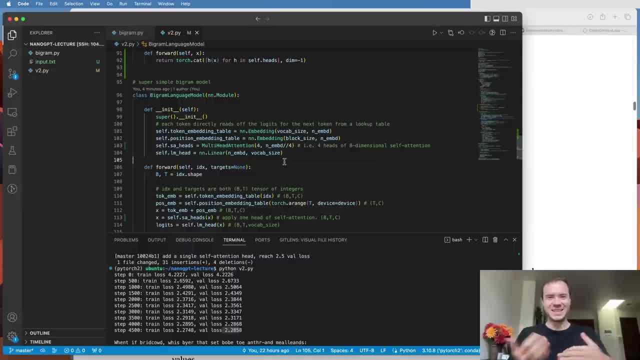 because obviously these tokens have a lot to talk about. They want to find the consonants, the vowels. they want to find the vowels just from certain positions, they want to find any kinds of different things, And so it helps to create multiple independent channels of communication gather. 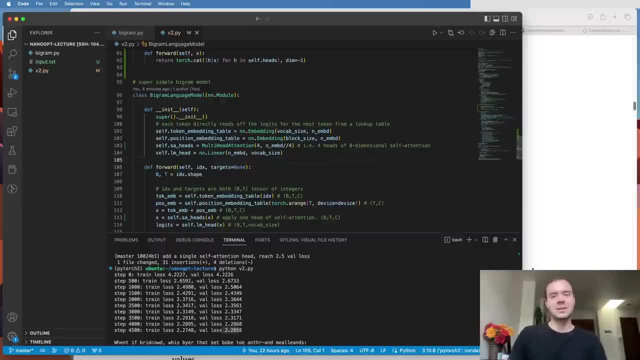 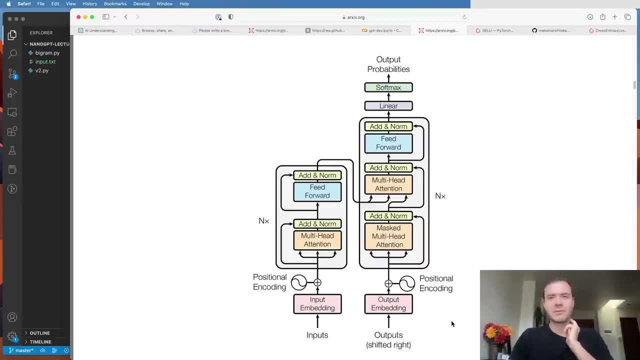 lots of different types of data and then decode the output. Now, going back to the paper for a second, of course I didn't explain this figure in full detail, but we are starting to see some components of what we've already implemented. We have the positional encodings, the token, 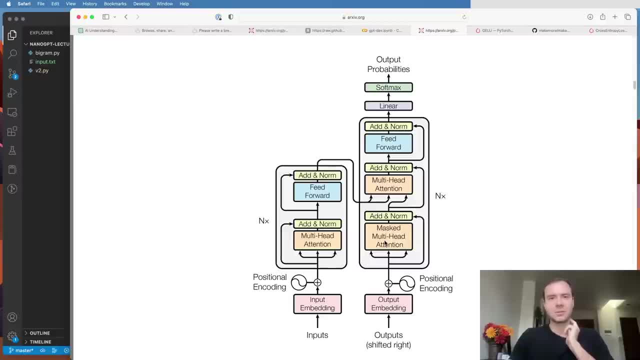 encodings that add: we have the masked multi-headings. we have the masked multi-headings. we have the multi-headed attention implemented. Now here's another multi-headed attention, which is a cross attention to an encoder which we haven't. we're not going to implement. in this case, I'm going to. 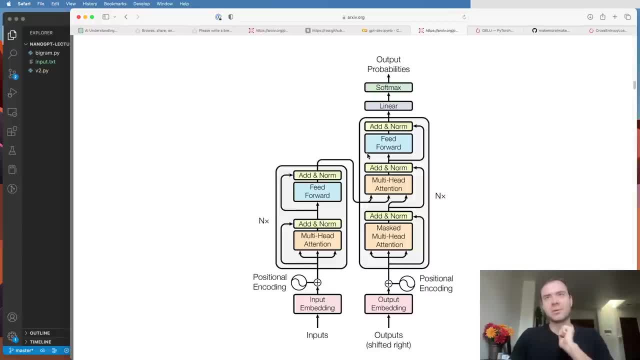 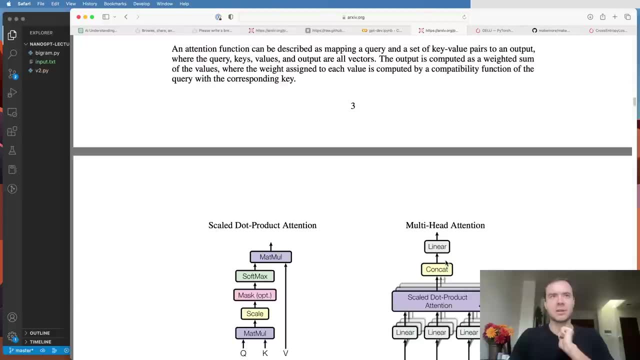 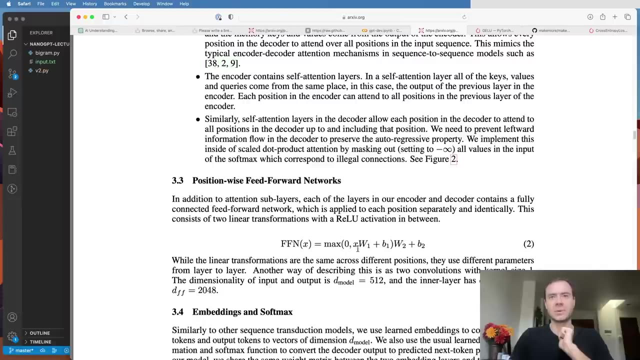 come back to that later, But I want you to notice that there's a feedforward part here and then this is grouped into a block that gets repeated again and again. Now the feedforward part here is just a simple multilayer perceptron, So the multi-headed, so here, position-wise feedforward. 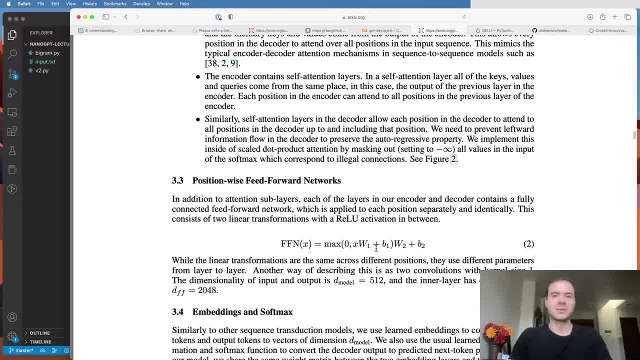 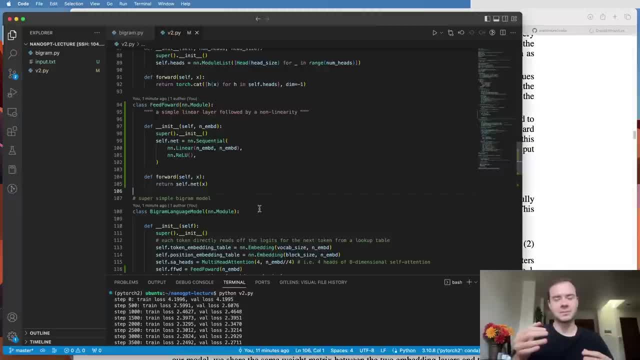 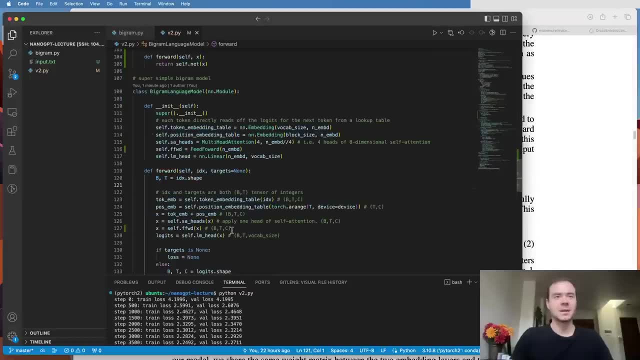 networks is just a simple little MLP, So I want to start basically in a similar fashion, also adding computation into the network, And this computation is on a per node level. So I've already implemented it and you can see the diff highlighted on the left here when I've added or changed things Now, before we had the multi-headed self. 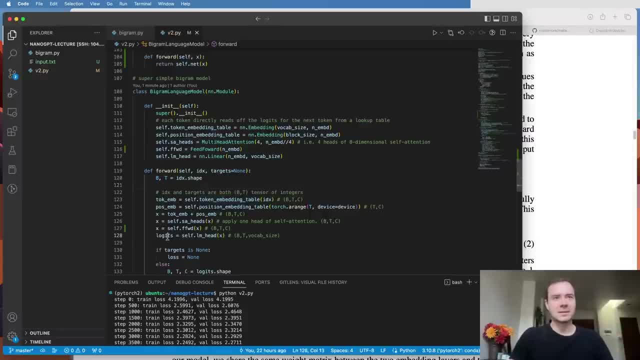 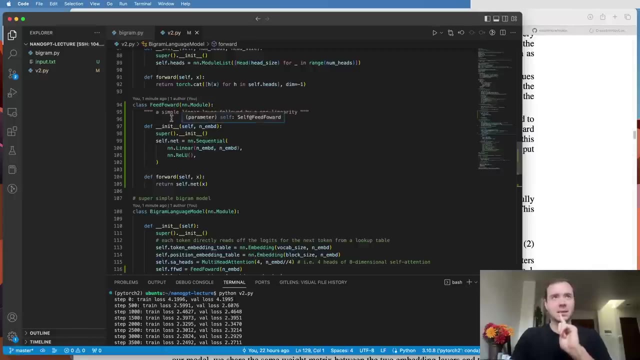 attention. that did the communication, but we went way too fast to calculate the logits, So the tokens looked at each other but didn't really have a lot of time to think on what they found from the other tokens, And so what I've implemented here is a little feedforward single layer And this little 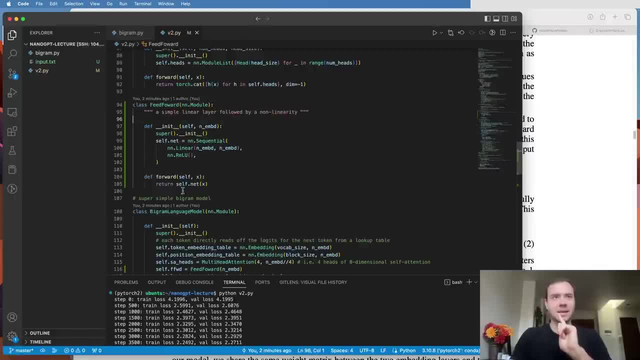 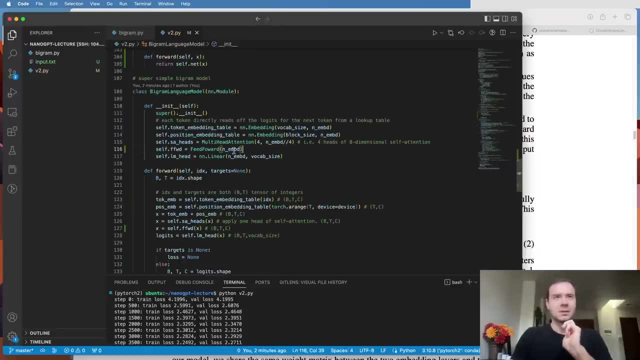 layer is just a linear, followed by a relu non-linearity, And that's it. So it's just a little layer And then I call it feedforward and embed, And then this feedforward is just called sequentially right after the self attention. So we self attend, then we feedforward, And you'll. 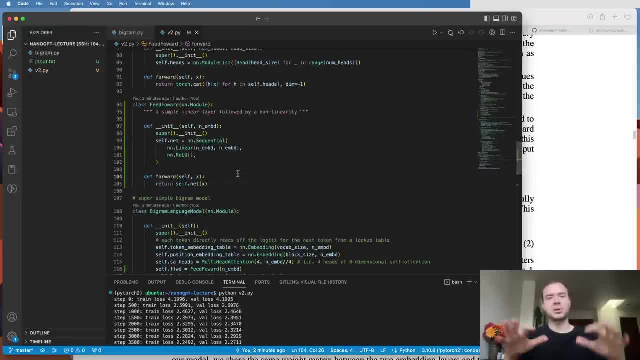 notice that the feedforward here, when it's applying linear this, is on a per token level, All the tokens. we do this independently, So the self attention is the communication, And then, once they've gathered all the data, now they need to think on that data individually, And so that's what feedforward is doing. 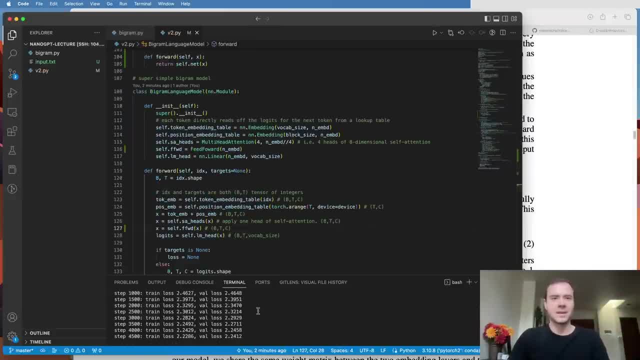 And that's why I've added it here Now, when I train this, the validation loss actually continues to go down, now to 2.24, which is down from 2.28.. The output still looks kind of terrible, but at least. 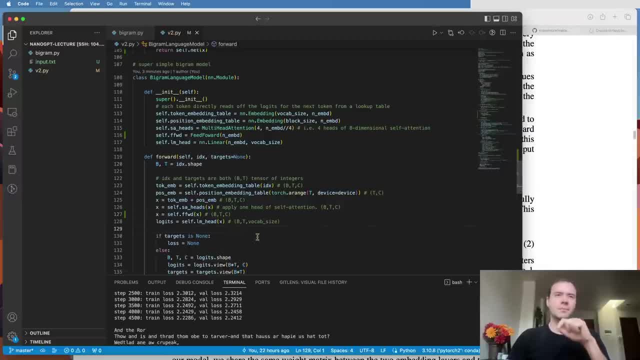 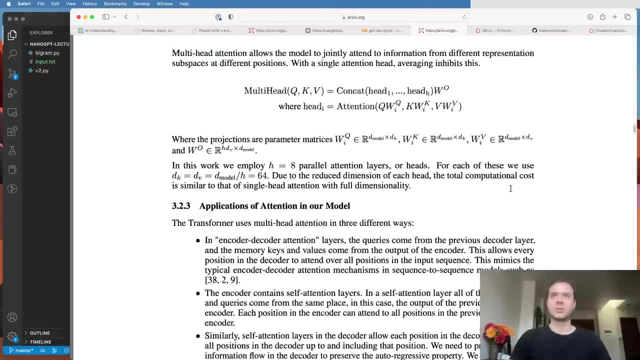 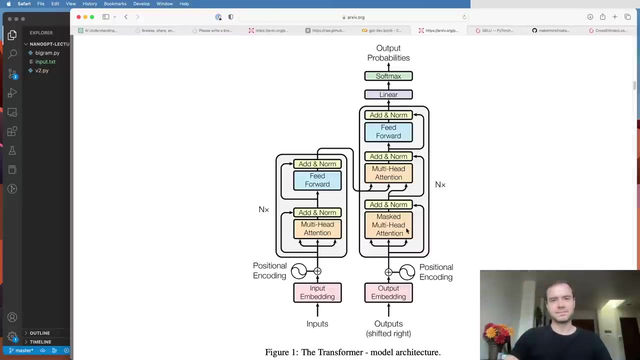 we've improved the situation And so, as a preview, we're going to now start to intersperse the communication with the computation, And that's also what the transformer does when it has blocks that communicate and then compute, And it groups them and replicates them. Okay, so let me show you. 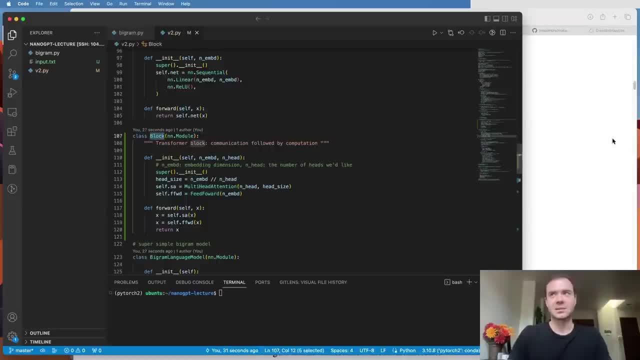 what we'd like to do. We'd like to do something like this: We have a block, And this block is basically this part here, except for the cross attention. Now, the block basically intersperses communication and then computation. The computation is done using multi-headed self attention And then 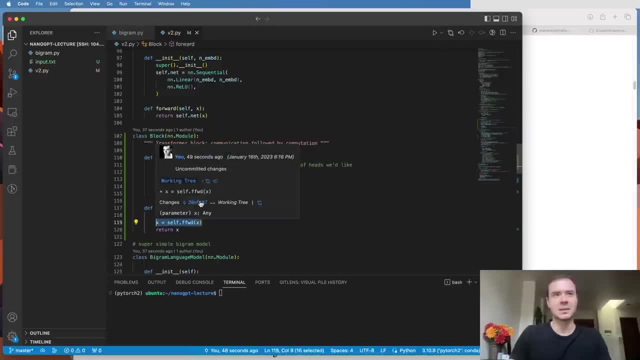 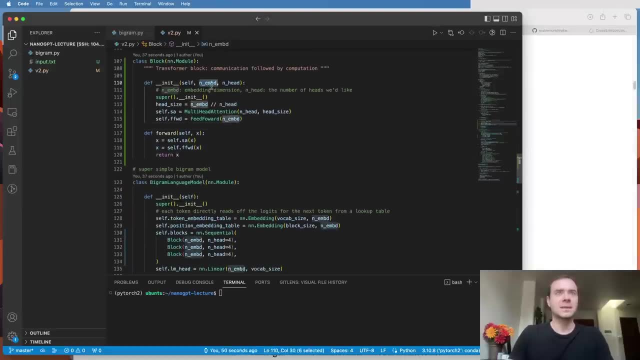 computation is done using a feedforward network on all the tokens independently. Now, what I've added here also is, you'll notice, this takes the number of embeddings in the embedding dimension and number of heads that we would like, which is kind of like group size in group convolution, And 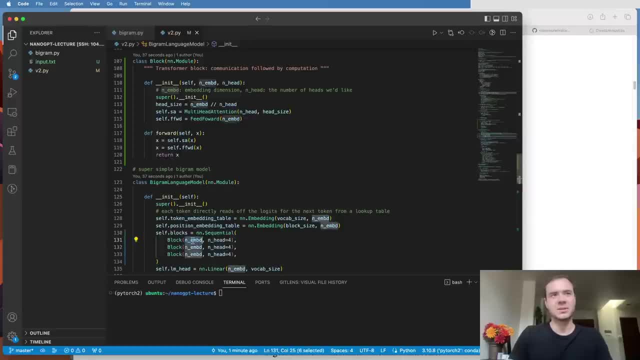 I'm saying that number of heads we'd like is four, And so because this is 32, we calculate that because this is 32, the number of heads should be four, The head size should be eight, so that everything sort of works out channel-wise. 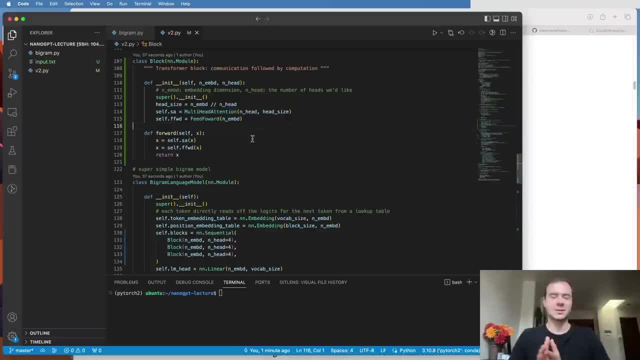 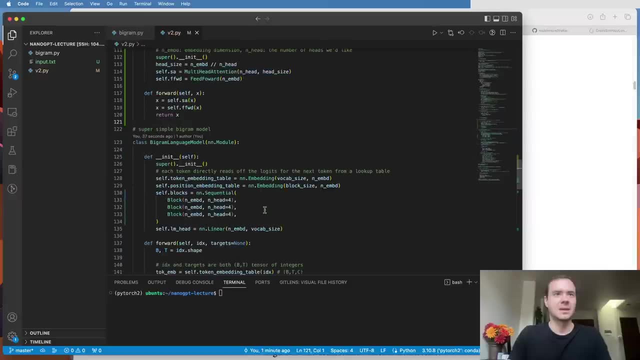 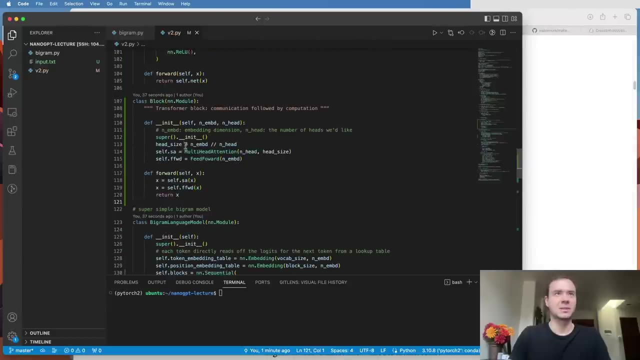 So this is how the transformer structures sort of the sizes typically. So the head size will become eight, And then this is how we want to intersperse them. And then here I'm trying to create blocks, which is just a sequential application of block, block, block. So then we're interspersing. 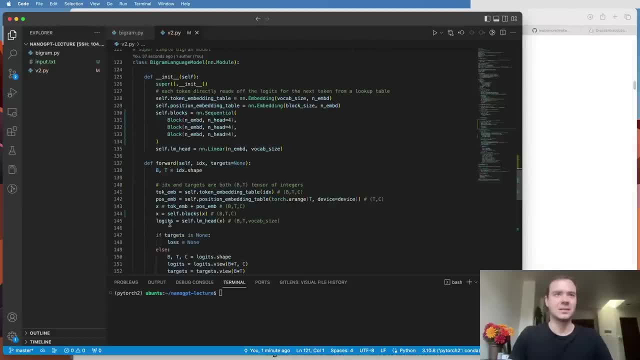 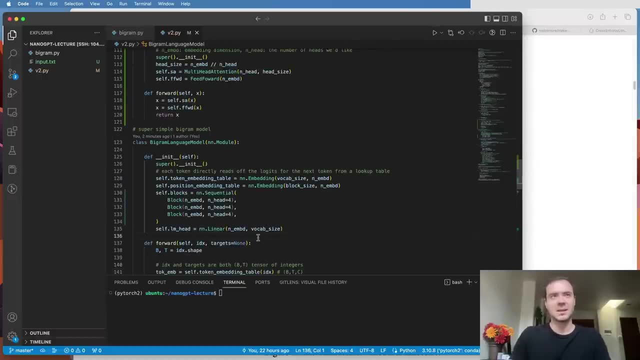 communication feedforward many, many times And then finally we decode. Now I actually tried to run this And the problem is this doesn't actually give a very good answer, a very good result, And the reason for that is we're starting to actually get like a pretty deep neural net, And deep neural 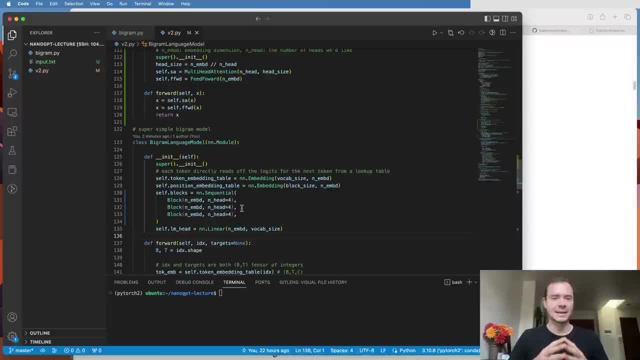 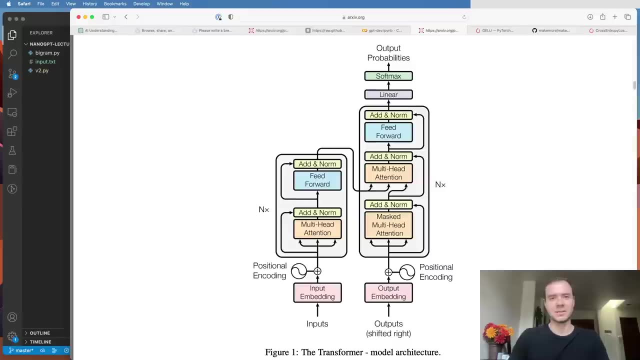 nets suffer from optimization issues, And I think that's what we're kind of like slightly starting to run into. So we need one more idea that we can borrow from the transformer paper to resolve those difficulties. Now there are two optimizations that dramatically help with the depth of these. 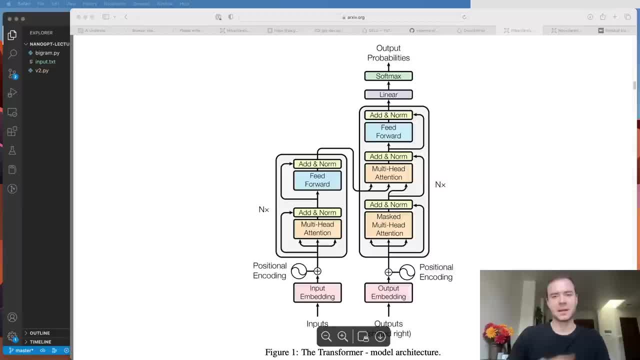 networks and make sure that the networks remain optimizable. Let's talk about the first one. The first one in this diagram is: you see this arrow here And then this arrow and arrow. those are skip connections, or sometimes called residual connections. They come from this: 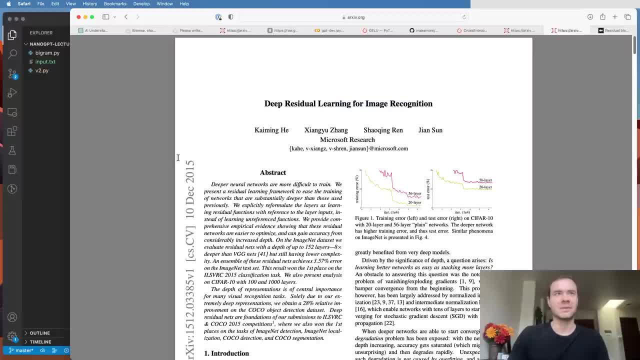 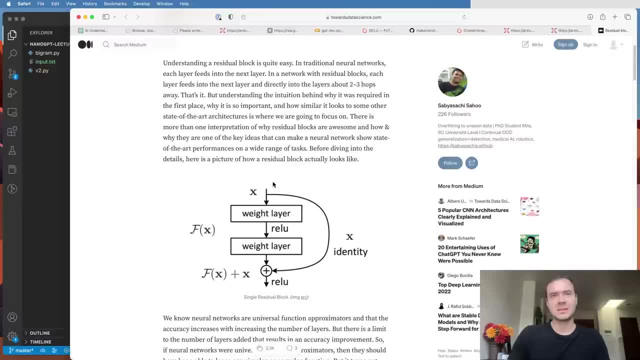 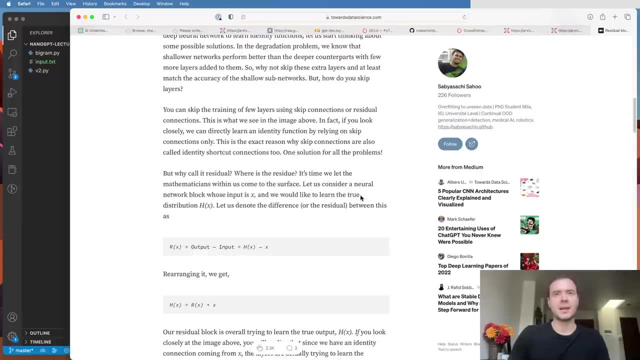 paper, the Procedural Learning for Image Recognition- from about 2015 that introduced the concept. Now these are basically. what it means is you transform the data, but then you have a skip connection with addition from the previous features. Now the way I like to visualize: 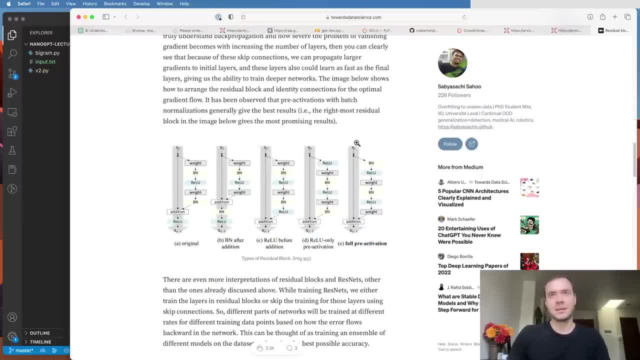 it that I prefer is the following: Here the computation happens from the top to bottom And basically you have this residual pathway And you are free to fork off from the residual pathway, perform some computation and then project back to the residual pathway via addition. 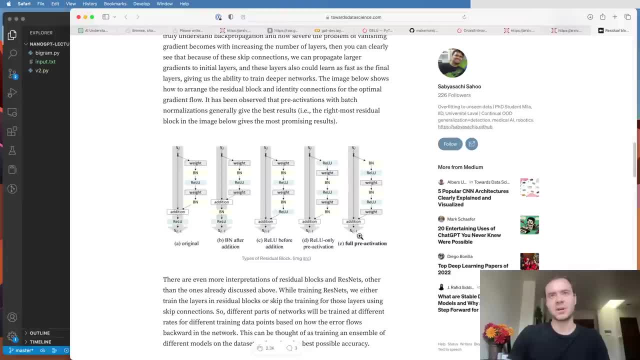 And so you go from the inputs to the targets only via plus and plus and plus. And the reason this is useful is because during that propagation- remember from our micrograd video earlier addition- distributes gradients equally to both of its branches that fed as the input. 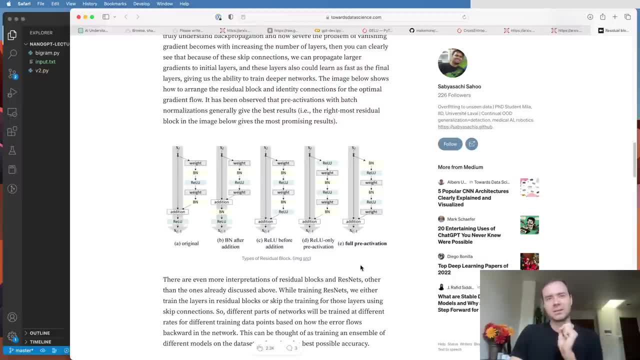 And so the supervision or the gradients from the loss hop through every addition node all the way to the input and then also fork off into the residual blocks. But basically you have this gradient superhighway that goes directly from the supervision all. 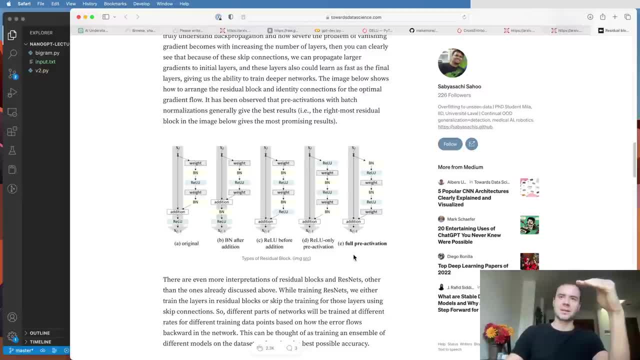 the way to the input unimpeded. And then these residual blocks are usually initialized in the beginning, so they contribute very, very little, if anything, to the residual pathway. They are initialized that way, So independently. instead of a little bit they arepricher, they are explained. 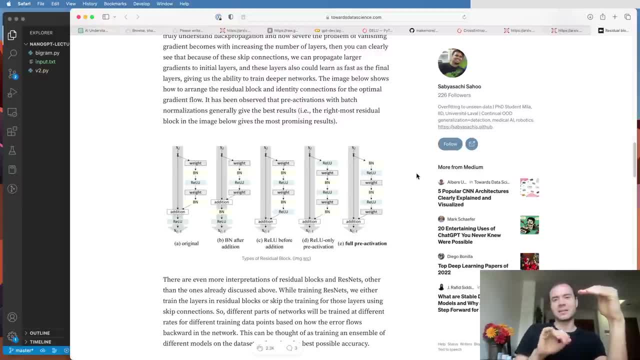 they contribute very, very little, if anything, to the residual pathway. they are initialized that way, So independently. So in the beginning they are almost kind of like not there, But then during the optimization they come online over time and they start to contribute. 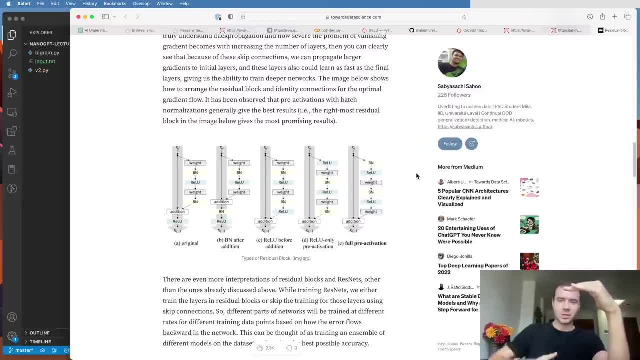 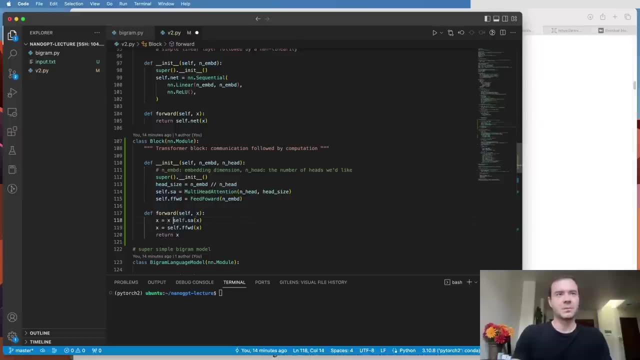 But at least at the initialization you can go from directly supervision to the input Gradient is unimpeded and just flows, And then the blocks over time kick in, And so that dramatically helps with the optimization. So let's implement this. So, coming back to our block here, basically what we want to do is we want to do x equals x plus. 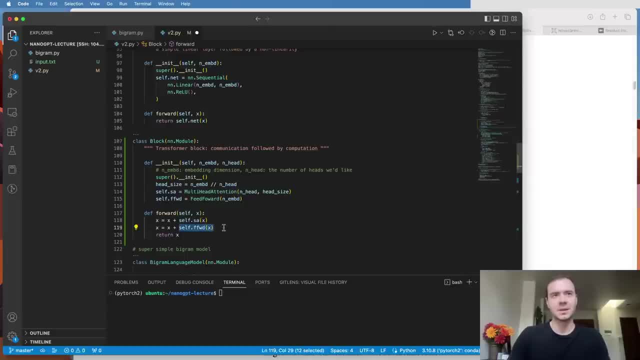 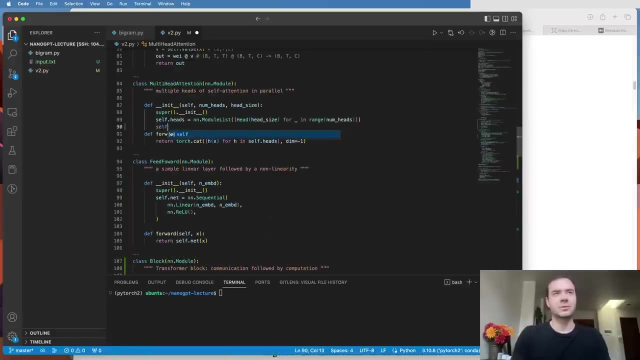 Self-attention, and x equals x plus selffeedforward. So this is x, And then we fork off and do some communication and come back. And we fork off and we do some computation and come back. So those are residual connections. And then, swinging back up here, we also have to introduce this projection. 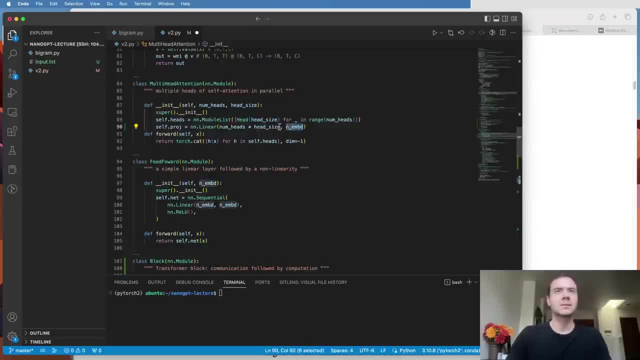 So nnlinear, And this is going to be from after we concatenate this. This is the size and embed. So this is the output of the self-attention. It's self, But then we actually want to apply the projection And that's the result. 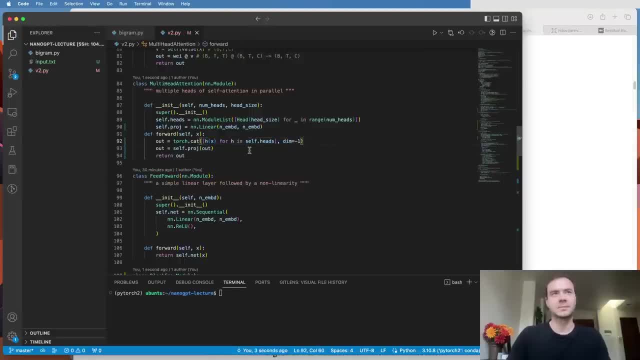 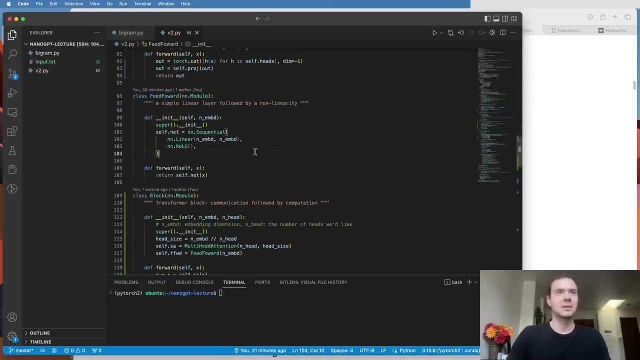 So the projection is just a linear transformation of the outcome of this layer. So that's the projection back into the residual pathway And then here in the feedforward it's going to be the same thing. I could have a selfprojection here as well. 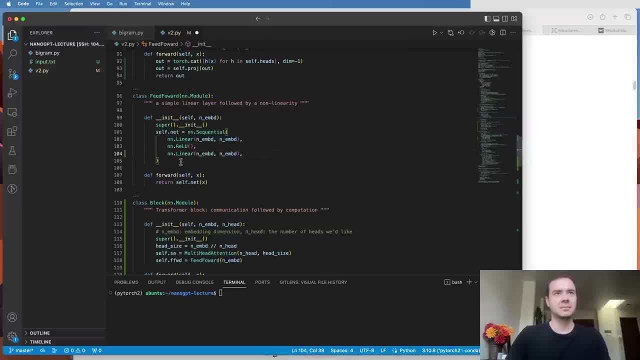 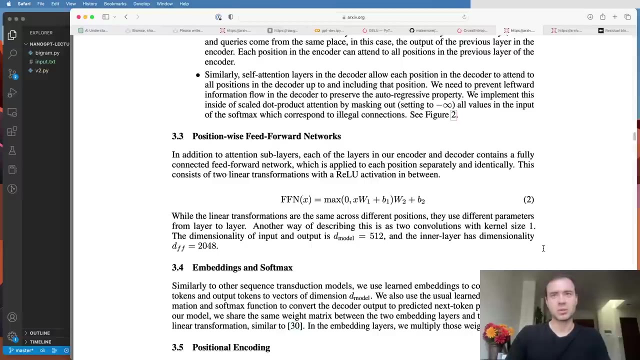 But let me just simplify it And let me couple it inside the same sequential container, And so this is the projection layer, And this is going back into the residual pathway, And so that's it. So now we can train this. So I implemented one more small change. 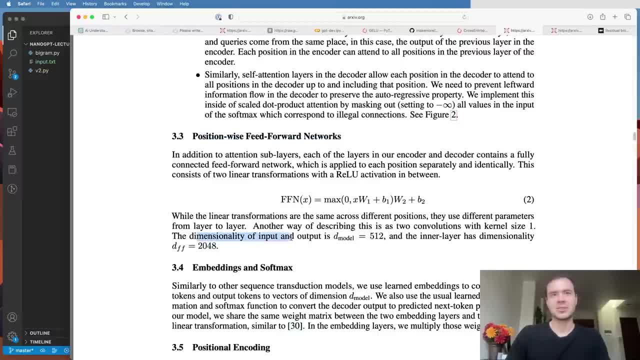 When you look into the paper again, you see that the dimensionality of input and output is 512 for them And they're saying that the inner layer here in the feedforward has dimensionality of 2048.. So there's a multiplier of 4.. 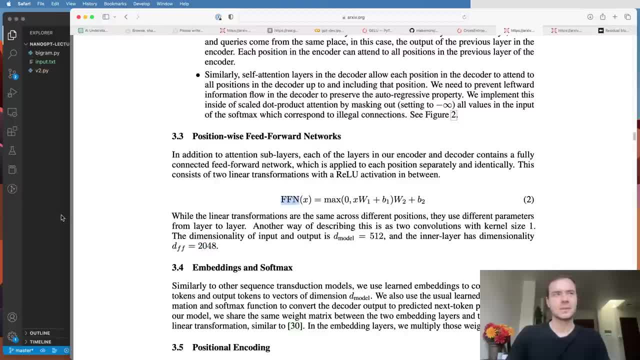 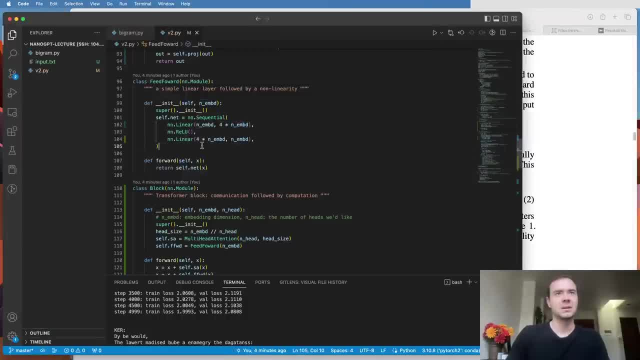 And so the inner layer of the feedforward network should be multiplied by 4 in terms of channel sizes. So I came here And I multiplied 4 times embed here for the feedforward, And then from 4 times unembed, coming back down to unembed when we go back to the projection. 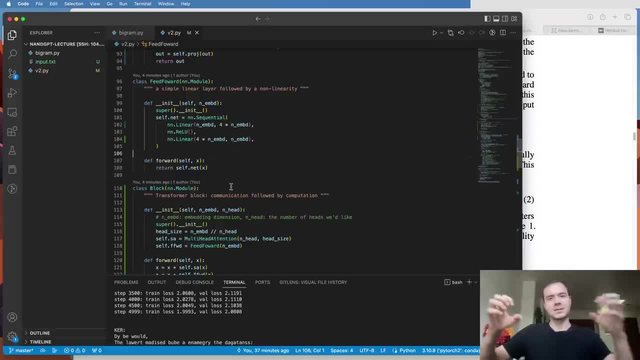 So adding a bit of computation here and growing that layer that is in the residual block on the side of the residual pathway. And then I train this And we actually get down all the way to 2.08 validation loss. And we also see that the network is starting to get big enough that our train loss is getting ahead of validation loss. 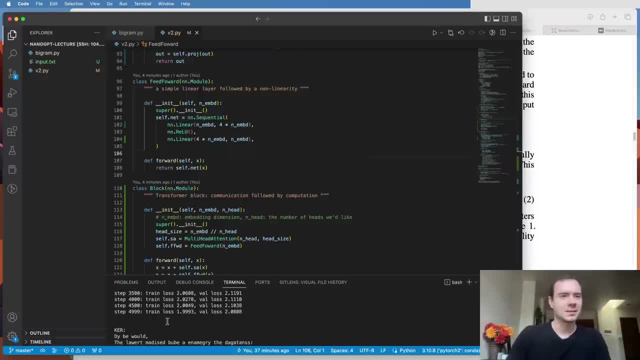 So we start to see like a little bit of overfitting And our generations here are still not amazing, But at least you see that we can see like is here this? now grief sink Like this starts to almost look like English. 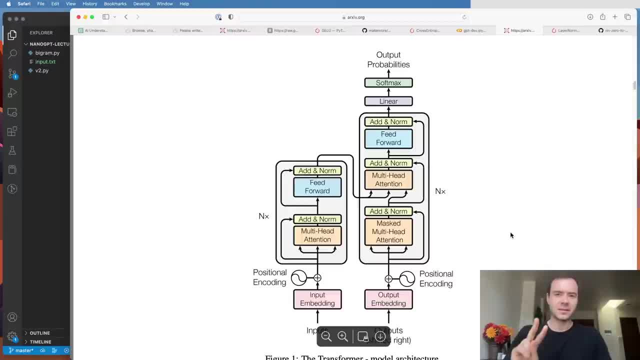 So, yeah, we're starting to really get there. OK, and the second innovation that is very helpful for optimizing very deep neural networks is right here. So we have this addition now. That's the residual part, But this norm is referring to something called layer norm. 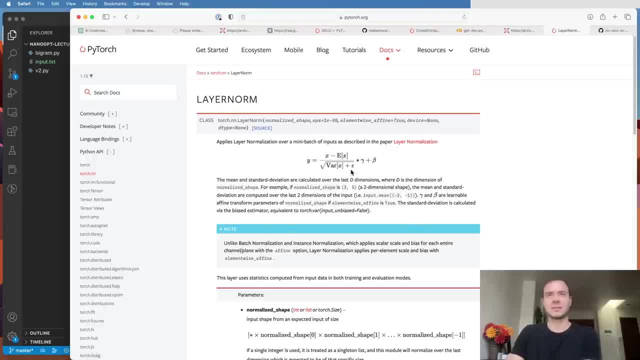 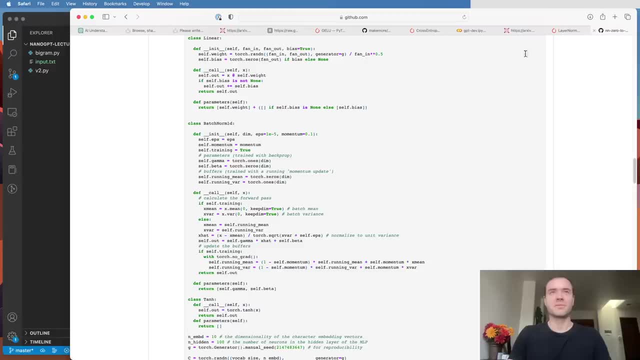 So layer norm is implemented in PyTorch. It's a paper that came out A while back here, And layer norm is very, very similar to bash norm. So remember back to our make more series, part three: We implemented bash normalization. 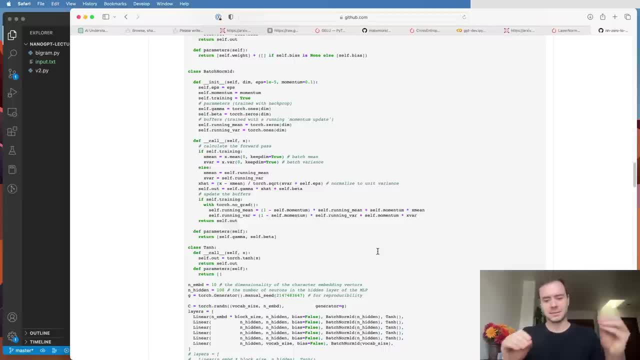 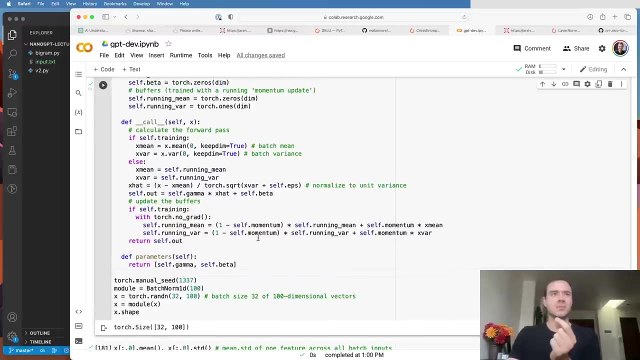 And bash normalization basically just made sure that across the bash dimension any individual neuron had unit Gaussian distribution. So it was zero mean and unit standard deviation, one standard deviation output. So what I did here is I'm copy pasting the bash norm 1D that we developed in our make more series. 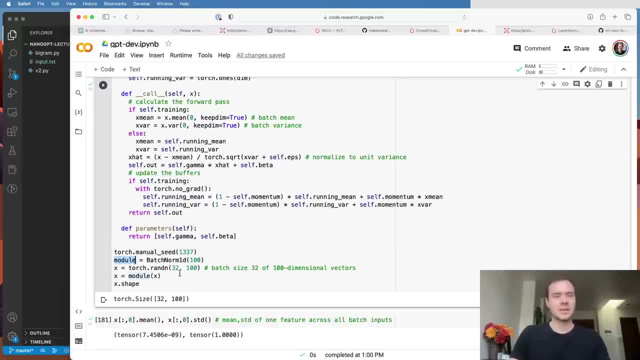 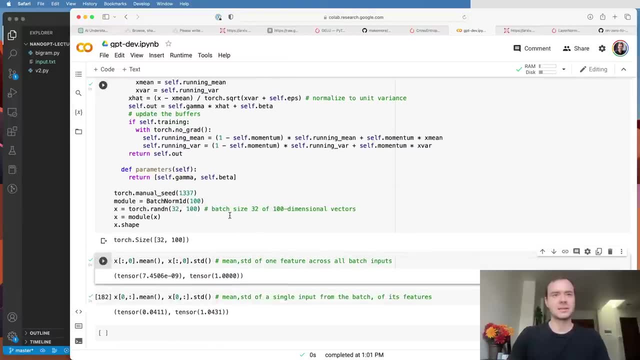 And see, here we can initialize, for example, this module and we can have a batch of 32, 100 dimensional vectors feeding through the bash norm layer. So what this does is it guarantees that, when we look at just the zeroth column, 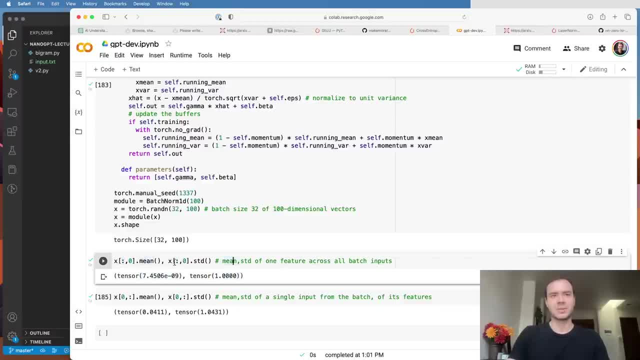 it's a zero mean, one standard deviation. So it's normalizing every single column of this input. Now the rows are not going to be normalized by default, because we're just normalizing columns. So let's not implement layer norm. It's very complicated. 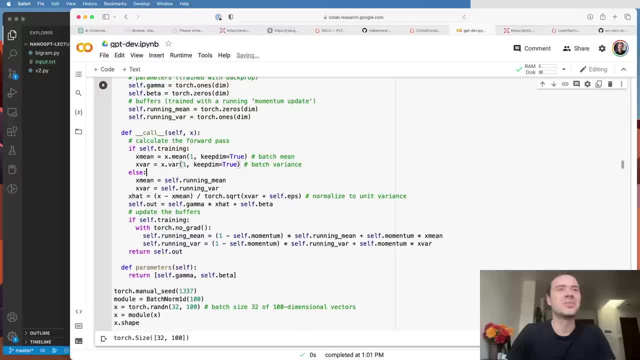 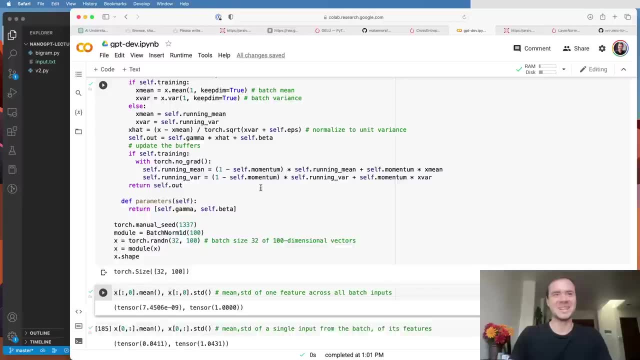 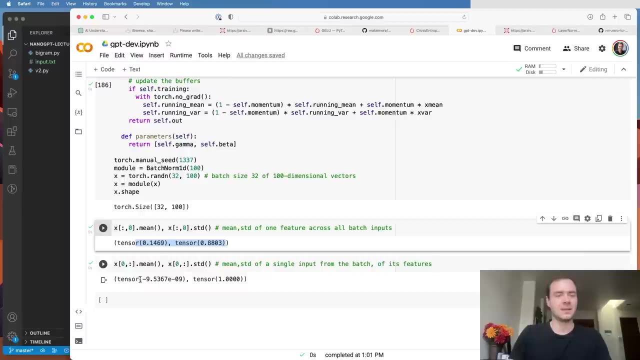 Look, we come here. We change this from zero to one. So we don't normalize the columns, We normalize the rows. And now we've implemented layer norm. So now the columns are not going to be normalized, but the rows are going to be normalized for every individual example. 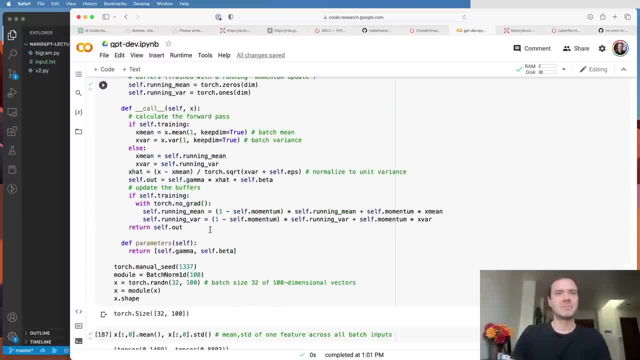 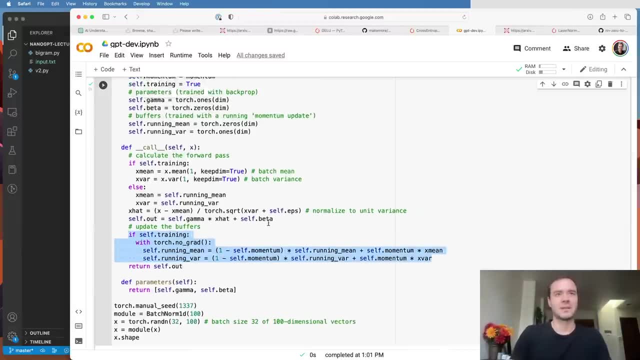 It's 100 dimensional vector is normalized In this way And because our computation now does not span across examples, we can delete all of this buffer stuff because we can always apply this operation and don't need to maintain any running buffers. So we don't need the buffers. 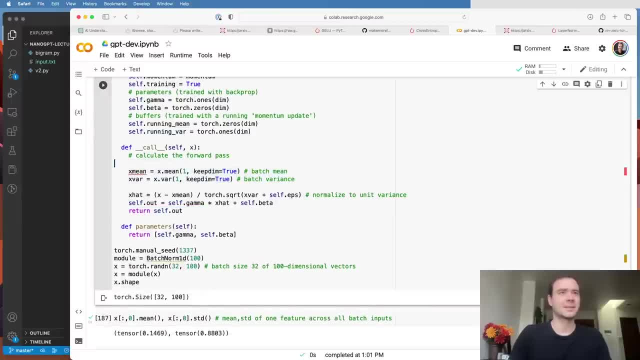 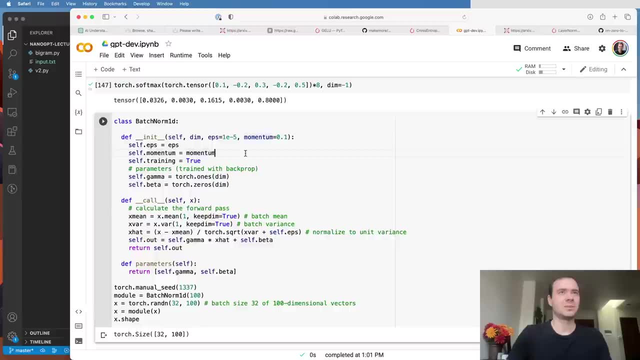 We don't. There's no distinction between training and test time And we don't need these running buffers. We do keep gamma and beta. We don't need the momentum, We don't care if it's training or not, And this is now a layer norm. 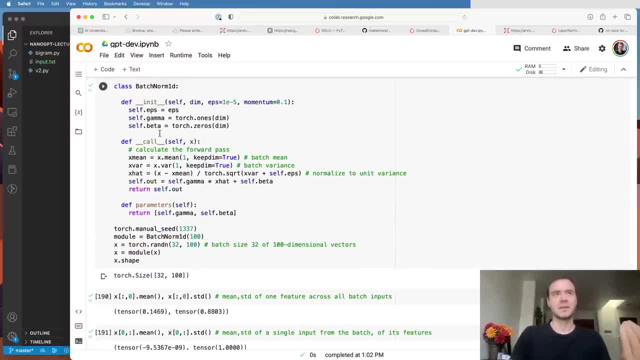 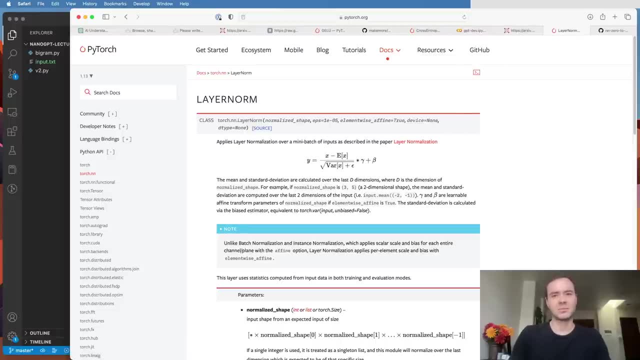 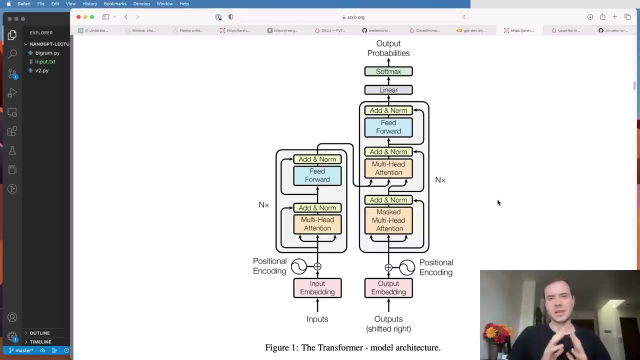 and it normalizes the rows instead of the columns, And this here is identical to basically this here. So let's now implement layer norm in our transformer. Before I incorporate the layer norm, I just wanted to note that, as I said, very few details about the transformer have changed in the last five years. 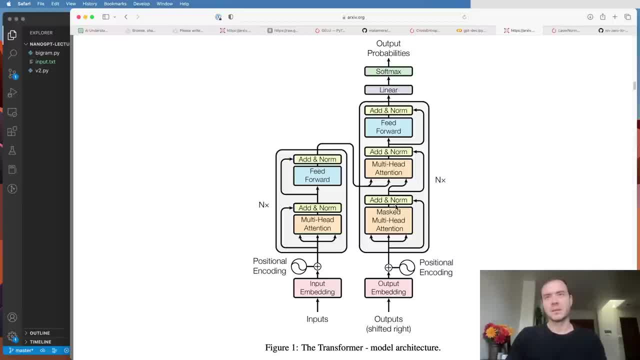 But this is actually something that's likely departs from the original paper. You see that the add and norm is applied after the transformation, but now it is a bit more basically common to apply the layer norm before the transformation. So there's a reshuffling of the layer norms. 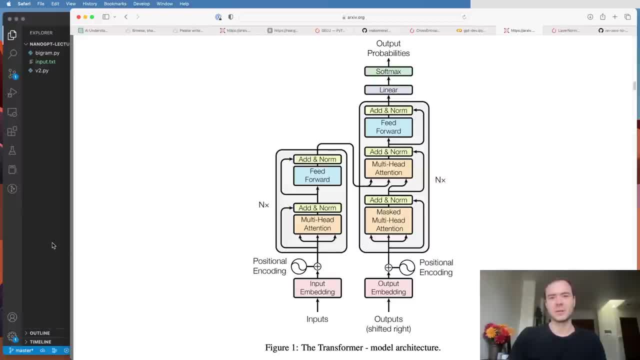 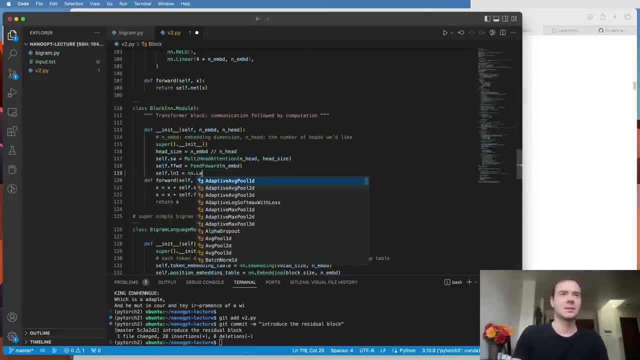 So this is called the pre-norm formulation And that's the one that we're going to implement as well. So slight deviation from the original paper. Basically, we need two layer norms. Layer norm one is an n dot layer norm And we tell it how many. what is the embedding dimension? 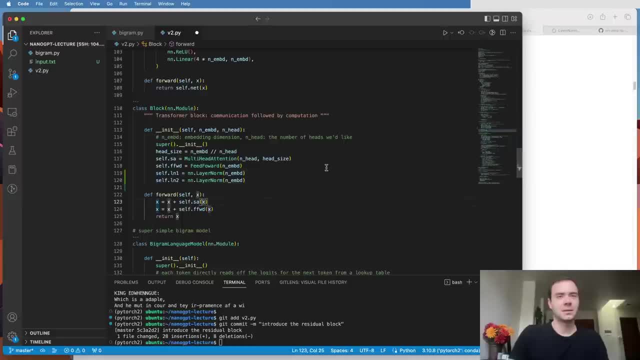 And we need the second layer norm. And then here the layer norms are applied immediately on X. So self dot layer norm one applied on X and self dot layer norm two applied on X before it goes into self-attention and feedforward. And the size of the layer norm here is an embed, so 32.. 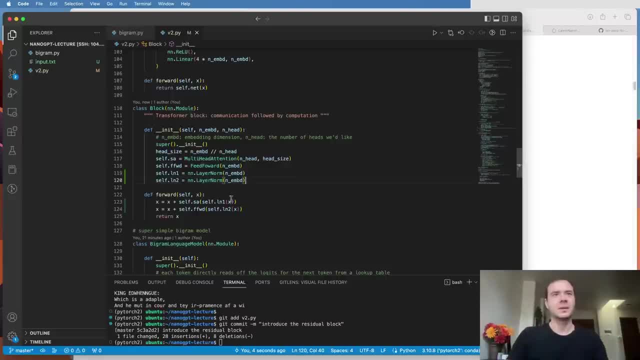 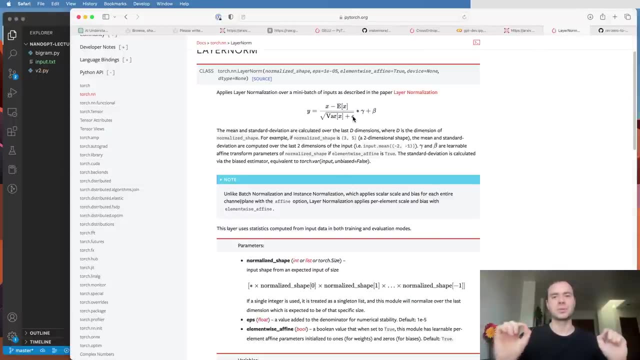 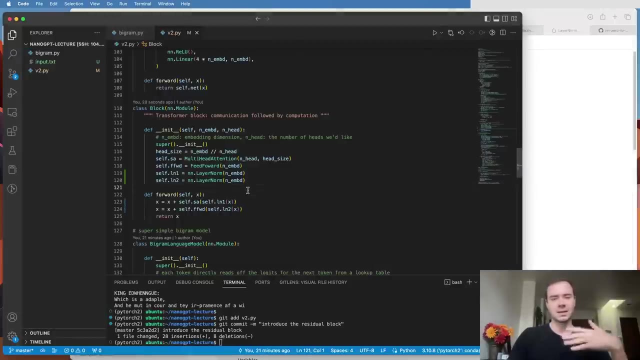 So when the layer norm is normalizing our features, it is the normalization here happens. the mean and the variance are taken over 32 numbers. So the batch and the time act as batch dimensions both of them. So this is kind of like a per token. 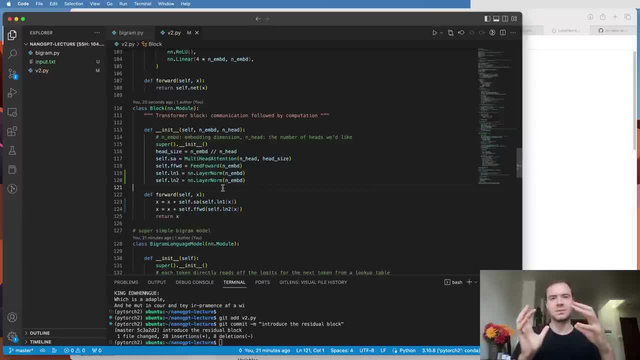 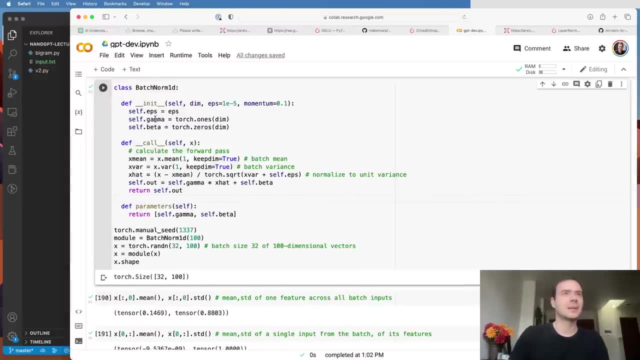 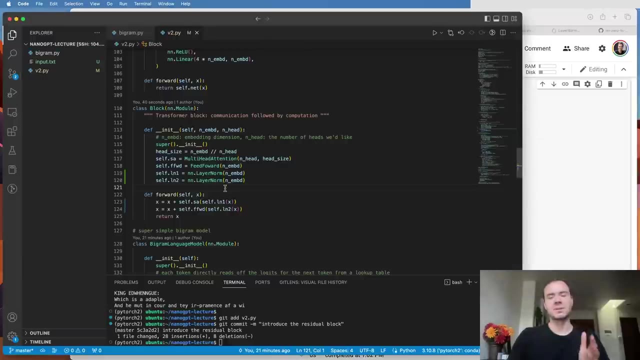 transformation that just normalizes the features and makes them unit mean unit Gaussian at initialization. But of course, because these layer norms inside it have these gamma and beta trainable parameters, the layer norm will eventually create outputs that might not be unit Gaussian, But the optimization will determine that. 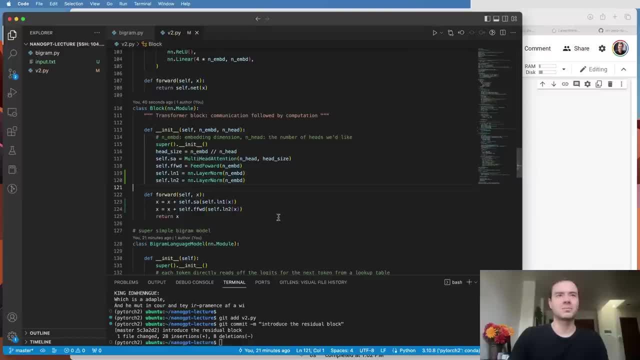 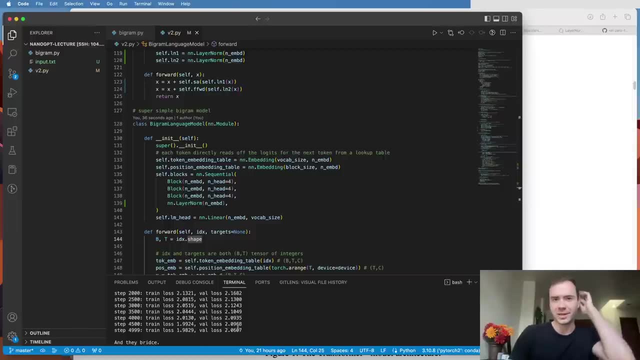 So for now, this is incorporating the layer norms and let's train them up. Okay, so I let it run and we see that we get down to 2.06, which is better than the previous 2.08, so a slight improvement by adding the layer. 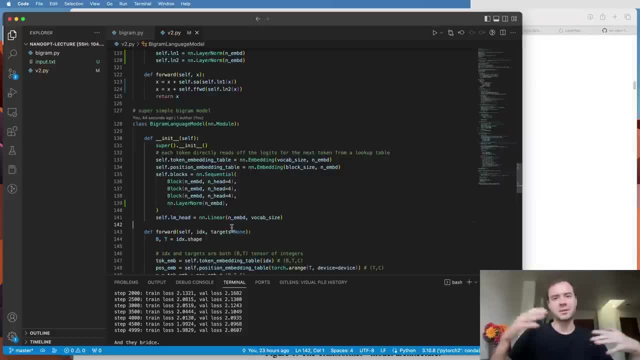 norms, and I'd expect that they help even more if we had bigger and deeper network. One more thing I forgot to add is that there should be a layer norm here also, typically as at the end of the transformer and right before the final linear layer. 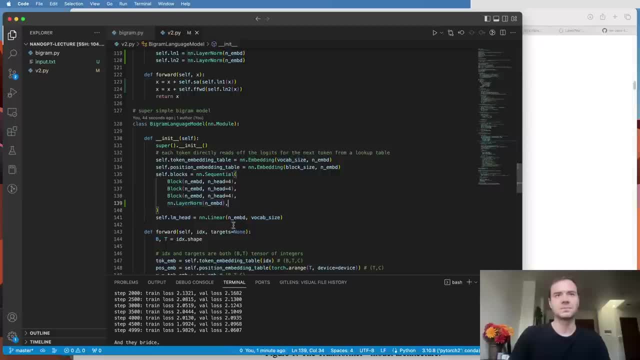 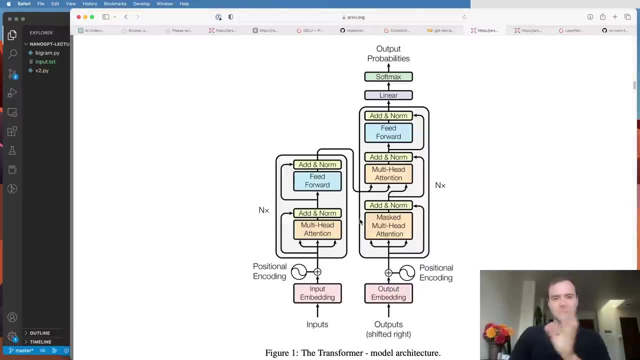 that decodes into vocabulary. So I add that. I added that as well. So at this stage we actually have a pretty complete transformer, according to the original paper, And it's a decoder-only transformer. I'll talk about that in a second. 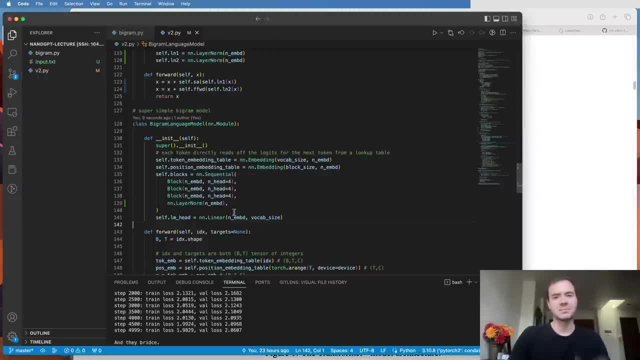 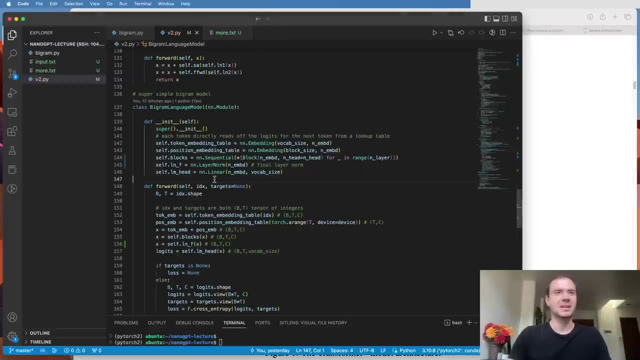 But at this stage the major pieces are in place, So we can try to scale this up and see how well we can push this number. Now, in order to scale up the model, I had to perform some cosmetic changes here to make it nicer. 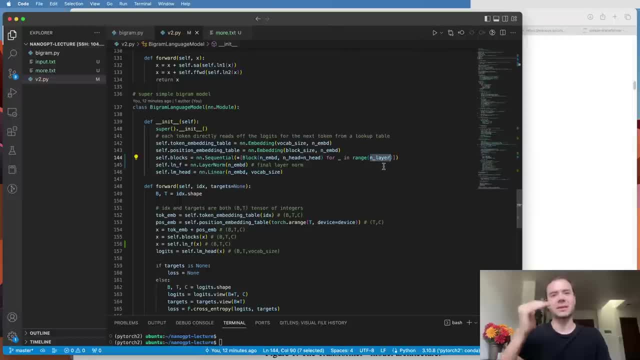 So I introduced this variable called nlayer, which just specifies how many layers of the blocks we're going to have. I create a bunch of blocks, and we have a new variable number of heads as well. I pulled out the layer norm here, And so this is identical. 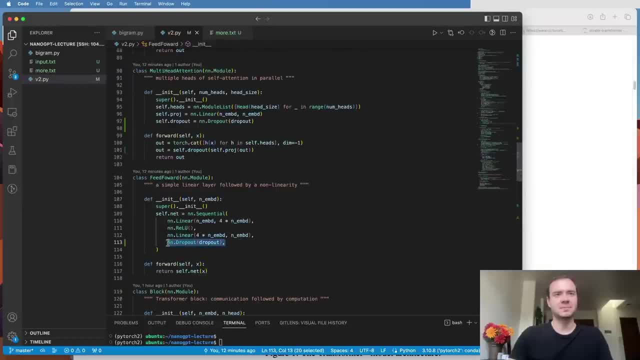 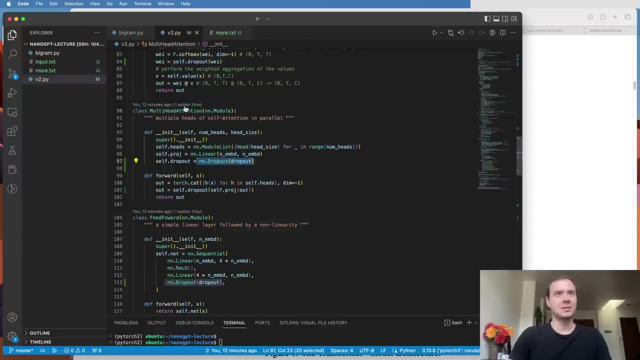 Now, one thing that I did briefly change is I added a dropout. So dropout is something that you can add right before the residual connection back into the residual pathway. So we can drop out that as the last layer here. We can drop out here at the end of the multi-headed extension as well. 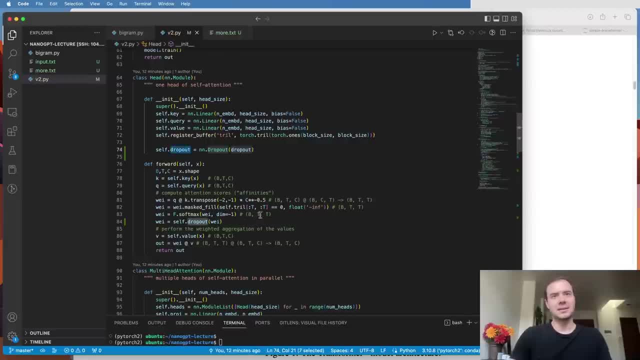 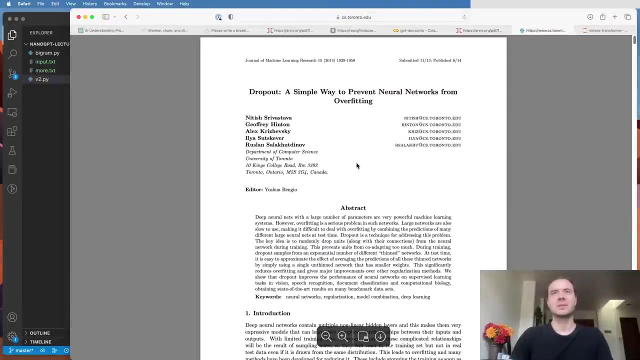 And we can also drop out here. when we calculate the basically affinities and after the softmax we can drop out some of those so we can randomly prevent some of the nodes from communicating And so dropout comes from this paper from 2014 or so. 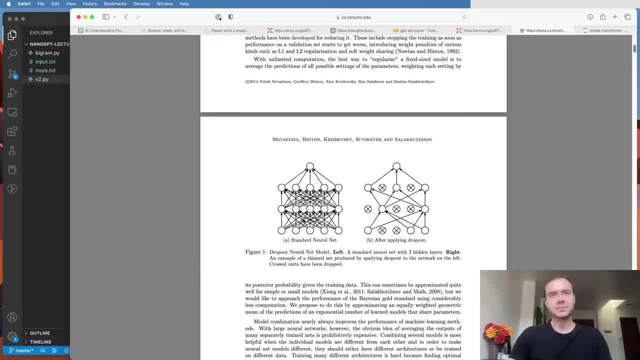 And basically it takes your neural net and it randomly, every forward, backward pass, shuts off some subset of neurons, So randomly drops them to zero and trains without them. And what this does effectively is because the mask of what's being dropped out has changed every single forward. 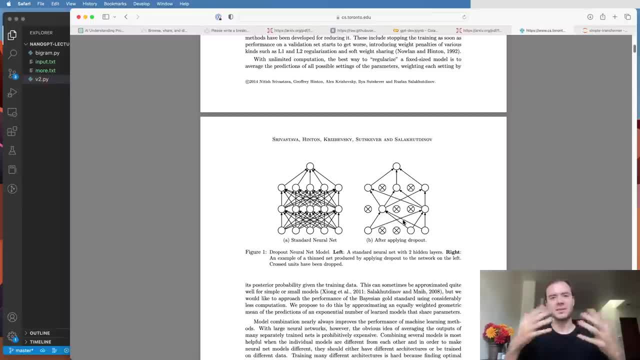 backward pass. it ends up kind of training an ensemble of sub networks And then at test time everything is fully enabled And kind of all of those sub networks are merged into a single ensemble, If you want to think about it that way. 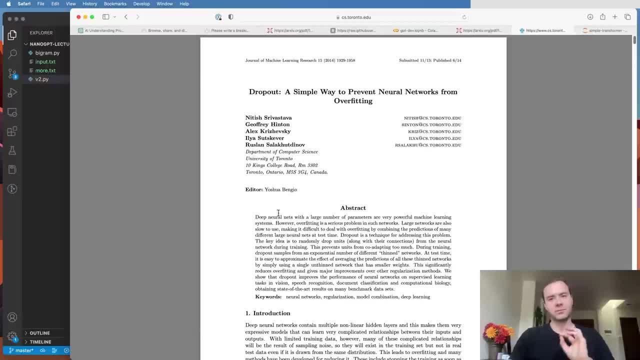 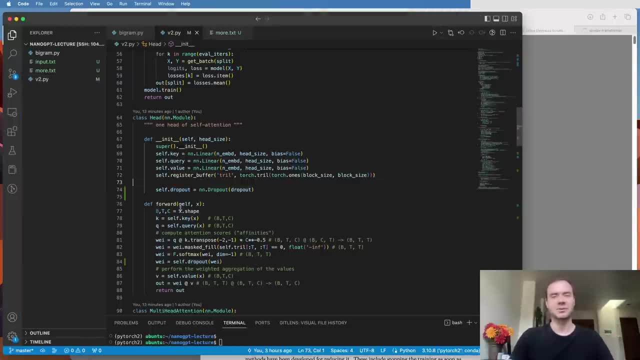 So I would read the paper to get the full detail. For now we're just going to stay on the level of. this is a regularization technique, and I added it because I'm about to scale up the model quite a bit And I was concerned about overfitting. 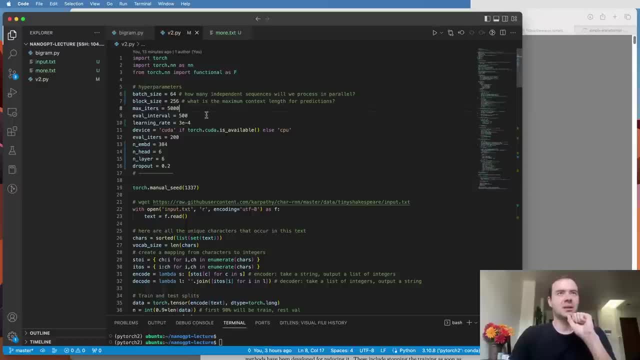 So now when we scroll up to the top, we'll see that I changed a number of hyperparameters here about our neural net, So I made the batch size be much larger. Now it's 64.. I changed the block size to be 256. 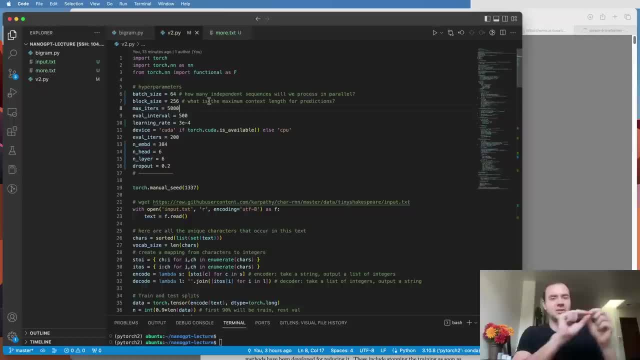 So previously it was just eight, eight characters of context. Now it is 256 characters of context to predict the 257th. I brought down the learning rate a little bit because the neural net is now much bigger. So I brought down the learning rate. 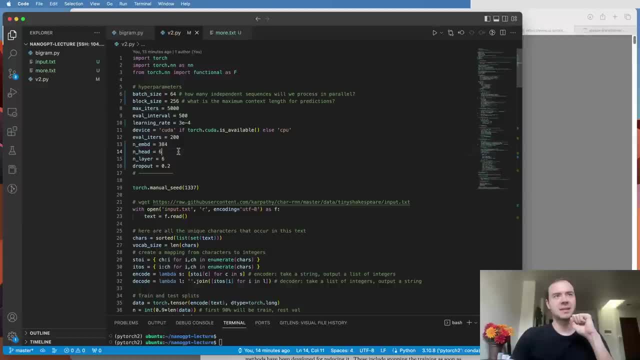 The embedding dimension is now 384.. And there are six heads. So 384 divided by six means that every head is 64 dimensional as a standard, And then there are going to be six layers of that And the dropout will be a point two. 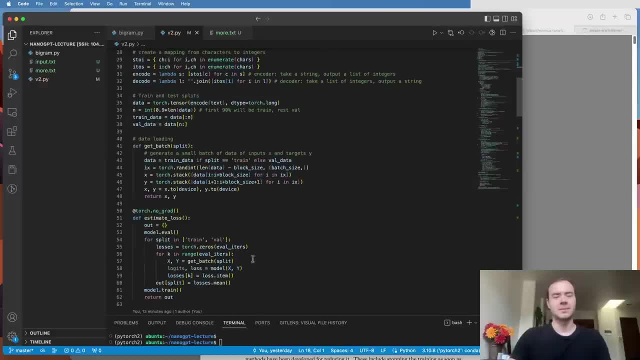 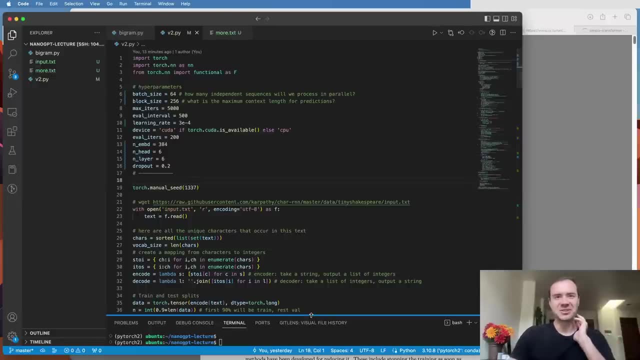 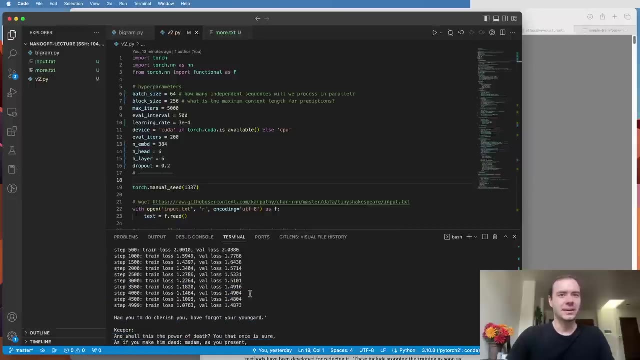 So every forward, backward pass, 20 percent of all of these intermediate calculations are disabled and dropped to zero. And then I already trained this and I ran it, So drum roll, how does it perform? So let me just scroll up here. We get a validation loss of 1.48, which is actually quite a bit of an. 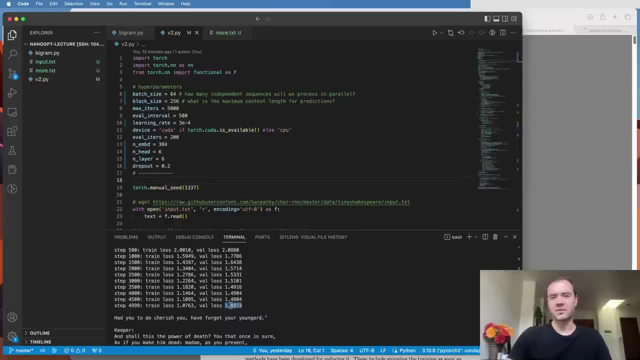 improvement on what we had before, which I think was 2.07.. So we went from 2.07 all the way down to 1.48, just by scaling up this neural net with the code that we have, And this, of course, ran for a lot longer. 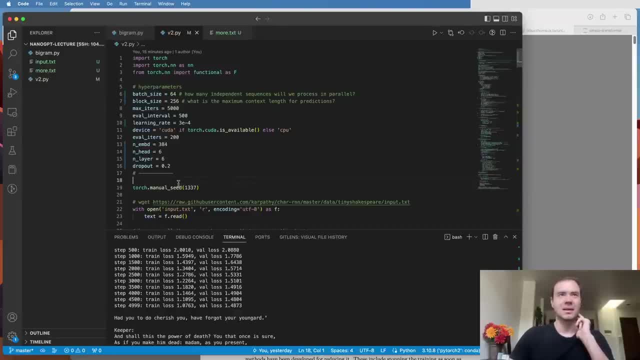 This may be trained for. I want to say about 15 minutes on my A100 GPU, So that's a pretty good GPU, And if you don't have a GPU, you're not going to be able to reproduce this On a CPU. this would be. I would not run this on a CPU or a MacBook. 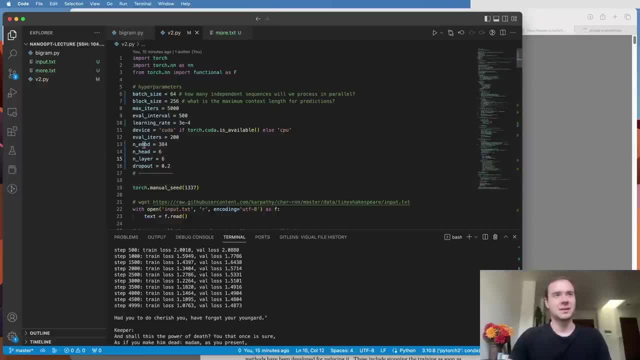 or something like that. You'll have to break down the number of layers and the embedding dimension and so on, But in about 15 minutes we can get this kind of a result. And I'm printing some of the Shakespeare here, But what I did also is I printed 10,000 characters, so a lot more. 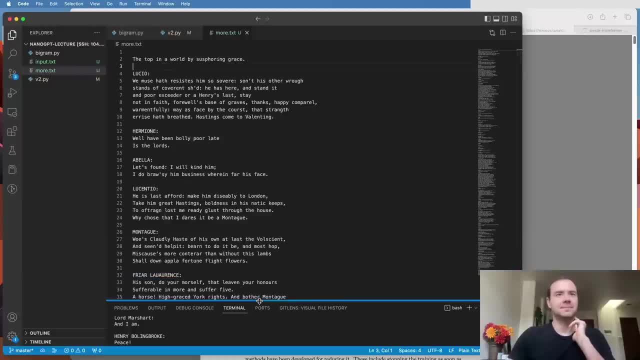 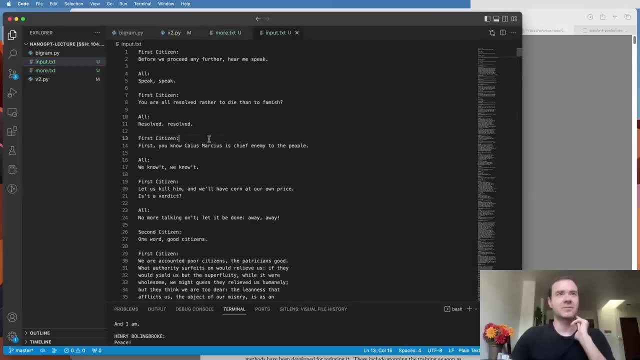 And I wrote them to a file And so here we see some of the outputs. So it's a lot more recognizable as the input text file. So the input text file, just for reference, looked like this. So there's always like someone speaking in this manner. 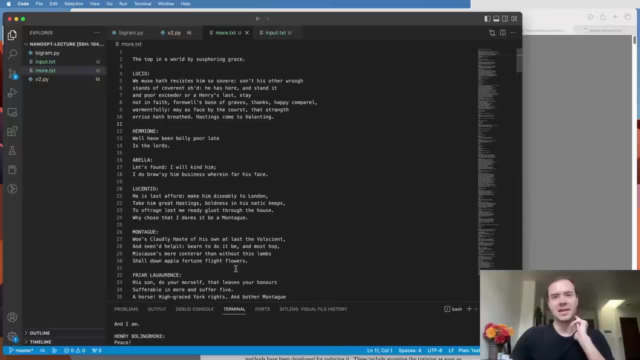 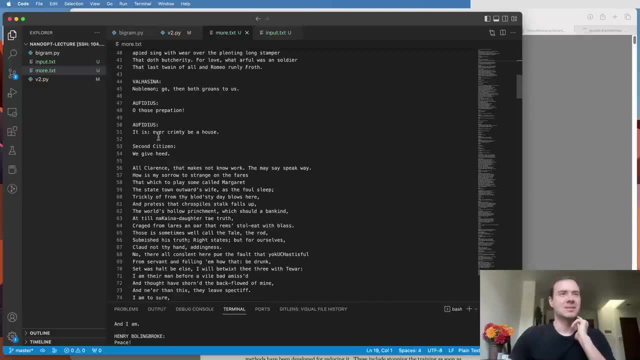 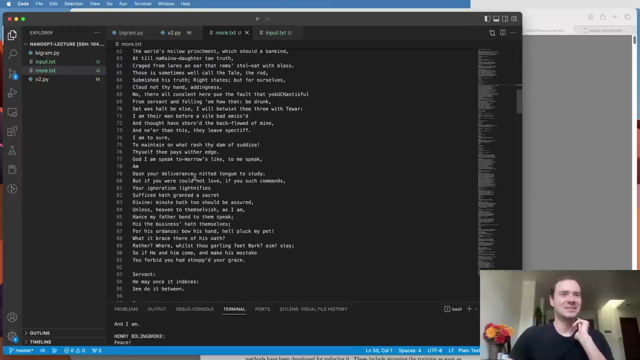 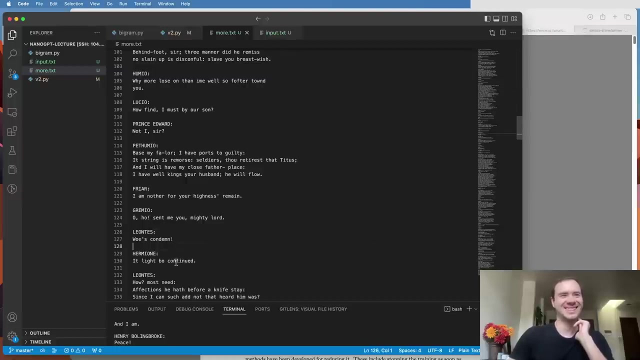 And our predictions now take on that form, Except, of course, they're nonsensical when you actually read them. So That is, every crimpty be a house. Oh, those prepation We give heed, You know, Oho, sent me you mighty lord. 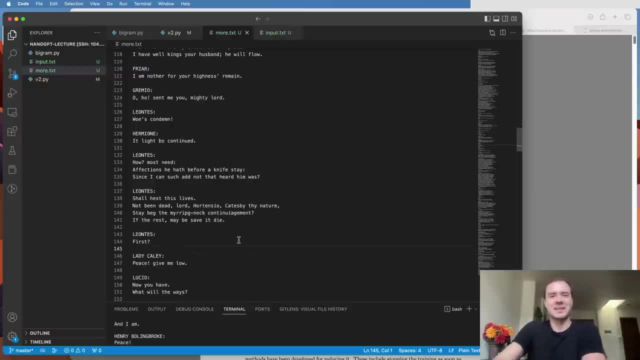 Anyway, so you can read through this. It's nonsensical, of course, but this is just a transformer, trained on the character level, for one million characters that come from Shakespeare, So there's sort of like blabbers on in Shakespeare, like manner. 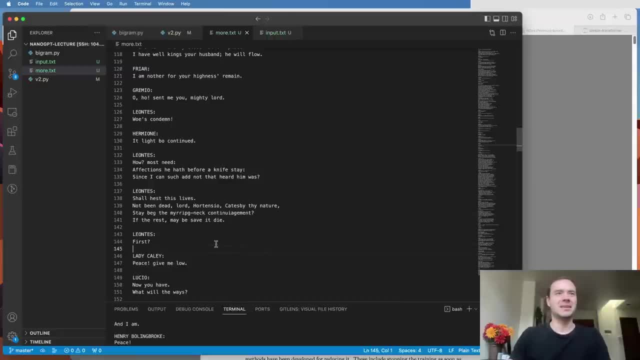 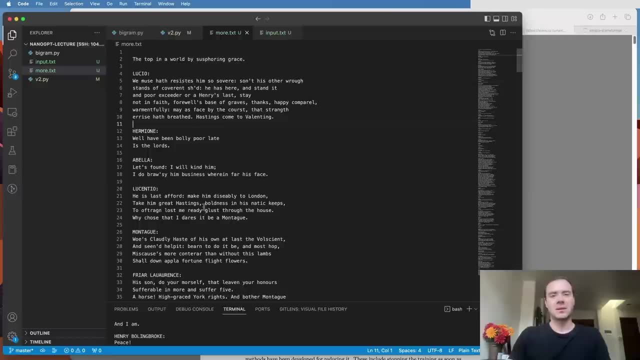 But it doesn't of course make sense at this scale, But I think I think still a pretty good demonstration of what's possible. So now, I think that kind of concludes the programming section of this video. We basically kind of did a pretty good job. 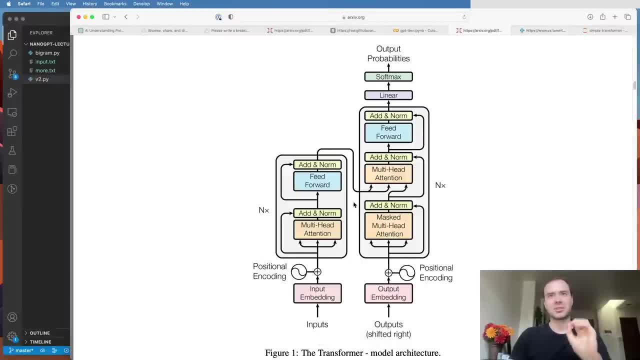 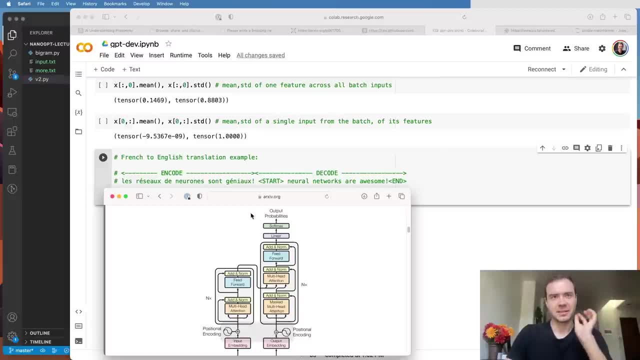 And of implementing this transformer, But the picture doesn't exactly match up to what we've done. So what's going on with all these additional parts here? So let me finish explaining this architecture and why it looks so funky. Basically, what's happening here is what we implemented here is a decoder, only transformer. 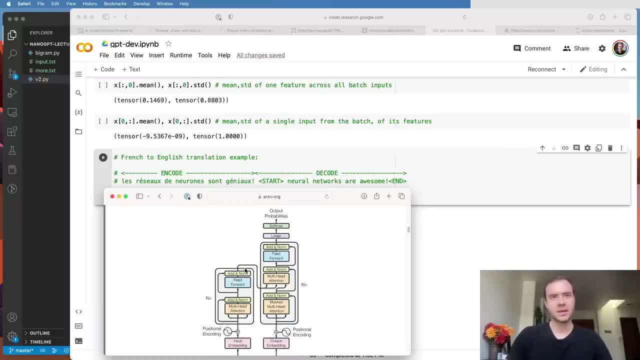 So there's no component here. This part is called the encoder, and there's no cross attention block here. Our block only has a self attention and the feed forward. So it is missing this third in between This piece here. this piece does cross attention. 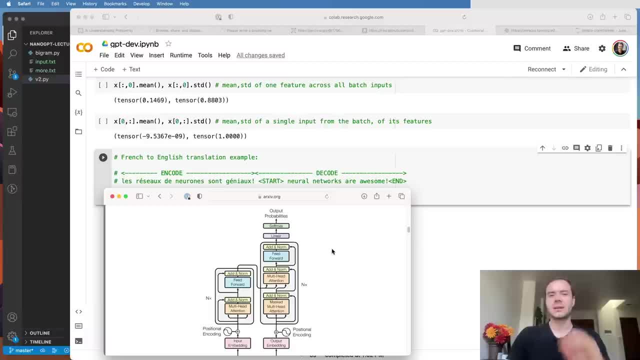 So we don't have it and we don't have the encoder, We just have the decoder. And the reason we have a decoder only is because we are just generating text and it's unconditioned on anything. We're just, we're just blabbering on according to a given dataset. 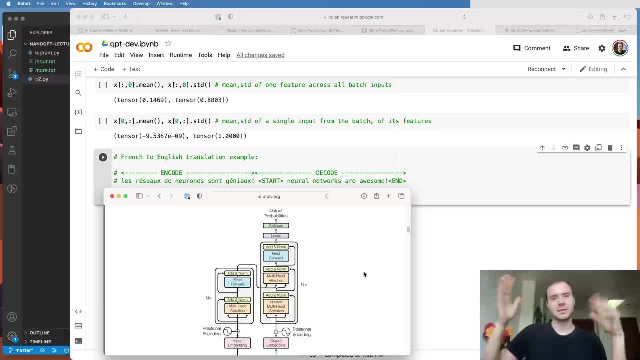 What makes it a decoder is that we are using the triangular mask in our transformer, So it has this autoregressive property where we can just go and sample from it. So the fact that it's using the triangular mask to mask out the attention makes it a decoder and it can be used for language modeling. 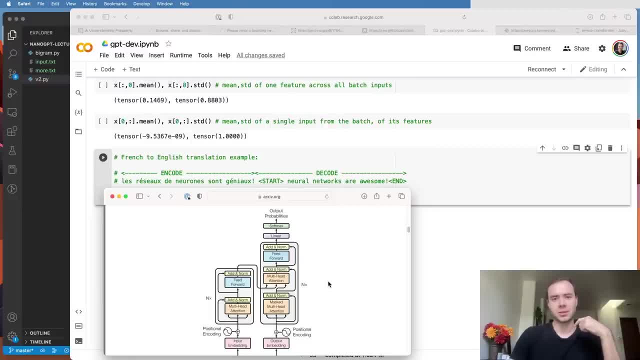 Now, the reason that the original paper had an encoder decoder architecture is because it is a machine translation paper, So it is concerned with a different setting. In particular, it expects some tokens that encode, say for example French, And then it is expected to decode the translation in English. 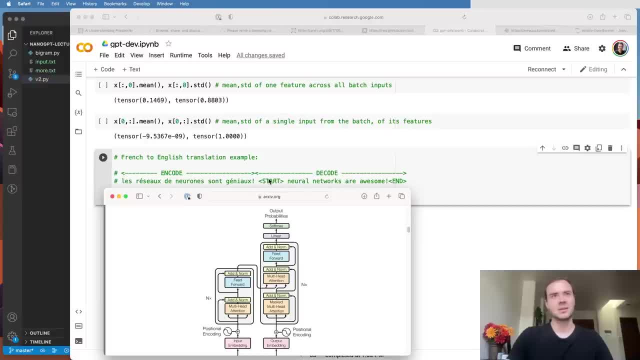 So so you typically these here are special tokens, So you are expected to read in this and condition on it, and then you start off the generation with a special token called start. So this is a special new token that you introduce and always place in the beginning. 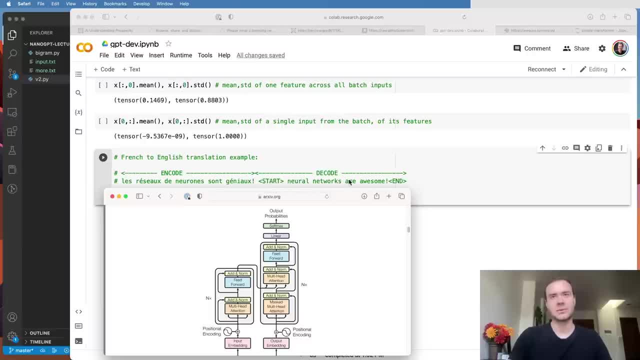 And then the network is expected to output neural networks are awesome, and then a special end token to finish the generation. So this part here will be decoded exactly as we. we've done it. Neural networks are awesome- will be identical to what we did. 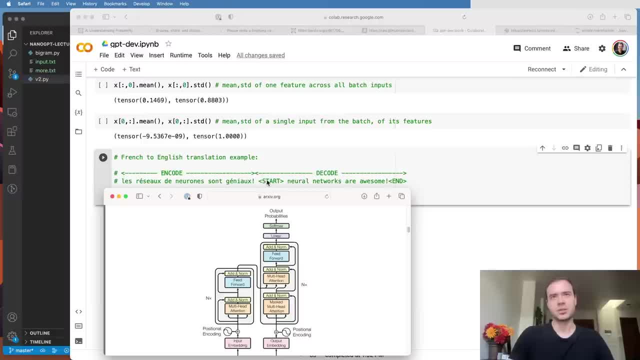 But, unlike what we did, they want to condition The generation on some additional information, And in that case, this additional information is the French sentence that they should be translating. So what they do now is they bring the encoder Now. the encoder reads this part here: 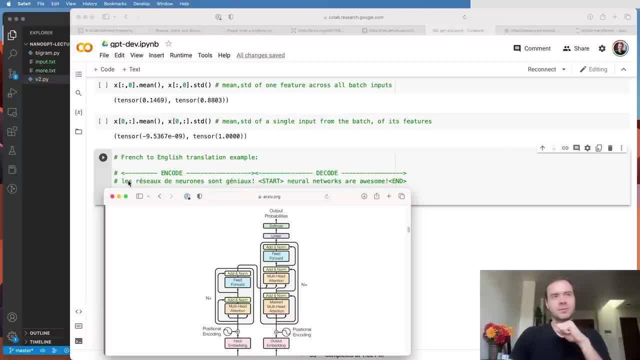 So we're only going to take the part of French and we're going to create tokens from it, exactly as we've seen in our video, And we're going to put a transformer on it, But there's going to be no triangular mask, And so all the tokens are allowed to talk to each other as much as. 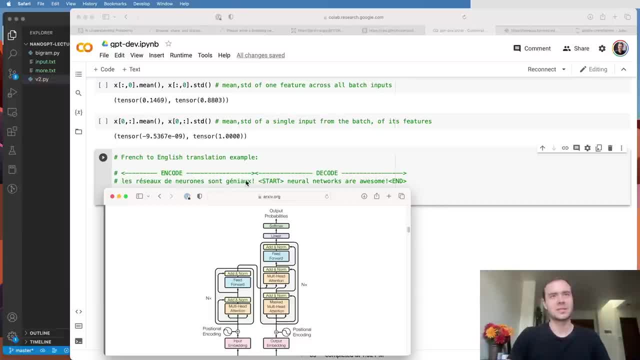 they want and they're just encoding whatever the content of this French sentence. Once they've encoded it, they they basically come out in the top here, And then what happens here is in our decoder, which does the language modeling. there's an additional connection here to the outputs of the encoder. 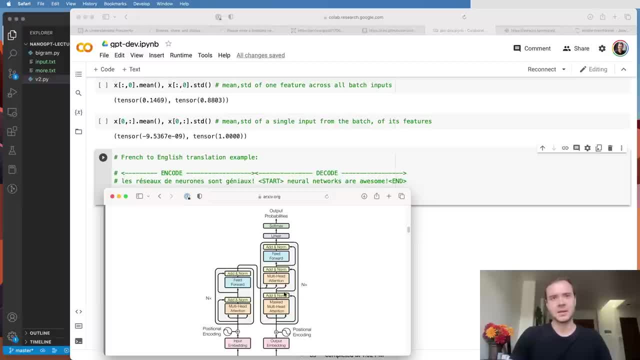 And that is brought in through cross attention. So the queries are still generated from X, but now the keys and the values are coming from the side. The keys and the values are coming from the top, generated by the nodes that came outside of the encoder. 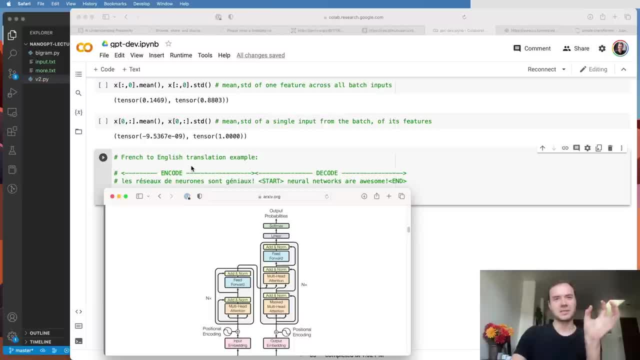 And those tops, the keys and the values there, the top of it, feed in on a side into every single block of the decoder, And so that's why there's an additional cross attention. And really what it's doing is it's conditioning the decoding. 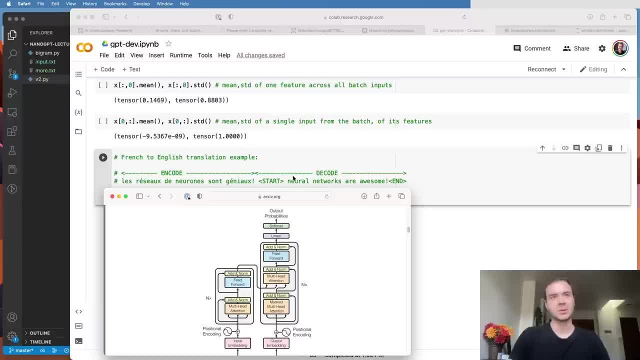 not just on the past of this current decoding, but also on having seen the full, fully encoded French prompt sort of. And so it's an encoder, decoder model, which is why we have those two transformers and an additional block and so on. 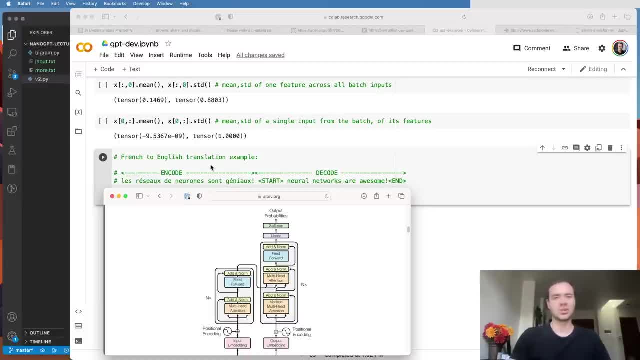 So we did not do this because we have- no, we have nothing to encode, There's no conditioning. We just have a text file and we just want to imitate it, And that's why we are using a decoder, only transformer, exactly as done in GPT. 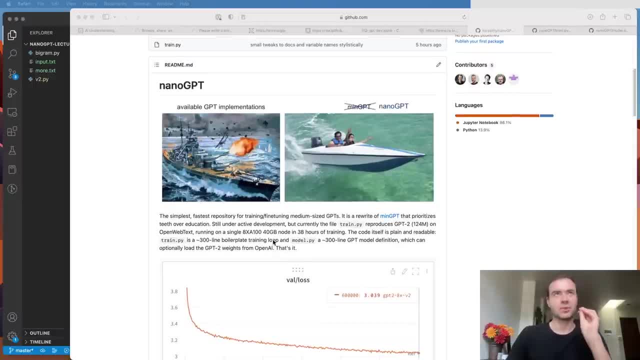 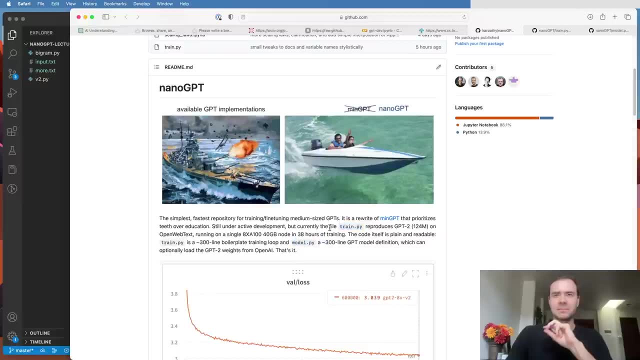 OK, so now I wanted to do a very brief walkthrough of NanoGPT, which you can find on my GitHub. And NanoGPT is basically two files of interest. There's trainpy and modelpy. Trainpy is all the boilerplate code for training the network. 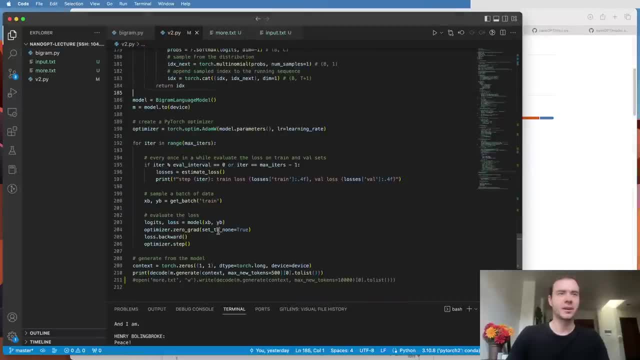 It is basically all the stuff that we had here is the training loop. It's just that it's a lot more complicated because we are saving and loading checkpoints and pre-trained weights and we are decaying the learning rate and compiling the model and using distributed training across multiple nodes or GPUs. 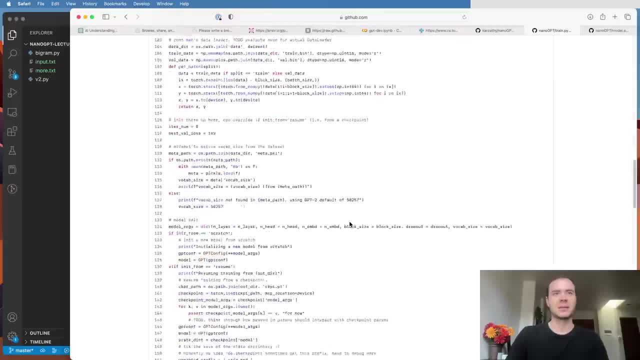 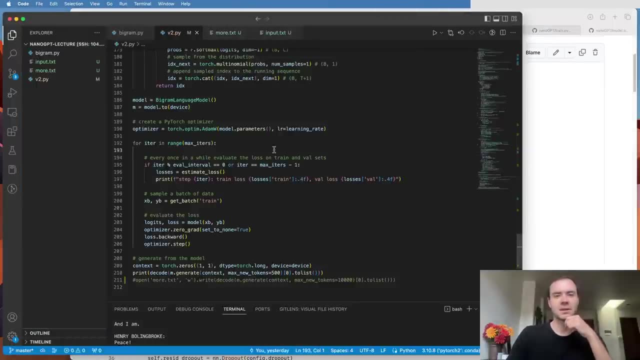 So the trainingpy gets a little bit more hairy, complicated, There's more options, et cetera, But the modelpy should look very, very, very similar to what we've done here. In fact, the model is almost identical. 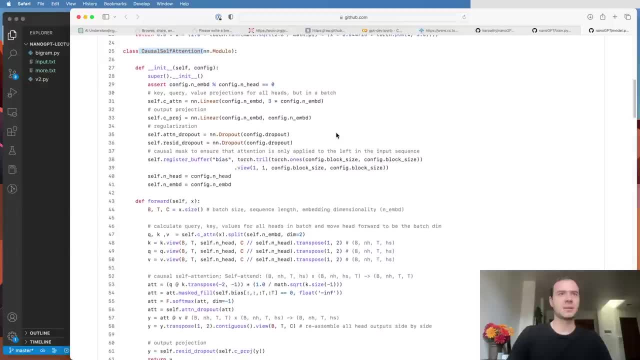 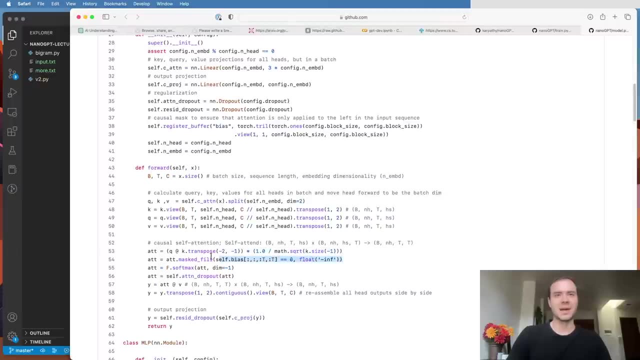 So first, here we have the causal self-attention block, And all of this should look very, very recognizable to you. We're producing queries, keys, values. We're doing dot products, We're masking, applying softmax, optionally dropping out. 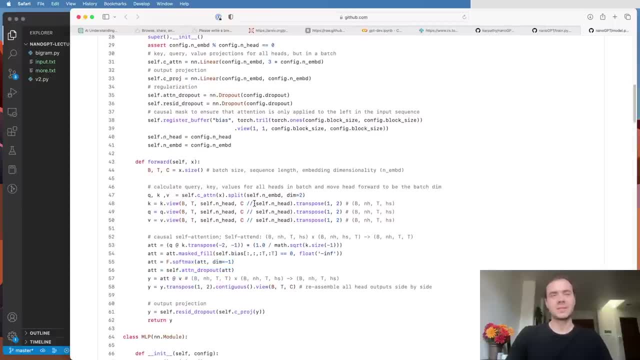 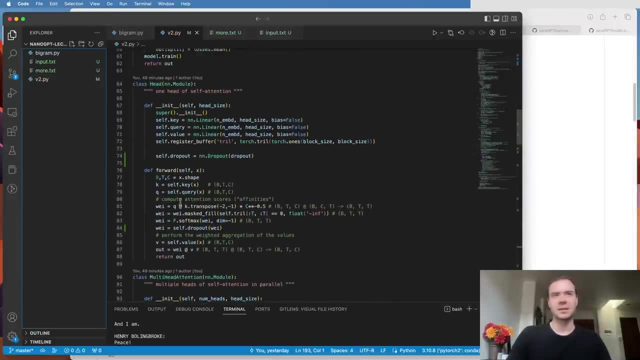 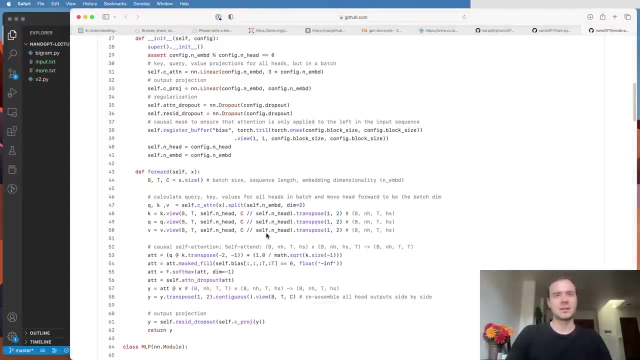 And here we are pooling the values. What is different here is that in our code I have separated out the multi-headed attention into a single individual head, and then here I have multiple heads and I explicitly concatenate them, whereas here all of it is implemented. 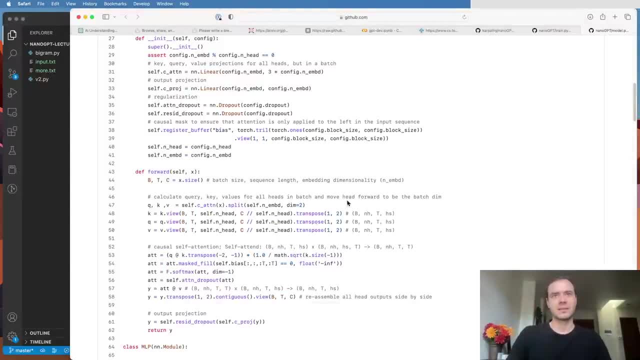 in a batched manner inside a single causal self-attention, And so we don't just have a B and a T and a C dimension, We also end up with a fourth dimension, which is the heads, And so it just gets a lot more sort. 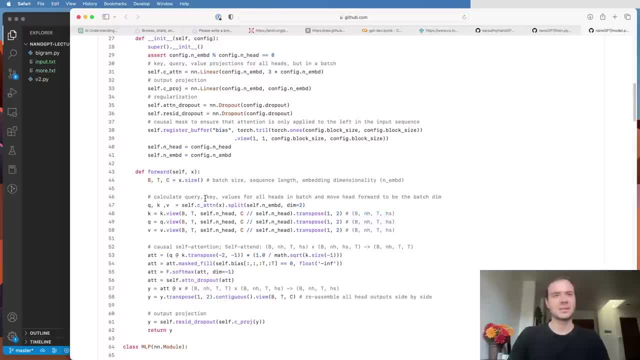 of hairy because we have four-dimensional array tensors now, But it is equivalent mathematically, So the exact same thing is happening as what we have. It's a bit more efficient because all the heads are now treated as a batch dimension as well. 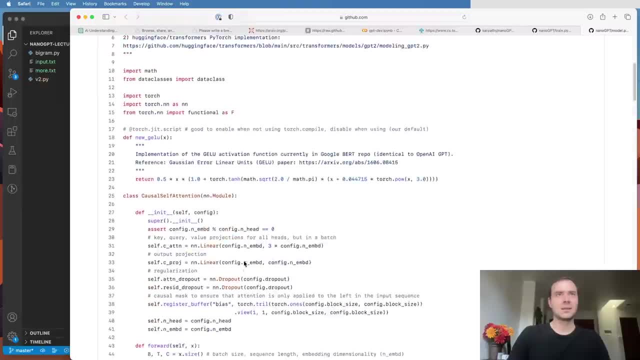 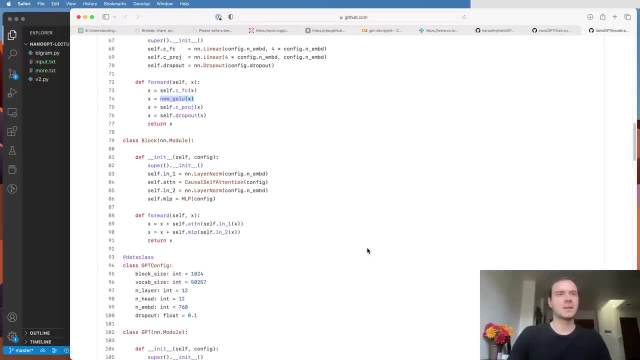 Then we have the multi-layered perceptron. It's using the GELU non-linearity, which is defined here, instead of RELU, And this is done just because OpenAI used it And I want to be able to load their checkpoints. 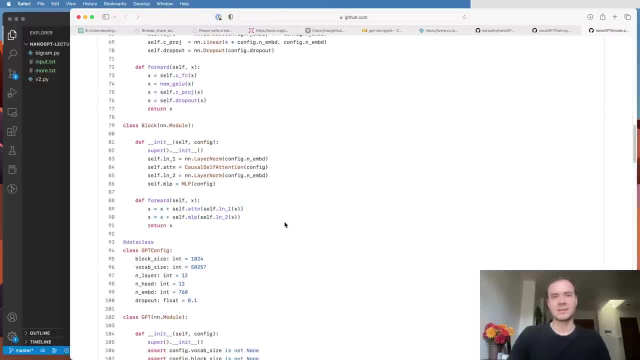 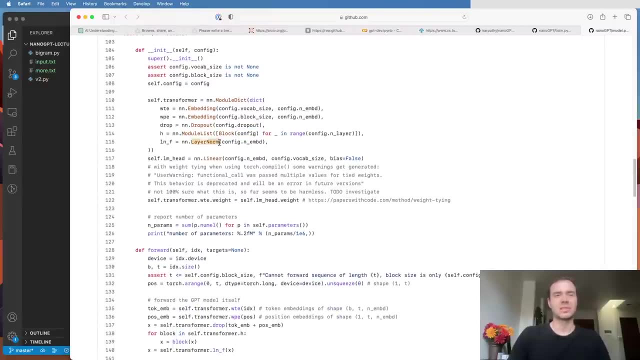 The blocks of the transformer are identical: the communicate and the compute phase, as we saw, And then the GPT will be identical. We have the position encodings, token, encodings, the blocks, the layer norm. at the end, the final linear layer. 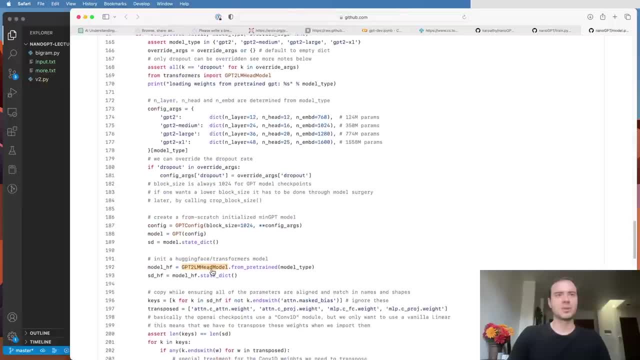 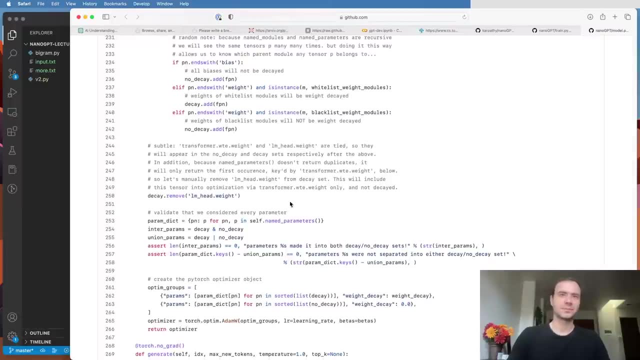 And this should look all very recognizable. And there's a bit more here because I'm loading checkpoints and stuff like that. I'm separating out the parameters into those that should be weight decayed and those that shouldn't, But the generate function should also be very, very similar. 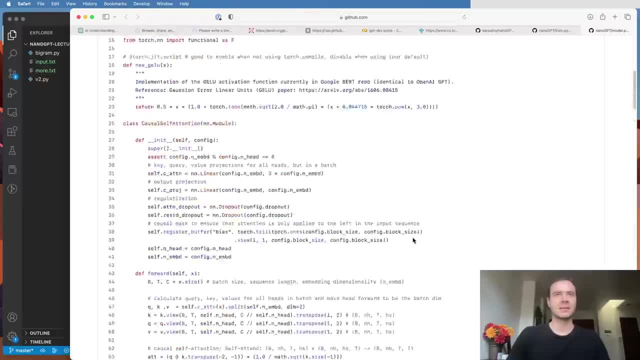 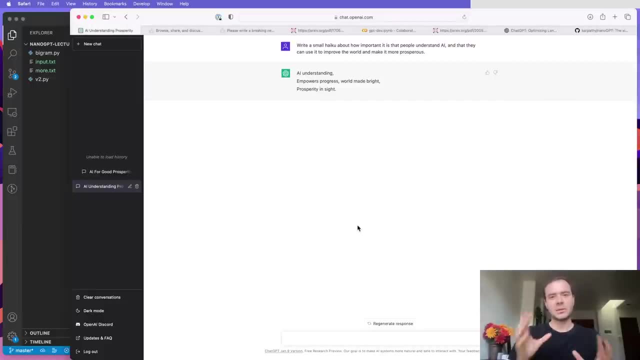 So a few details are different, but you should definitely be able to look at this file and be able to understand a lot of the pieces now. So let's now bring things back to ChatGPT. What would it look like if we wanted to train ChatGPT ourselves? 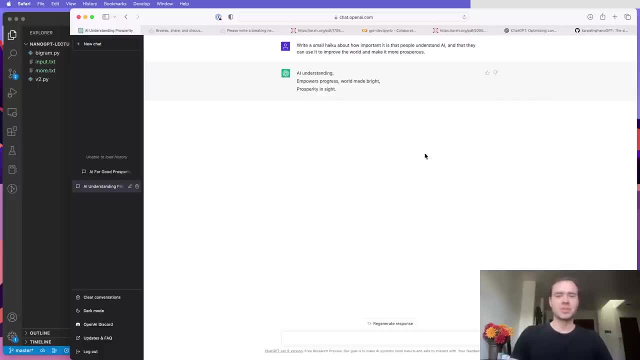 And how does it relate to what we learned today? Well, to train ChatGPT, there are roughly two stages. First is the pre-training stage and then the fine tuning stage. In the pre-training stage, we are training on a large chunk of. 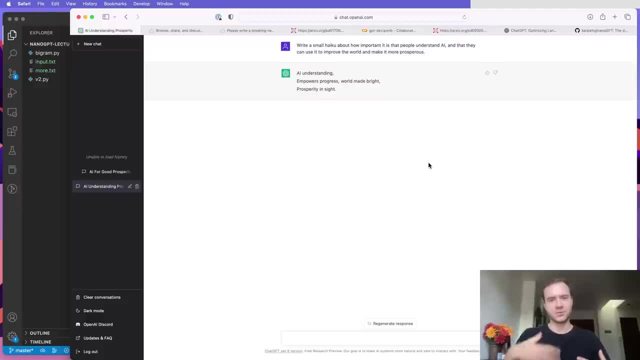 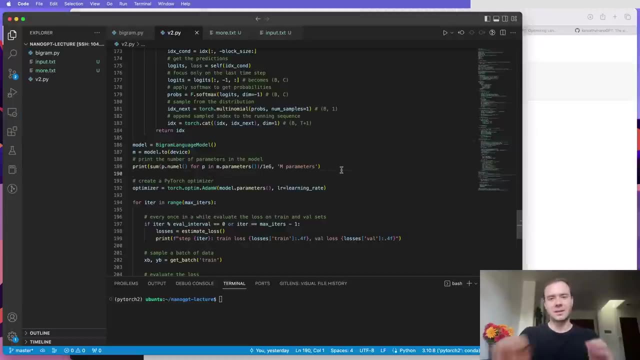 internet and just trying to get a first decoder-only transformer to babble text. So it's very, very similar to what we've done ourselves, except we've done like a tiny little baby pre-training step. And so in our case, this is how you print a number of parameters. 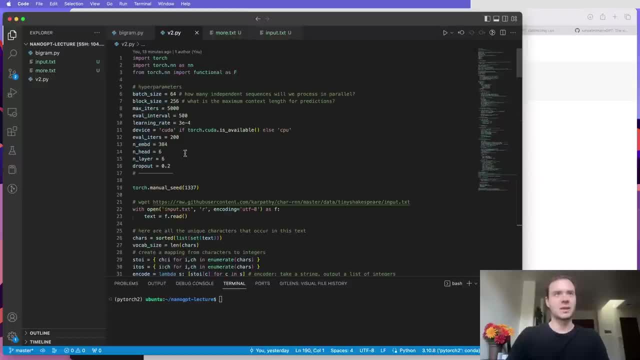 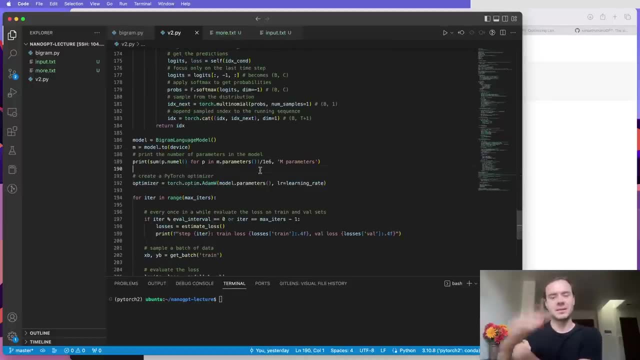 I printed it and it's about 10 million. So this transformer that I created here to create a little Shakespeare transformer, was about 10 million parameters. Our dataset is roughly 1 million characters, so roughly 1 million tokens. But you have to remember that OpenAI uses different vocabulary. 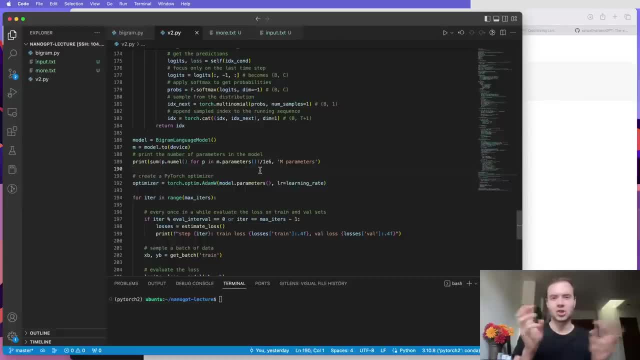 They're not on the character level. They use these subword chunks of words, And so they have a vocabulary of 50,000 roughly elements, and so their sequences are a bit more condensed. So our dataset, the Shakespeare dataset, would be probably around 300,000. 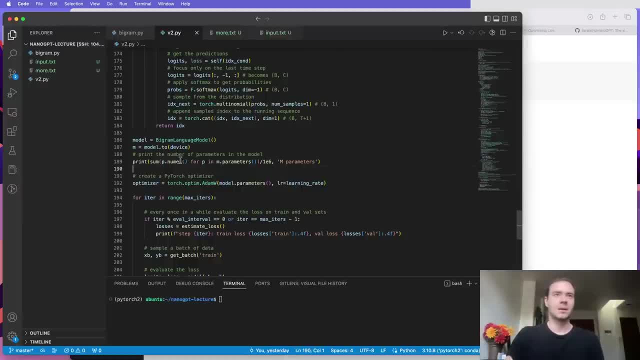 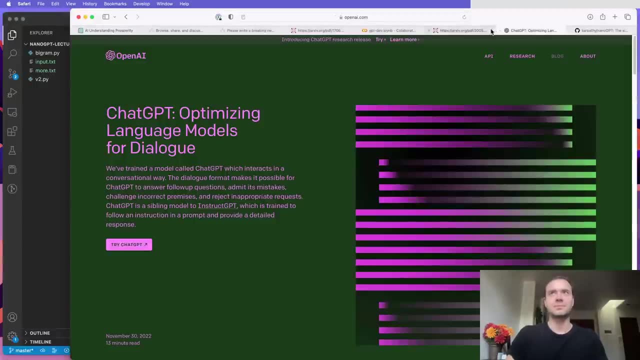 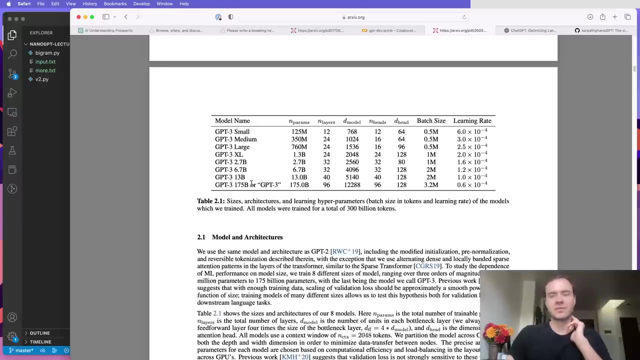 tokens in the OpenAI vocabulary, roughly. So we trained about 10 million parameter model and roughly 300,000 tokens. Now, when you go to the GPT-3 paper and you look at the transformers that they trained, they trained a number of transformers of different sizes. 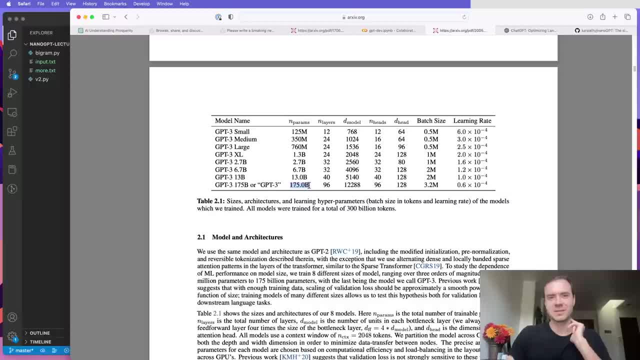 But the biggest transformer here has 175 billion parameters, So ours is again 10 million. They used this number of layers in the transformer. This is the N embed, This is the number of heads And this is the head size. 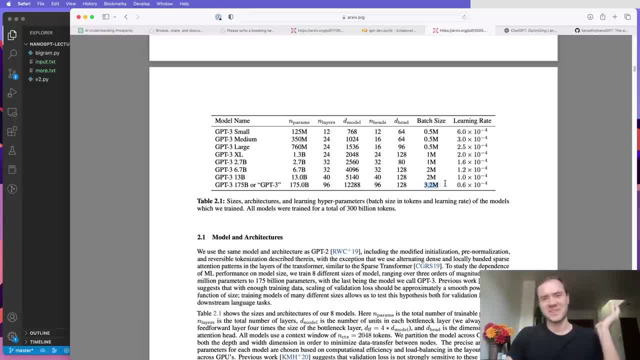 And then this is the batch size. So ours was 65.. And the learning rate is similar. Now when they train this transformer, they trained on 300 billion tokens. So again, remember, ours is about 300,000.. So this is about a million fold increase. 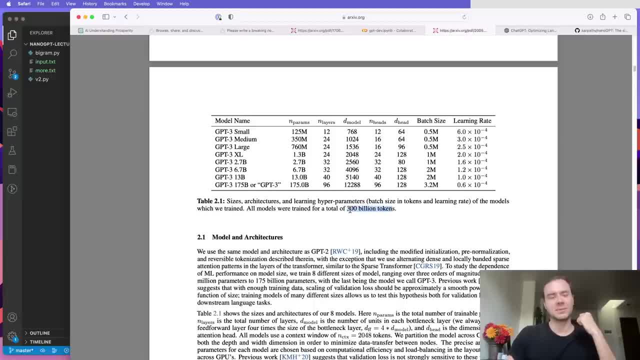 And this number would not be even that large by today's standards. So you'd be going up one trillion and above. So they are training a significantly larger model on a good chunk of the Internet, And that is the pre-training stage. But otherwise these hyperparameters should be fairly recognizable to you. 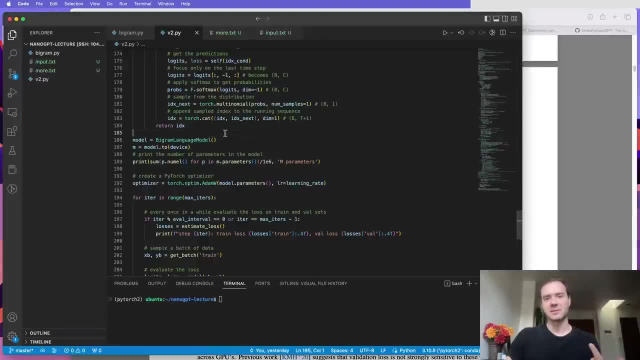 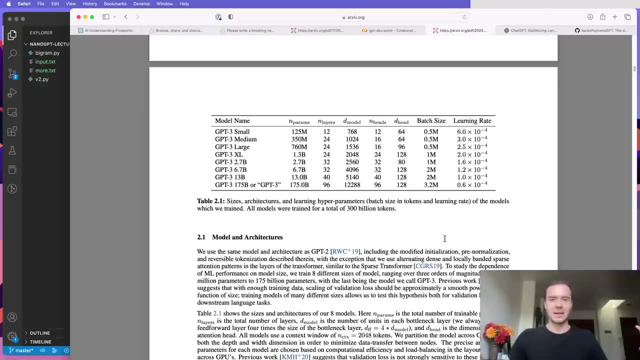 And the architecture is actually nearly identical to what we implemented ourselves. But of course, it's a massive infrastructure challenge to train this. You're talking about, typically, thousands of GPUs having to talk to each other to train models of this size. So that's just the pre-training stage. 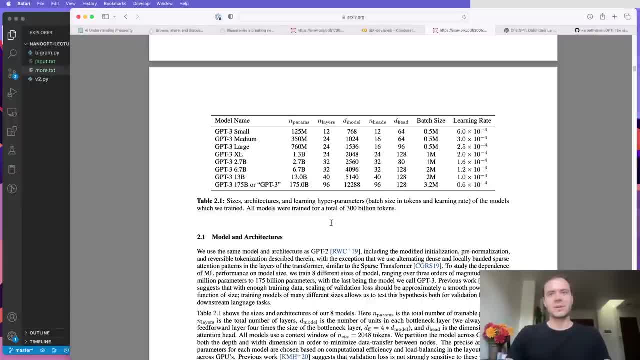 Now, after you complete the pre-training stage, you don't get something that responds to your questions with answers And it's not helpful, and et cetera. You get a document completer right, So it babbles, but it doesn't babble Shakespeare. 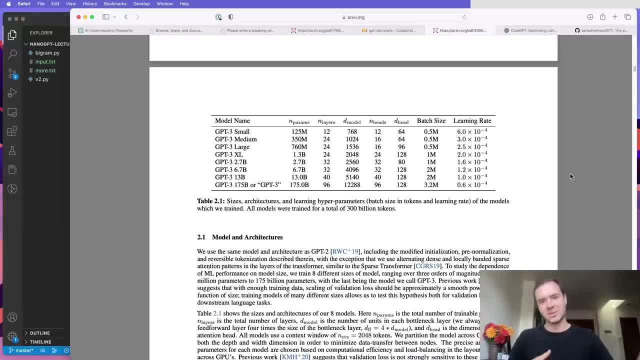 It babbles Internet. It will create arbitrary news articles and documents and it will try to complete documents because that's what it's trained for: It's trying to complete the sequence. So when you give it a question, it would just potentially just give you more questions. 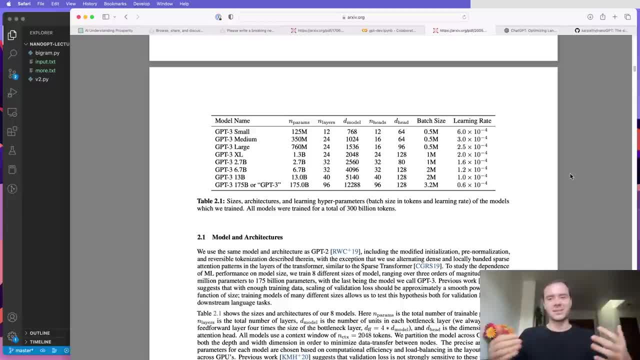 It would follow. It would more questions. It will do whatever it looks like some closed document would do in the training data on the Internet, And so, who knows, you're getting kind of like undefined behavior. It might basically answer two questions with other questions. 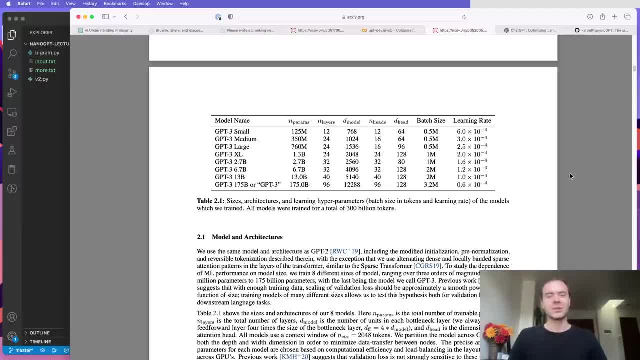 It might ignore your question, It might just try to complete some news article. It's totally unaligned, as we say. So the second fine tuning stage is to actually align it to be an assistant, And this is the second stage. And so this ChatGPT block post from opening. 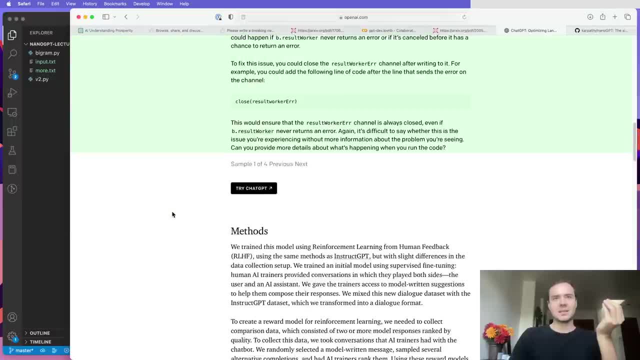 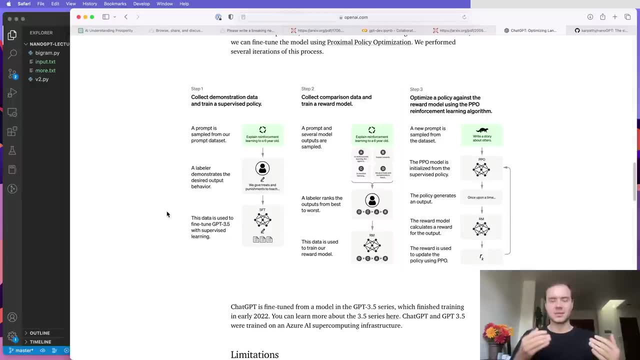 AI talks a little bit about how the stage is achieved. We basically there's roughly three steps to this stage. So what they do here is they start to collect training data that looks specifically like what an assistant would do. So there are documents that have the format where the question is on top and 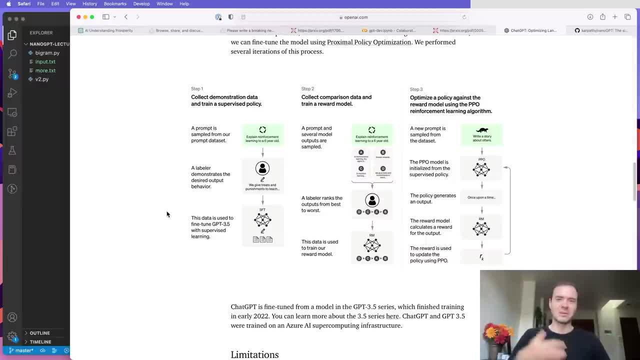 then? an answer is below. and they have a large number of these. That's probably not on the order of the Internet. This is probably on the order of maybe thousands of examples, And so they. They then fine tune the model to basically only focus on documents that look like that. 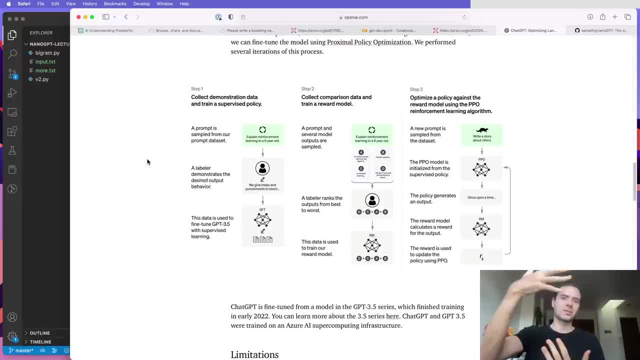 And so you're starting to slowly align it. So it's going to expect a question at the top and it's going to expect to complete the answer. And these very, very large models are very sample efficient during their fine tuning, So this actually somehow works. 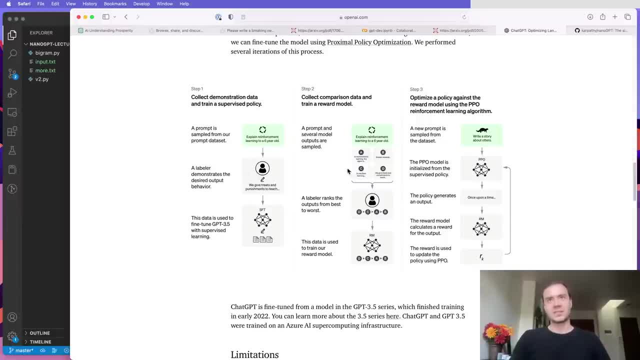 But that's just step one, That's just fine tuning. So then they actually have more steps where OK. the second step is you let the model respond and then different raters look at the different responses. You rank them for their preference as to which one is better than the other. 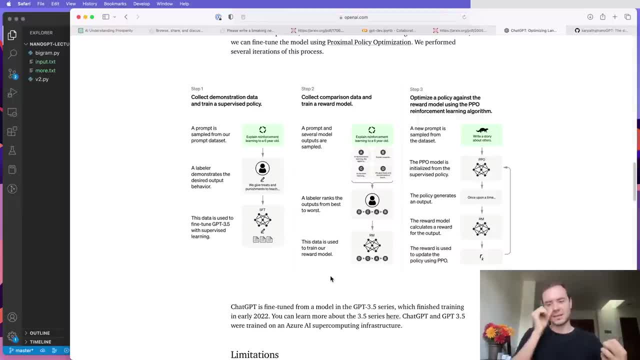 They use that to train a reward model so they can predict, basically using a different network, how much of any candidate response would be desirable. And then, once they have a reward model, they run PPO, which is a form of policy gradient reinforcement learning optimizer, to fine tune this sampling policy. 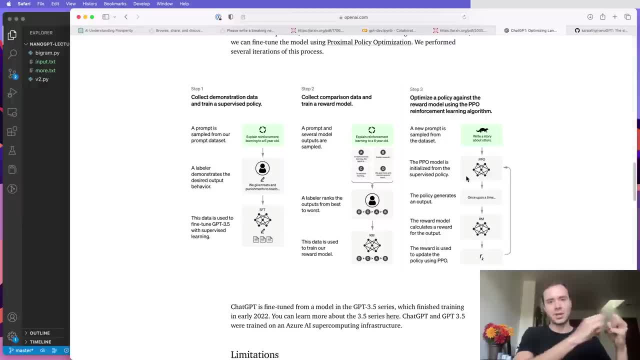 so that the answers that the chat GPT now generates Are expected to score a high reward according to the reward model, And so basically there's a whole aligning stage here, or fine tuning stage. It's got multiple steps in between there as well. 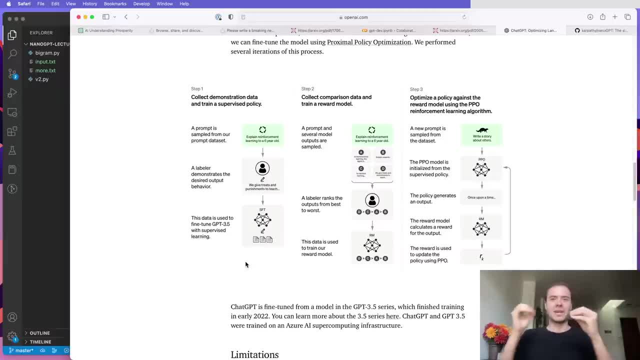 And it takes the model from being a document completer to a question answer And that's like a whole separate stage. A lot of this data is not available publicly. It is internal to OpenAI and it's much harder to replicate this stage. 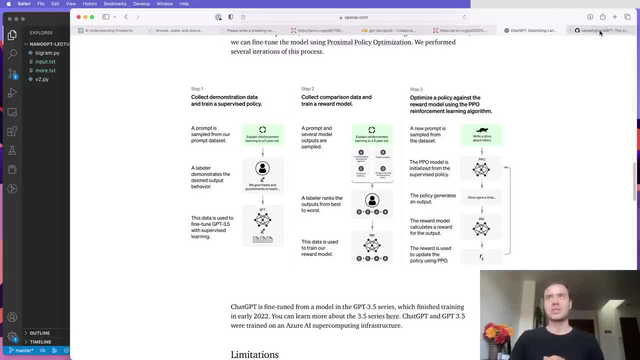 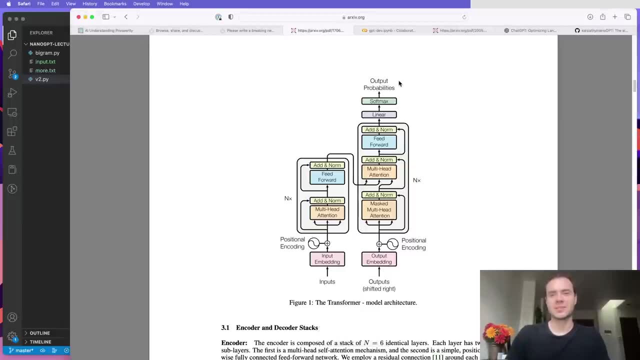 And so that's roughly what would give you a chat. GPT and nano GPT focuses on the pre-training stage. OK, and that's everything that I wanted to cover today. So we trained- to summarize- a decoder only transformer, following this famous paper. 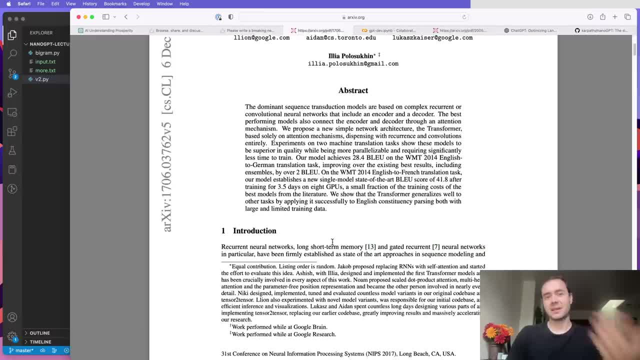 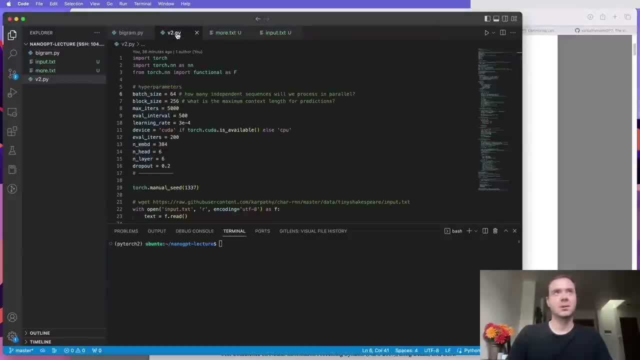 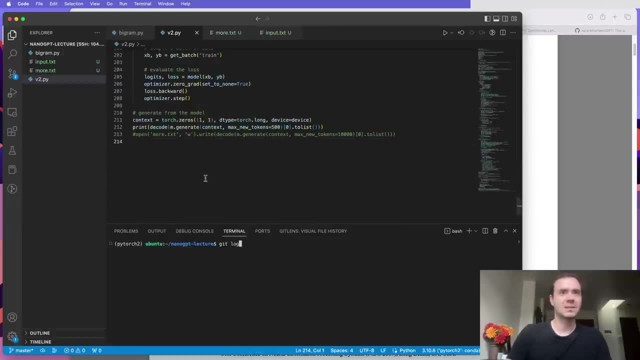 Attention is all you need from 2017.. And so that's basically a GPT. We trained it on a tiny Shakespeare and got sensible results. All of the training code is roughly 200 lines of code. I will be releasing This code base. 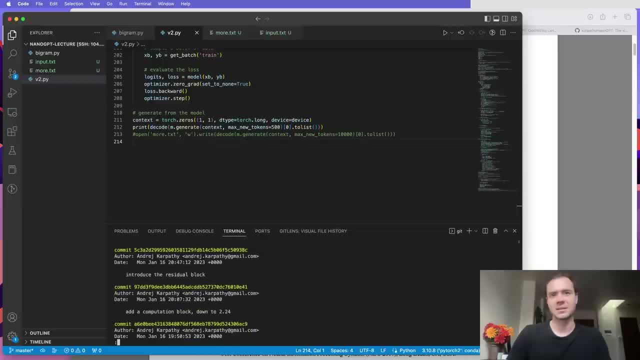 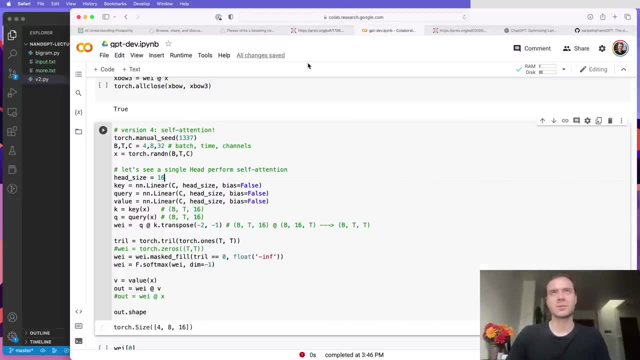 So also it comes with all the Git log commits along the way as we built it up. In addition to this code, I'm going to release the notebook- of course, the Google Colab, and I hope that gave you a sense for how you can train. 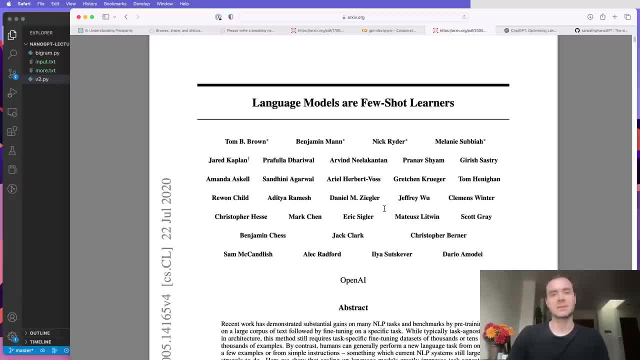 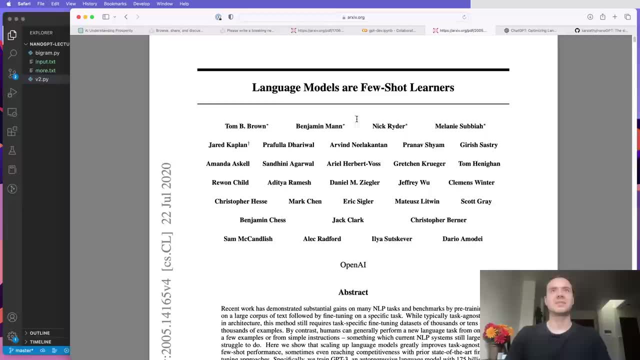 these models, like, say, GPT-3, that will be architecturally basically identical to what we have, but they are somewhere between ten thousand and one million times bigger, depending on how you count, And so that's all I have for now. 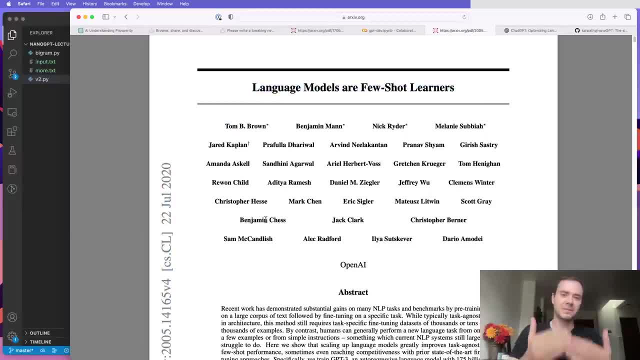 We did not talk about any of the fine tuning stages that typically go on top of this. So if you're interested in something that's not just language modeling but you actually want to, you know, say, perform tasks, or you want them to be aligned in a specific way, or you want 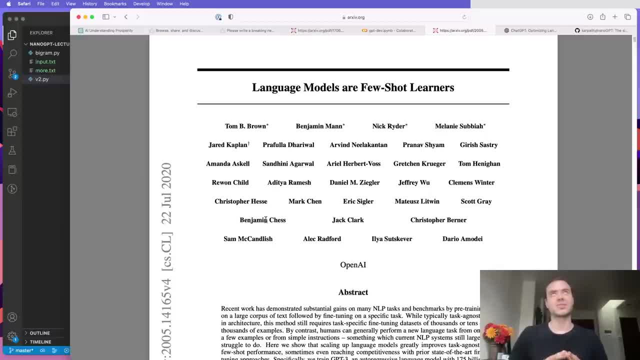 to detect sentiment or anything like that. Basically, any time you don't want something that's just a document completer, you have to complete further stages of fine tuning, which we did not cover, And that could be simple, supervised fine tuning, or it can be something more fancy. 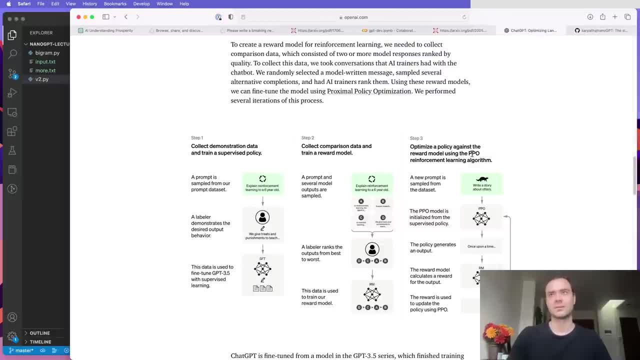 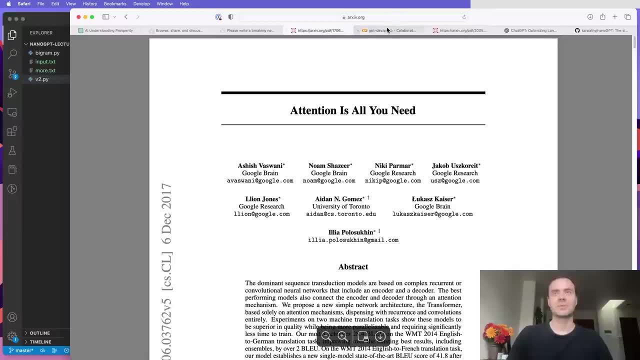 like we see in ChaiGPT, we actually train a reward model and then do rounds of PPO to align it with respect to the reward model. So there's a lot more that can be done on top of it. I think for now we're starting to get to about two hours mark. 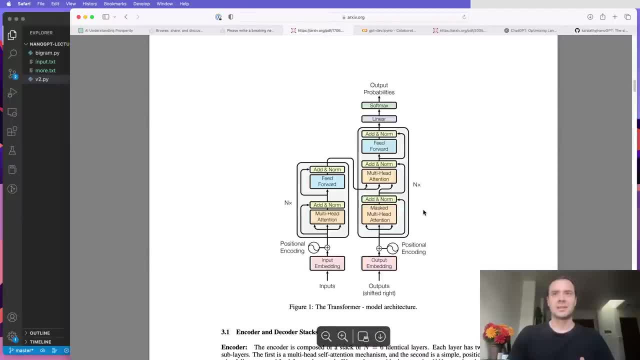 So I'm going to kind of finish here. I hope you enjoyed the lecture and, yeah, go forth and transform. See you later. 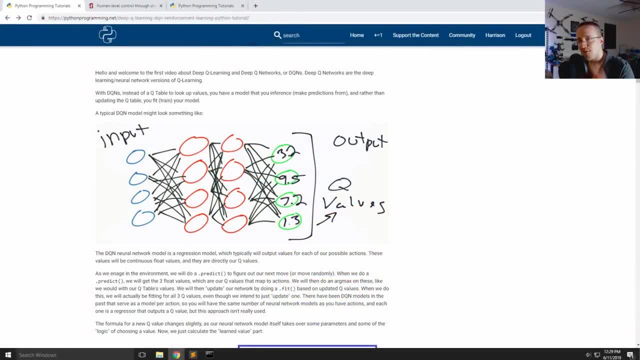 What's going on, everybody, and welcome to part five of the reinforcement machine learning series. In this video and subsequent videos, we're going to be talking about deep Q learning, or DQNs or deep Q networks, And to start the prerequisites. if you don't know deep learning, stop. 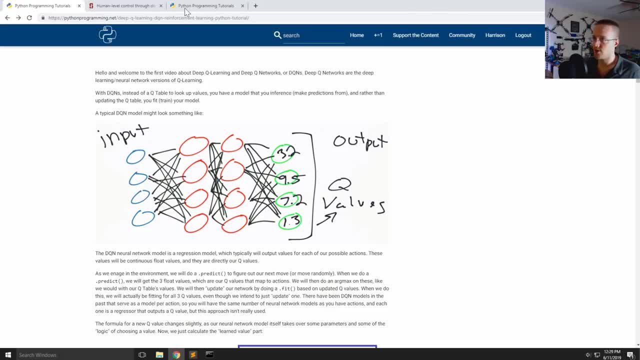 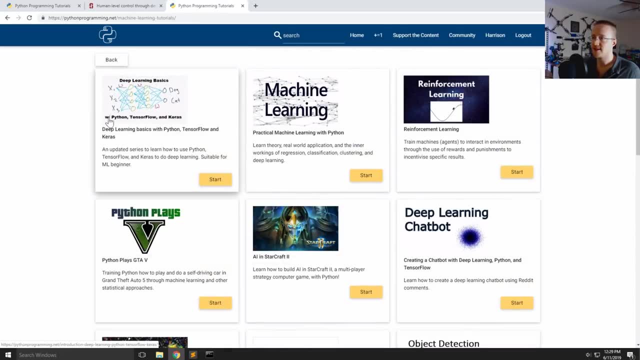 pump the brakes. You got to learn deep learning. So if you want, you can go to the homepage of pythonprogrammingnet, click on the machine learning here and then do this: deep learning basics with Python, TensorFlow and Keras. At least do like the first two tutorials I want to